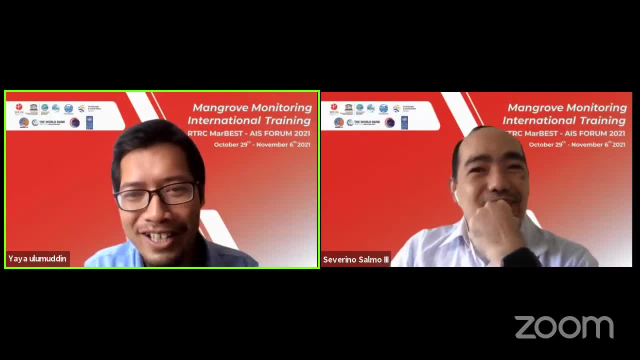 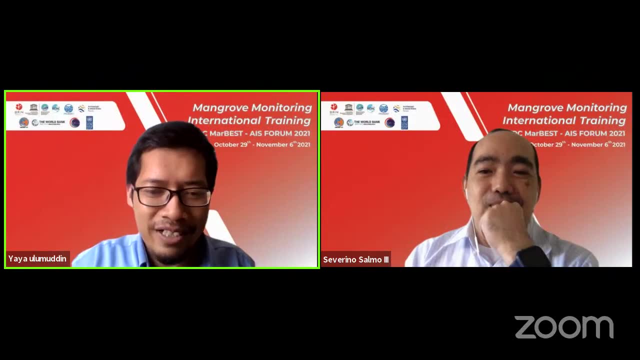 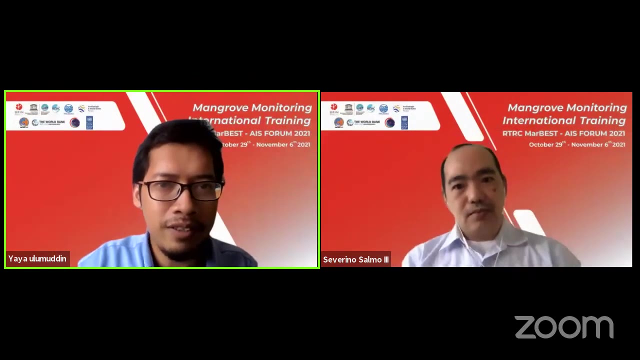 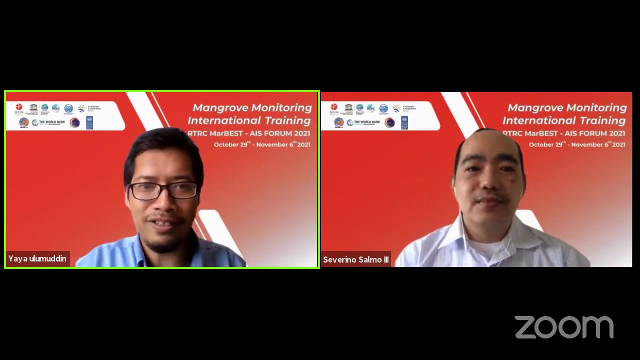 Good afternoon and good night for everybody across the world. So today we have Dr Severino Salmo from the Philippines. Sorry, I forgot to open your personal data, So I don't remember all the things about your curriculum today. Okay, It's better if I read your bio, but not all the information on it. 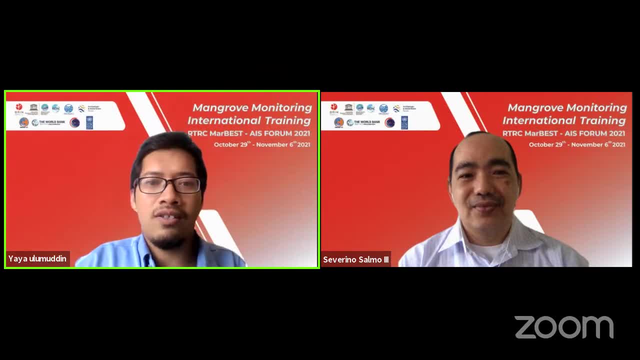 So his name is Severino G Salmo. He is from the Philippines. He got his PhD degree from the University of Queensland, Brisbane, Australia. His thesis is about early post-typhoon effects on the restoration trajectory of planted mangroves. 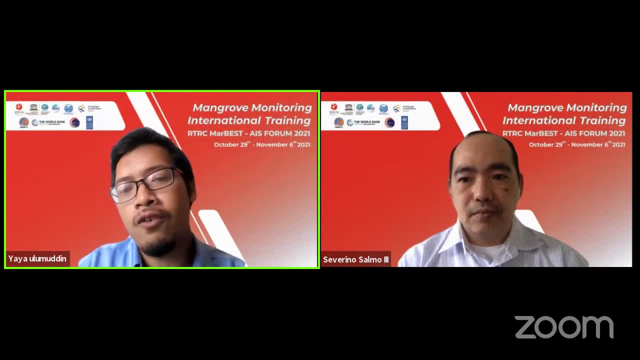 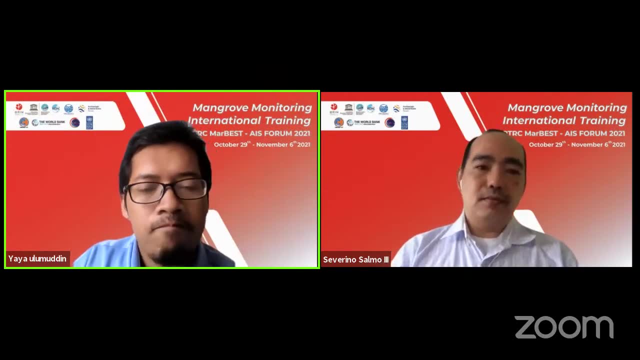 implications for forest development and macrofauna communities. And then he has been doing many research related to mangroves, Like comparative blue carbon assessment in conserved versus disturbed seagrass, in machine-locked- sorry- in seagrass. And then 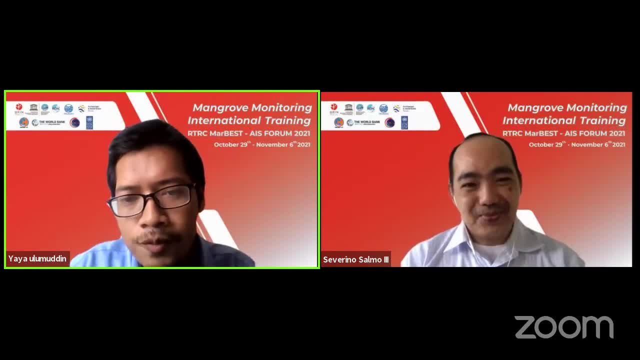 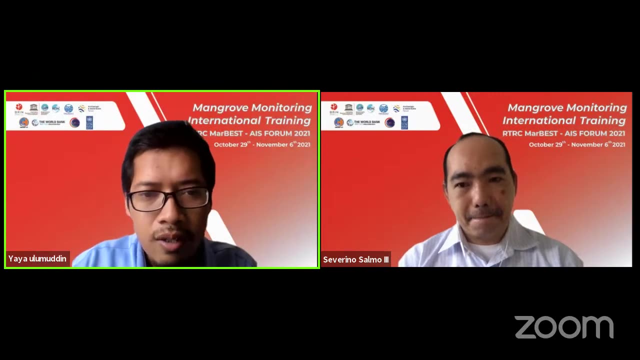 Oh, this one. Development of new ecological studies of mangroves by using metagenome barcoding And then comparative analysis among disturbed, restored and natural mangrove stands in the vulnerability and adaptability against climate change. Blue carbon initiative technique consultancy. 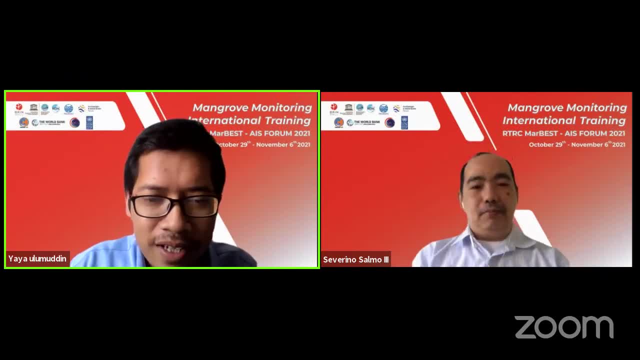 And, Ah, this one, Enhancements of Philippines research capability in understanding the rule of mangrove ecosystem health in the adaptations and mitigation against natural disasters. So I think from his research background we know that he, he, he. I think he has been very informative, very doing, very worthwhile and valuable speakers today. 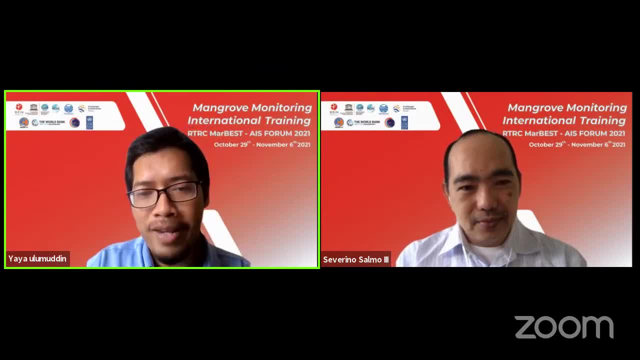 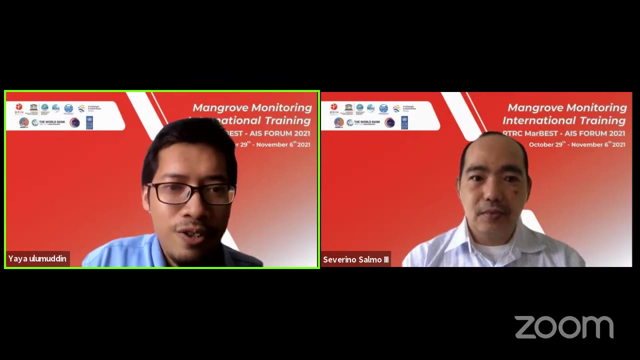 And so very related with this training. Particularly, We are going to talk about mangroves. Especially we are going to talk about, about data and mangrove health and et cetera. So today the time is yours, Dr. 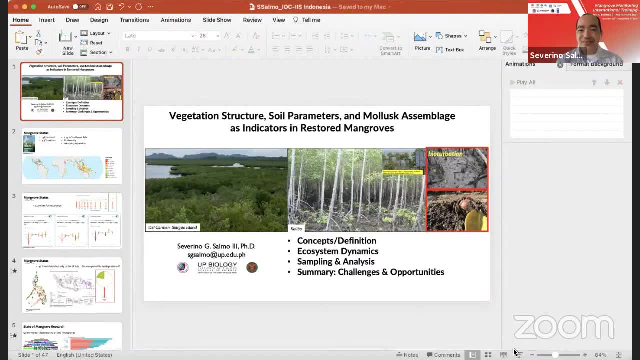 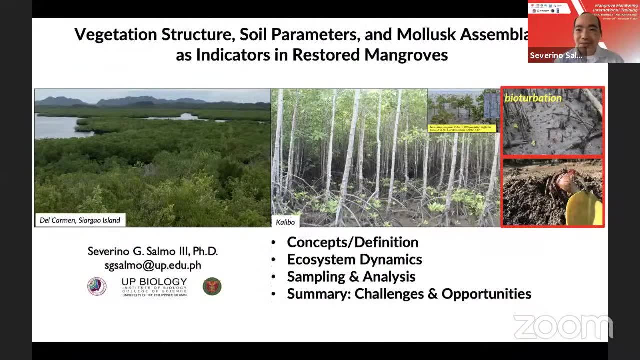 it must a great presentations and valuable for us, please, sir. yeah, hello, good afternoon i'm. i'm trying to show my powerpoint file. yes, clear, is it clear? now clear, and my my audio is clear. okay, very good, all right. um, good afternoon fellow southeast asian, our neighbor from indonesia. 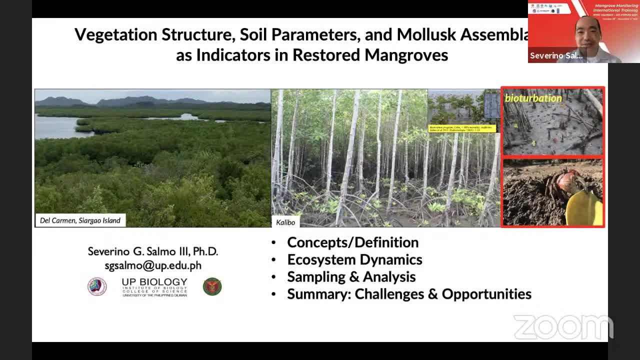 and uh, i'm very honored to have your time for today. i just did a quick browse of the programs that you are intending to do within this uh training period. i actually tried to attend the gee session this morning and before my talk i i heard some of you talking about it. 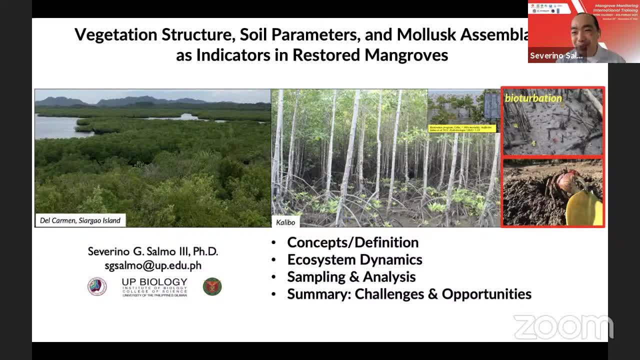 about the dee, so don't worry about it. i'm, i want to learn dee, but i'm also traumatized with the, with the coding and uh, you, you said, you even said python. those are very intimidating terms for me. i do r, i i like r, but uh, your training this, uh, this morning, definitely is very, very interesting. 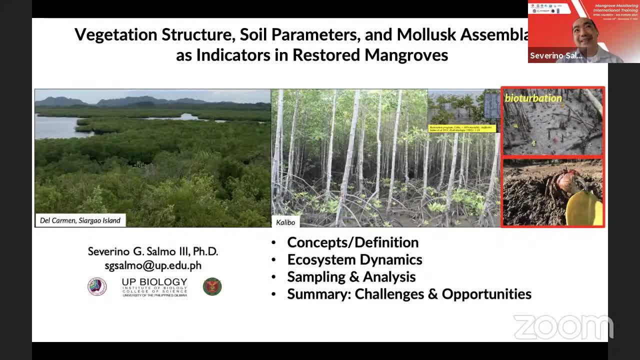 and uh, that's why i also tried to attend uh the session, but i wasn't. i wasn't able to finish it, um. but yeah, i definitely agree it's. it's really very important, as uh introduced by uh yaya. um, i'm an ecologist and specifically, i'm a restoration. 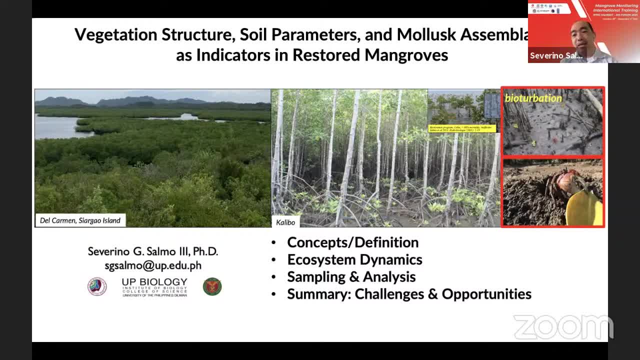 most of my studies are obviously implemented here in the philippines, but i do have collaborative works with a malaysian fellow, i don't know if you know. uh, dr aldri amir and i collaborated with several indonesian fellows. uh, i can name a few, um. 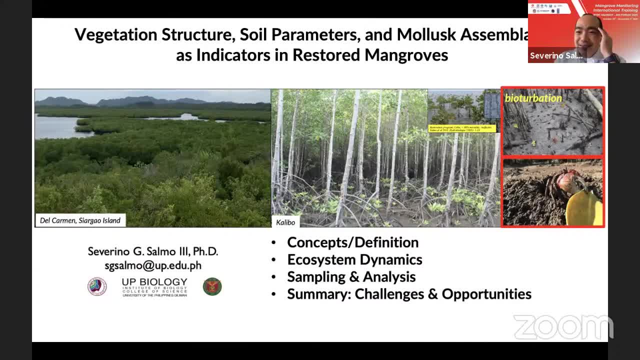 maybe you know dr frida siddiq and, of course, yeah, yeah, uh, also with the novi uh and several other guys who i worked with in the past for the genetics and e-dna. uh, yeah, i already mentioned about my interests and it's all about restoration, ecology, the, the research designs, the. 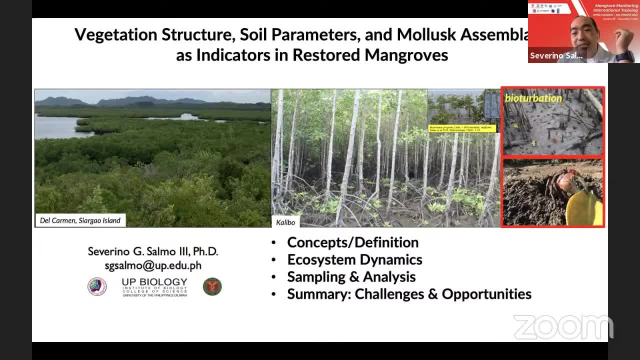 monitoring and so on and so forth. for this session i'll be presenting very briefly about the some concepts on restoration ecology and and i hope that will be a good complement for your training this week. it's about complementing the restoration ecology to those of the tools that you are trying to learn for the weeks, so i'll be presenting some basic concepts. 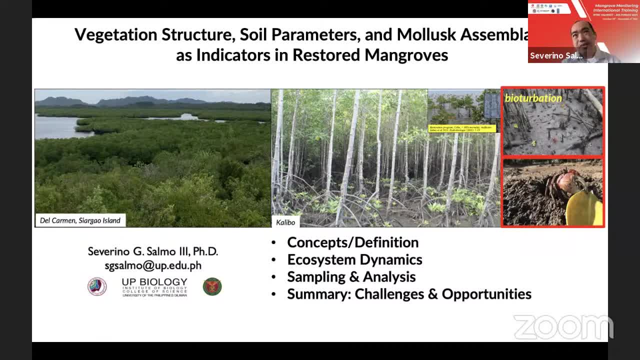 what is restoration? what is restoration ecology? how do an intact system, uh, manage or conserve or restored? what about the restored system? how do the restored system meet the restoration goals or targets? then i'll be presenting a bit about the sampling and analysis, mainly my experience. we won't have the time to do the actual analysis. more so, if you talk about the actual sampling etc. 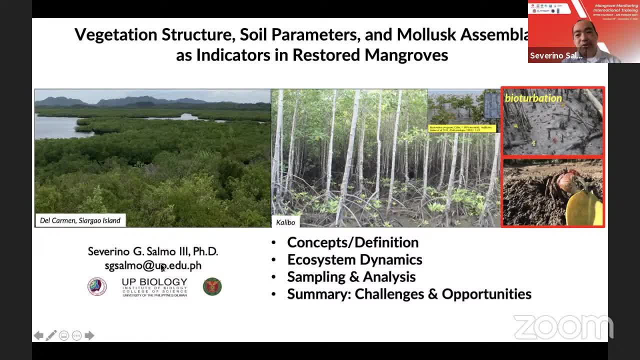 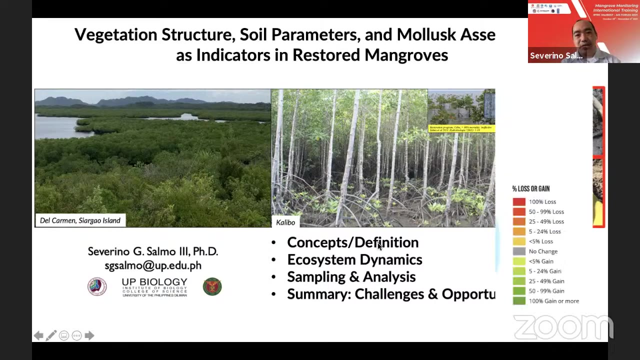 but uh, here is my email ad. if you have concerns later on, uh feel free to contact me and uh, hopefully, towards the end i'll be presenting some challenges and uh opportunities for mangrove restoration ecology, not just for the philippines, but especially for southeast asian context. so before i go into concepts on restoration, allow me to present this very recent report from: 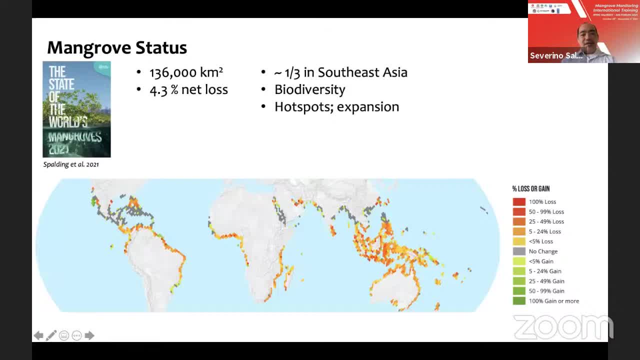 spalding et al about the state of the world's mangroves 21- i think it was released just less than two months ago or maybe just last month- wherein the world at the moment has around 136 000 square kilometer and through the years there was a net loss of around 4.3 percent. most of these are found in 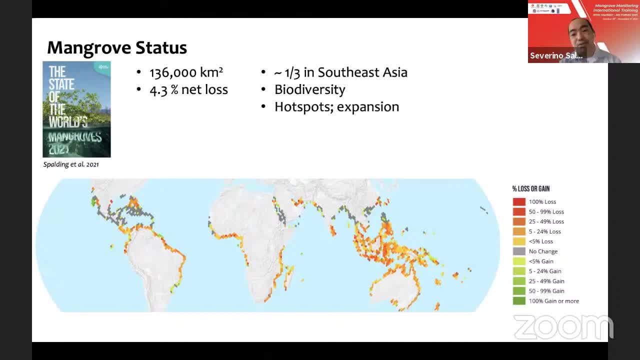 southeast asia, mainly in in indonesia and malaysia. in the past, philippines has a good contribution with the mangrove cover in southeast asia. now it's declining, but nonetheless the mangroves in southeast asia occupy around one-third, or maybe even higher than that, for the entire world. 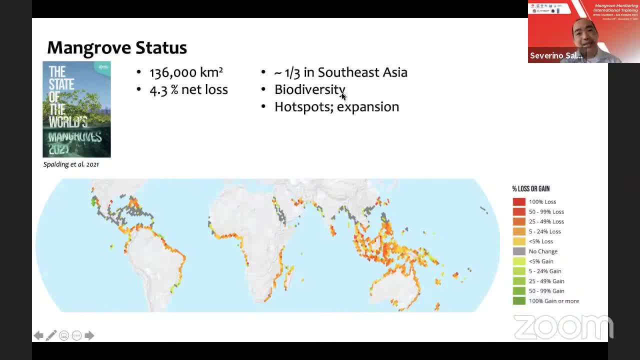 and those mangroves are known for biodiversity. unfortunately, that's also the sites and i hope you will agree with me: although we have the largest mangrove cover, that is also the site we have the highest mangrove losses and in this report there was a mention that. in general, 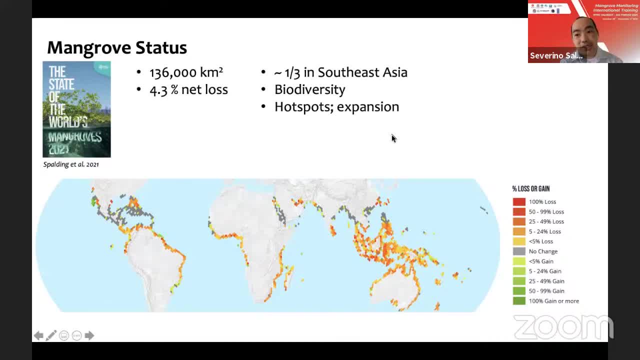 there are some areas that there are expansion of mangroves, meaning mangroves have expanded from their current limit, so some of it will actually grow bigger in terms of area. but there's this net loss and if you look at the map from spalding et al, those orange yellows are those mangroves that experience losses. so in 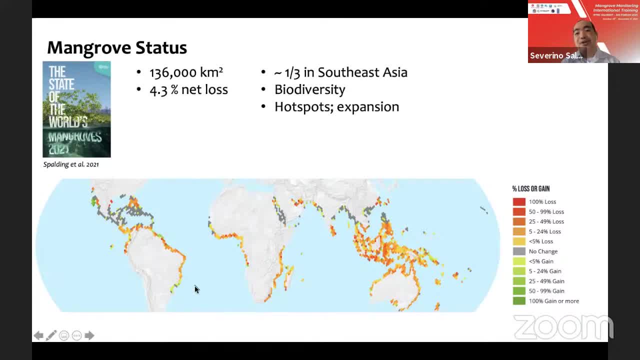 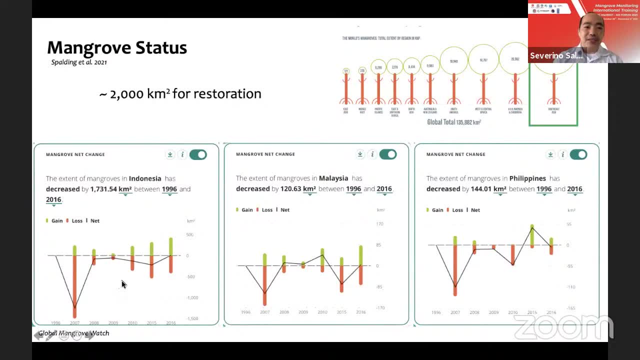 some places there are expansion, but in our region there are actually more losses. now, uh, out of that figures, this is forget. this is indonesia, this is malaysia, then this is philippines. um, out of the estimated mangrove areas in the region, it's around 2 000 square kilometer- are potential restoration areas. that's a lot. it's even bigger. 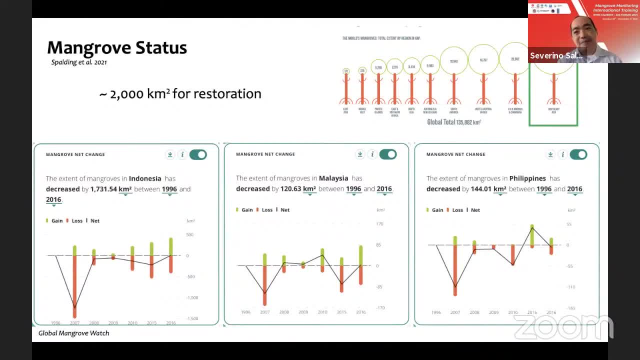 than one entire crown tree. if you sum it up, and where can we do the restoration? uh, you have in the case of indonesia, you lost a lot. same thing with that with philippines and and malaysia. but if you will compare the scale, uh, it's, it's mainly because you have wider mangrove areas. and if you 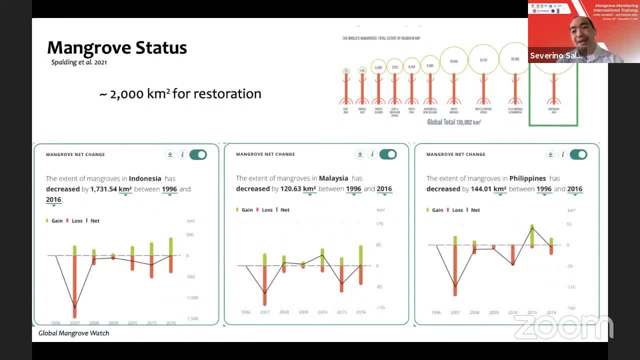 uh, if you have the degraded mangroves and therefore that degraded mangroves will also be the same site, that could be a good candidate for restoration. so i'm saying this because you know that, uh, 2021 to 2030 is the decade of restoration, so maybe 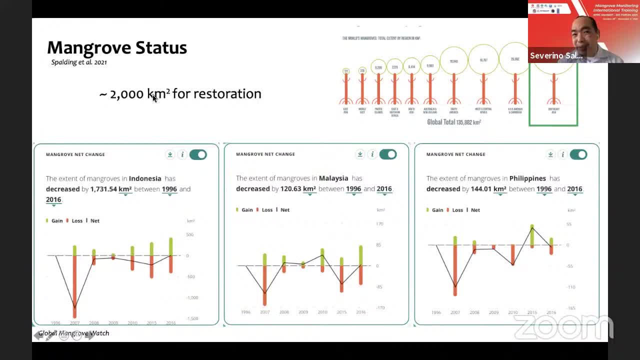 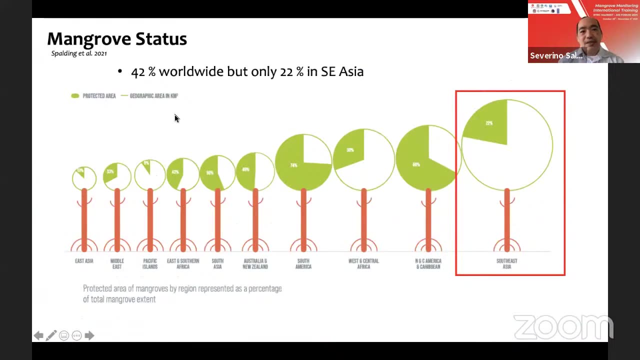 year 2030. maybe this will be reduced, because i hope at least more than 50 percent of it will already be restored by 2030, hopefully, so. think about these figures. um, most mangroves in the world- uh, it's almost 50 percent worldwide. those mangroves are already. 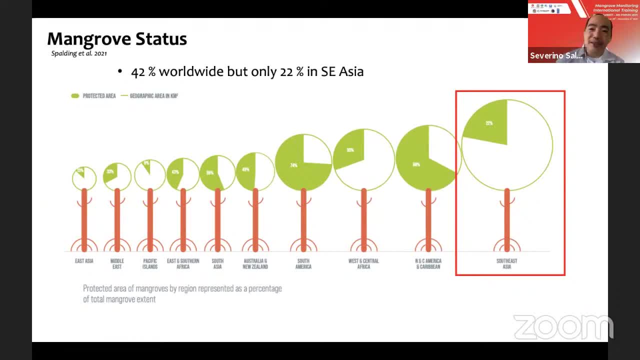 declared as a protected area, maybe a mangrove protected area or a key biodiversity area or key protected area- there are several terms. but if you look at the figures worldwide, yes, it's very good to see 42 percent, but in southeast asia only 22 percent of it is declared as a protected area, so less than one half of the total mangrove. 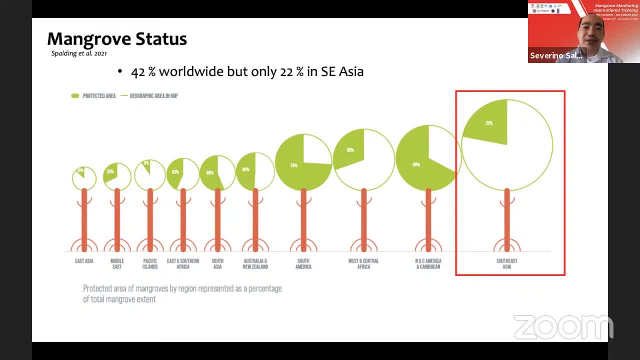 protected area, now, assuming those are already protected, in the case of the philippines, for example? um, yes, we do have mangrove protected areas, but it's not evenly distributed. some of it are actually not protected at the moment, but, yes, maybe one third of it is already protected. 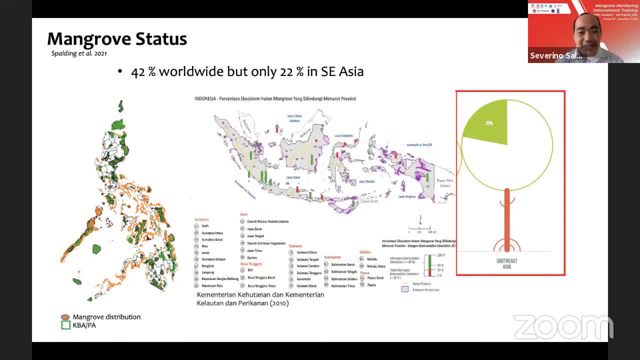 now. um, i got this slide from dr sidik and this shows the distribution of protected area for indonesia. i think we have a similar case. if you have a protected area, well we do have it, but not all of it. not all mangroves are protected, and even those that are already protected. 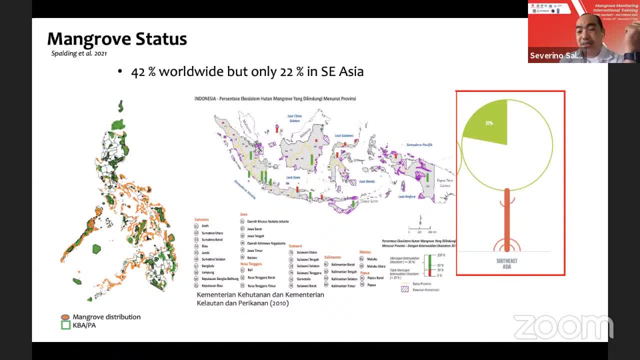 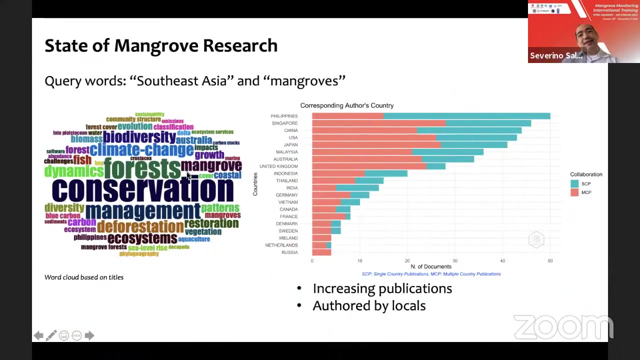 are actually subject to disturbances, various forms of disturbances. which leaves us to that question: are those mangroves that are protected areas really protected? if yes, then that's good, but if not, then maybe that would be a good candidate for restoration areas. right, and then i did a quick uh web of scholar- sorry, web of science- search, and i did a quick. 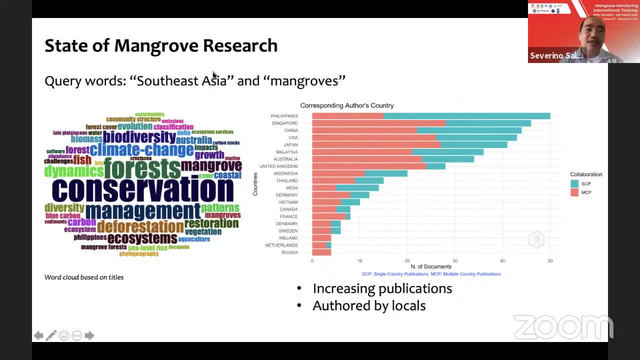 bibliographic search. uh, i used the words southeast asia and mangroves and then i did a quick bibliographic search and i ran, uh, different countries, southeast asian countries, and came up with this: uh trend, um, this is the number of papers that were published, if you look at it. philippines. 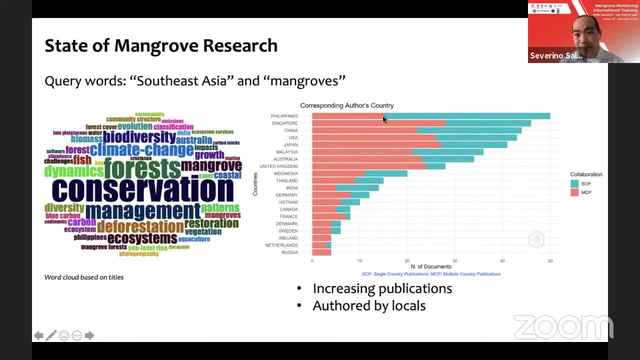 well, in in records, we do have higher number of papers published, but if you carefully look at it, uh, there were, there are more authors that are non-filipinos. i don't know if you can see my, my, my cursor. uh, singapore, there are more singaporeans, quote-unquote singaporeans, because there are. 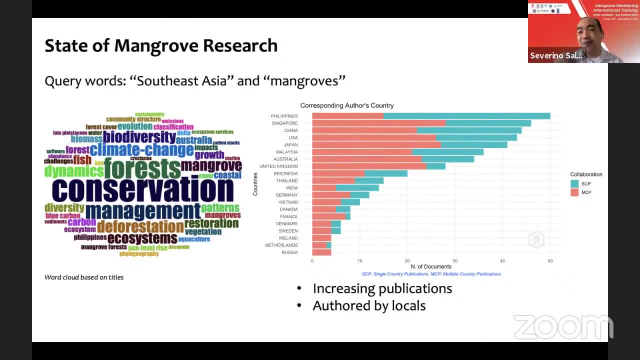 foreign workers who are affiliated with singaporean university, although they are not really singaporeans, right? uh, malaysia is doing good here. there are more malaysians who have more publications than foreign counterparts. uh, indonesia, almost even you have indonesian authors and at the same time, 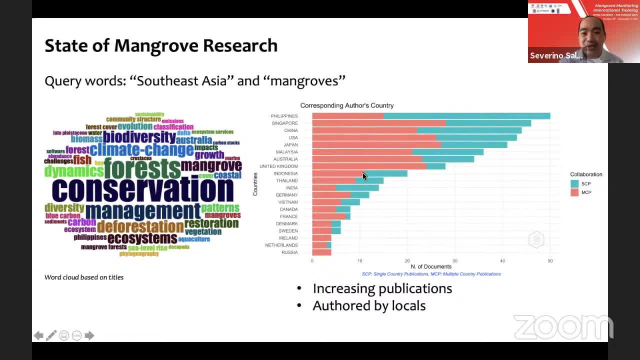 we outside NortheastTV non-Indonesian authors. Thailand is doing good And, I think, similar with Vietnam, All other Southeast Asian countries. there are very minimal publications But we see that there are interest in mangroves And I'd like to highlight here. 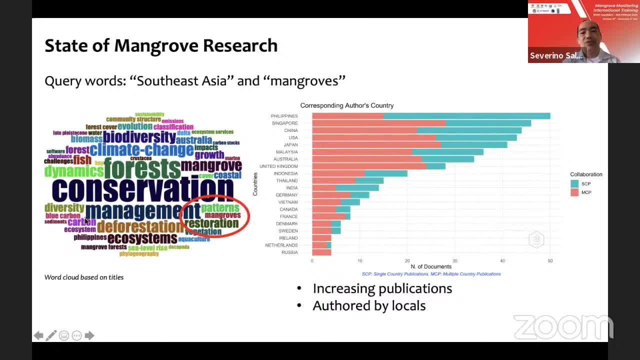 this is a word cloud based on titles. What are the common terminologies that are used in this publication? So there are so many things, but it's mostly about conservation, management And very recently, it's all about restoration, vegetation and patterns. 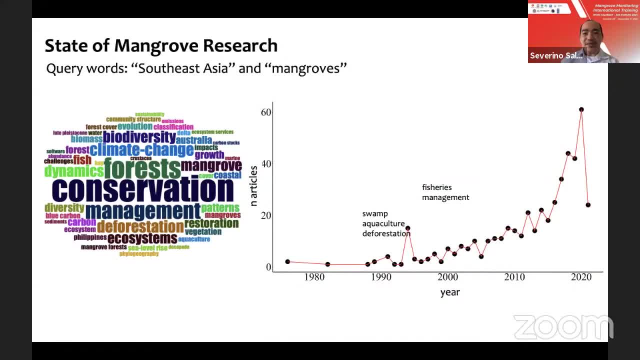 And that could be very interesting for us. Now I dig deeper and I try to analyze what are the interests in the region. So there could be several explanations. 1980s: it's like general mangrove ecology, It's like general mangrove forest, et cetera. 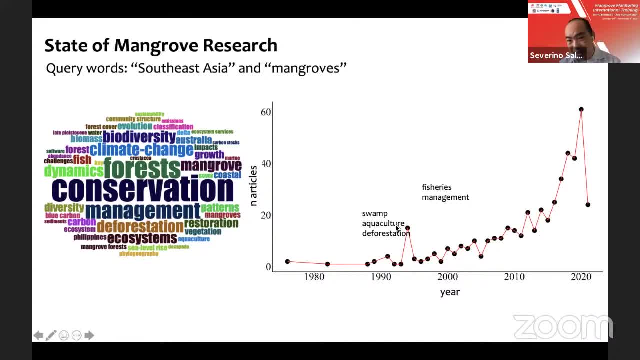 1990s there was a shift in interest about aquaculture and deforestation And you know that more than 80% of the mangrove losses in Southeast Asia, on the average, is attributed to aquaculture. We call it a fishpond. 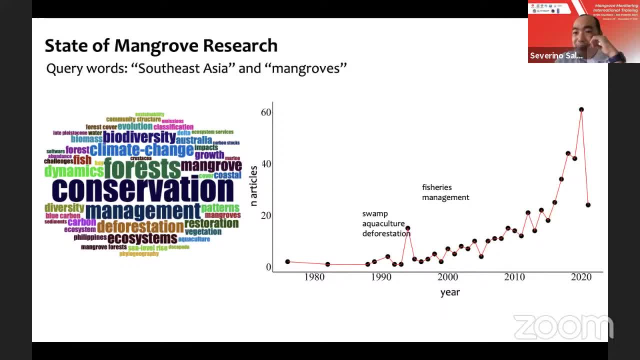 I think you're calling it tambak something. I don't know if I got it correctly. Yes, tambak, Tambak, all right. So 1990s, actually it started out as a fishpond. So 1990s: actually it started out as a fishpond. 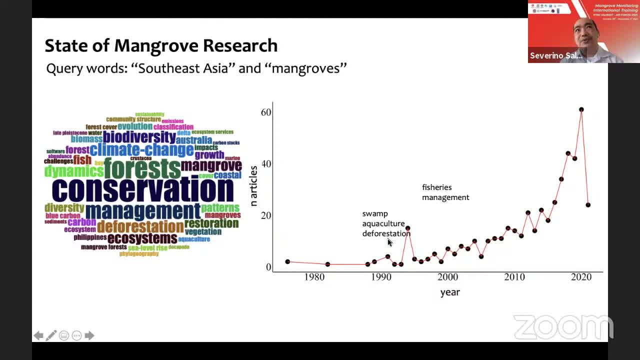 So 1990s. actually it started out as a fishpond, So it started 1970s But 1990s. we do recognize that we lost mangroves because of tambak And therefore, if we want to do restoration, 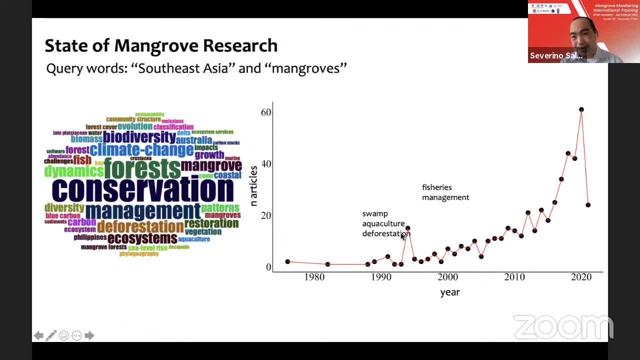 then we might need to do restoration in those tambak, in those fishpond area. Then year 2000,. it's all about realization of fisheries and the contribution of mangroves, about fisheries, mangrove management and so on and so forth. 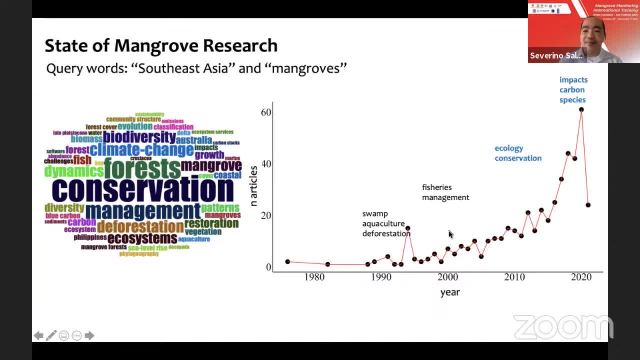 Now year 2010,. there was a shift about conservation And the interest on mangrove ecology in general because of the biodiversity studies and so on and so forth. In 2020, the interest now shifted about impacts, carbon sequestration, blue carbon. 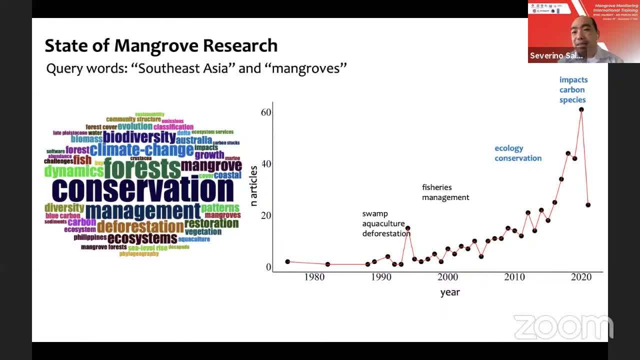 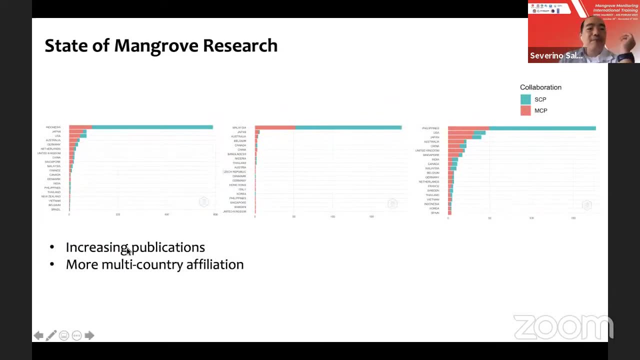 and species diversity. I think Indonesian scientists have contributed a lot about blue carbon publication. Now I dig deeper about the publications for Indonesia here, Malaysia and then Philippines. These are our collaborators. okay, So for Indonesia, most of your collaborators are mainly from Japan and Australia. 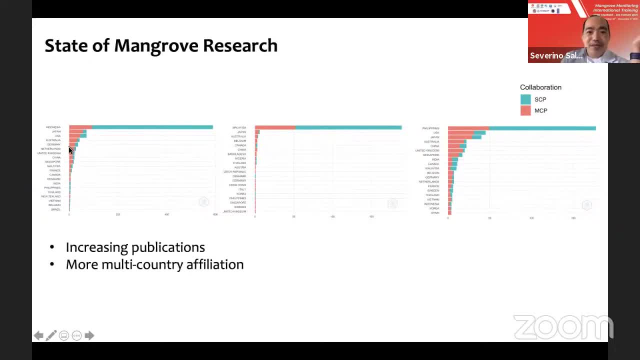 and some other countries like Germany, Europe For Malaysia it's mostly, I think, about 100,000 people, Mostly about Japan and Australia, very minimal from the US right Philippines. obviously we do have more collaboration with the US and Japan and to some extent 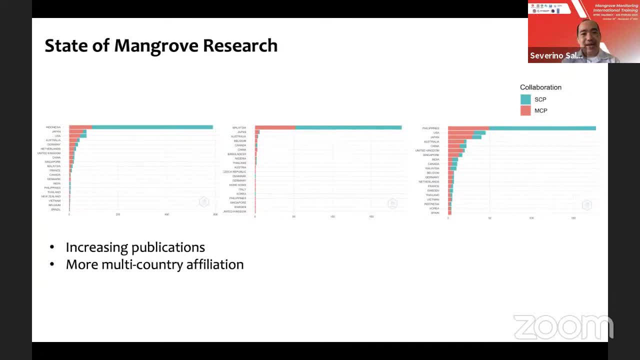 Australia and European countries. Now, why am I showing this slide? Because the you know, the interest on publication, interest on basic researches, will really be tied up with that target agenda, with that target agenda of the collaborators. For example, in 2010, there was this interest. 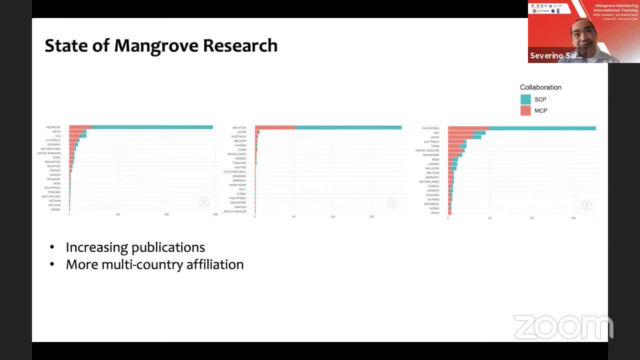 on biodiversity conservation and therefore the focus would be about conservation. Now, very recently, to some extent, sea level rise was mentioned, and therefore many people are doing researches on sea level rise. Now it's about blue carbon, climate change, adaptation. 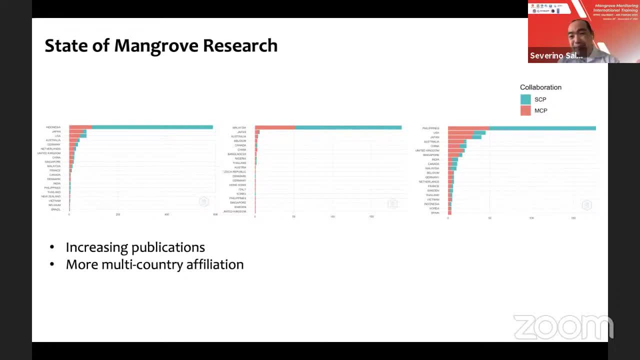 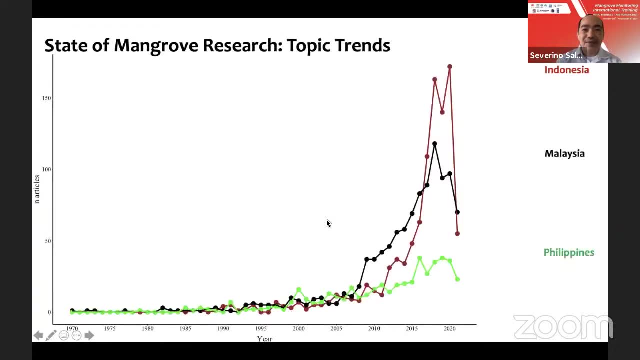 and mitigation and so on and so forth. Maybe next year we will have a discussion about that. Next year will be about COVID or something else. maybe right Now I did some analysis on what's the interest among Indonesia, Malaysia and Philippines. 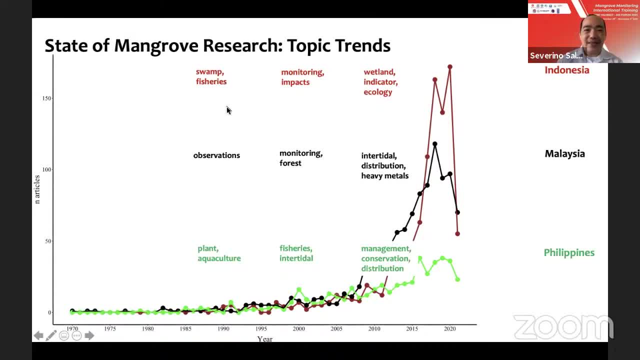 So here you have your different interests In 1990, you have this: You've been doing monitoring since that time, Year 2010.. You see this, You see this. We started about indicators and ecology. Malaysia, sorry, we do have some common trends. 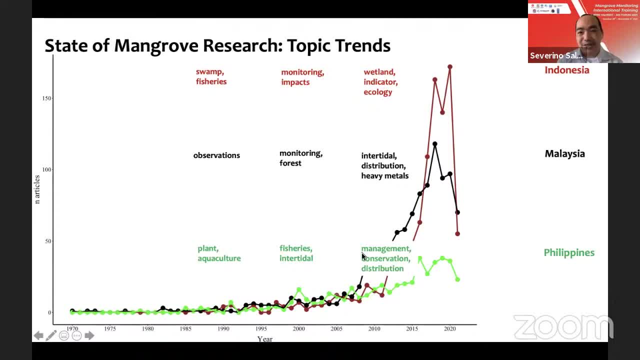 about monitoring fisheries, so on and so forth. conservation: To some extent we have similarities- I mean Indonesia and Philippines- about conservation, restoration and ecology. Malaysia: they have issues with plastics, microplastics, heavy metals and therefore their interest is quite 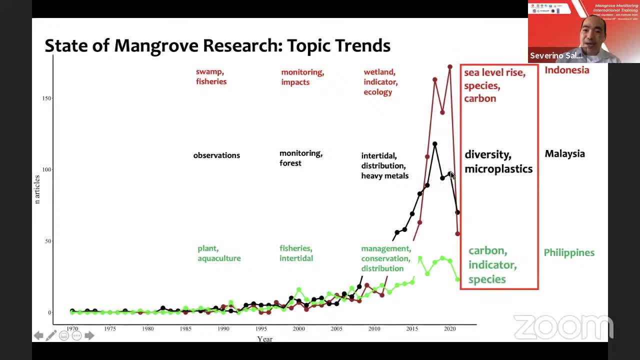 you know very high. They are really different. Now again, it's all about this common interest on climate change adaptation and mitigation indicators, species restoration and biodiversity right. So in the next coming years, this would be the emerging trends based on the research. 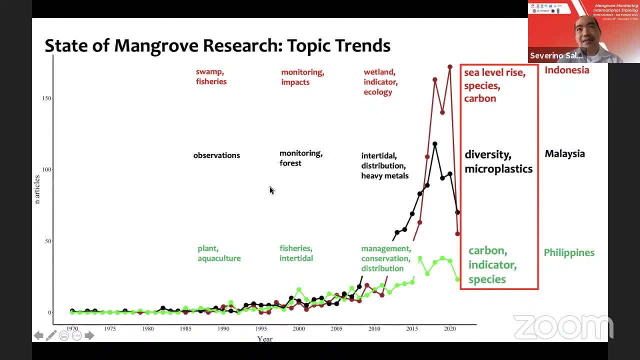 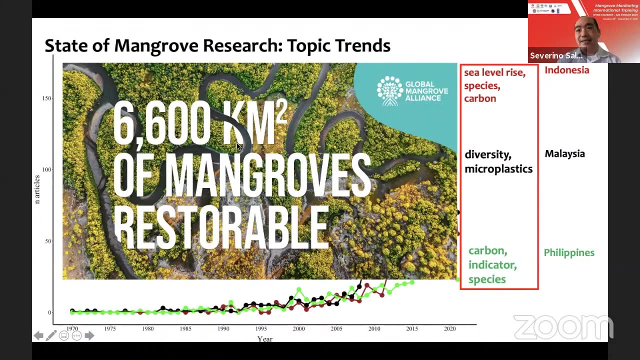 interests of Indonesia, Malaysia and Philippines, And this is a work in progress. I'm doing this with Dr Audrey Amir from Malaysia and Dr Siddiq from Indonesia. Okay, why am I showing this? Because Global Mangrove Alliance, the Global Mangrove Alliance. 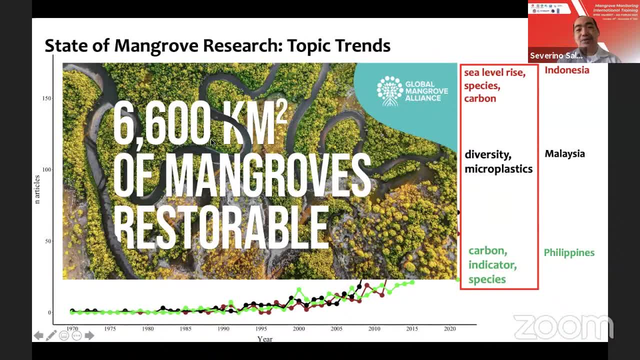 estimated that worldwide there could be around 6,600 square kilometers of mangroves that are candidate for restoration. This is worldwide. The challenge for us now is: if we do restoration- the honest-to-goodness restoration- how much can we really be restoring come 2030?? 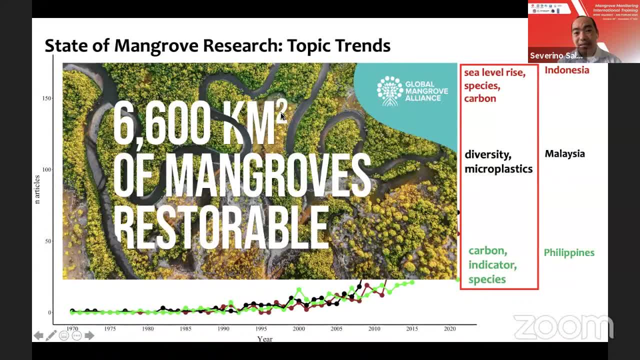 And what do we really want to see by 2030?? So maybe, if this is the restoration targets, maybe there could also be a good research target for mangrove restoration. I'm hoping that maybe the trends in publication would somehow shift to interest on restoration. 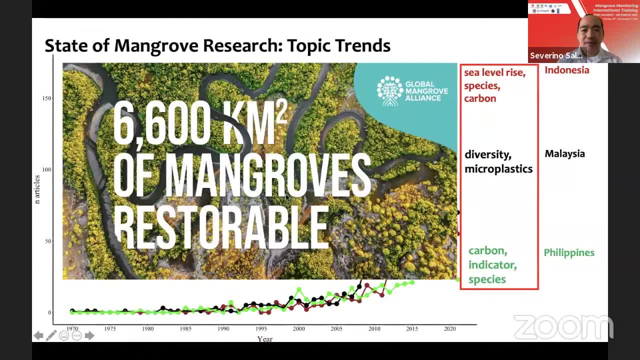 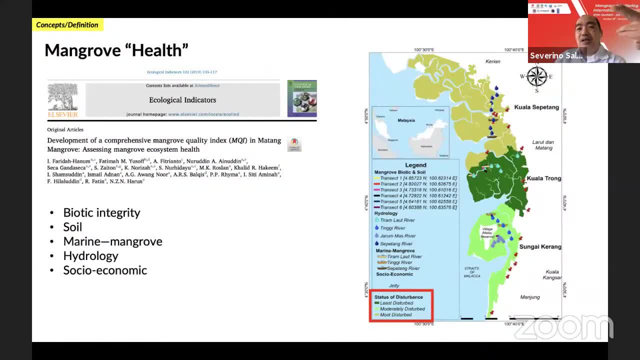 ecology. Okay Now, sorry for that long introduction. Let me focus now on my topic about restoration indicators. I'll be defining first the concepts and definition. There are several terms. Some people call it mangrove health, mangrove integrity, ecosystem health, ecological health. 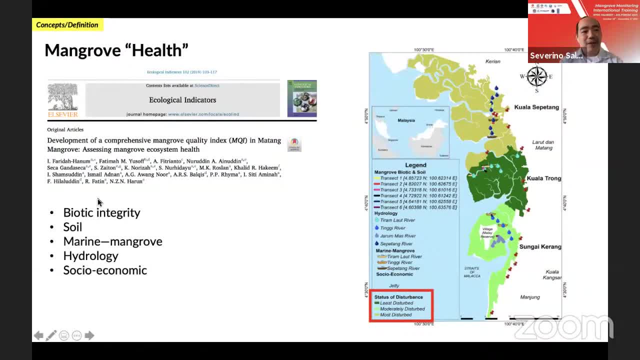 and so on and so forth. I found this paper by Parida Hanum, published in 2019.. They used the model in matang mangroves in Malaysia, wherein they came up with mangrove ecosystem health right, So they used the term ecosystem health and they quantified based on five components. 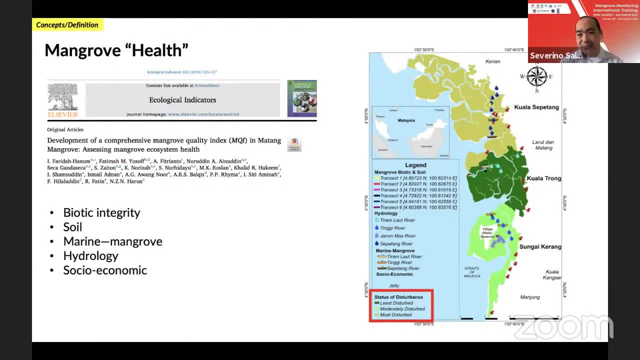 the biotic integrity, mainly the forest structure. if there are foresters here, it's all about the stand structure, diameter, height and so on and so forth. For the soil it's about the physicochemical parameters, organic matter, nutrients, etc. 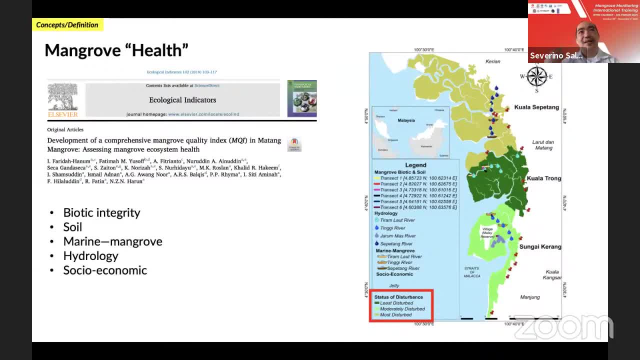 Marine mangrove is about the plankton, the different organisms. Hydrology is about the water exchanges, nutrient exchanges, and then they factored in socioeconomic factors right in matang mangroves. Now, when they compiled these five parameters, they came up with the state of disturbance. 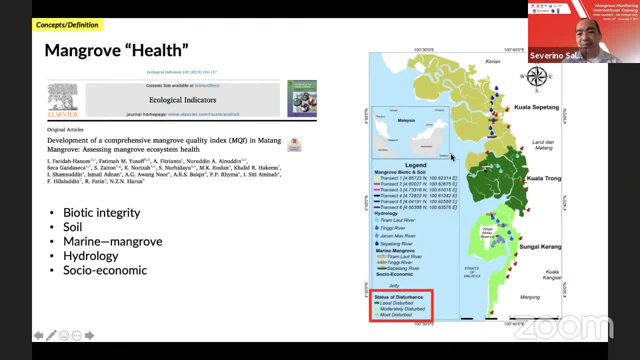 They qualified and quantified least disturbed, here in the internal matang, the moderately disturbed and the most disturbed mangroves. Well, we can use the same approach and define what is, quote unquote, healthy mangroves disturbed. 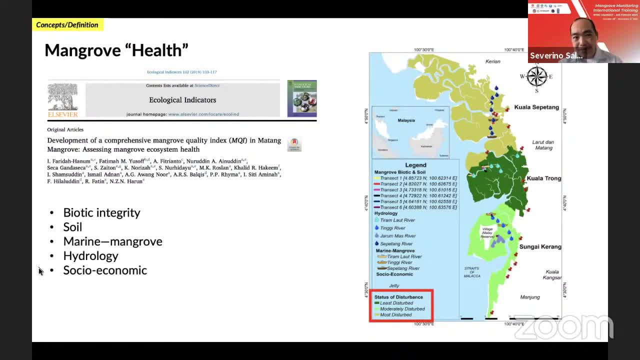 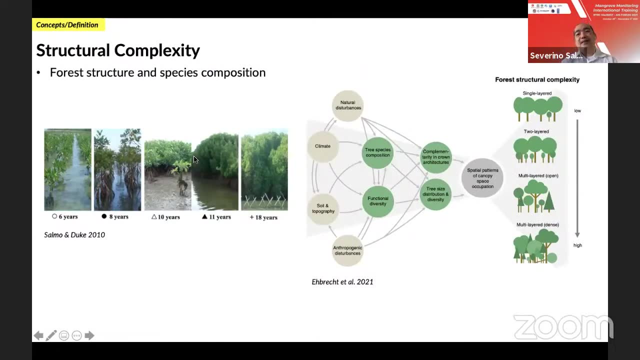 These are mangroves and restored mangroves, based on certain rubrics. It's about the stand, the soil, the fauna and so on and so forth. Now, so that's mangrove health. Mangrove health is, of course, related to the structural complexity of the forest. 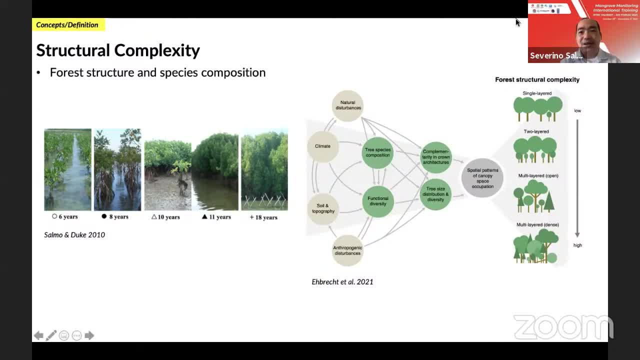 The term was used by Haldrich in 1970s. It's all about the forest's environmental health. It's all about the resource. It's all about the environment structural complexity, but the concept was really applied for upland forests, wherein commonly there. 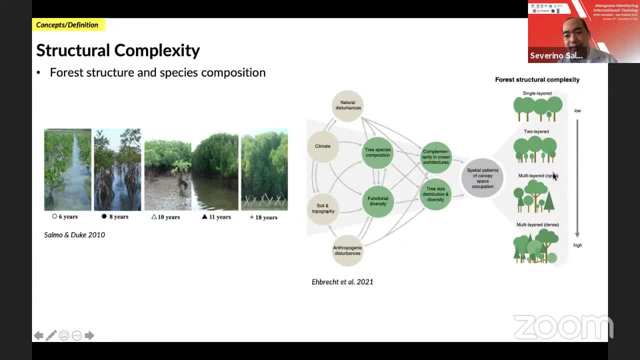 are two layered or multi-layered canopy strata and sometimes there are dense forests with not so dense forests, and it's all about regulated by three species composition and the functional diversity. the canopy overlaps the canopy structure of the forest. now, if we will apply this concept to restored mangroves- obviously this is my site in the philippines- 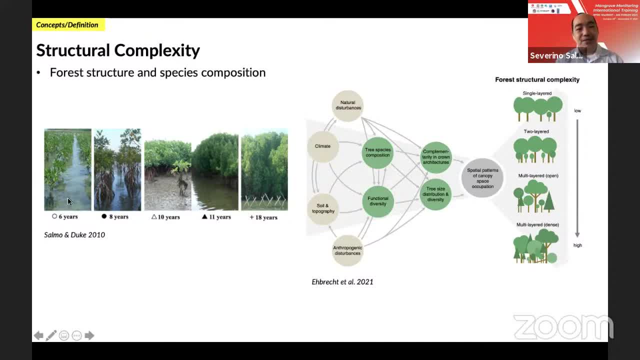 if you plant mangroves now, after six years it will look like this: uh, eight years, ten years, maybe it will look like this until such time that it becomes. the canopy is now closed. now that could happen in around 11th year, but if you plant now, you expect that there will be. 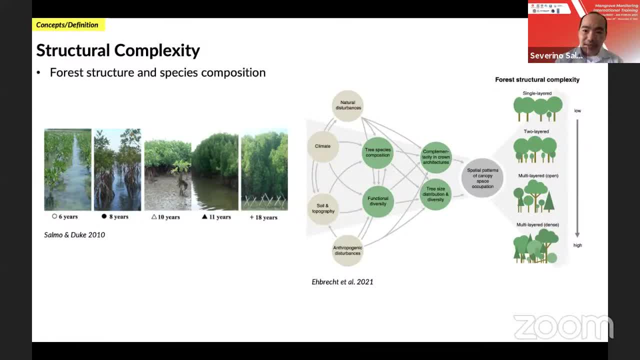 a gradual development of the forest. uh, very rare that you will see a multi-layered canopy structure in mangroves, and if you're doing mangrove research for a long time you know that it's very clean. it looks messy from the outside, but when you go inside you will rarely see a multi-layered canopy. 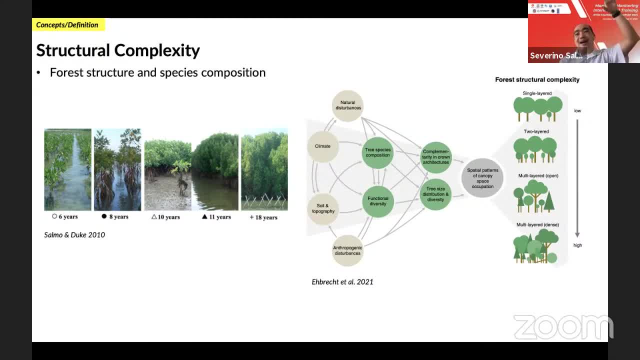 strata most likely. you have your very clear canopy structure, very minimal understory right, and these things are regulated by natural disturbances- climate, soil and anthropogenic disturbances. so right there and then we can see the link between the vegetation, the vegetation structure, the vegetation health, which are also equally affected by the soil or the 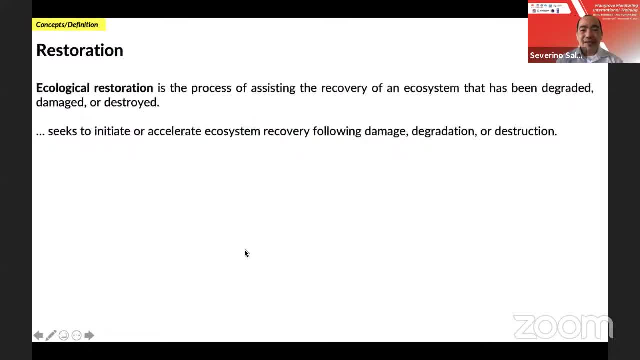 sediment. right Now I'm borrowing this terminology from the Society of Ecological Restoration. I'm a member. I don't know if there are members. there are participants here who are members of the Society for Ecological Restoration. So when you say restoration sometimes it is often interchanged by rehabilitation and 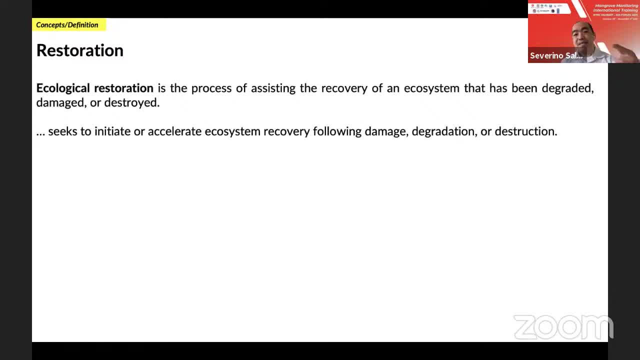 sometimes planting, But planting is different with that of restoration and that of rehabilitation. Rehabilitation, you're referring to the habitat right, But then if there are foresters here, I'm not. I'm an ecologist. If there are foresters here, I'm not an ecologist. 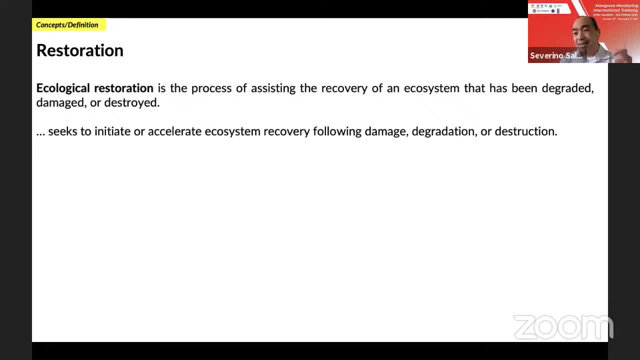 If there are foresters here, I'm not an ecologist. If there are foresters here, I'm not an ecologist. You have another term- it's called assisted natural regeneration right, Wherein you let the forest naturally plant or replant in itself. 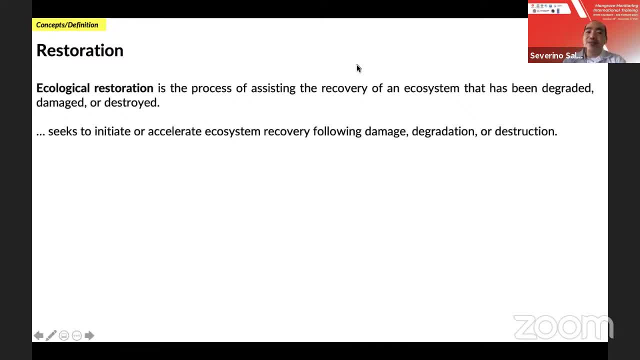 But there are several concepts. But for restoration, I'm referring to ecological restoration, mainly because I'm a restoration ecologist. It's defined as the process of assisting the recovery of an ecosystem that has been degraded, damaged and destroyed. Take note of that qualifier. 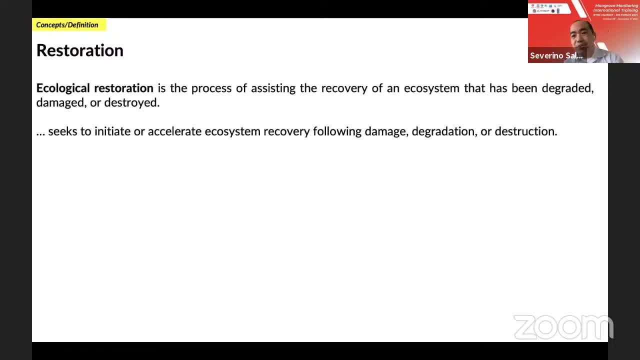 For you to say that it is restoration, the system should have been degraded, damaged or destroyed. If not, then it's not an ecological restoration. The other qualifier is that when you do ecological restoration, it seeks to initiate or accelerate ecosystem recovery. 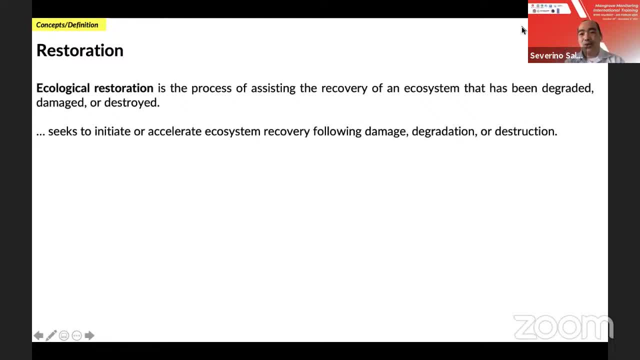 Now we're talking about recovery. What do we want Rehabilitation to recover? is it about the vegetation, the sediment or biodiversity, right? so i'll put a question mark first. now, if this is ecological restoration, sometimes it is often confused with the term ecosystem restoration. it's quite similar in concept, but it has a different purpose. now i'm 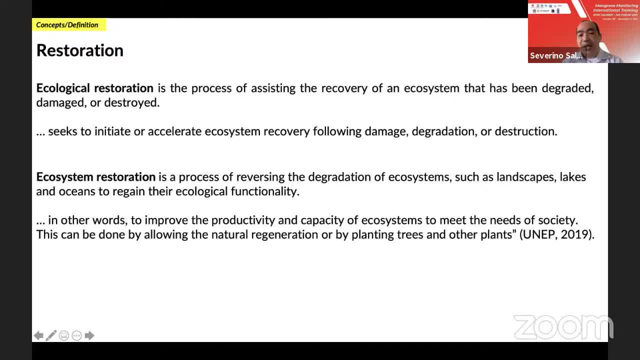 using the terminal. the definition from unep. and the definition is that ecosystem restoration is a process. it's a process, it's not a one-time activity. you want to reverse the degradation of ecosystems. in this case, it's all about mangroves. but then they specified ecological functionality. 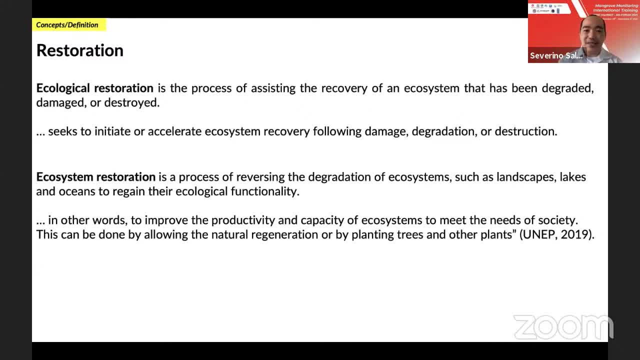 the delivery of ecosystem services. now, when you say ecosystem restoration, you want to improve productivity and capacity of the ecosystems to meet the needs of us society, and you want to do that. you want to do ecosystem restoration through natural regeneration or by planting of trees and other plants. so, uh, we have to be very clear on the definition, if you 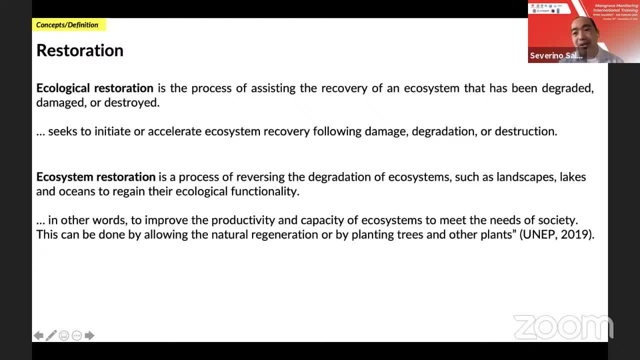 want planting, that's fine. you do planting, but you cannot call it ecological restoration or ecosystem restorations, not even a rehabilitation if you're really just doing planting. there are clear-cut rules on what is restoration and what is not a restoration. but then again we have to be very clear: are we doing ecological restoration or ecosystem? 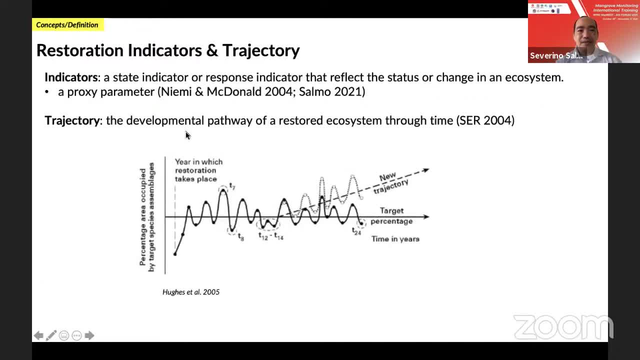 restoration now related to restoration. is the term restoration indicator right? so when you say restoration indicator it could mean the state indicator, referring to the state of the system, or a response indicator, meaning how do the system respond to a particular restoration or disturbance. but indicators would have to reflect the status. 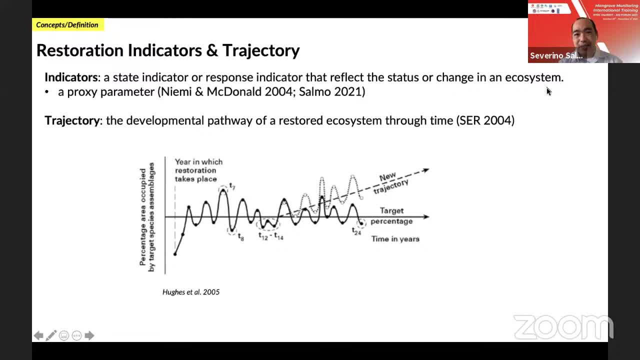 or change in the ecosystem, and naomi and mcdonald called it a proxy parameter. i also use that term in one of my publications this year. i use the term indicator as a proxy parameter, not as an absolute indicator, but only as a proxy parameter for the state. 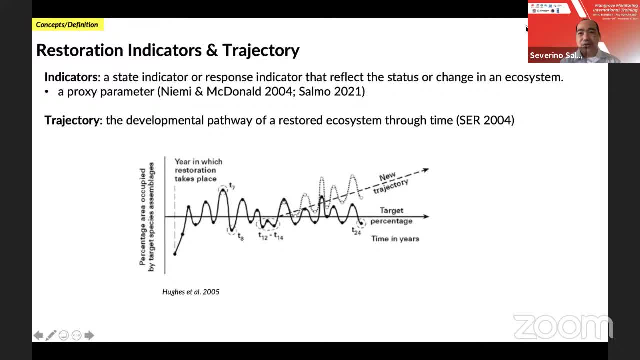 of the system, right? so when you do restoration indicator, it will also follow that restoration trajectory is related to that of the restoration indicator. first, what are indicators? maybe a vegetation indicator, a sediment indicator or a biodiversity indicator. if you look at those indicators and if you plot that over time, you have your time zero. 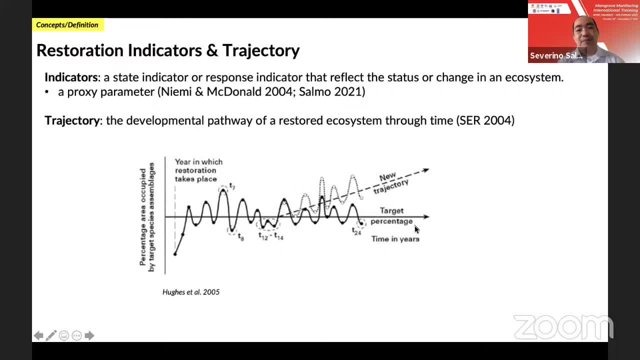 and your target time in here, for example 10, 20 or 50 years. then you track, you assess the changes in those indicators over time. so maybe time zero, you start with something or you start with nothing. in year 10, maybe you develop a forest, but the forest alone. 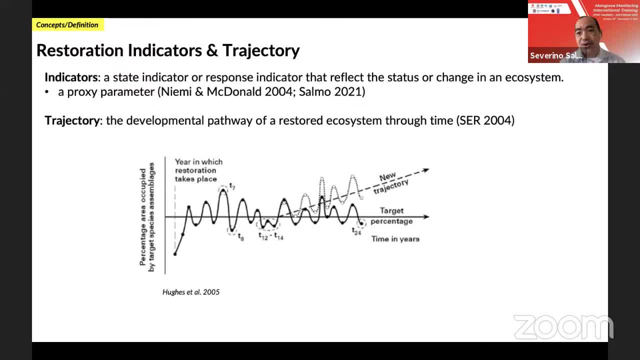 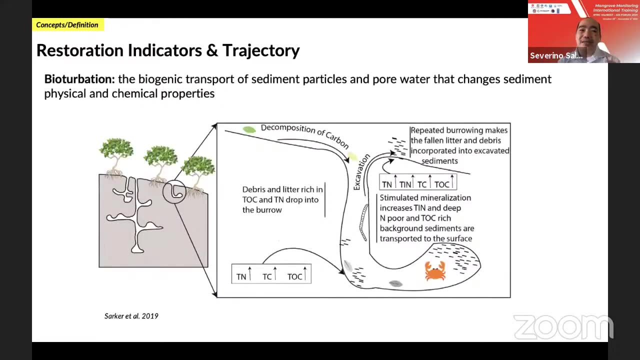 may not necessarily be an indicator of restoration. there are several criteria for you to say what is a restoration indicator? what is a restoration trajectory? now, because my talk is about vegetation, sediment and, uh, mollusk, let me introduce. i don't know if there are biologists here. somehow i'm also a biologist, but i'm more of an ecologist. 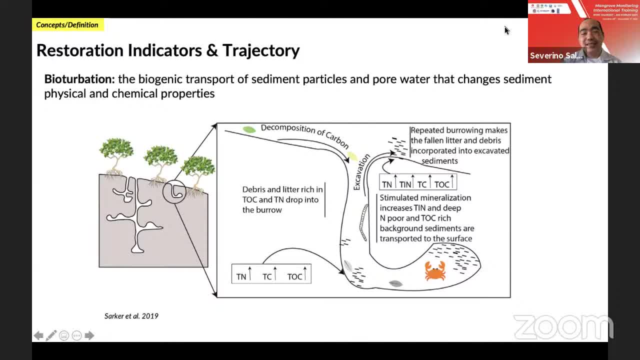 when you say bioturbation, it's like a biogenic transport. uh, there's a transport of sediment particles. we are, of course, depending to the mangrove sediments and there's this alteration of pore water, not the surface water, not the groundwater, but the pore water within the sediment. 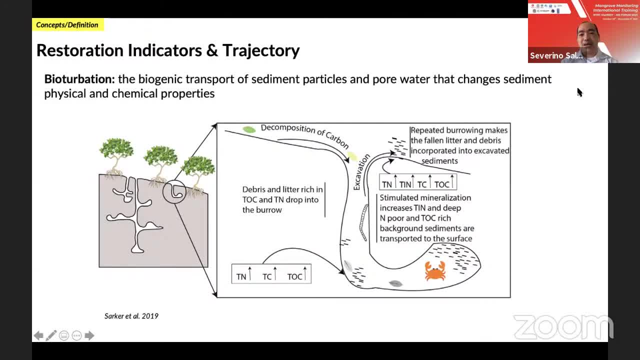 that could change sediment physical and chemical properties. in this review paper by sarker et al they specified scrubs and to some extent i think shrimps, but of course, if you look at the mangrove ecosystem, mollusks are actually a super compact system of sediment. you can see here in this diagram: 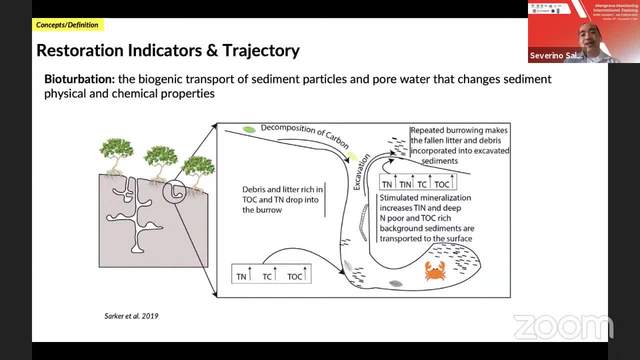 are actually more dependent and more affiliated in the mangroves and the mere action of the, of the molus and even crab, for this matter. you know, when there's a litter material here from the leaves, from the foliage, that litter materials will be deposited in the forest floor right. 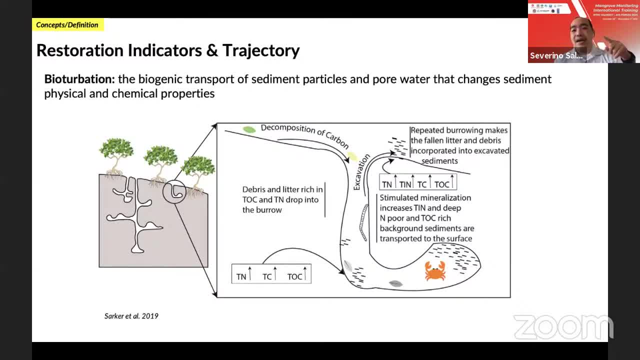 so right there and then your litter materials are actually contributing to nutrient retention and nutrient enrichment of your vegetation. but without the fauna, without the models, without the crabs, it will take a longer period for those litter materials to be to become available for use of the mangroves. luckily for us, there are crabs and molus that are feeding on those. 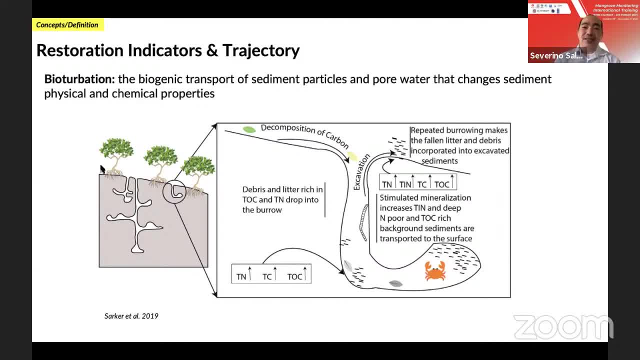 litter materials. so when they feed on the litter materials here in the other forest floor, they enhance the, the biodegradation of those leaf components and it will become converted into nitrogen, organic matter and veterinary carbon and then there will be cycling. now, uh, if you're working on mangroves, you know that. we know that mangroves are living in. 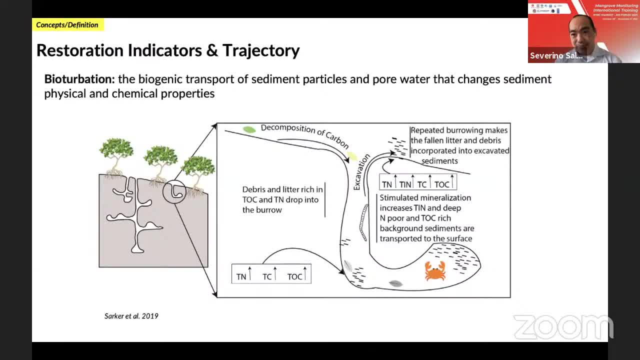 an environment that is deprived of oxygen right now because of such conditions. so that means the feeding activities of the molus. they go deep, they go deep and deep and deeper in the sediment. once they do that, they actually facilitate the process of aeration or simply providing air to the otherwise uh sediment that lacks oxygen. 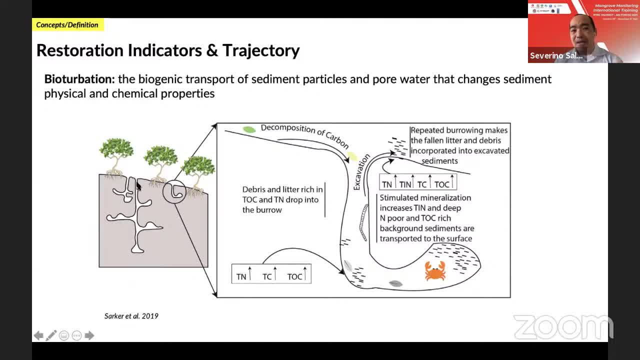 so the feeding and the borrowing activities of the molus are actually, When the mangrove is fed, what do they caught? including the feeding activities of the molus actually a good indicator that your mangrove is healthy, right. otherwise, even if you have litter production here but it is not available for the mangroves to absorb then those materials. 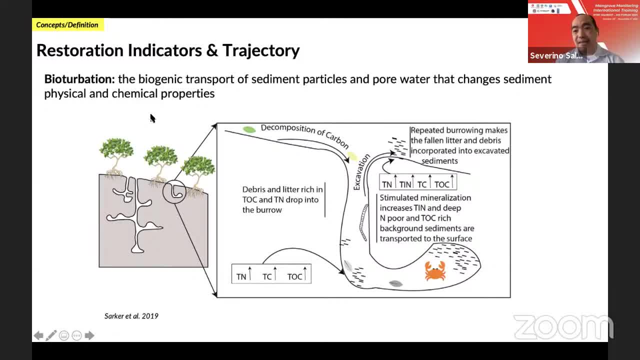 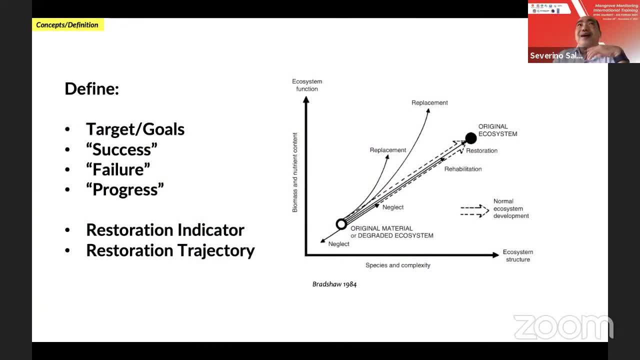 will just be left out in the sediment. that's why I inserted this slide on bioturbation. okay, now we talk about uh restoration, we talk about ecosystem Dynamics. we talk about uh indicators and trajectory. I'm using this slide on the link between biodiversity in the x-axis and the biomass. 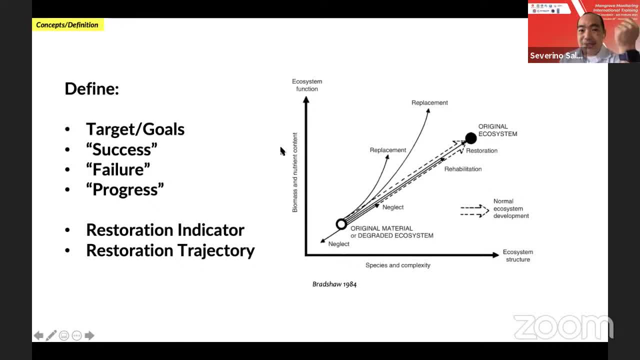 and nutrient content in the y-axis, but you can substitute any ecosystem services, for example carbon, in your y-axis. with that knowledge, then I can ask you: what is your restoration Target or restoration goals? okay, what do we want to achieve? how do we call restoration a success? 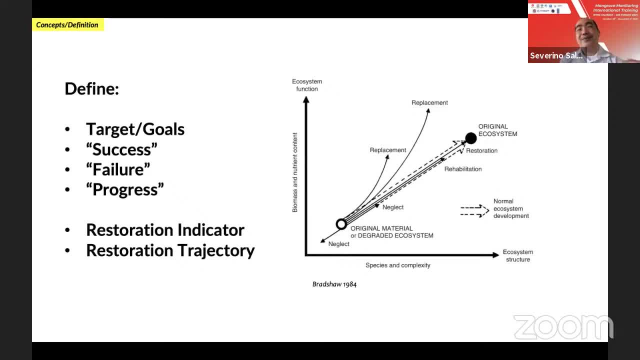 commonly here in the Philippines, if the if the mangrove survived in 10 years, sometimes two years, sometimes one year, if the mangrove survived, they call it success. okay, but if you ask me, hold on, because I know that mangroves will grow. in 10 years time I will have 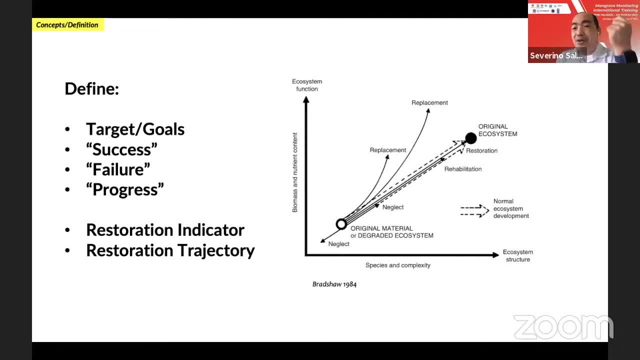 to wait until 10 years for me to say that your mangrove restoration is a success right now? when you say success, what would be your criteria for success? is it about the growth rate of the seedlings, or the survival rate of the seedlings or the development of the forest, for example here: 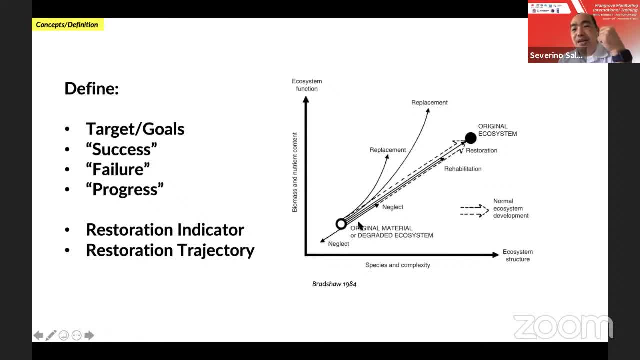 if you have a degraded system and then you do restoration, are you saying your restored mangrove as a successful restoration? because your restored mangrove has an equal or or almost similar attributes to that of a reference system. okay, or maybe We can call it failure. If the planted mangroves didn't survive, then simply it is a failure. 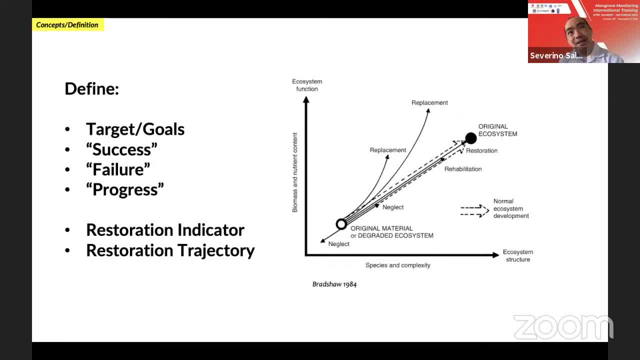 It's very easy, right? You plant mangroves now and next year you don't see any mangroves. then it's very simple. It's a failure, right? Or maybe we want to call it progress or the lack of progress in restoration. 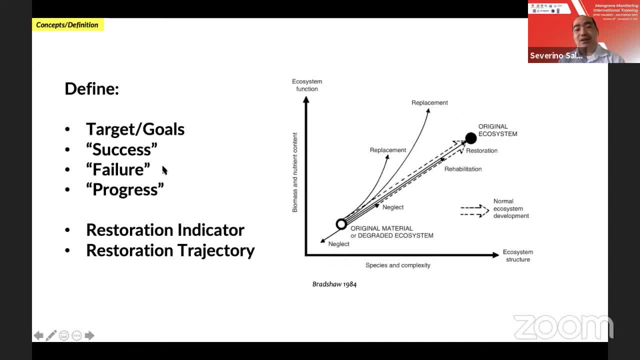 Either way, whether you call it success or a failure, it has to come up with a rubrics Here. what are we measuring? And for that matter, I'm leaving the criteria to the audience. What do you think would be the suited restoration indicator? 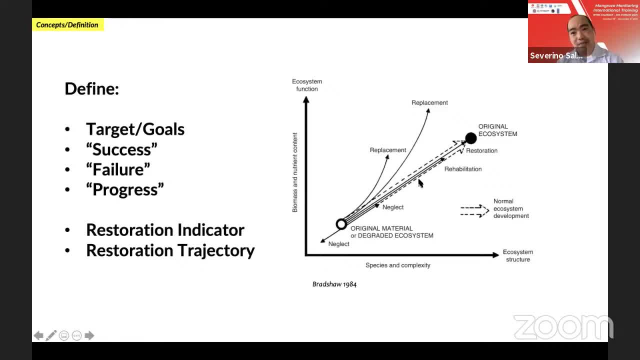 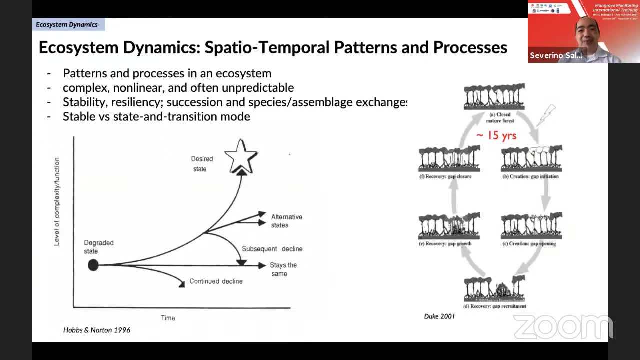 What could be a reasonable restoration trajectory to be expected. Okay, Now if we look at the Ecosystem dynamics Here, for example, same slide as before. If you have a degraded state and you don't do any restorations, then obviously it will forever remain degraded, right? 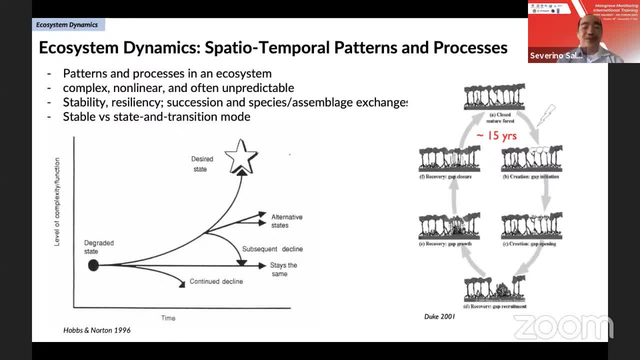 Because nothing is changing. Unless you do something else, then that degraded state will be remaining as degraded Now. if you plant, if you do restoration now, here, time zero, maybe in 10 years' time it will become like this, based on your restoration indicator: right. 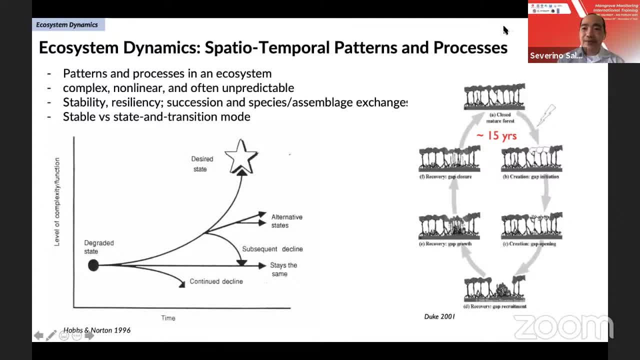 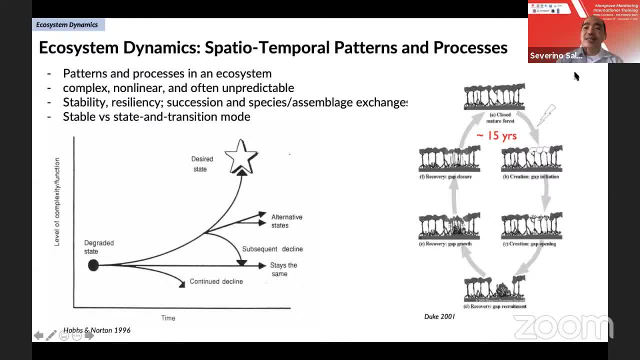 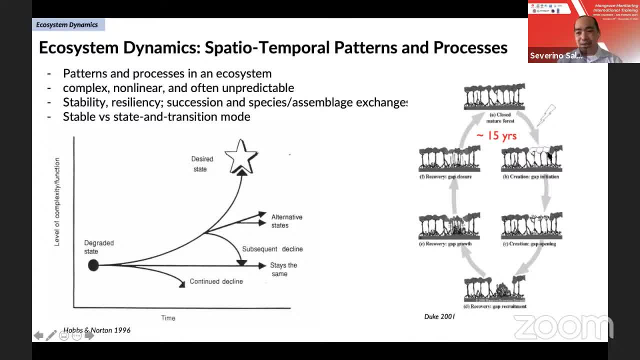 So when there's a lightning strike there could be canopy- sorry gap, initiation, gap opening until such time that there will be a full gap closure. In Australia, the average time that you can see canopy closure is- it's around 10 years. the philippines it's around 15 years, i think, in in malaysia, indonesia, it's. 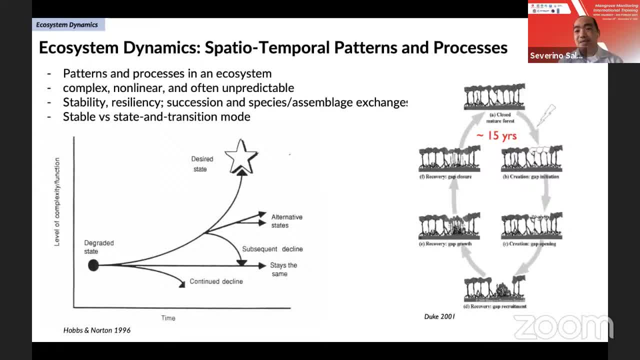 around 15 to 20, sometimes 15 to 25 years. it will depend on your ecosystem dynamics, but we know that the growth and development of a forest is non-linear. oftentimes it is very unpredictable. and why, why unpredictable? in the philippines, there are several disturbances. we do have typhoons. 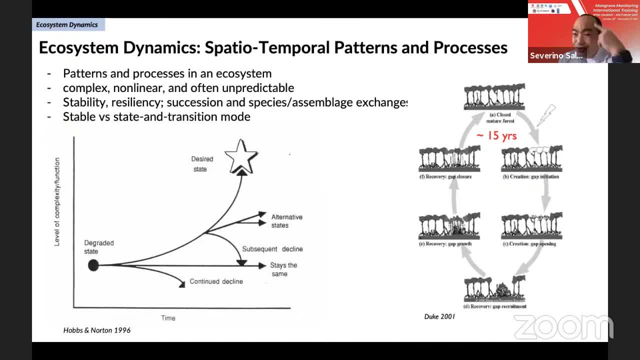 or i don't know- i think you're calling it cyclones, or you. you don't have typhoons, right? no, no, no, okay, we have. uh, we have typhoons here, uh, around 20 typhoons in a year, and every time there's a typhoon, you expect that there could be changes in your forest. it's a. 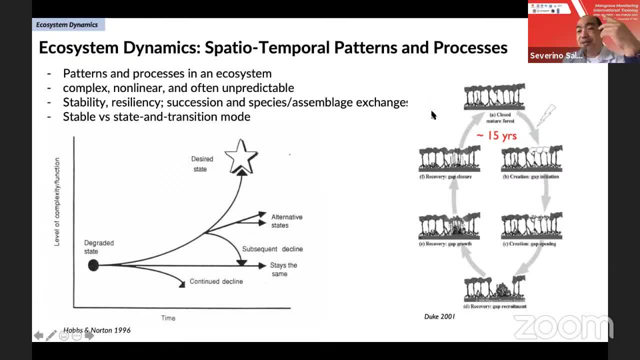 natural phenomenon and that could contribute to the changes in your forest right now. this kind of mix is believed to be related to the stability or resiliency of your system. so if you do restoration, you plant mangroves now and then there's a disturbance tomorrow. do not expect that your 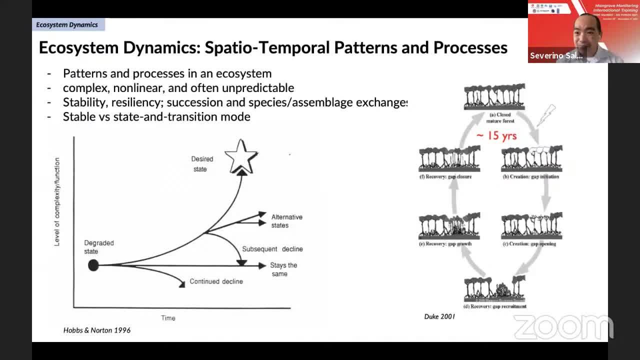 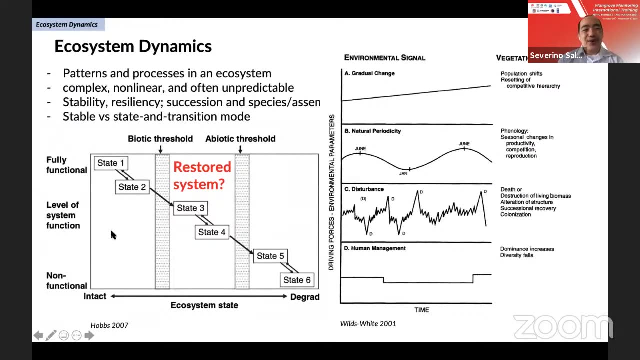 mangroves will be stable or will be resilient. it will take at least 10 to 15 years before your mangroves will achieve stability status. okay now, um, what is fully functional versus that of a non-functional? and again, this will be related to the degree of intactness of your forest and the degree of degradation of your forest right. so in 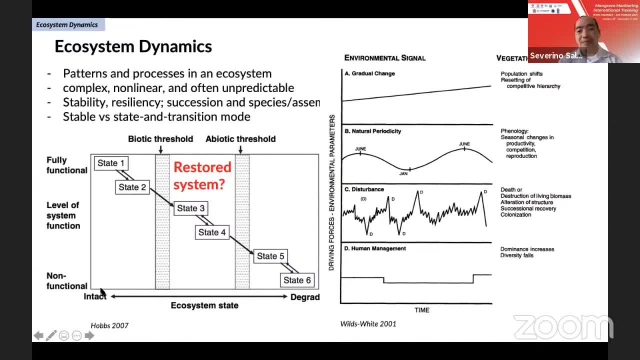 this concept: if you have a healthy mangroves, a natural mangroves, intact- and you have a lot in indonesia- uh, it is believed that you have a fully functional mangroves and i believe that right. but if you do have a degraded mangroves, then you are in state six, meaning your functionality. 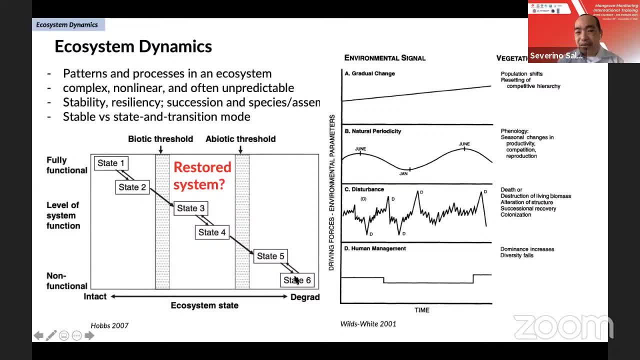 level is a very minimum in between is your restored system. it could be state three or state four, but the idea is that the stored system would be somewhat shifting to a state one and state two functionality of the restored system. but we have to factor in what is the natural variability, things that are naturally occurring. 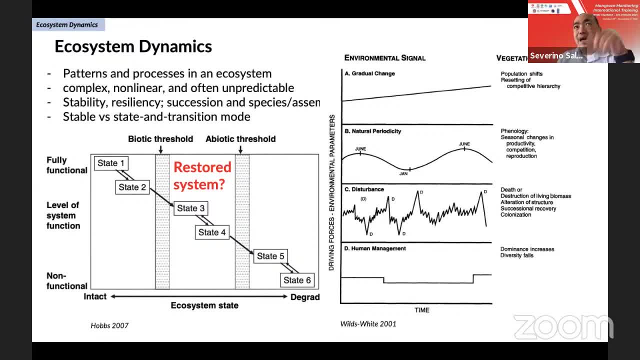 natural phenomena, natural disturbances, every time you factor in anthropogenic disturbances, and it's very difficult to predict. if you cut mangroves now, deliberately cut by humans, then obviously it's not, it's not a natural phenomenon. then this model might have to be shifting right and that's the reason why. 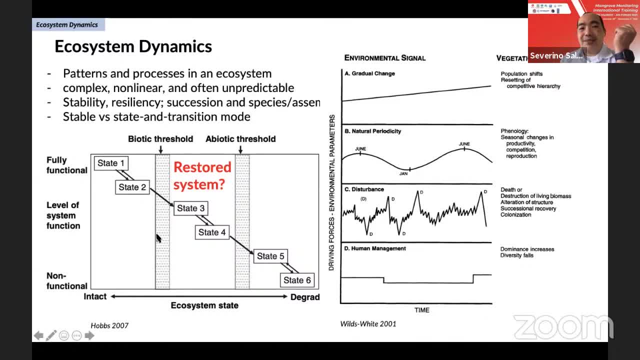 it's not really that clear to you, Dr. so you want to talk about the variability in the nature of mangroves and how it affects the natural environment, Dr, that's a good question and i think it's very clear that mangroves and mangroves are not linear, but what i'm saying is that there are natural. 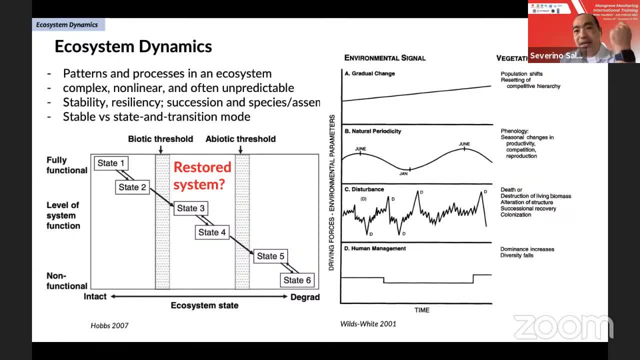 patterns and processes that are observed in unnatural mangroves. if we will compare a restored mangroves here, hopefully it will follow the lead of a natural system. but it is also possible that your restored system might be experiencing disturbances and therefore it might not reach full functionality. 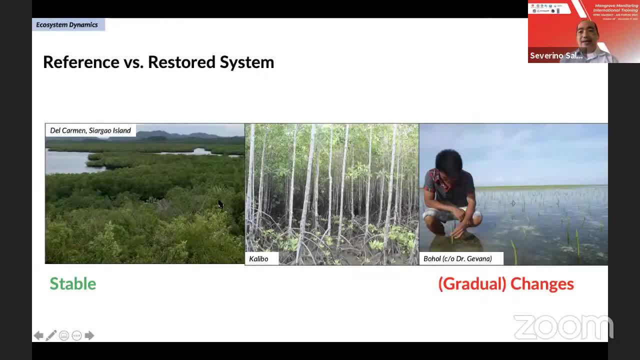 Dr. okay, Dr right. so some examples. this is one of my favorite sites in the philippines, a stable state, the largest mangrove, contiguous mangrove in the philippines. this is, in southern part of the country, a key biodiversity area. we do have crocodiles here in the in this, in this spot, not in the farm. 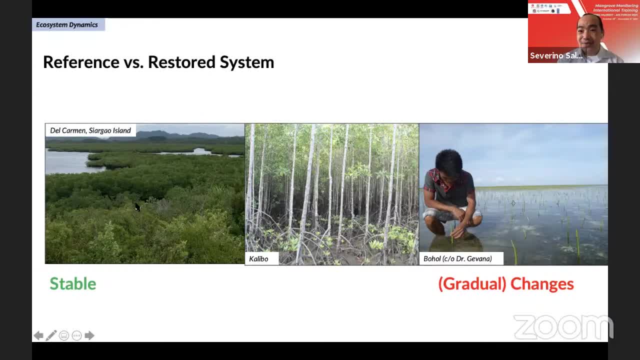 not in the zoo, but in the wild here. so you can see that it's really healthy and but even that this site is known to be absorbing a lot of typhoons. i think this month will be the period when there could be a lot of type ones in this area. now. the other site is this one in kalibo also. 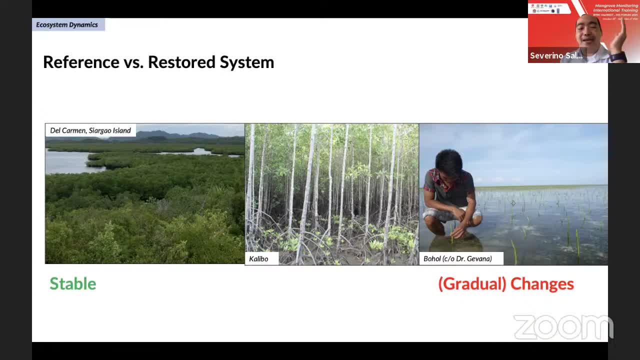 again in in the south, in in visayas area. this is around 17- 18 year old forest right Dr. so look, this could be more than 100, maybe even more than 200 years old. this one is around 18 years old. it's not really that comparable, but you see that there's this alignment. 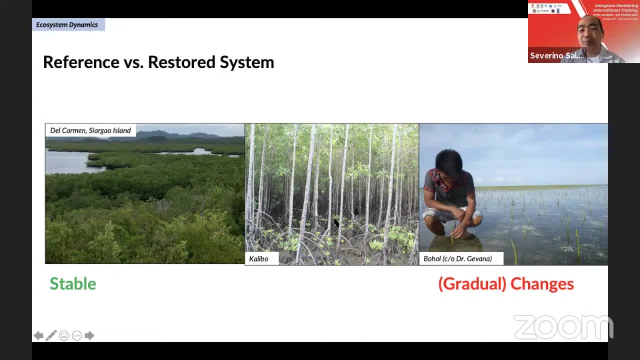 because it's planted. you see, there's this one to 1.5 meter distance between trees, and it's because the, the humans, planted it that way, and you see that in even in 18 years time, that arrangement can still be observed. Now, if you do this, photocopies. 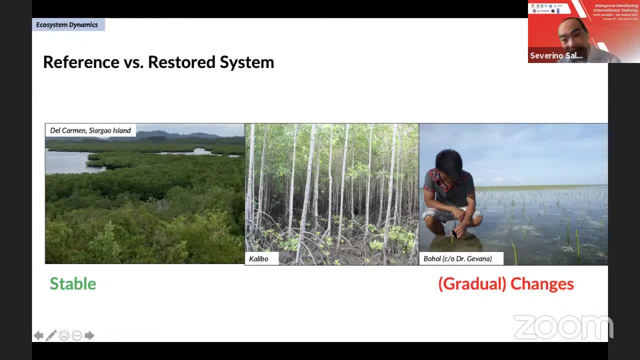 of Dr garbana. you plant these mangroves in sea grass and you know that it's flooded, then it will take time before before they grow and we become like this. and i you know, some of you are smiling because we have similar case, don't worry, uh, malaysia is also with us and i think even vietnam and maybe thailand. so we are. we are not in the rondelle area, but we can plant mangroves. Galileo honor, you're going to visit us sometime soon. there's a but, les pern lamb. but we've talked for a while and sorry to also ask if you want to ask some questions of. 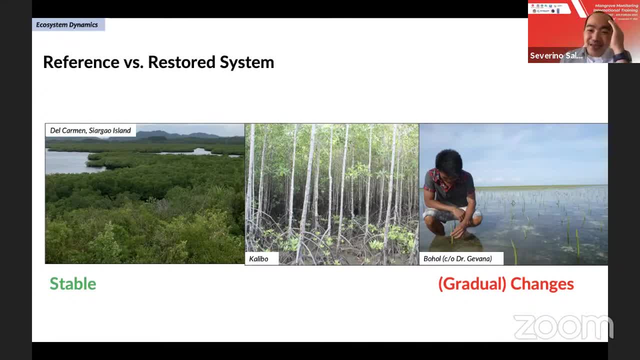 so we are. we are on the same setting, so take note: uh, it will take 15 to 25 years before we can have a stable forest like this. meantime, while it is not 15 years old, and assuming there's a disturbance, obviously you cannot achieve this level of vegetation structure because it's still developing. 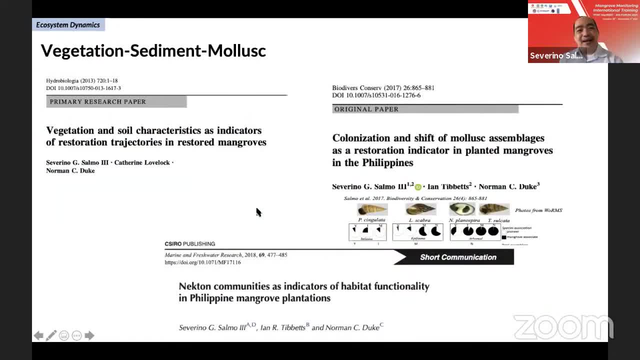 next. right, uh, i'm sharing these papers more. most of my slides are came from this uh paper. uh, this one's 2013, this one 2017, this one 2018.. it's all about. it's all about the vegetation soil molus that i studied. if you're interested, if there are interested people here about 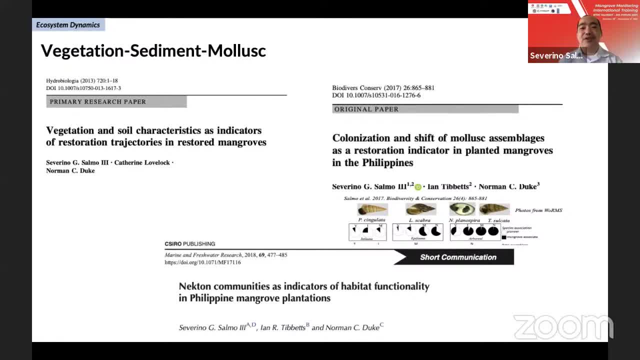 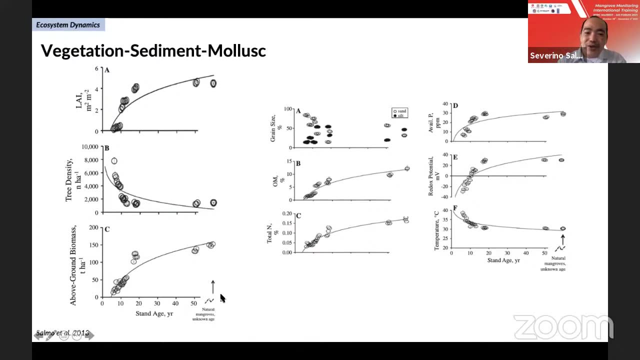 necton about fishes or crabs. let me know i can discuss that with you, but i will be focusing more about vegetation, soil and the molars, right. so okay here. um, i was lucky enough to document a natural mangroves in my x-axis and 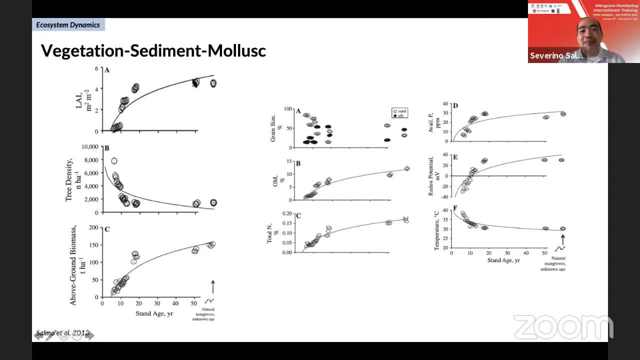 we know we are lucky enough that we do have a planted mangroves that is around 50 years old. okay, now my main site is really this: around 20 year old. the oldest is 20 and then this is six, six and eight years old when i- when we track the vegetation development, of course we measure. 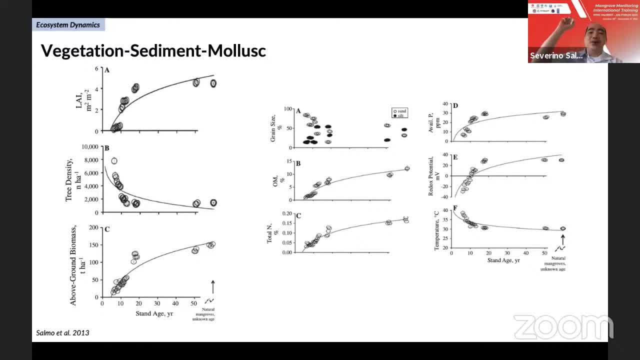 uh, three diameter, three height: canopy height, total height, canopy diameter, canopy shape: this is, and so that so many other things litter, litter, production, uh, et cetera. uh, at some point, there's this uh pattern wherein it will have to be reaching almost that same level of a reference system, right? so, in terms of flip area index, 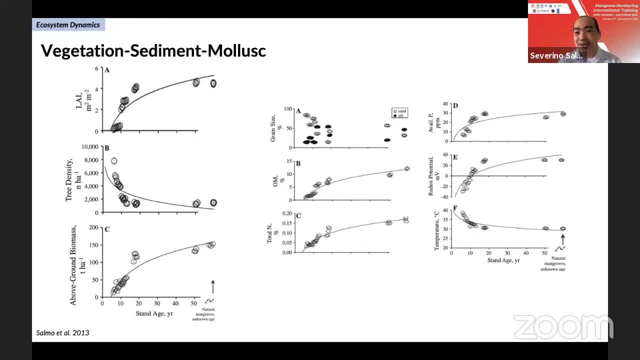 and i i've heard you in your ge session this morning. you have your lip area index or evi something or ndvi. i think it's somewhat related. related to lai- yeah, that that term right. and then there's this three density. now, if you plant mangroves- and it's very dense over time, mangroves- 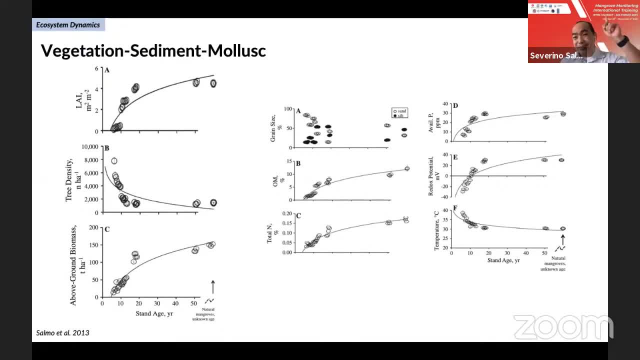 cannot, cannot grow all the way to heaven. right, there must be a competition between and among seedlings, and that's the reason why you will have your reduction of tree density over time, and you will be lucky to observe that there could be- because this is my reference point- the, the, 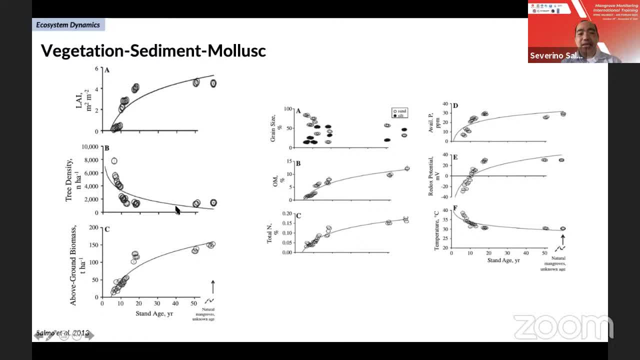 natural mangroves. if the tree density is somewhat equal to that of the natural mangroves then i can say: ah, they are quite similar. right same goes with above ground biomass here, uh. but take no, even for 20 year old mangroves it's not really that similar to well, very close, but still not. 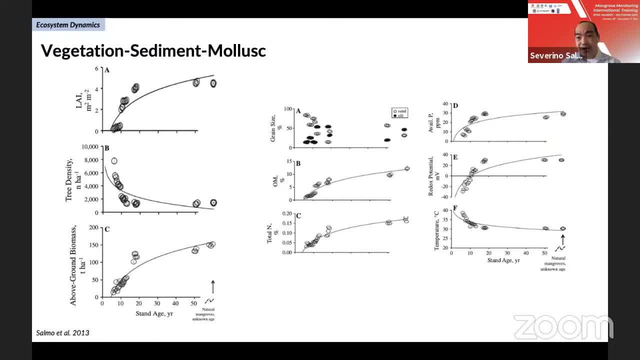 similar as compared to a natural mangrove right, and for for several reasons. now this is for vegetation i i mentioned. i i also meant i also measured many other vegetation parameters similar to basic ecological and forest assessment methods within that, out of those vegetation these three parameters are uh have shown good relationship with aids. of the mangroves, the 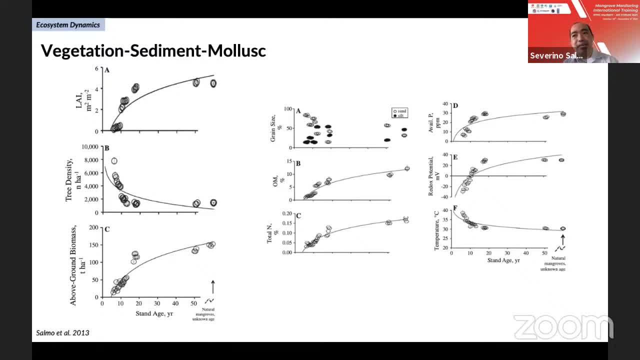 restoration aids. i forgot to mention the seedling density and something. density- it also has a good trend, but i think these are very, very apparent, very obvious patterns. now, this is for vegetation, but for sediment there's no clear pattern with grain size, the sun-sealed clay structure not really, and but in some cases you see that there's this increase. 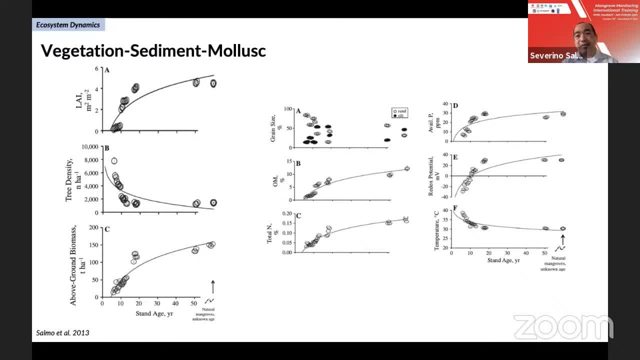 in silt content or clay content, not much of a sandy or a course uh sediment structure, but it is site specific, depending on where you are. what we found out is that there are clear increase and development matter and organic carbon for that matter, total nitrogen, phosphorus, redox oxygen. 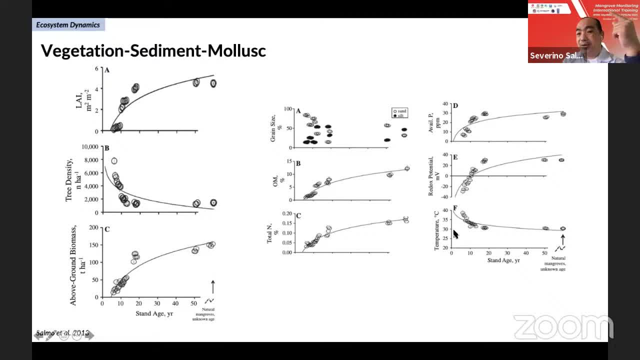 is increasing and temperature is being regulated, right, Because as the mangroves develop, the canopy increases, the biomass increases, structural complexity increases and it facilitates the trapping of organic material. So you have this increase in organic matter over time, right? 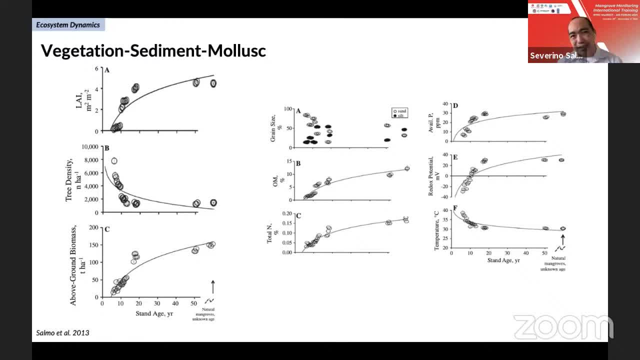 And as the canopy develops, the soil temperature is also somewhat regulated, and so on and so forth. Same goes with redox potential. right And again, take note that 18-year-old mangroves have very similar sediment properties with a 50-year-old and a natural. 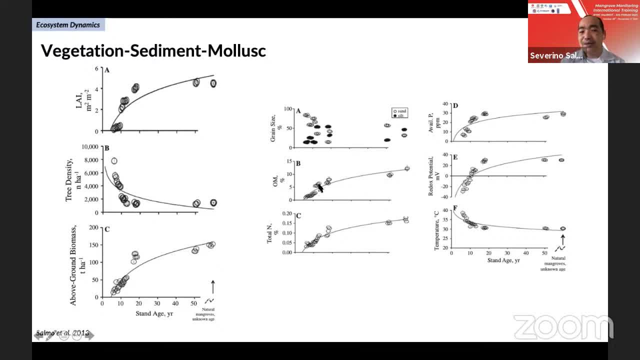 In between you have your well, quite similar but not quite. and then you have your young mangroves that are still developing at that time and it's still not comparable with that of a reference system. It takes time for you to see a clear vegetation and sediment patterns over time. 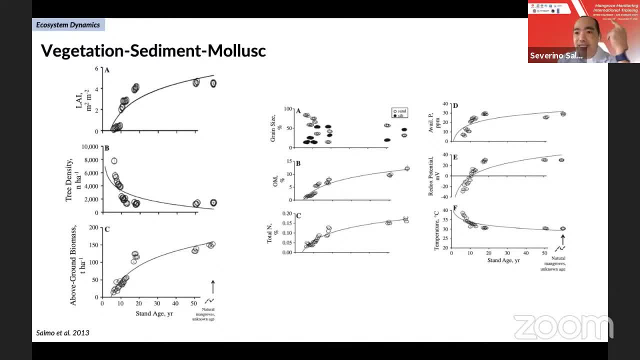 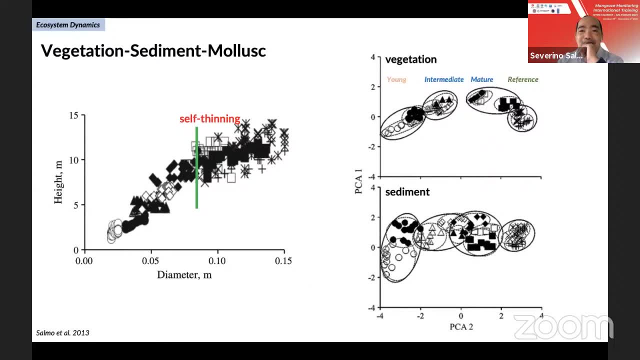 The idea is that you have to compare that with a reference system. okay, One thing that I found out is that if we want to find vegetation indicator- and assuming you have your clear documentation of your restored system- then we have to capture self-thinning. 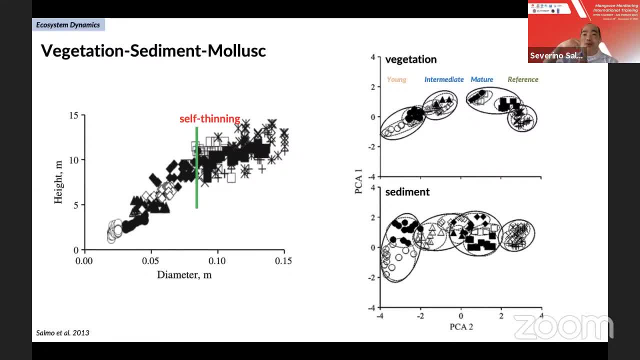 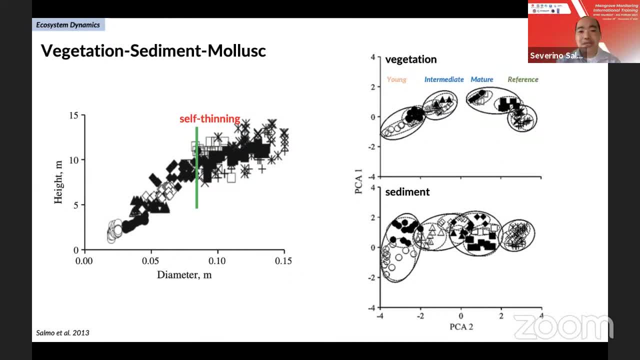 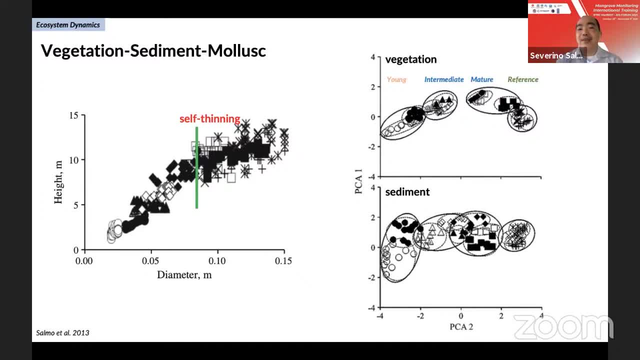 you observe self-thinning. that would be the time wherein your vegetation is not as good. vegetation structure will be very similar to your reference system right, and i hope foresters and ecologists will be able to capture self-cleaning. it's a simple ratio of three. 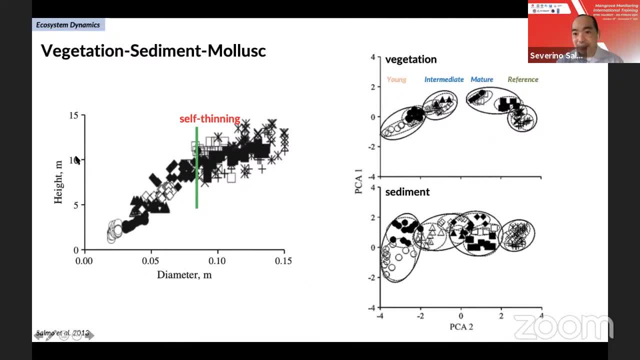 diameter and that of three height. okay, obviously, if you have a plantation, you have one is to one ratio, right, one centimeter maybe to one meter, and then, as the as the tree grows, there will be a development of structural complexity, there will be pacing and outpacing of forest development and 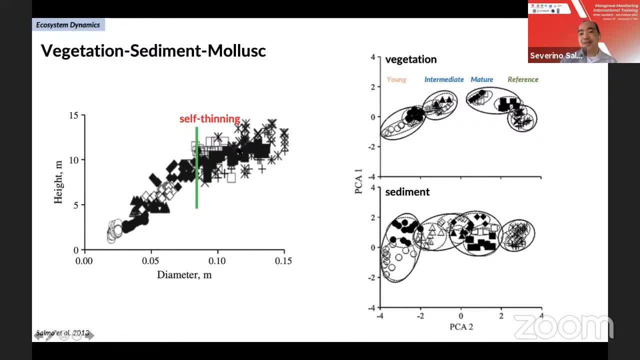 you'll be able to see fluctuations here. with that uh criterion i was able to document to say that, ah, if it's less than eight years old, here i will still call it a young mangrove. it's still undergoing uh forest development. if it is 8 to 12 years old, then i will call it. 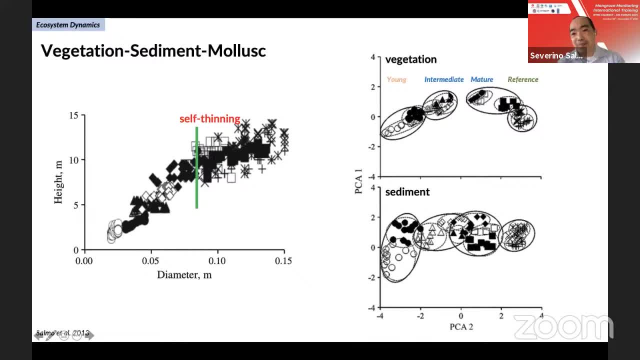 maybe intermediate stage of forest development. if that is around more than 15 years old, because it has very close similarities in terms of vegetation and sediment with that of a restored mangrove, then i can say that it is already a mature mangrove. but, guys, i need to. 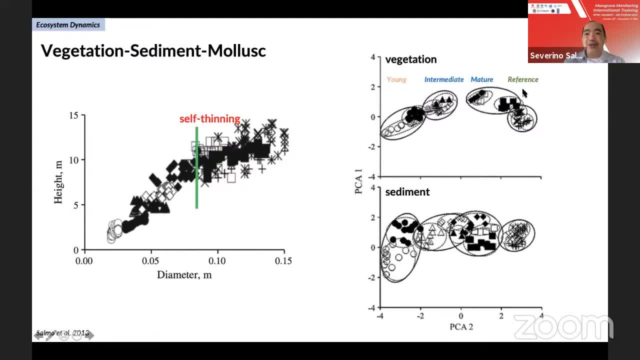 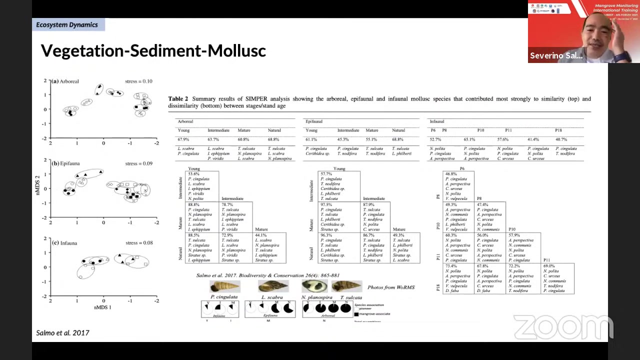 like here, that you're making a comparison because you have something to compare. if you don't have a reference system, then it will be very difficult for us to say what is a young, intermediate and mature restoration progress. right, okay, now i've shown that. just this, uh, clear development in terms of vegetation and sediment. 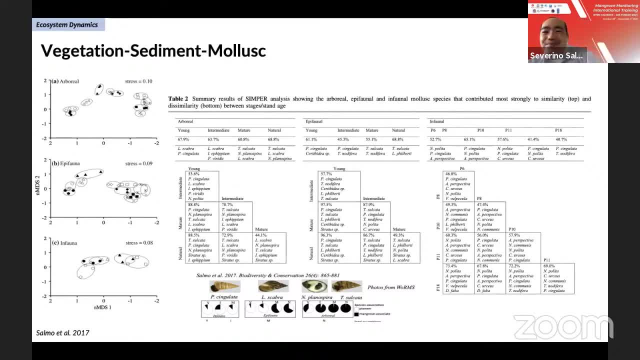 now in terms of the animals, because that's this improvement in vegetation cover, improvement in sediment maturity. you would also expect that there would be a recruitment of fauna. the animals- Maybe fishes, maybe crabs, shrimps, but for this particular study I studied mollusks here. 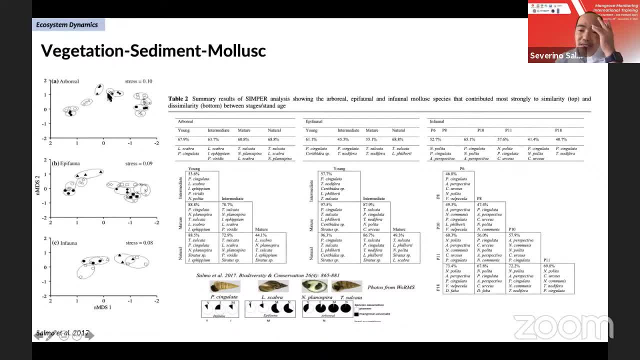 So we collected. there are different types of mollusk assemblages. One that is connected to the mangrove trees, For example, in the roots, leaves, stems, those are your arboreal fauna or arboreal mollusks. The other type of assemblages is the mollusks that are collected within the sediment surface. 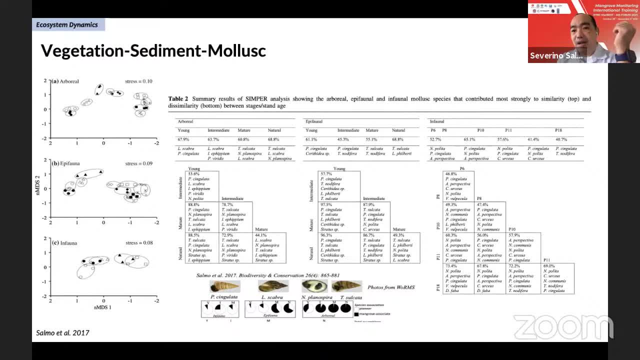 And those are the epifaunal mollusks. Now, if you collect mollusks within the sediment, if you do a core, if you pour the sediment in the mangroves and then you collect that sediment, mollusks that are found inside the sediment, 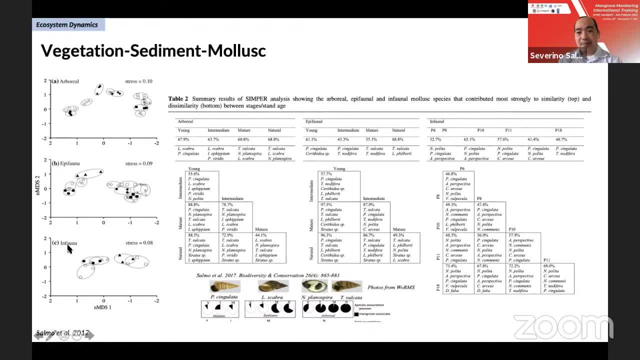 are what we call the enfaunal assemblages. So in this study we compared what are the mollusks that are dominant in arboreal epifauna and that of enfauna. What are the dominant species in young mangroves? 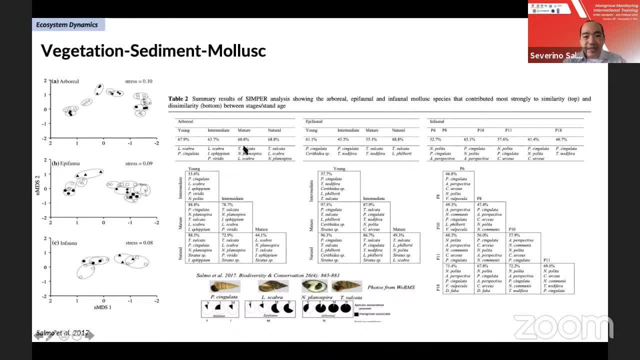 in intermediate mangroves, in the mature mangroves and that of unnatural mangroves, And we did the same thing for the epifauna and that of the enfauna. Simpler is similarity, percentage analysis. So when we found out the dominant species in different assemblages and in different stages, 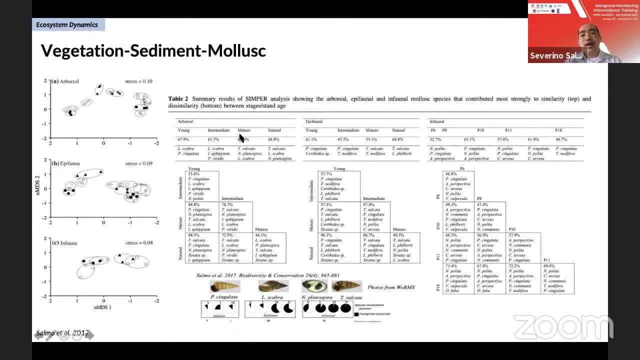 we also compared what are the species that are distinct to young, intermediate, mature and natural mangroves, and what are the common or shared species between a mature- here mature- mangroves and that of unnatural mangroves, And the percent similarity is actually quite high already. 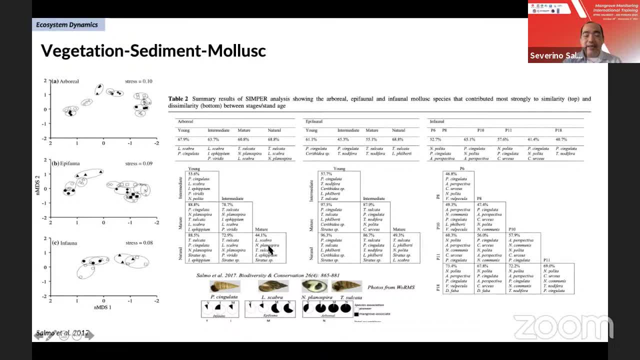 So around 44%. Okay, And it's very clear: if you talk about arboreal mollusks, same goes with that of epifaunal mollusk assemblages. But for enfaunal assemblages the species are very limited, simply because if the mollusks have a very suitable environment, 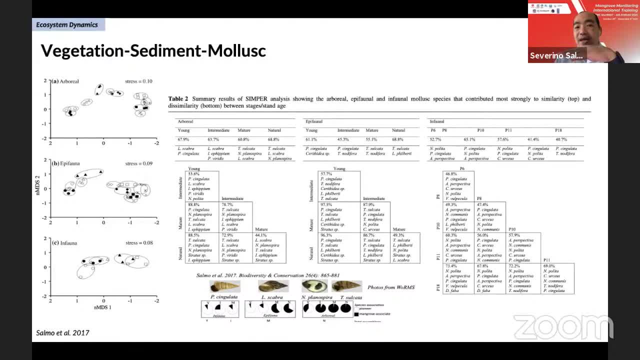 for example, in the surface, in the epifauna, and if the trees are really developing, then there could be more food in the surface and that in the mangrove parts. Why will the mangroves stay inside the sediment if there is a lacking oxygen? 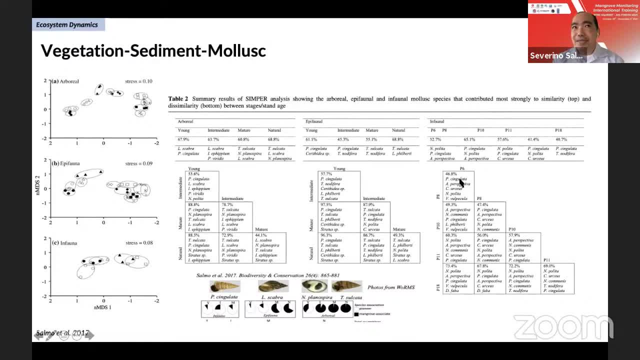 Then therefore, yes, the sediment in fauna is also a suitable environment, but there are a lot more suitable environment in the epifauna and in the arboreal environment. So those mollusk assemblages will have to go up in the surface or cling. 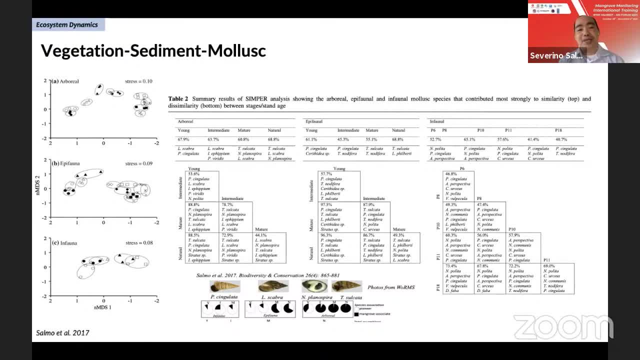 or be attached to the vegetation parts. Then I was able to show this shift: Pirinella singulata, dominant in fauna, I forgot Litorina scabra, dominant in epifauna, And this is Nerita planospira and Terebralia sulcata. 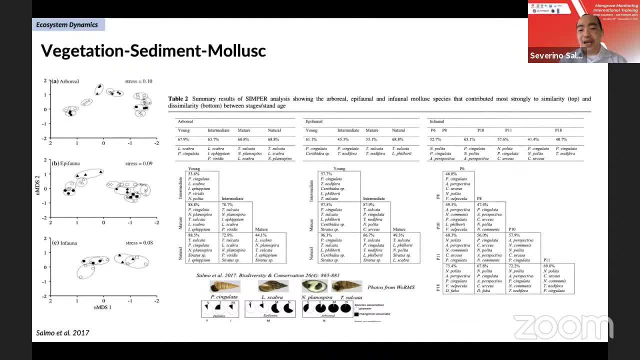 The common mollusk assemblages that are dominant in the mature and also that in unnatural mangroves. So if you see this species in your restored mangroves, then you will have an idea that your restored mangroves is really doing well. 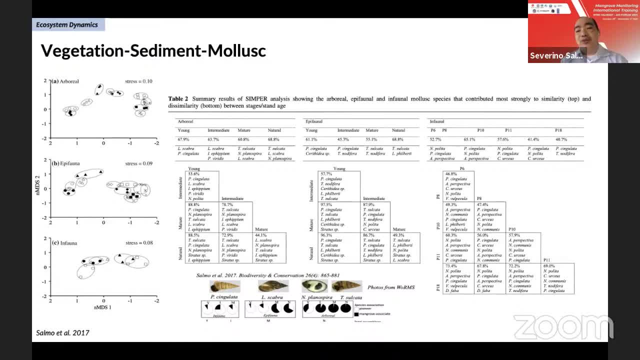 Again, let me qualify that statement. You can only do this comparison if, and only if, you have a reference system to compare with. Without our reference system, without a natural mangrove to compare with, it will be very difficult for us to assess this relationship. 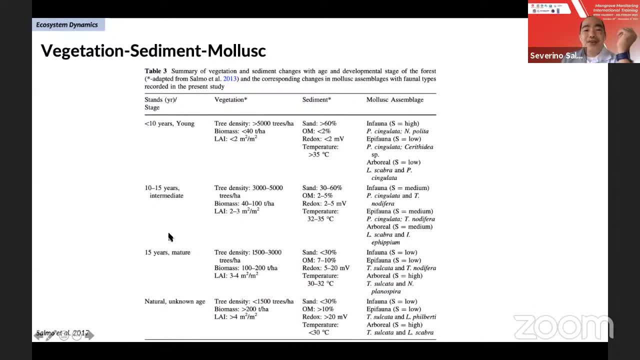 Now I came up with this table. We tried to come up with a description What happens if you have less than 10 years of a mangrove. What do you expect would be the vegetation, the sediment and the dominant species? So if you're young, if the restoration 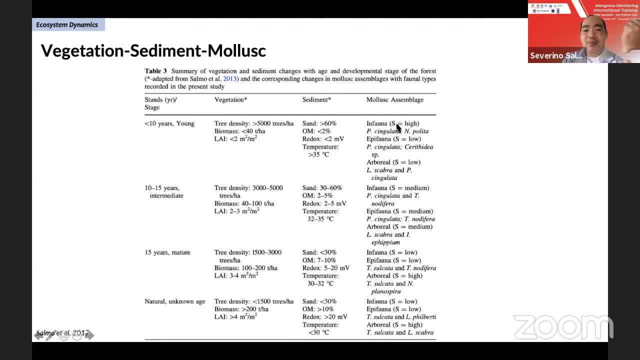 if the planted mangroves is young, then you will expect this vegetation sediment and attributes. But you will also see that slowly there is a shift or a change in vegetation, sediment and mollusk. Now, if the mangrove is mature, 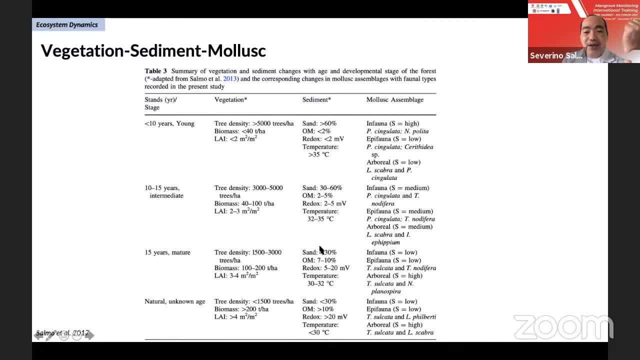 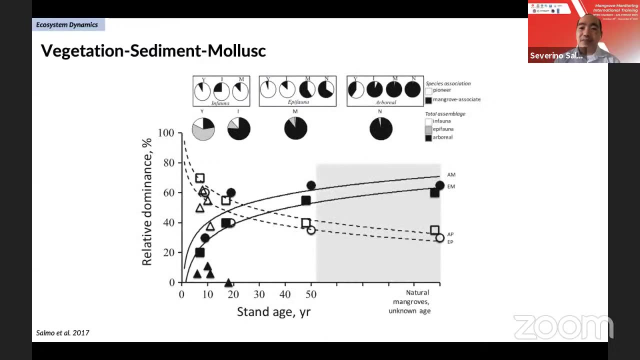 then it is almost very similar with that of a natural mangrove. A natural mangrove not just with vegetation and the sediment, but also with faunal assemblages, the mollusk especially. From that paper we came up with this model. 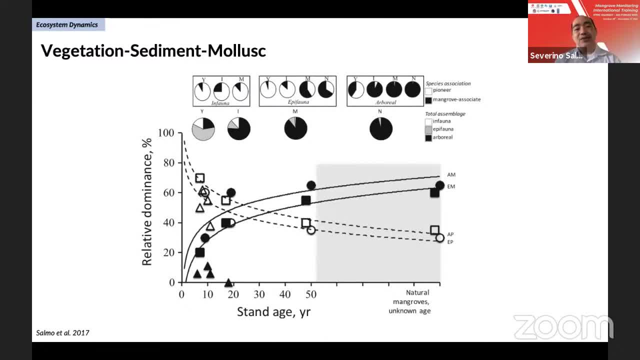 And it's very important again to document shift changes in the assemblages from the pioneer species to mangrove-associated species. Remember, if you plant mangroves now, that could be a good candidate for several faunal species to colonize your planted mangroves. 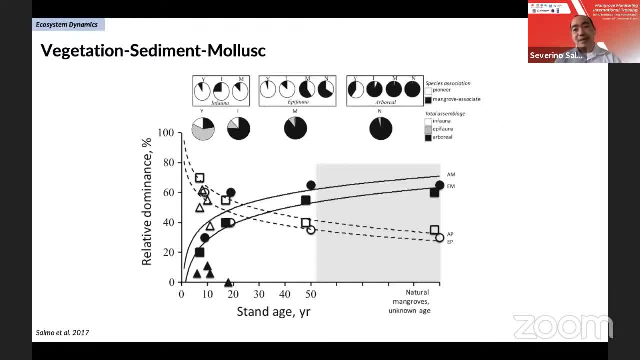 because you're providing a new environment. But what species will come into your young planted mangroves? those are most likely mangrove generalist species or the pioneer species. As the mangroves mature, when the vegetation and sediments develops, then you will be able to see a shift. 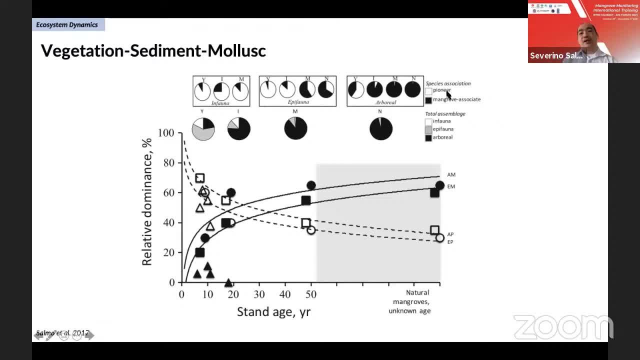 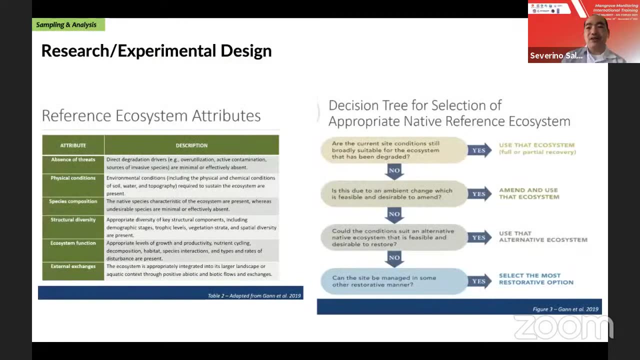 from a pioneer species to those that are mangrove-associated or mangrove-dependent species. Okay, Right, I'm into the third part of my talk. It's about the research and experimental design In doing restoration: ecology research, CER Society for Ecological Restoration. 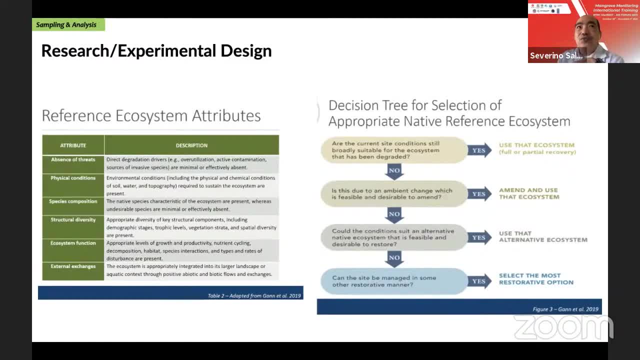 has a very strict criteria of how do you call a reference system a reference system? This table: There are six conditions that you need to satisfy before you can set a reference system. Again, this is not my framework. This is from CER. 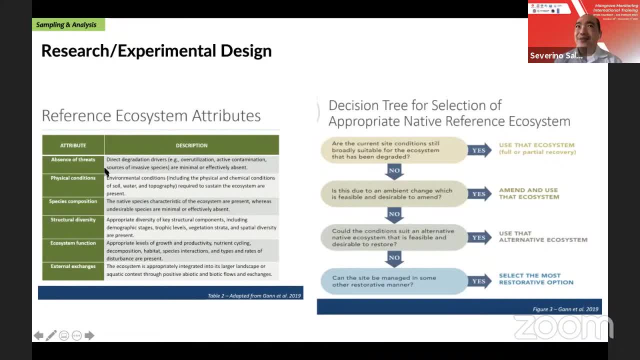 Absence of threats. I don't think in the Philippines we can meet this. There are several threats in the mangroves in the Philippines, So maybe I will not use this 100%. Maybe I can use 50 or 60% of it. 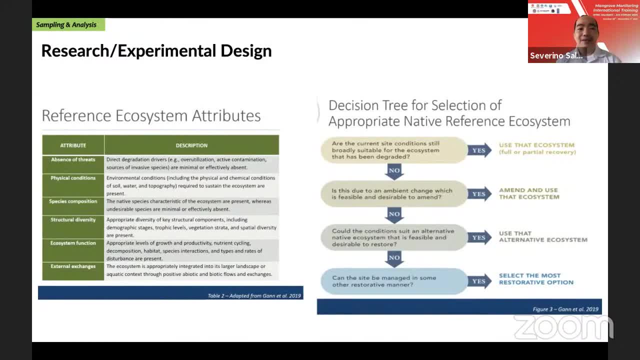 depending on where I am. If it's a protected area, maybe There would be a very minimal threat, Right, But in most cases in the country, in most places, there are a lot of threats. Okay, Criteria number two is the physical conditions. 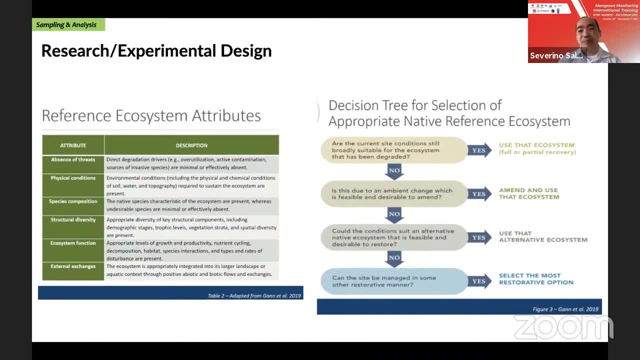 Are the conditions in your mangroves conducive enough for the mangroves to grow and develop? And there's this mention of soil water topography. Okay, Maybe in most cases in the Philippines we will be able to satisfy this. 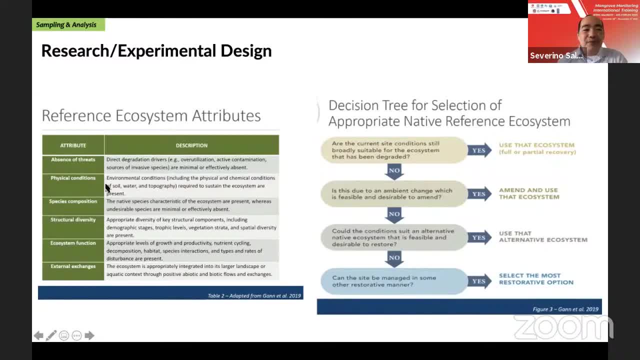 Okay. Now third would be the species composition. Should be the native species that are characterized of the reference system. Okay, You can satisfy this criterion if you know what was present in your reference system, in your natural system. Okay, If you don't have. 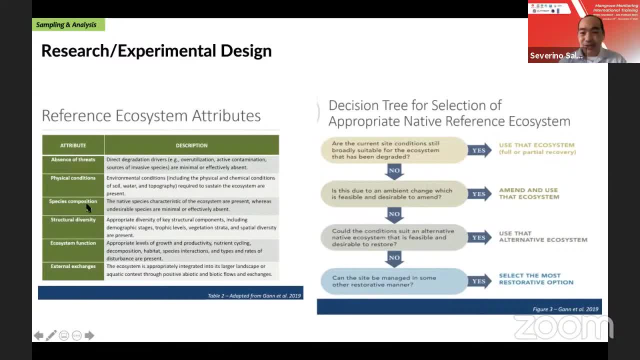 species composition from your natural system, then obviously you cannot do this, Okay. Another one is structural diversity. And how many times do we need to assess diversity in mangrove Right One time? something is not enough. you have to do it properly. 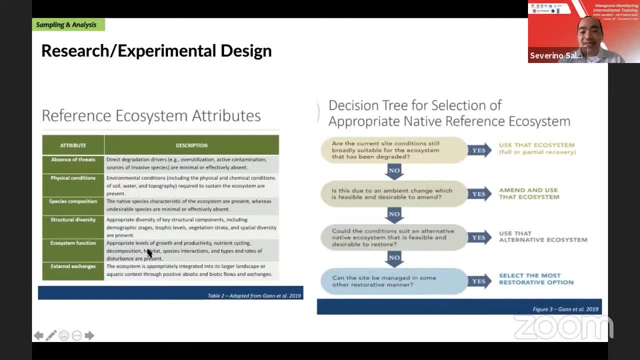 Another criteria is ecosystem functionality: levels of growth, productivity, nutrient growth, nutrient cycling, species interaction and so on and so forth. Another one is external exchanges- Right, Maybe a landscape or seascape context about positive biotic and abiotic flows. 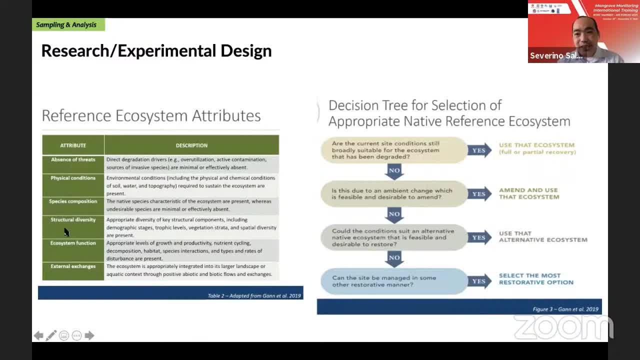 and exchanges Right. Six conditions. Without this, then we don't have a reference ecosystem Right. And then, third, come up with a suggestion of a decision tree for selecting a reference system Right Here, If you don't have a reference system. 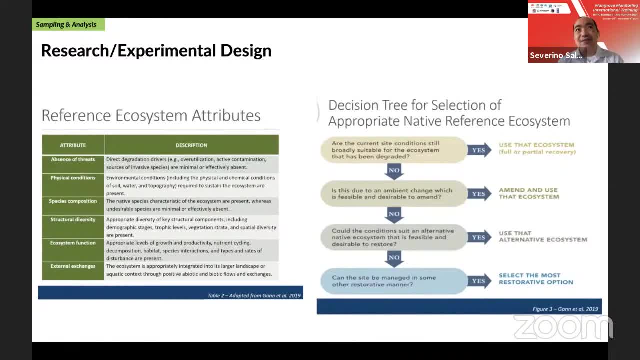 what would you do? Right? I find it funny, but it's also very intuitive. in the website of SIR They mentioned in the absence of a reference system. again, in the absence of a reference system. you have to find a reference system. 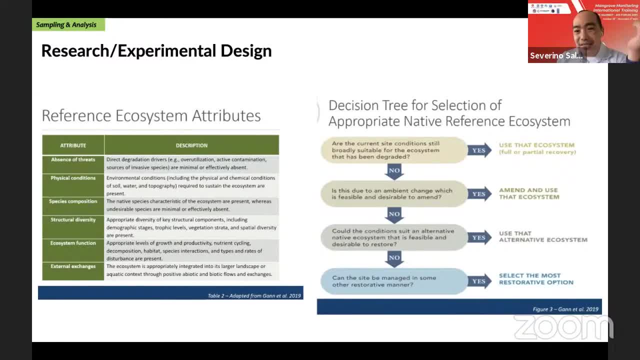 Let me repeat that In the absence of a reference system, you have to find a reference system. How come You don't have a reference system, but how can you find a reference system? Then they qualify the statement In the absence of a reference system. 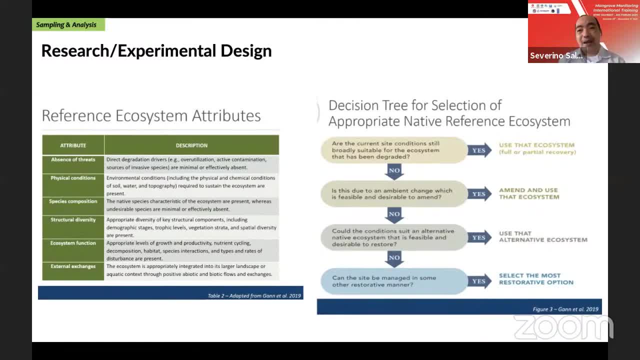 you have to find the best reference system possible. Okay, That's very clear. So maybe we will not be able to satisfy all of this, Maybe none at all, Maybe, But SIR suggested that we have to find the best possible reference system. 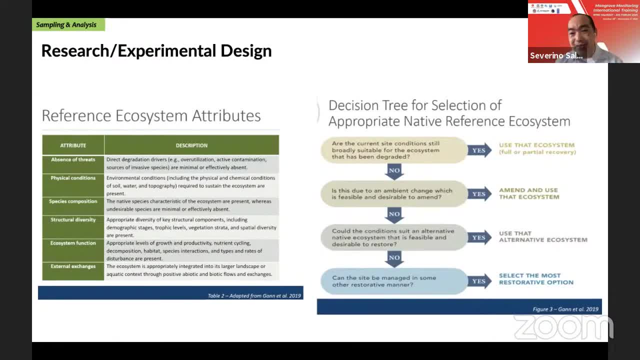 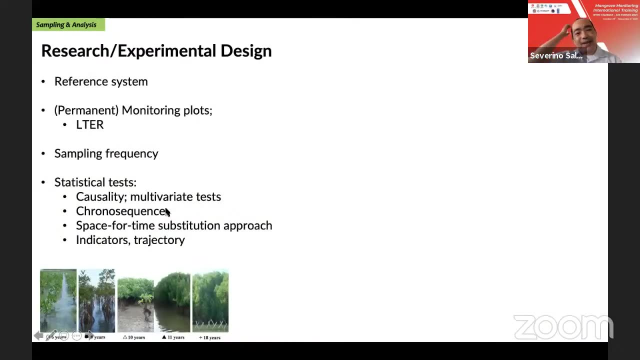 that would be workable now, Okay, But again, it will be a site-to-site basis, depending on where you are. The idea is that you have to come up with a reference system for you to compare with. Okay, Right, So again, let me repeat this reference system. 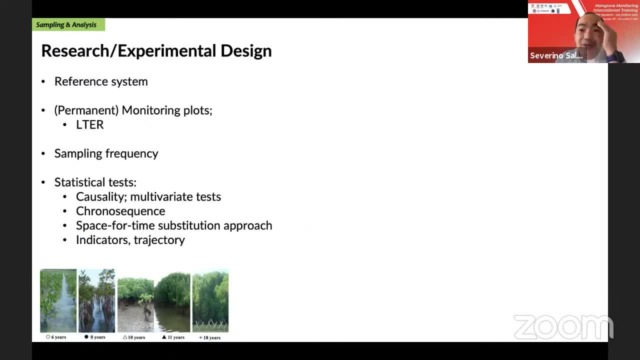 In the Philippines and, I think you will agree with me, even in Indonesia and in Malaysia. it's very difficult to come up with a reference system, Right, But you have some sites in, I think, in Papua. Maybe there are mangroves. 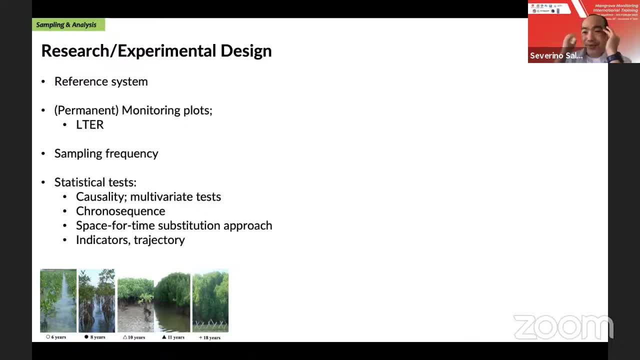 that are still inhabited. That would be a good site. You do that. Do that as soon as you can, because otherwise that may be disturbed. Maybe you will come up with a reference system. Maybe you will come up with a new airport or something else. 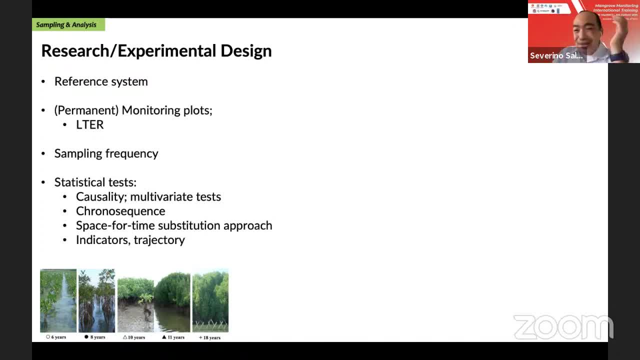 So hurry up After this webinar, go to your pristine mangroves and do the baseline studies. But seriously, though, when you set up a reference system, it's not enough. You have to establish permanent monitoring plans. So, in my case, 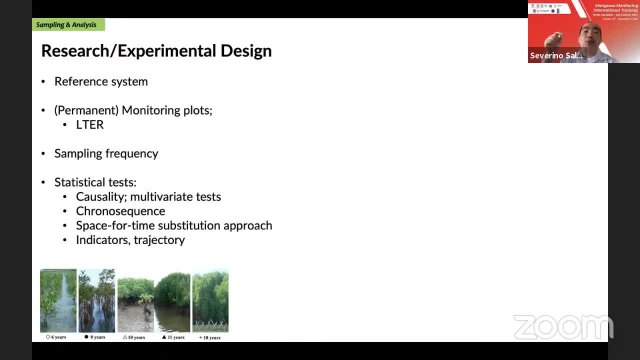 every time I do something, I have this twisty wire and a tape. So when I visit a new site, every time I go to a new site, it's like a hobby for me. I mark my plats The same way that the foresters. 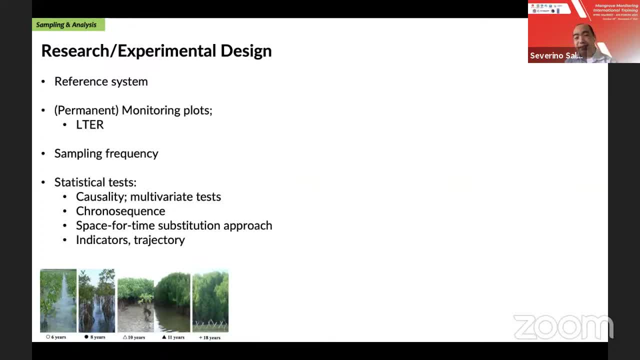 are doing their monitoring, they establish their plats and you take the GPS coordinates so that right there and then you will have a reference monitoring plan And then it's fixed, Unless someone will steal your marker or something else, But at least you know that. 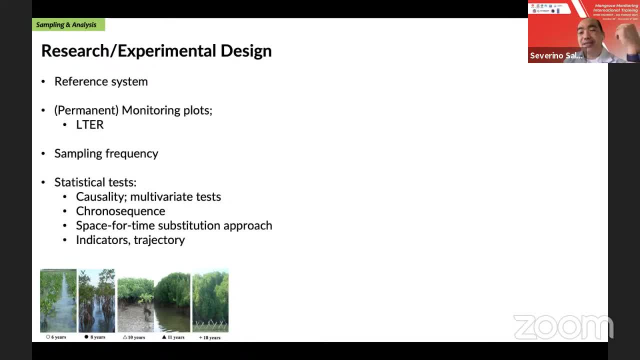 you have a reference monitoring plan And you keep monitoring the same plats over and over again, you will be able to document changes. Another one is sampling frequency. How often do you need to do the sampling? It depends on your purpose. I think in the Philippines. 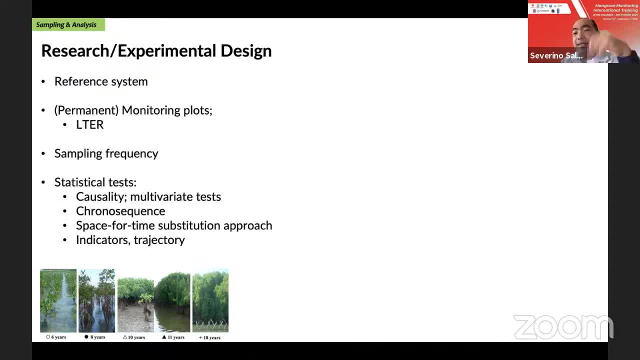 we have two seasons, the rainy and the dry season, So at least we have to do two sampling periods per year. I'll go back to that. I'll go back to this later, I will not discuss this further. but for vegetation, 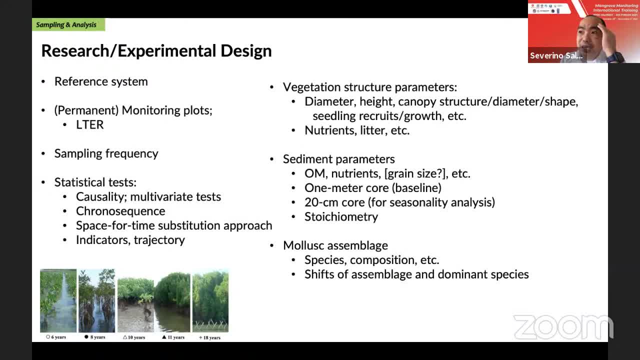 it's like a similar vegetation parameters that ecologists, biologists, botanists and foresters are measuring. It's about tree diameter, tree height, canopy structure, even canopy shape. seedling recruitment, seedling growth rate, seedling survival rate. 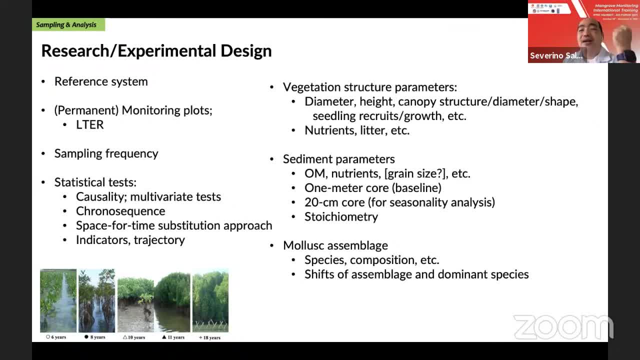 litter production, litter degradation rate, nutrient retention, nutrient recovery, nutrient enhancement. You can do several things. I will not discuss this further. In terms of the sediments, I like the well. the very obvious would be organic matter content. 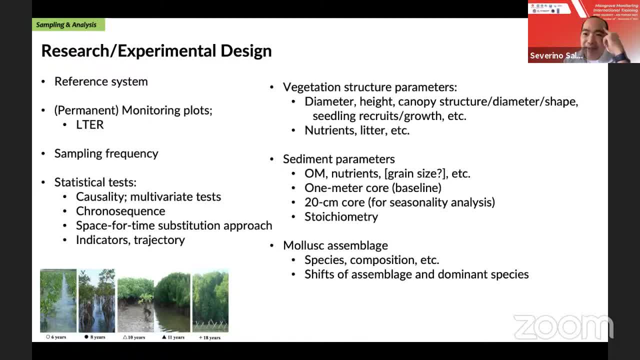 nutrient content, If you have time, even the litter degradation rate. But if I will relate this to sampling frequency, I want to see the one meter core. Maybe you can go even two, even three meters if you can, because that that one meter deep samples. 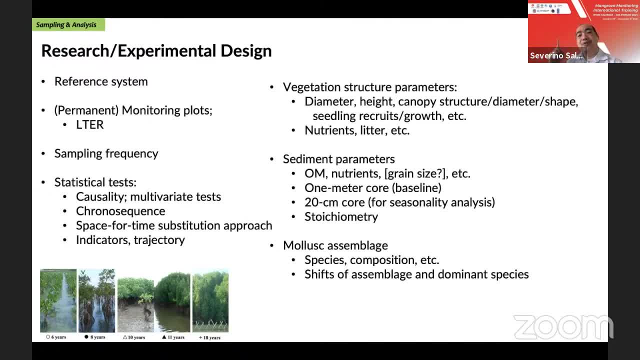 if you do gradation you will be able to analyze patterns, What happened over time in that core right. But for us in the Philippines we do have. we do practice 20 cm depth sampling. We want to account seasonality or seasonal changes. 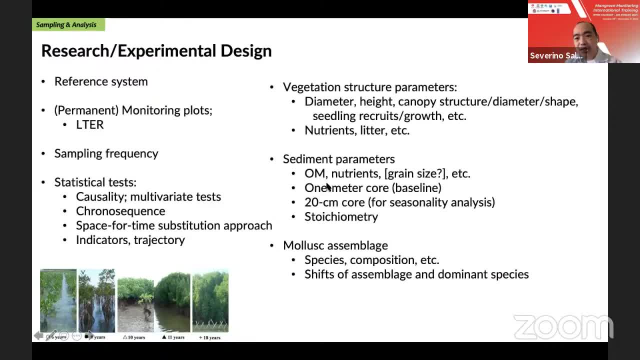 So we do one meter core sample and 20 cm core samples right, And then we analyze nutrient content- organic matter content over different depths- stoichiometry. Then we're trying to see the nutrient ratios: carbon, nitrogen, phosphorus. 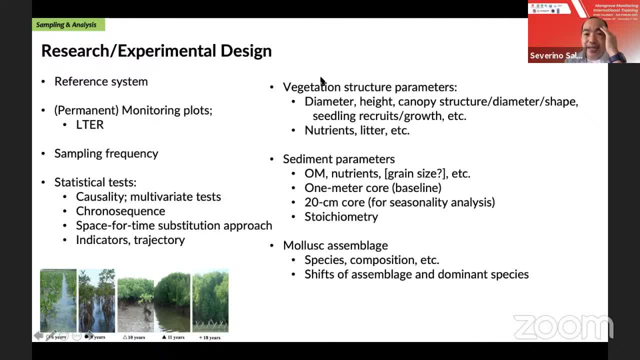 Those are very basic. Then you can relate that between the vegetation and the sediment. You compare lip nitrogen versus that of sediment nitrogen, Then you compare the ratio over time For mollusks. it's all about species composition, species richness, species diversity. 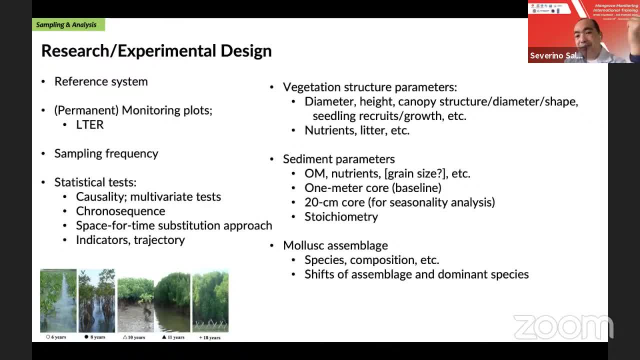 as I presented a while ago in some of my previous slides, But it's not enough. It's similar to the time that you need to capture self-cleaning for vegetation. It is very important if you want to capture faunal assemblages. 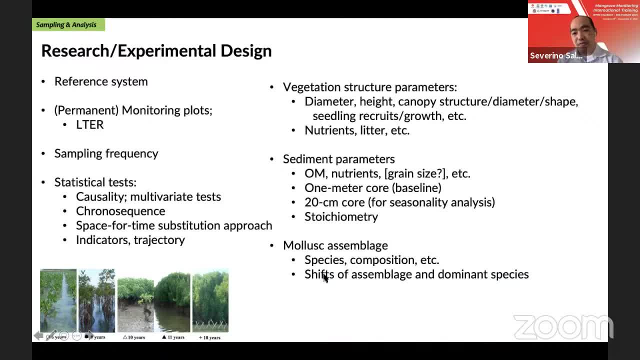 then you have to document the shape in dominant species and the shape in the assemblage type. Maybe you will have initially high in faunal density and in faunal biomass If you have a productive mangrove, if you have a good, healthy, restored mangrove. 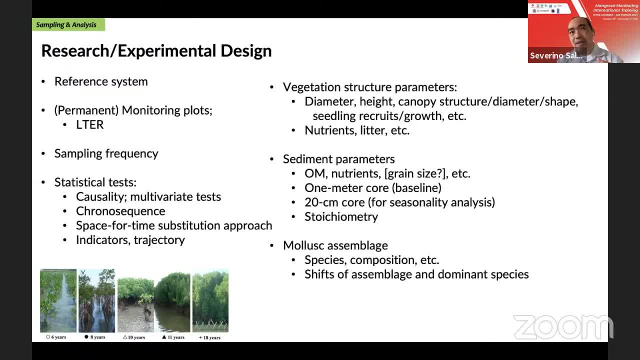 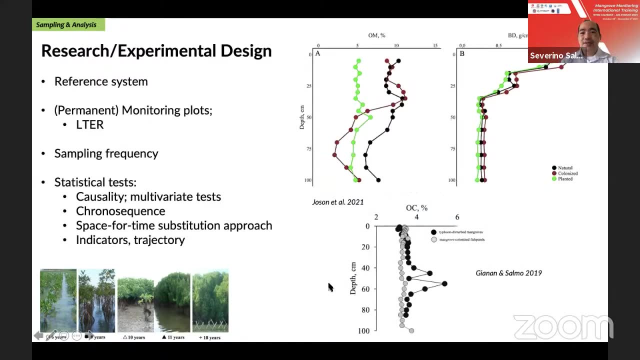 then it should be very common that you will have higher density, higher mollusk biomass in the arboreal and in fauna than that of the in fauna, And you have to capture that shape Right. Stoichiometry here. I forgot this. Hold on. 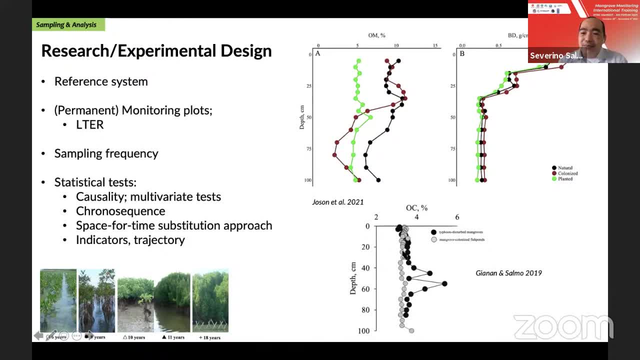 See here: This is the restored. This is the typhoon damage mangroves- This is mangrove. colonized fish plants. tambac- here. We know that here. maybe this was the time wherein tambac was constructed and therefore it resulted to massive loss in carbon. 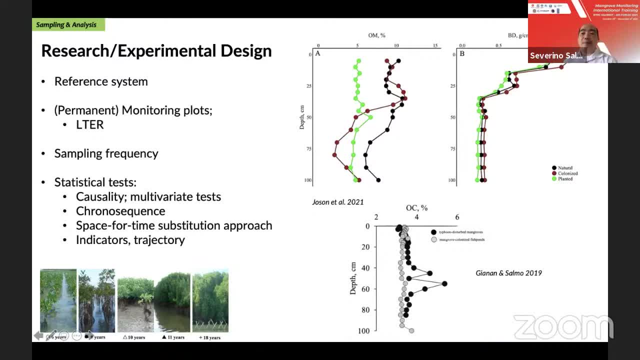 in organic matter. But then when tambac was abandoned, there was this mangrove colonization mangrove goat and then it was able to recover some organic matter. Unfortunately, that mangrove was hit by a typhoon, So there was again a dip in here. 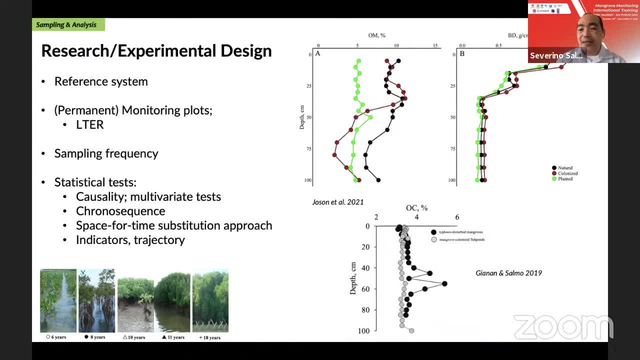 Maybe it's too small here. Now the other trend is this one: here You do. We have similar practice. I mean Indonesian Philippines. When you do, when you construct fish plant, you excavate mangroves, right, So you clear. 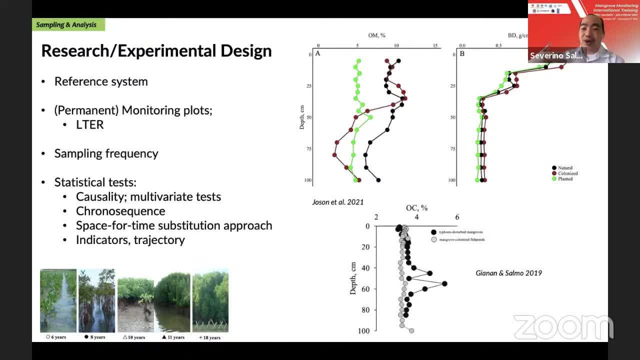 you clear the mangrove vegetation, but you also excavate one meter, maybe two meter deep sediment And therefore this would represent the loss in carbon right. When the mangroves grow and recover, then you will be able to see increase in organic matter content. 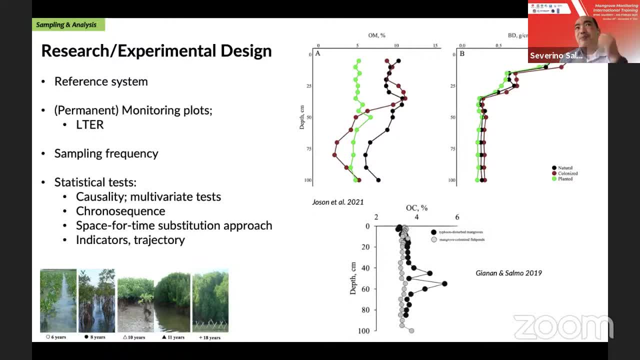 Okay. So that's the good thing, If you see, if you, if you assess sediment at one meter deep, because if you only assess 20,, 20 centimeter deep, then it may not be enough to capture the history of that site, right. 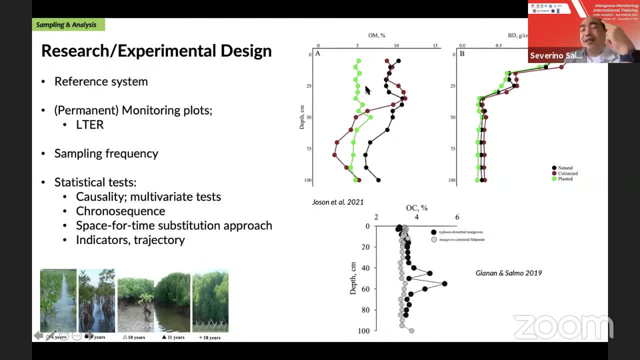 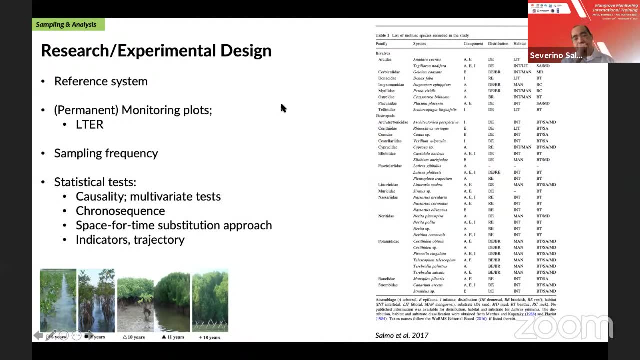 I forgot this thing. I think this was the site that was affected by Mount Pinatubo eruption. Natural mangroves, the planted mangroves and the colonized mangroves- they have a different organic matter content over them Now. 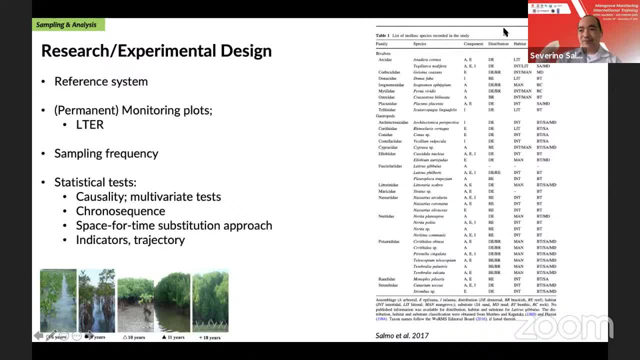 for the mollusks we usually collect. biologists love to collect specimens, So we do collect animals, identify them, put them in the museum and so on and so forth. But then we also assess: what component are these samples in? 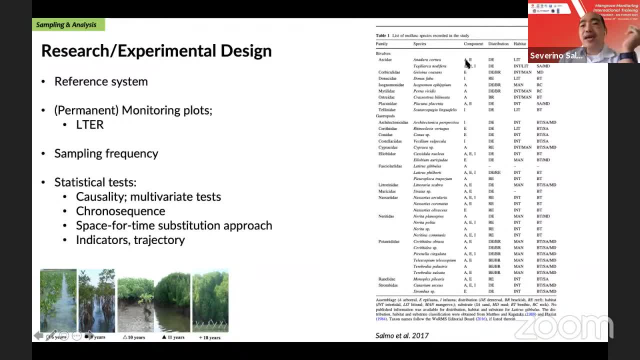 Are they found in A arboreal, E in epifauna or I in fauna? Or is that particular species only? is that particular species present in all assemblages? Yeah, Or maybe there are species that can be found, can only be found in epifauna. 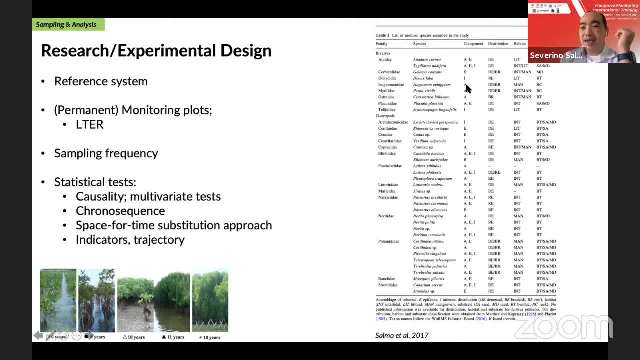 in fauna or in arboreal right. So that's a component. The other one is the distribution. I forgot, Is it the mersal brachys? Sorry guys, I forgot my terminology here. right, Then we also describe the habitat. 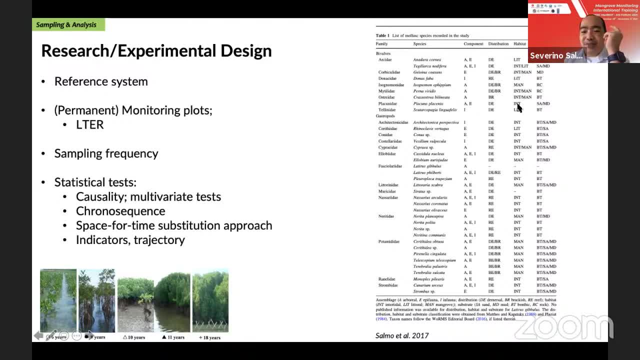 Is it littoral, intertidal? Is it mangroves? I use the reference by Matz and Kapetsky. Maybe there are newer references now, Plus shot, for example, But the new guide for marine species identification by Worms. 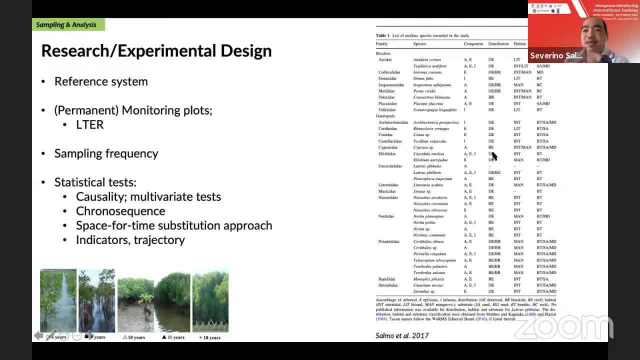 World's Register of Marine Species. Then you characterize the substrate type: Is it sandy, muddy or I forgot this thing Right? So, aside from collecting the specimen, you have to describe the family, the species and the other things here. 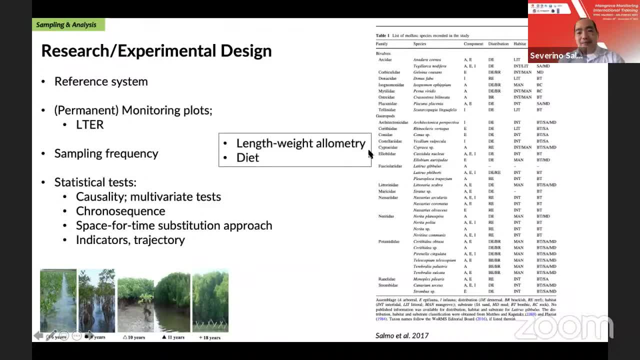 Yeah, just like what we did. Okay, But aside from that, we also analyze the length, weight and geometry of the mollusk, The length and the biomass of its collected specimen. It takes a lot of time to process everything, And I was doing my PhD then. 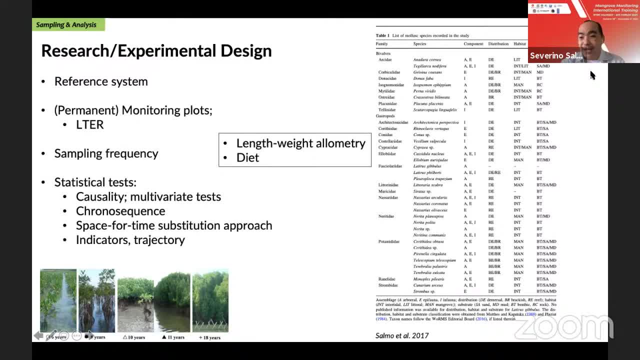 If I'm not attending conferences, I'm only doing my PhD. I devoted my time doing this thing. When I am doing my PhD, I think I collected more than 10,000 mollusks, Mollusk individuals. I measured those in my three to four years of PhD. 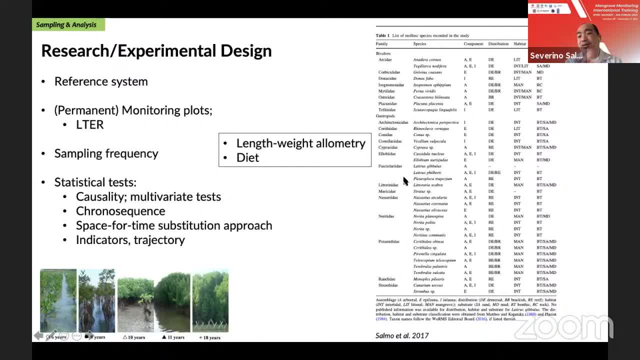 That's a lot of samples. aside from the vegetation sediment, I also did the necton sampling. It takes a lot of time And a lot of measurements that you need to do, But there could be other things that you need to consider. 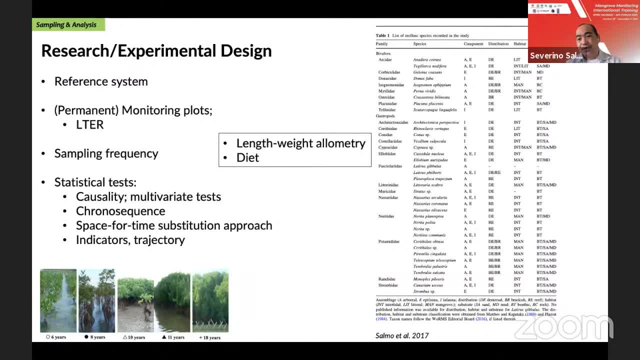 For example, the use of isotope to analyze the diet of the organism, Right? So those are the things that have to be considered in the sampling. In restoration ecology there's this always challenge on causality: How sure are you that the vegetation 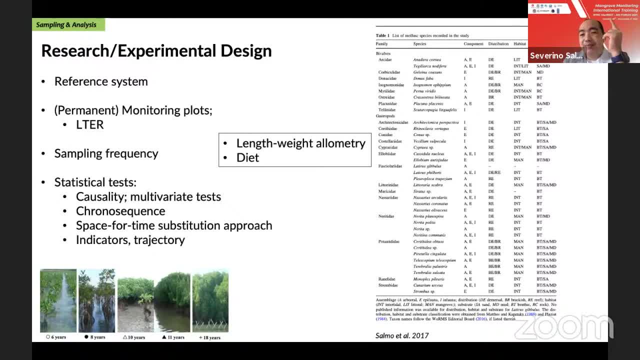 sediment and mollusk assemblages are attributed to the restored mangroves. Maybe you observe vegetation, sediment and mollusk because it is very close to unnatural mangroves Right. Usually you do chrono sequence just like this In one site. 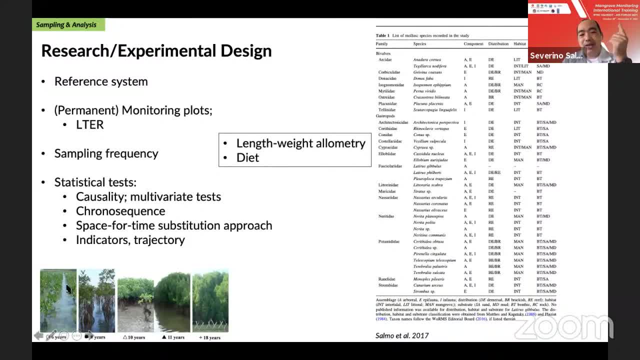 you compare what is the vegetation, sediment and mollusk found in 6-year-old, 8-year-old, 10,, 11, and 18-year-old? And, for that matter, the site in Matang is a very good classic example. 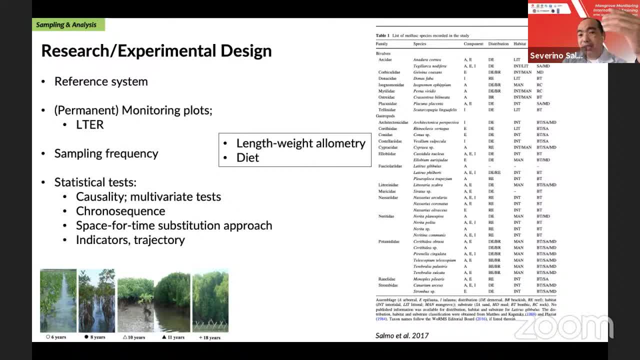 because they know the age of the mangrove. But in most cases this chrono sequence is very difficult to establish. Right Related to chrono sequence, the SFT, what they call the space-for-time substitution approach- If you know the age and if you know the development. 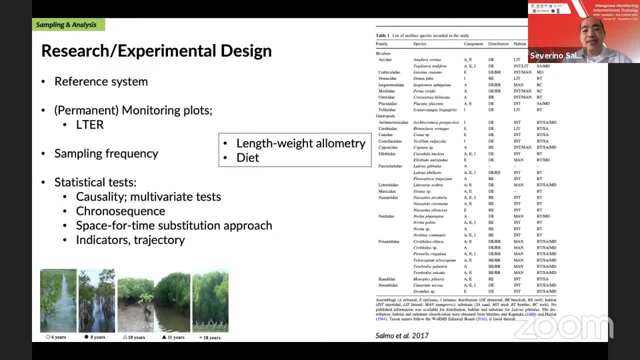 then you can infer or hypothesize that this could be a possible changes before and after the restoration. So I mentioned causality, chrono sequence and space-for-time substitution approach. More often than not restoration ecology studies are constrained with the normality of the samples. 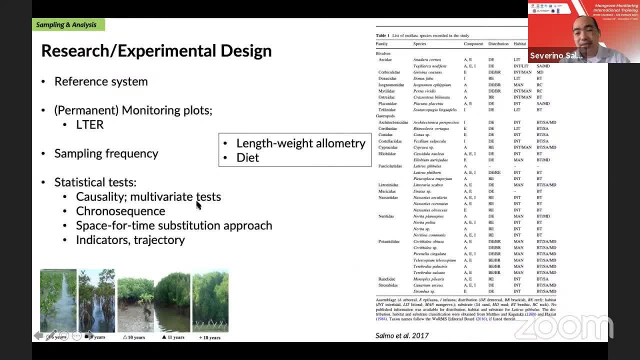 So most likely we will be using multivariate tests and ordination techniques, because we want to attribute the changes in vegetation, sediment and mollusk to that of the restored mangroves. To do that, then you will be in the right position to say: 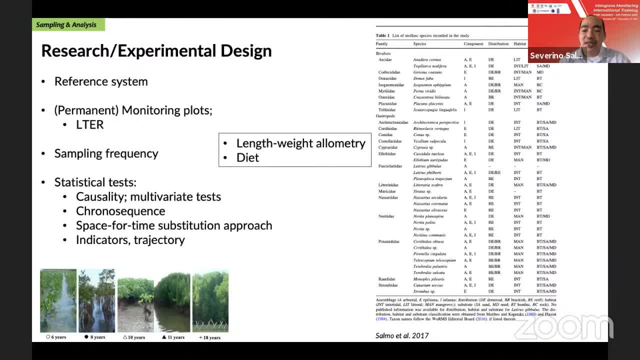 what would be a reasonable restoration indicator? And, more importantly, where am I? Where are you in your restored system? Are you in time 0? Or in time 10?? Is your progress in 100% Or 0%, Or? 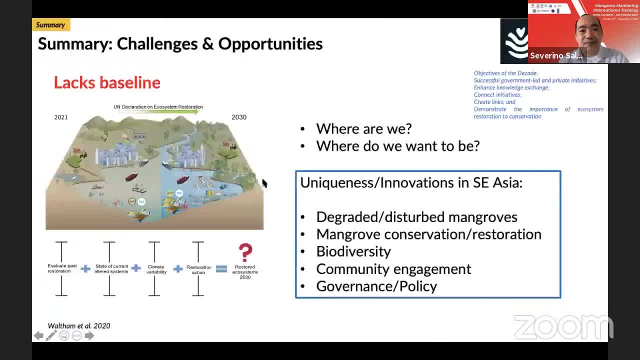 maybe in between. Okay, Right Down to my last two slides. This decade is about the UN Decade on Ecosystem Restoration. There are several programs, There are several objectives there. Hopefully, we will not wait until 2030 to see each other again. 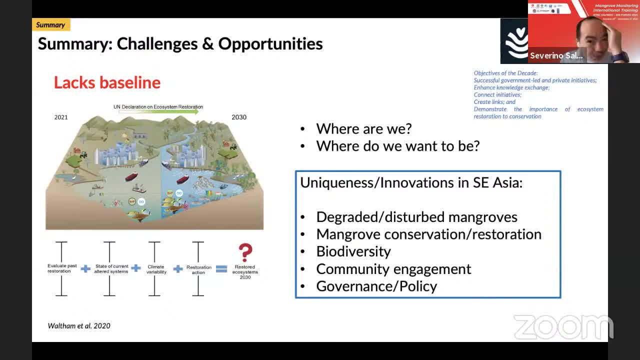 Yeah, yeah, Maybe we can see each other soon, Soon enough, all of you, We don't need to wait for 2030.. But your government, my government, signed for this treaty. There's nothing that we can do anymore. 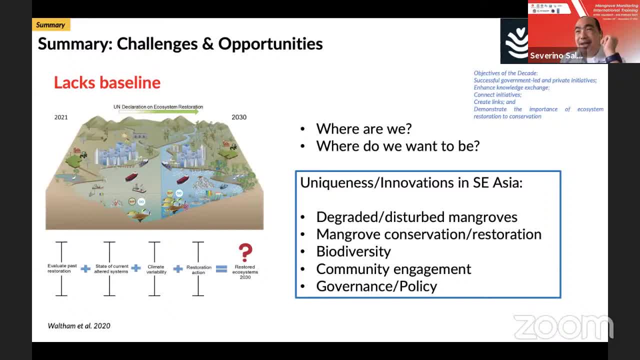 Year 2030, it's like a payback time. What have we done this year until 2030?? We know that we have problems with baseline. We lack baseline. Maybe in 2030, it will still be there, I don't know. 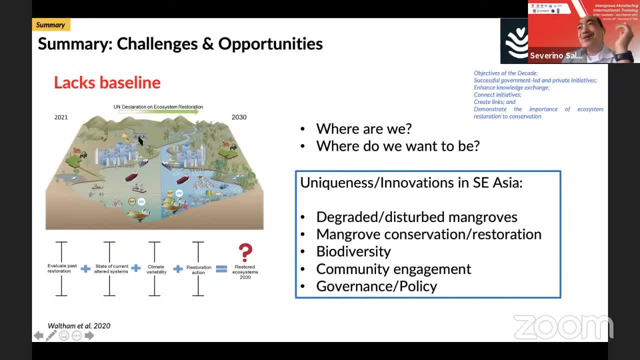 Still no baseline? I hope not. Maybe there will be a reduction in that issue on baseline. Where are we now? This is 2021.. Where do we want to be by 2030?? And there are unique mangroves in Southeast Asia. 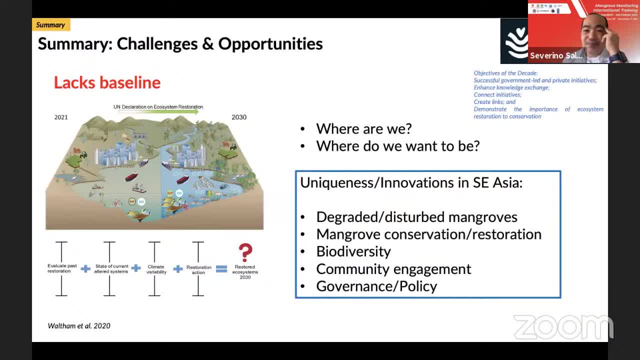 I'm not just referring to Philippines and Indonesia. We know that there are a lot of degraded and disturbed mangroves. If they are degraded, then those sites are already good candidates for restoration, Whether they will follow a healthy mangrove or a restored mangrove. 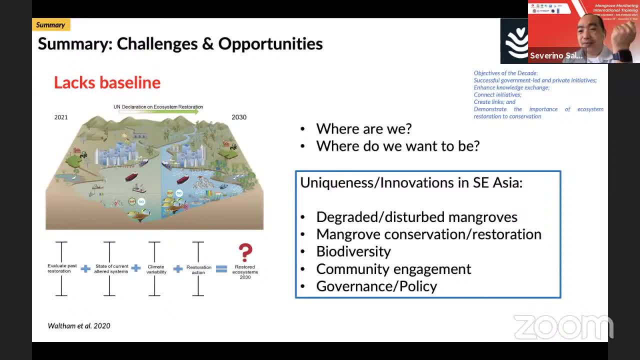 would be something for us to look at. If we actively manage our restored mangroves, biodiversity and ecosystem functionality will be high come 2030.. And again, very unique to Southeast Asian countries is that there are community engagement in terms of the restoration. 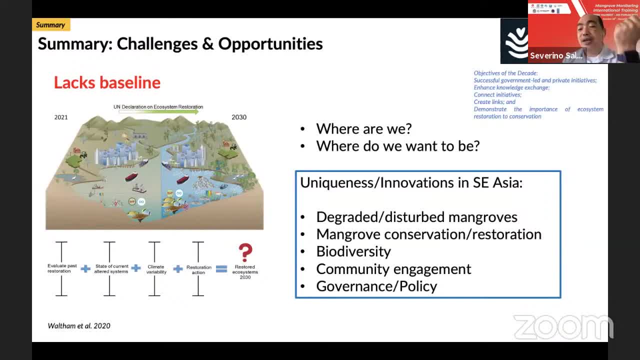 and conservation, and also with regard to governance and policy. Dr Siddiq sent me a slide before wherein school children are actively planting mangroves. We do have similar cases here- Not so many, but at least there are some places in the country. 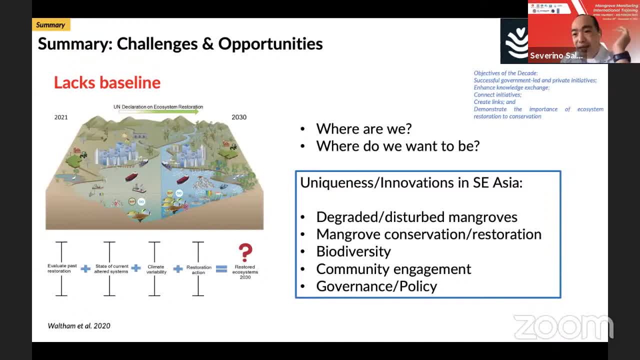 that are practicing community restoration projects, Very unique for Southeast Asian countries. So we are here 2021.. suggested that we evaluate our previous restoration program, So we look back. What have we done since 1990s In the Philippines? we do have 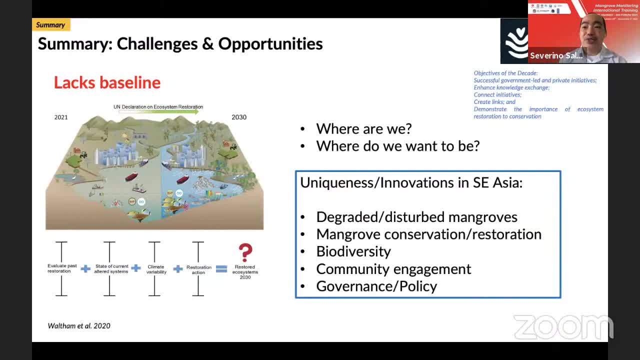 well, even Indonesia, you did have good restoration programs. Are they successful? Are they a failure? Are they still undergoing progress Come 2030,? I hope we are not evaluating those restoration programs anymore. Maybe we will be in this direction already. 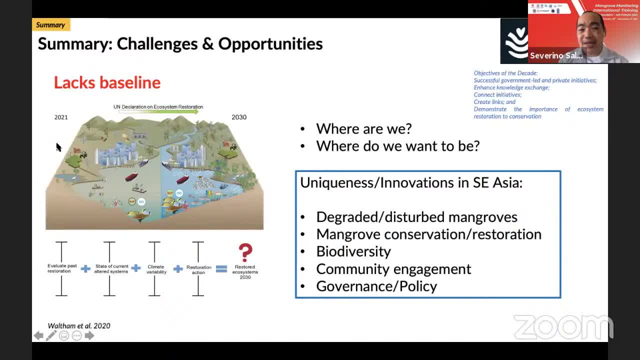 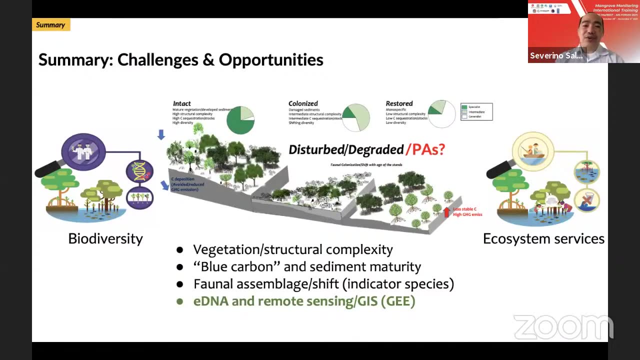 I hope, Because if you are still stuck in here, then we can say in 2030, something didn't went well Right Now. for me, this is our priority. for now We want to do a comparison of an intact mangrove. 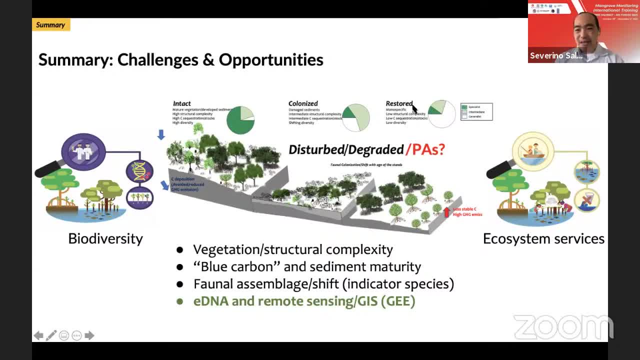 a reference mangrove versus that of a restored mangrove, And we want to factor in colonized mangroves. What will happen to the thumb back areas if we will just let them abandon? Why not? Why not Do restoration programs in thumb back areas? 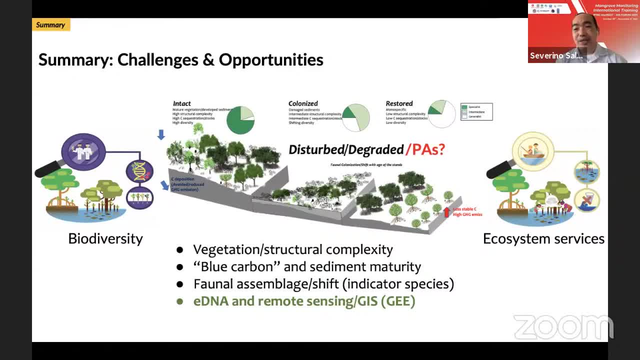 Right Because it's abandoned already. Why not do it more productive? Right In the Philippines? because we are signatory to the IUCN treaties, we will always be prioritizing biodiversity and ecosystem services, And maybe in Indonesia, in the case of Indonesia. 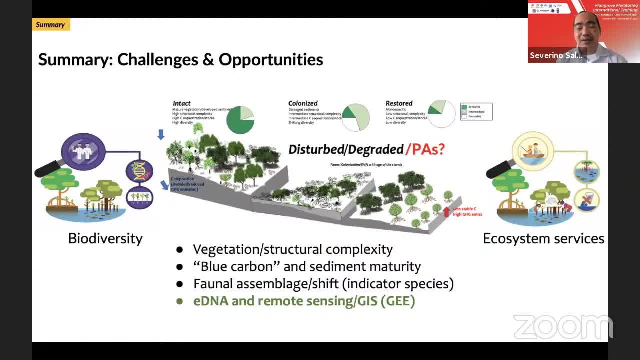 blue carbon, the same way that we are prioritizing blue carbon. It's very famous now: the eDNA approach. I'm collaborating with another Indonesian guy. I don't know if you know Basuni. Do you know him? I know him. 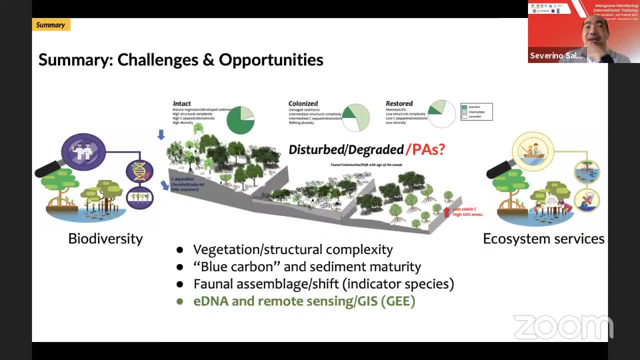 Yeah, yeah, yeah. So we are collaborating with the JSPS in a JSPS funded project, together with the Dashi Sensei. This is a revolutionary approach. We want to assess biodiversity in different types of mangroves. I said revolutionary because it's relatively new. 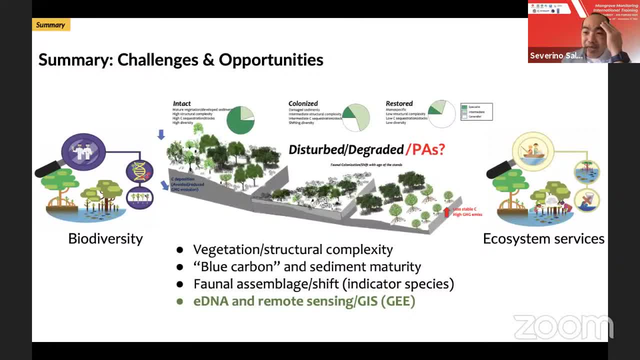 but we haven't done anything yet. because of the pandemic, We never had the chance to do sampling. We never sent the samples to Japan yet, And it's very difficult at the moment. I don't know when we can do the sampling, And this morning. 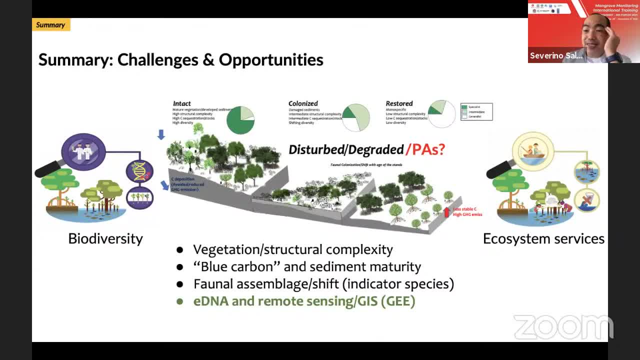 I've heard you guys. I wasn't able to finish the morning session. It's very difficult for me, but I'm willing to learn. That's why I will be requesting Yaya to send me the training materials I want to know. 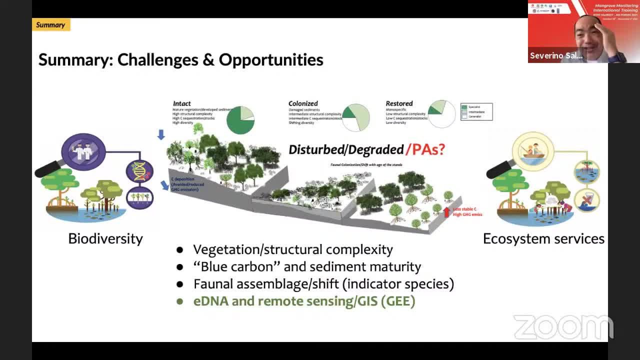 and maybe that will be a good learning skill for me in the next coming years. These are the challenges and opportunities. GEE is almost synonymous to environmental DNA. Those are relatively new tools. Maybe come 2030, we will be able to come up with more intact mangroves. 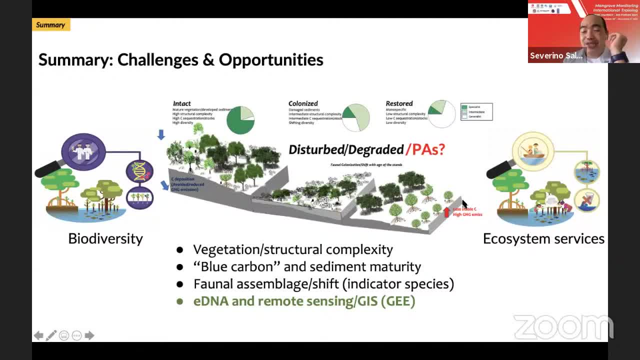 And very few disturbed mangroves, Because we believe that by then, by year 2030, the restored mangroves that we had in the past will be somewhat synonymous already to unnatural mangroves. And thank you very much, Thank you so much. 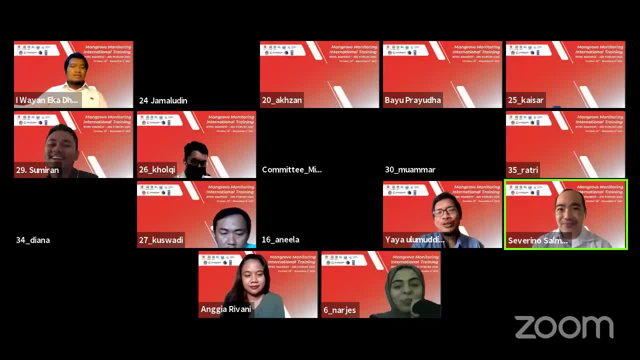 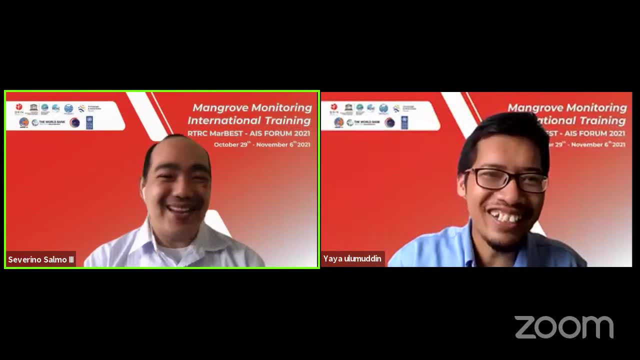 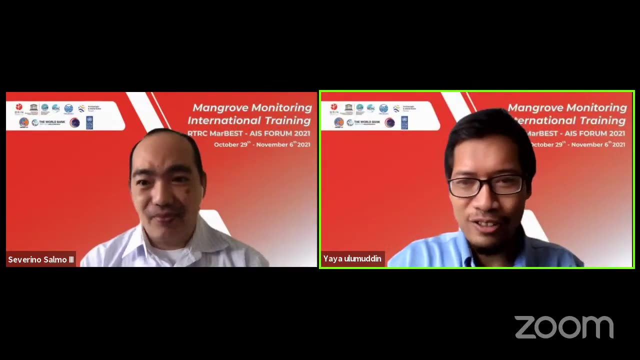 Thank you very much, Thank you, Thank you very much, Thank you, Thank you. Oh, nice, Nice one, All right, Thank you again, Dr Severino-Samo. That's a very interesting topic And it's very related to our training today. 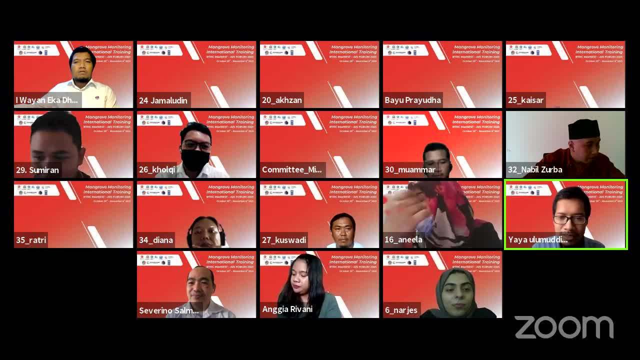 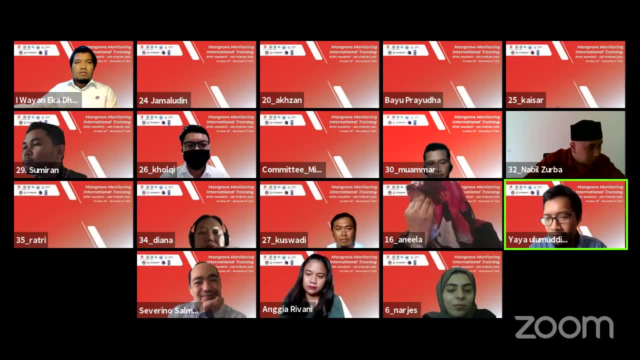 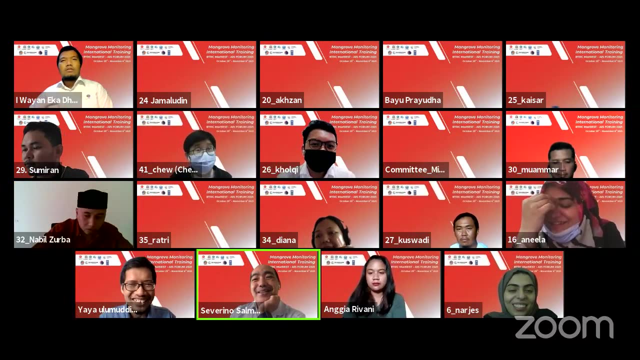 this week, So it's time for discussions. We still have plenty of time, If we look at the schedules, until 3.30 pm. Yeah, Yeah, Yeah, That I will be speaking for 45 minutes. I think I went more than one hour. 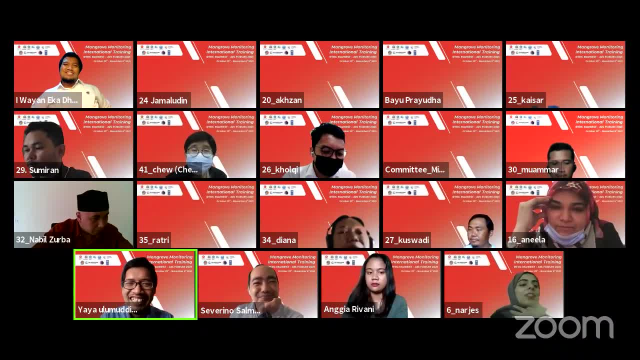 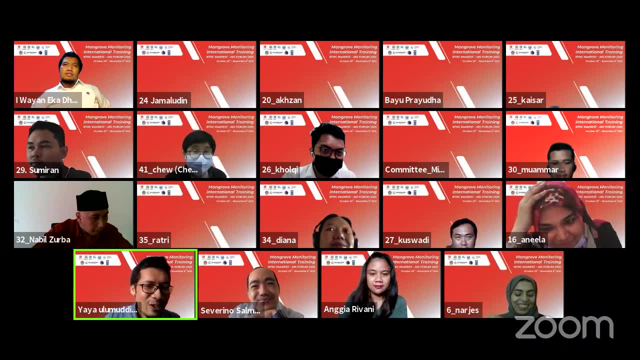 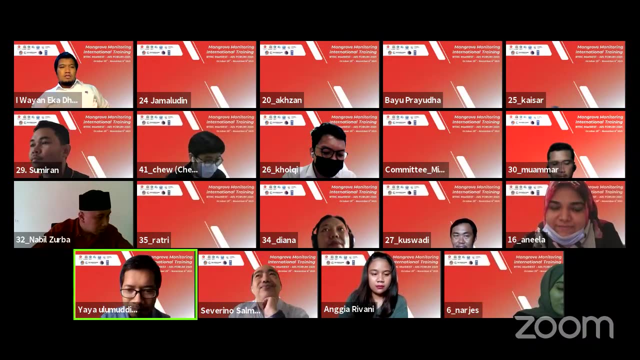 Yeah, Don't worry about it. Don't worry, Yeah, So please, if there's- Oh, it's already two, Somebody raised their hand. Three, Okay, So first question will be from Anggia. Please, Please, Anggia. 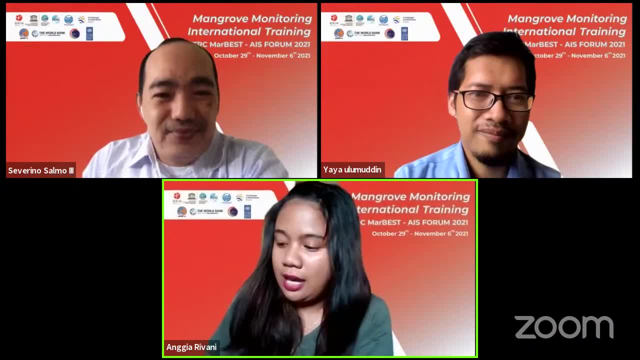 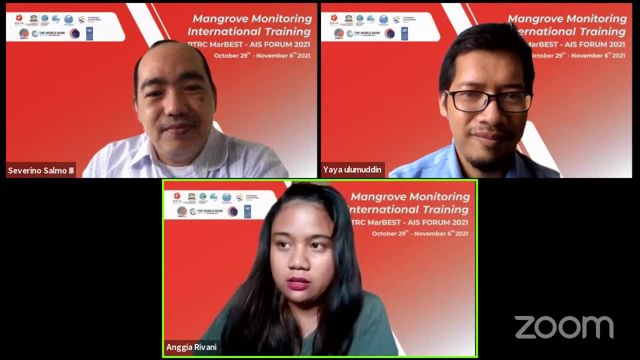 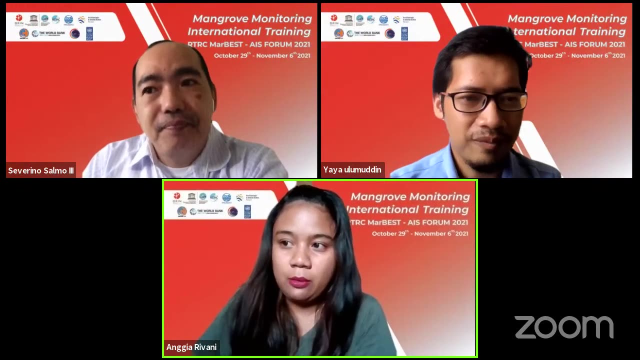 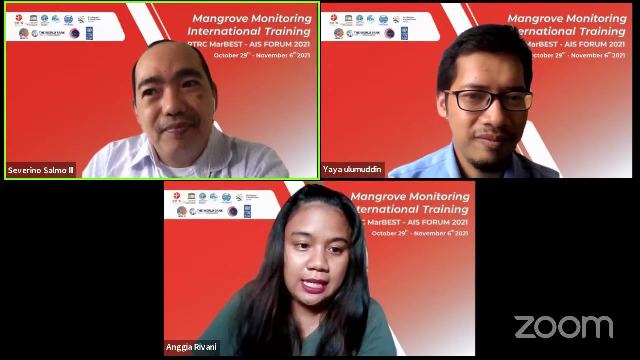 Hello, My name is Anggia, from Indonesia. I'm working in marine protected area in Indonesia. As you mentioned earlier that restoration is a process of reversing a degradation. In this case, what if this area not experiencing degradation? Do you think this area still need restoration or not? 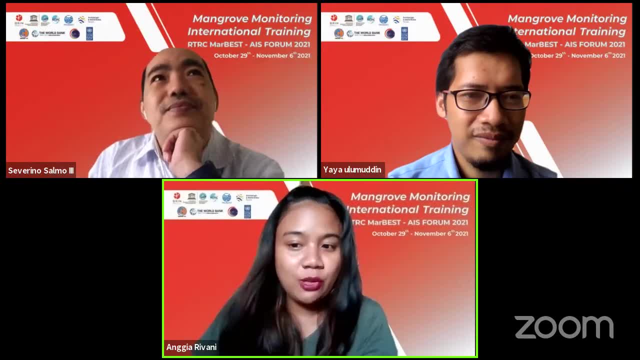 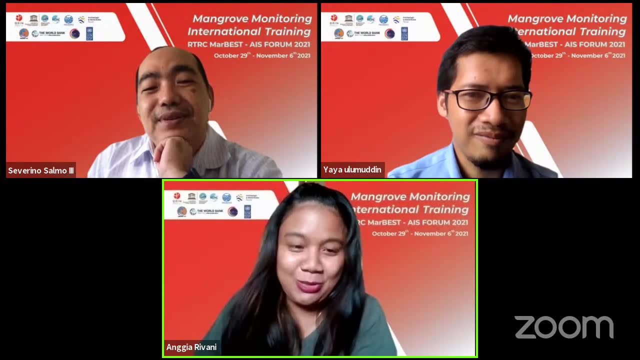 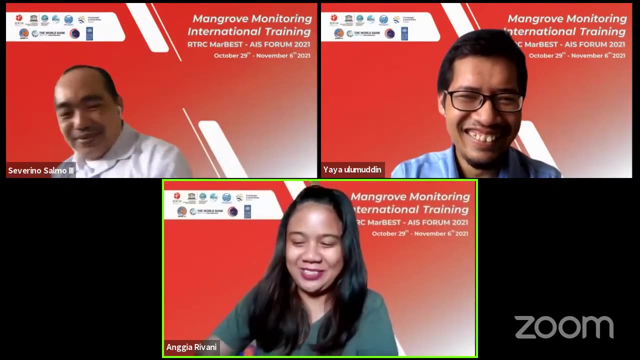 And what if this area is marine protected area? Yeah, Yeah, Yeah, Yeah, I got your point. Yeah, Yeah, I have two question. May I? Yeah, Hold on. I need my pen. Yeah, Okay, Sure. 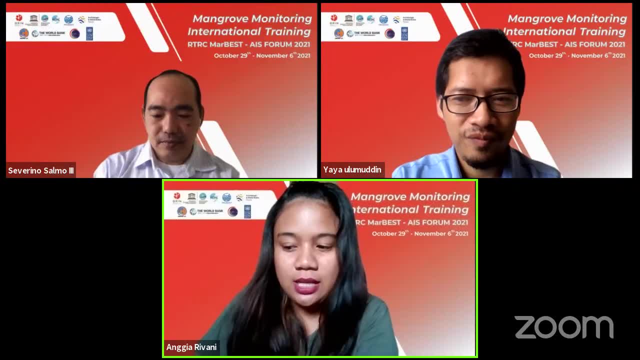 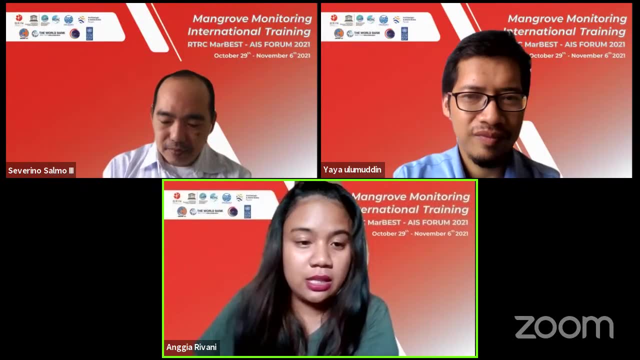 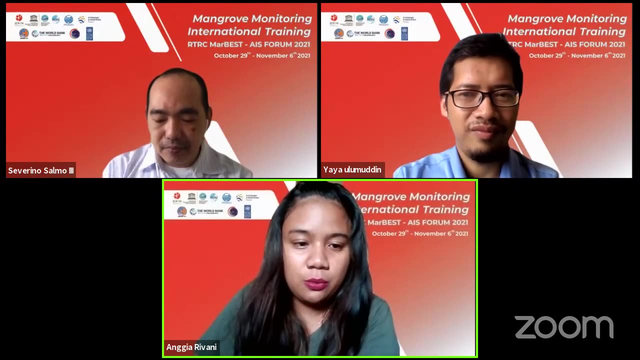 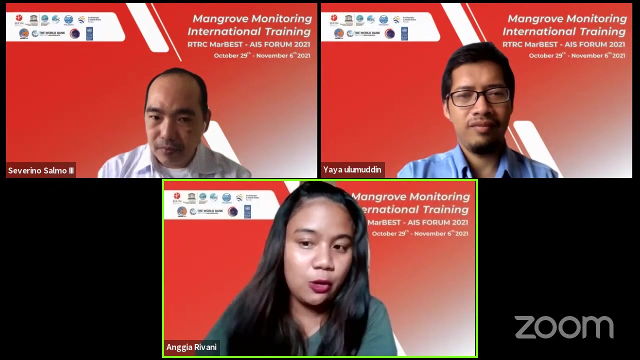 Okay, Go on. And the second question, that the picture you show before in your presentation is the result of restoration. The tree is very tall and dense. What factor affect that the growth of restoration? Is there any special treatment or just let it be? 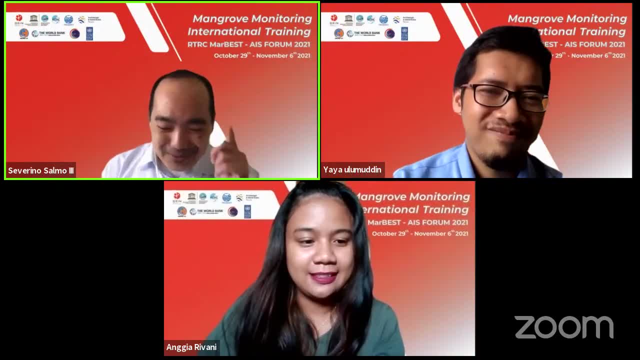 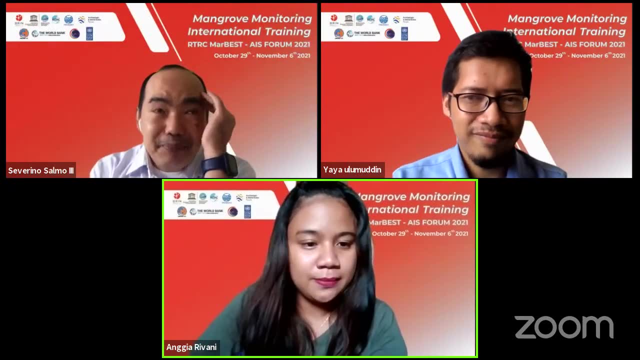 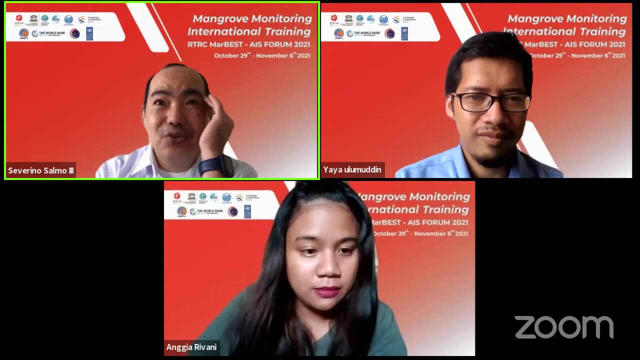 Thank you, I will have to ask you again for the second question. Let me answer the first question first. Okay, If the site is not degraded and it's already a protected area, my answer is that: why will you do restoration program there? 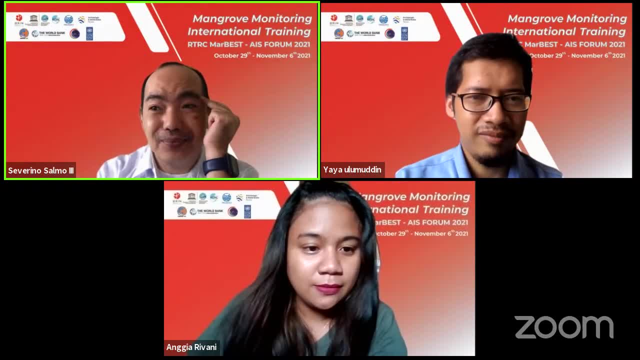 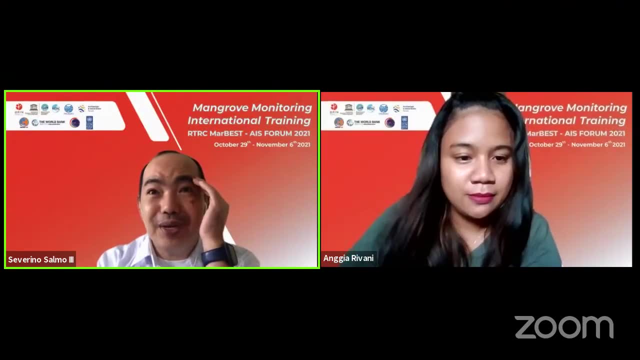 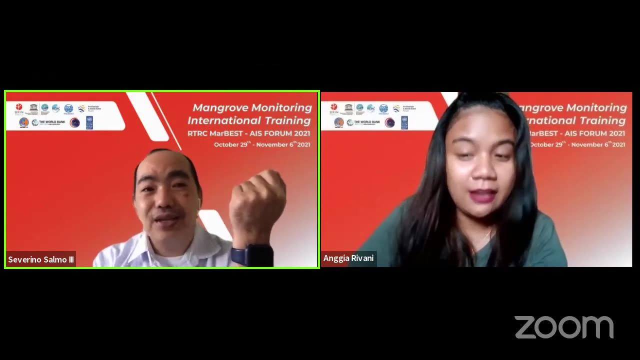 We have cases in the Philippines like that And I don't know. I don't see the reasoning, But we've been doing that. Well, if you have money, why not? If you have the time to spend, why not? But there are other degraded areas. that needs to be prioritized. 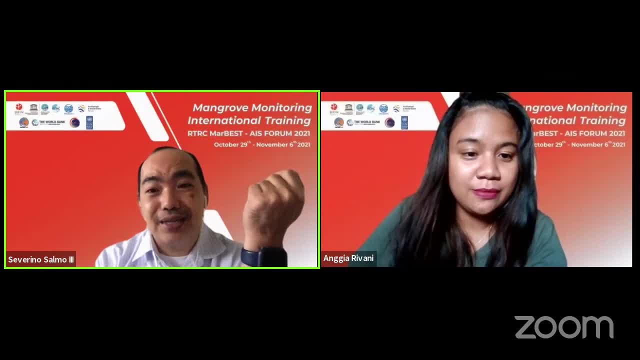 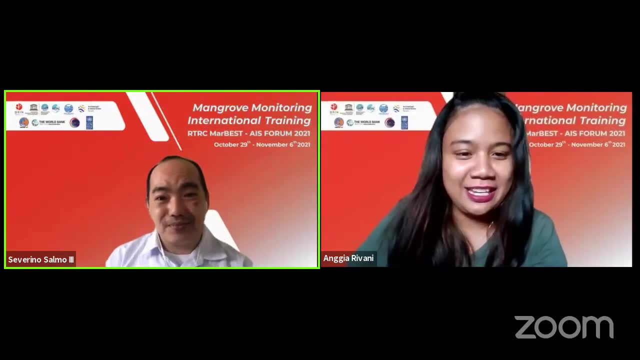 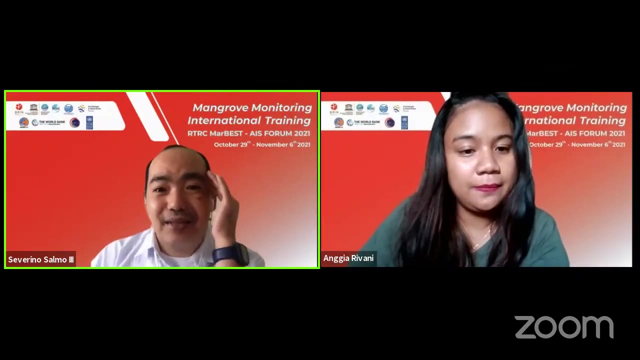 Why? Why don't we do restoration in the restored site, Right, Right. Well, if you have the money and personnel, why not? If we have the money, why not? Yeah, But it's not a priority for me because it's already protected. 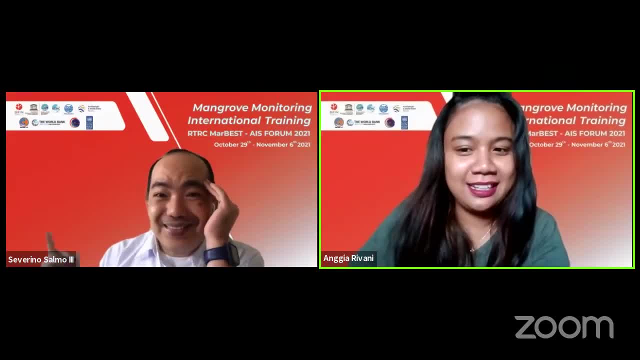 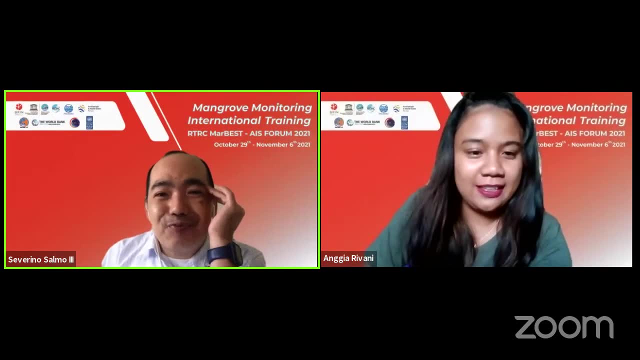 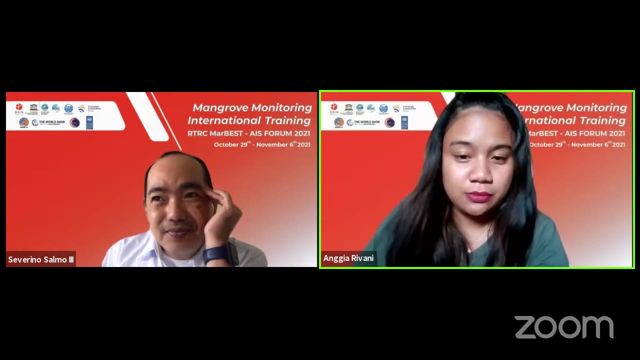 Why restore? Yeah, That's confusing, because this is marine protected area, Exactly Then why, Exactly Now? pardon me, I have to ask you for your second question. The picture that you show on your presentation show the tree is so very tall. And then what factor affect that growth of restoration? Is there any special treatment, or Yeah? Well, in mangrove biology and mangrove ecology, different species will have different preferences And sometimes, When you plant mangroves in areas that are above the mean tidal level, that's the site. 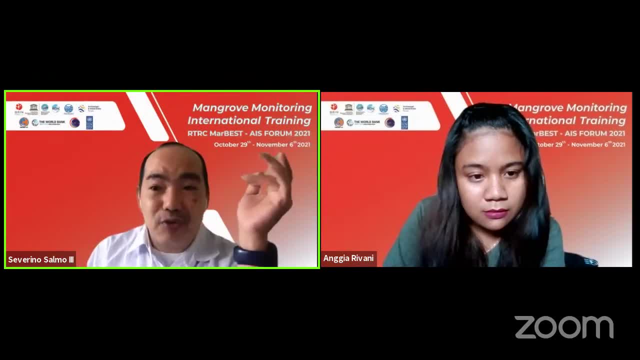 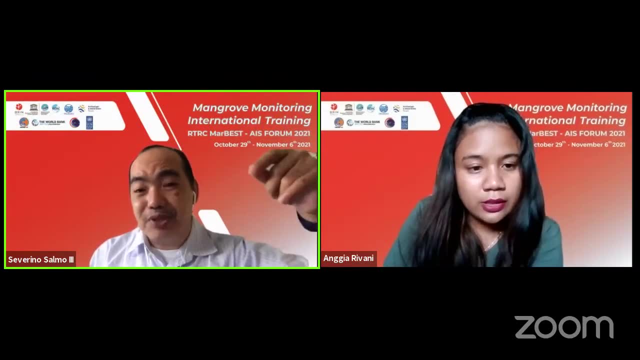 wherein the mangroves will favorably grow. They don't want to grow in the areas that are inundated, Right? So if you see stunted mangroves, it's because they are located in inundated site. When the site is inundated, Salinity is very high. Remember, mangrove is not a strict marine species, Right, It's a relative to a terrestrial species And therefore it's very sensitive to salinity. The other one is that as you go away from the shoreline, then that's a very favorable. 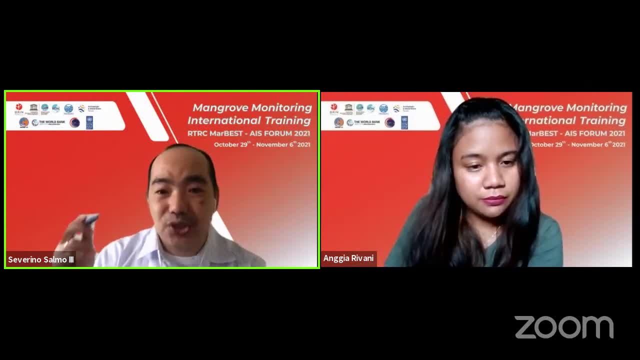 environment for them, Maybe because you have a source of fresh water Right. So when you plant mangroves in above intertidal area, that's very conducive for mangroves And of course you have to consider the species-specific growth requirement. 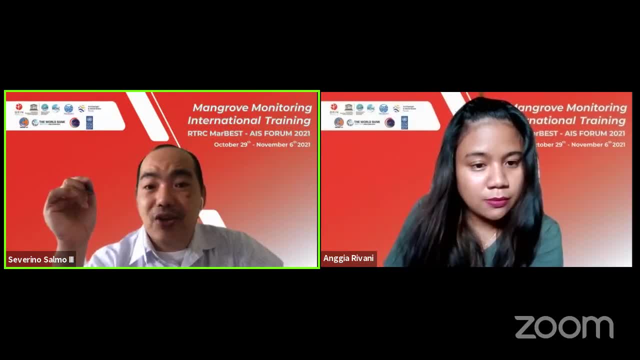 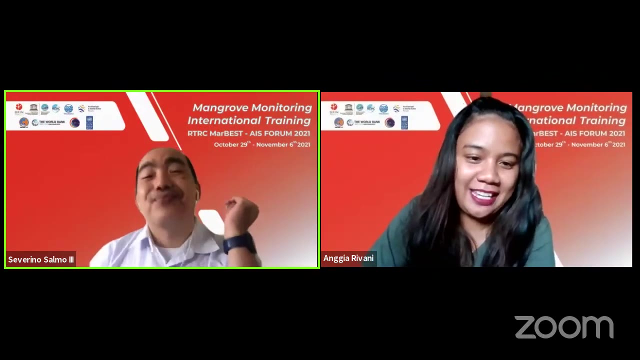 You know the species succession in mangroves. In the shoreline, you have Abyssinian sonoratia. at the back, At the landward area, you have the bruguera. Did I answer your question? Yes, Thank you for a complete answer. 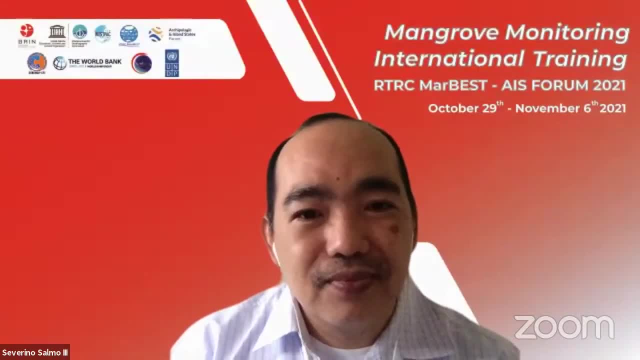 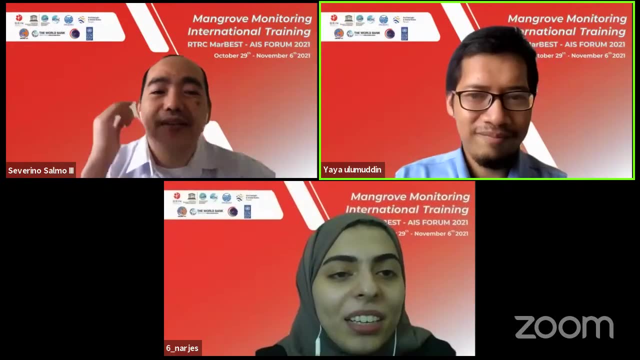 Thank you. Okay, All right, Thank you. Next question is from Nargis. please, Hello, Hi, Can you hear me? Yes, Yes, Yes, Hi, My name is Nargis. I'm an environmental scientist from the Supreme Council for Environment in Bahrain. 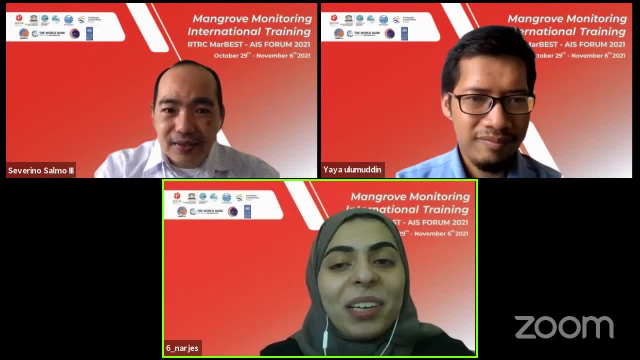 And first of all I just want to thank you, Dr Salma, for this amazing presentation. I learned a lot And it's got me thinking about a lot of things. now My question is also two parts, like Anjouya. 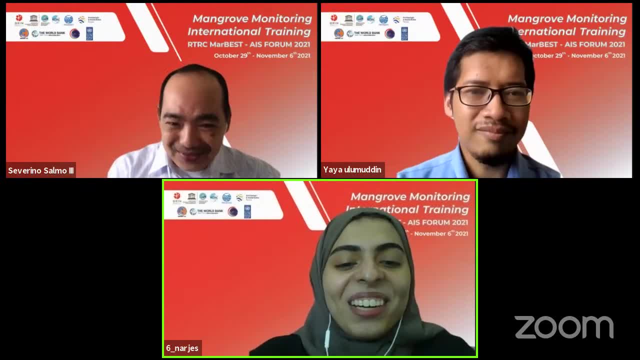 First of all, where I'm from, we only have two locations with naturally-appearing mangroves. The rest are where mangroves are found, And then we have two locations with naturally-appearing mangroves And then we have two locations with naturally-appearing mangroves. 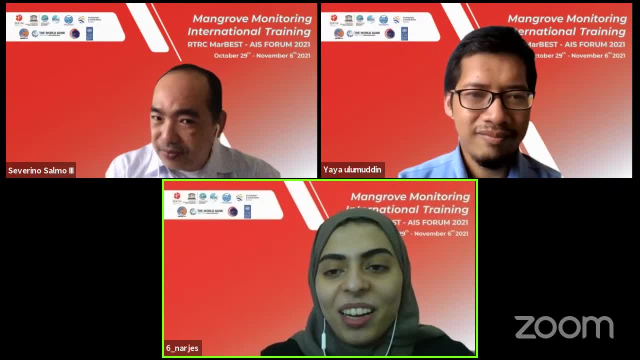 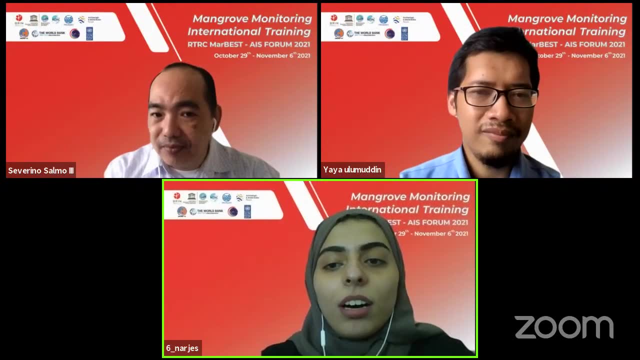 And then we have two locations with naturally-appearing mangroves. The rest were manually transplanted. So the new locations were manually transplanted. So the first part of the question: can we consider those places as part of the restoration? 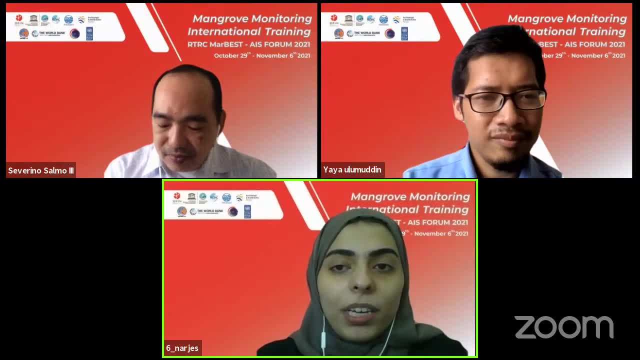 project. Yeah, Even though they weren't existing there before. Yes, Yes, Yes, Sorry, I forgot to mention: Even in the definition of restoration, we have to keep in mind that there is a part of the restoration project that's not yet been completed. And so there's a lot of things that we have to do before that, And I think that's a very important part of what you're talking about. But I think it's very important that we consider those parts as part of the restoration project. 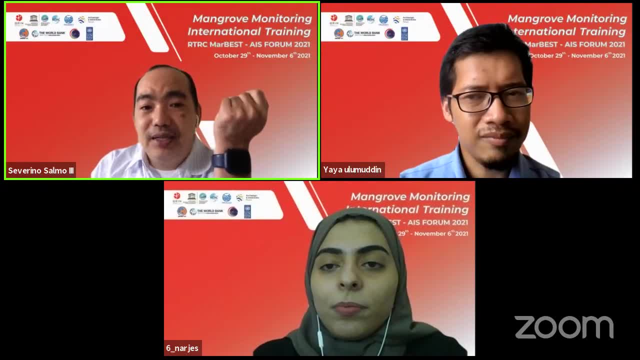 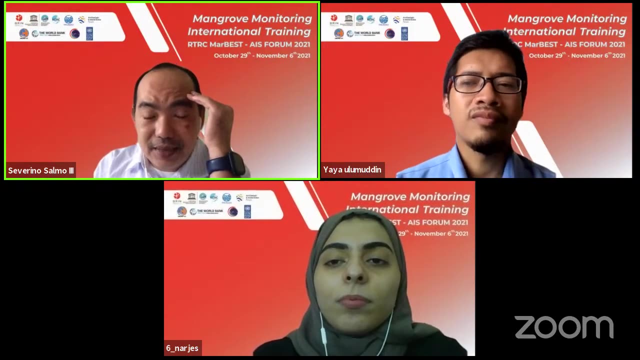 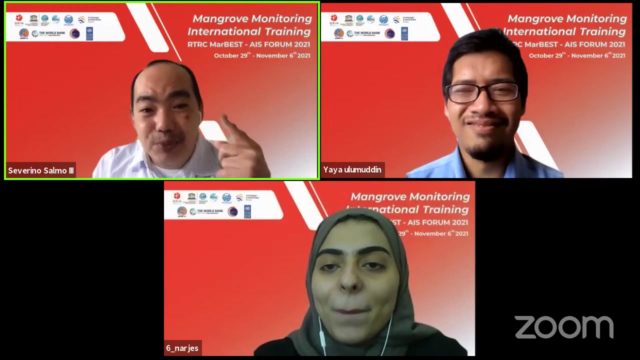 even though they weren't existing there before. Yes, Yes, Yes, sir, society for ecological restoration. they have a qualifier like full recovery versus partial recovery, and it will depend on your, your ecosystem attributes that you want to assess. but yes, well, i would say you're lucky in a way. how come? because you all, you said you only have two. 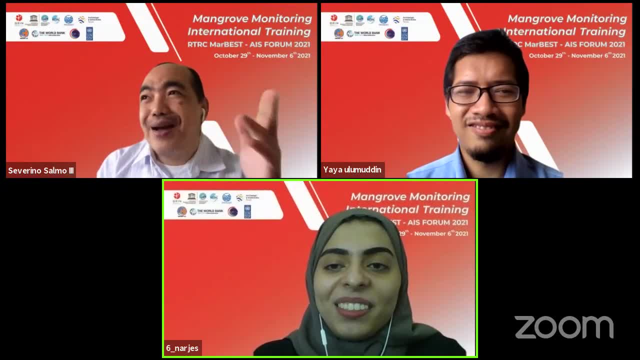 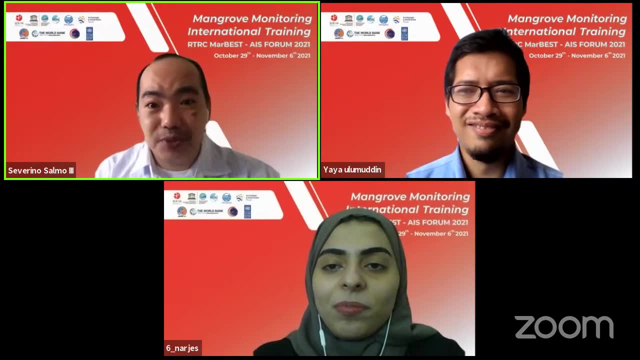 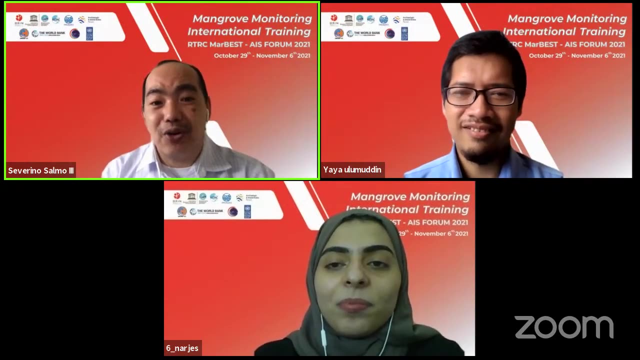 natural systems naturally occurring. yeah, so, so sorry. um, when i say lucky because you have, you have two sites. if you go to indonesia, how many natural mangroves you have? if you go to the philippines, how many natural mangroves do we have and how many mangrove ecologies do we have in the 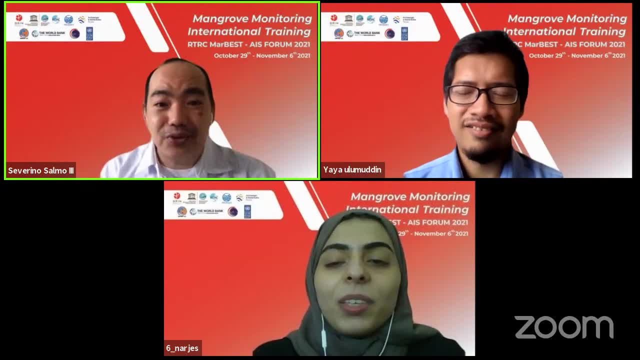 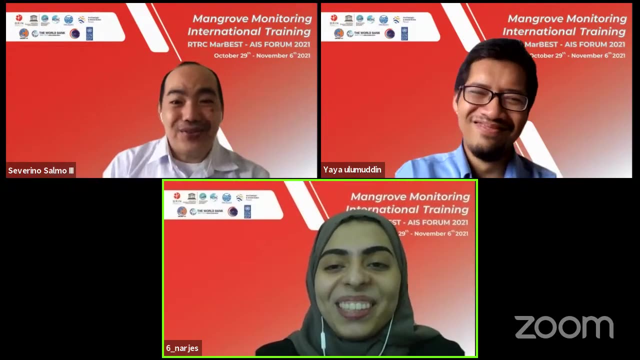 countries, i think my count is less than 20. i, i don't know in indonesia. so if you only have two months, two natural mangroves, then i could say you can easily, well, relatively, you can relatively assess it. maybe you can. you can start tomorrow and definitely right. 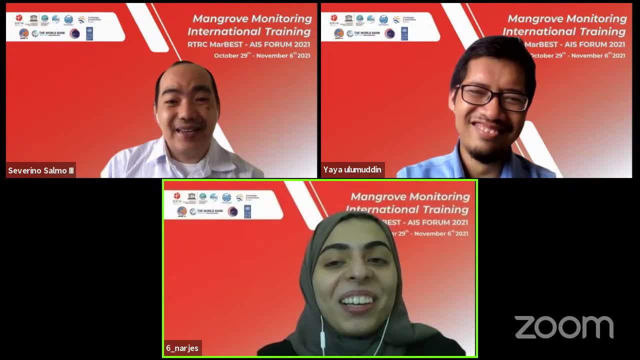 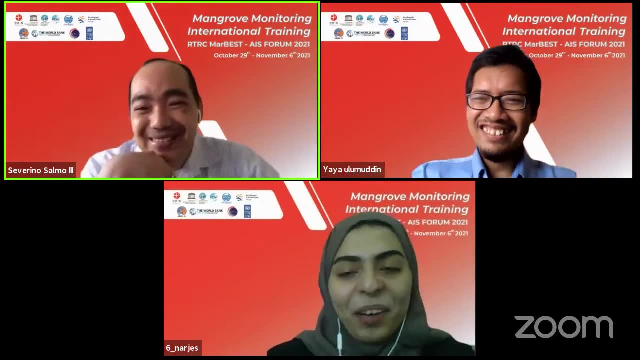 that's what i mean. that's what i meant. your presentation got me thinking: okay, there's a lot before you make a new airport. definitely, yeah, so i mean that's. the second question is connected to what you just said. so with the manually transplanted mangroves, would the new research? 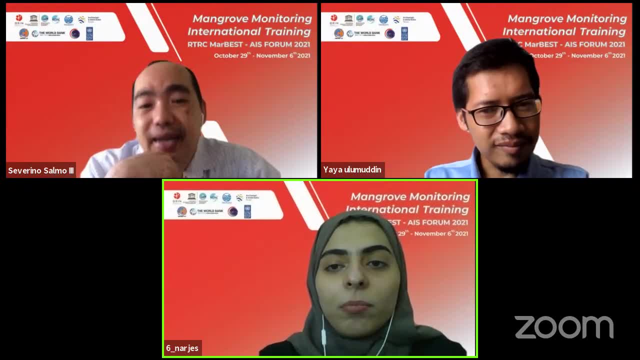 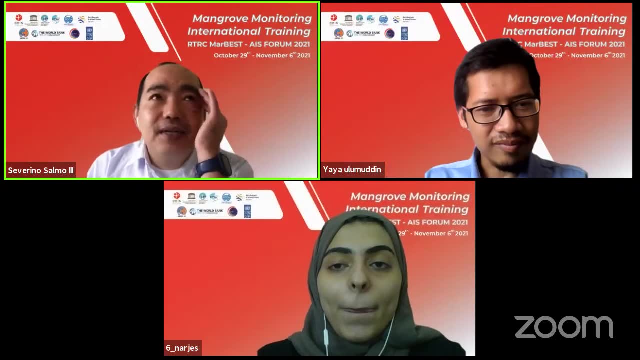 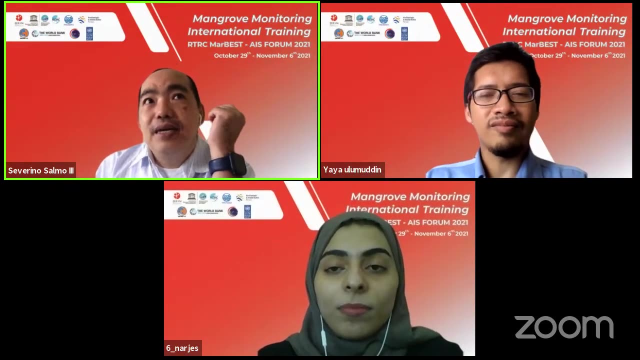 approach be the same. so, establishing a reference? uh, yeah, yeah, maybe looking at indicator species? yes, so we'd apply the exact same approach, right? yes, yes, yes, uh, the the sir is very the society for a logical restoration is very strict with the, with the terminologies, and there will always be an. 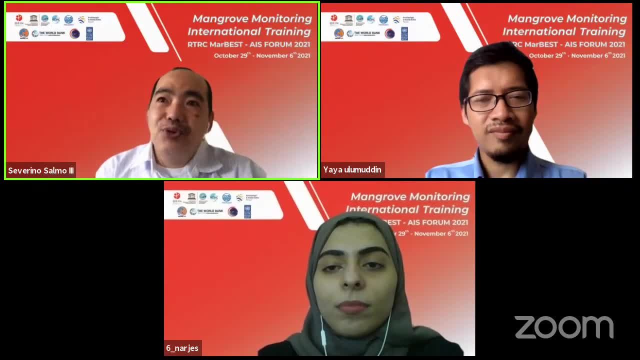 issue with causality in statistics. how sure are you that your outcome is dependent on your restoration program? that will always be a question, but remember, sir, has always this notion that you have to find the best available reference, and i think that would answer your, your, your question. 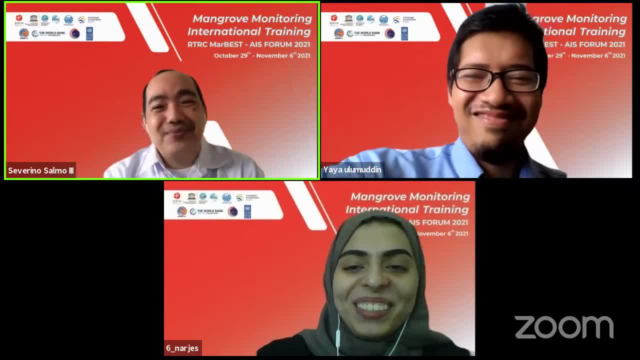 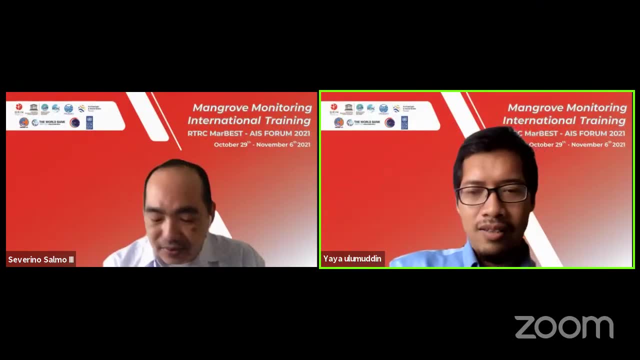 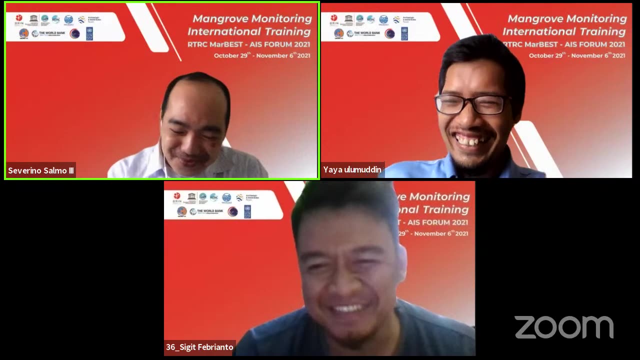 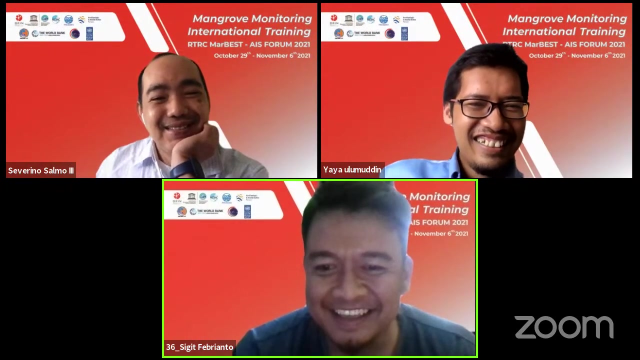 yeah, it did. yeah, yeah, thank you, that was very helpful. thank you welcome. thank you. so next question: uh, maybe from sigit, please sigit, sigit sasmita, that's not different. i'm, i'm i'm kidding like name. okay, thank you, dr sofrino, my name is ikit, i'm from university. i have a question: what is the effect of molusca abundant between restore mangrove with one species like chrysopora and natural mangrove? what caused the difference in mangrove growth in its location and another location? example: uh mangrove in sumatra and java, or? 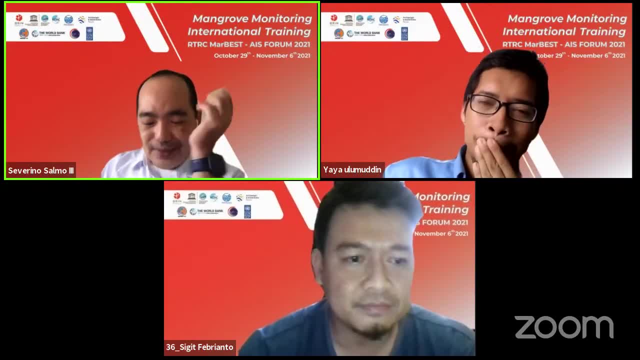 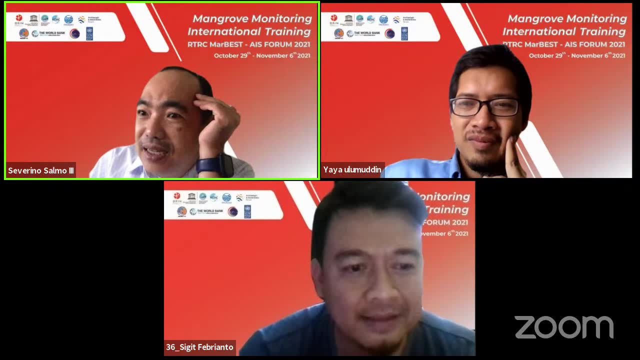 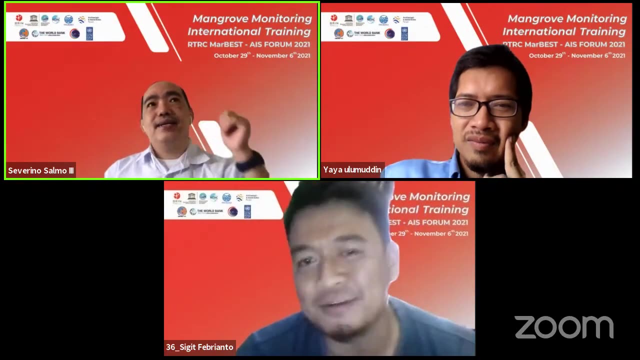 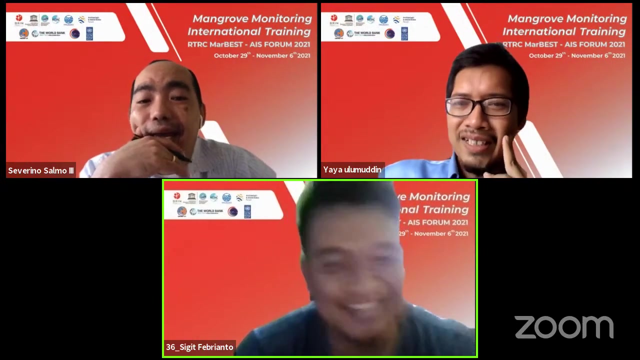 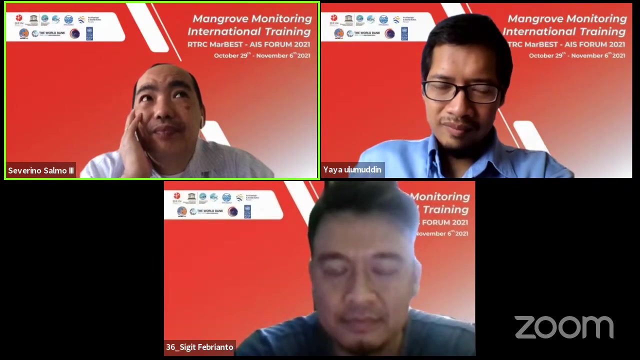 papua. thank you, uh, your first question. i, i didn't get that sorry. molus in molus, uh, molus abundant in mangrove restoration, yes, yes, yes, yes, yes, because uh, restoration one species, yeah, yeah, yeah, yeah, yeah, yeah, i know, uh, again, i in encircling, so i'm given another two more interesting. um, we have two more very valuable. 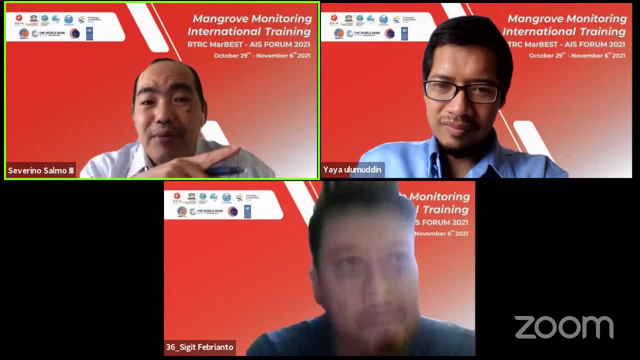 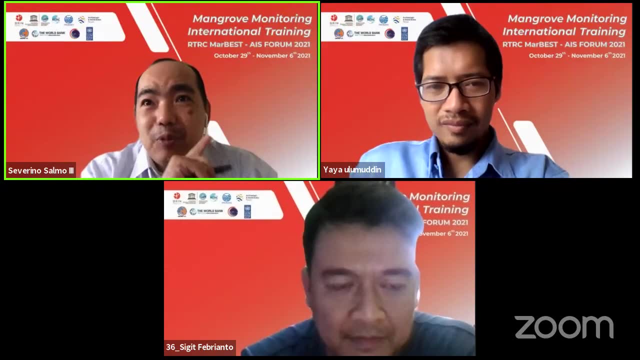 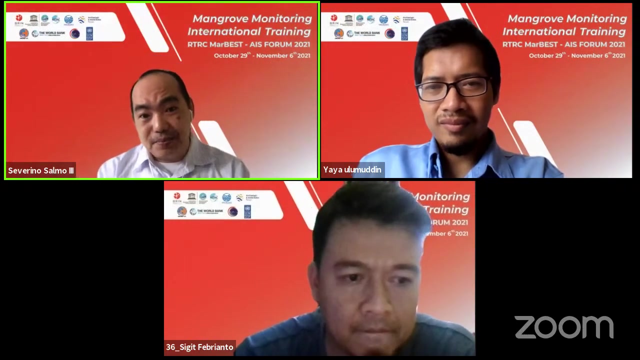 questions which are, as i indicated in chapter two, about the, about the operation of Mangroves. what type of molus are we seeing? if you see, if you planted resopura, then obviously the answer is that molus that will be attracted to resopura are those models that are attracted to reservoir. as simple as that. but if you plant mangroves that are diverse, for example, if you dig a mangrove, that will be attracted to reservoir. as simple as that. but if you plant mangrove that are diverse, for example, if you dig a mangrove, if you dig, so what kind of mangroves, like r Centers, will be Pikani mollus. they will always, will always be sabe l controversy. but there will also be dead mangroves and in one singleと思, lunges of corn will improve their rooms. life. life is never occurd. the dirt of the divide is always. Lorca, you want much, but owner chimera none has something. 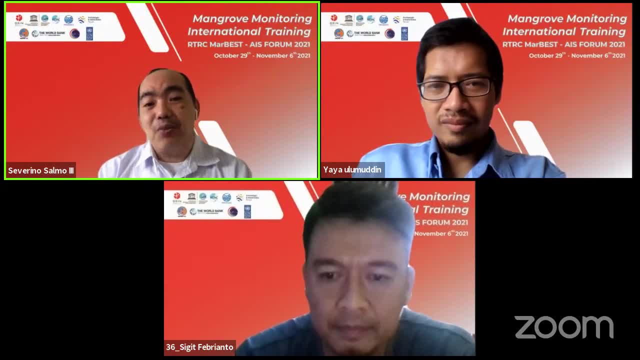 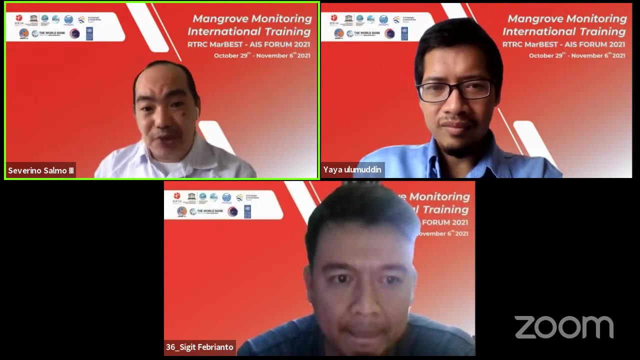 example, abyssinia sonaracha, then you will attract more species. that's the reason why i don't really suggest molus abundance and molus biomass as indicator of restoration. i wanted to capture the ship, the change in species composition and yes, we have similar case. and if you plant resopora, 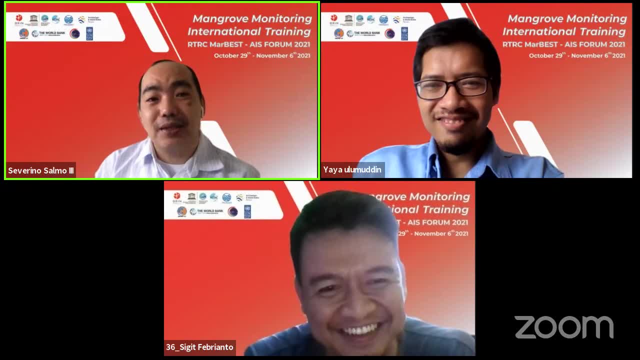 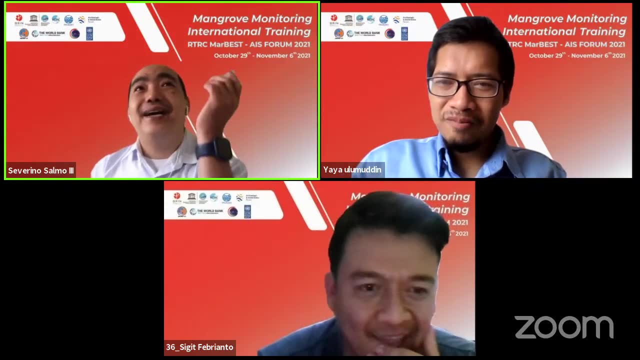 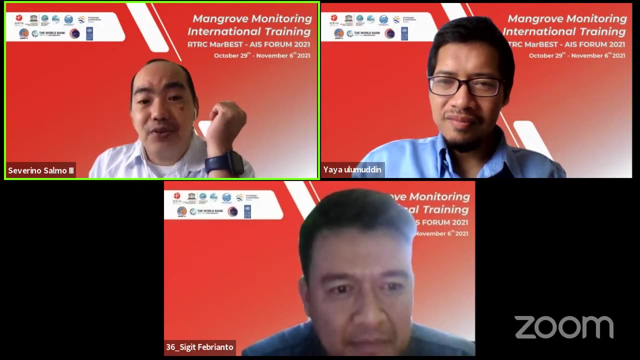 what would you expect? you will get molus that are attracted right now. for the next question, the difference in mangrove growth: yeah, uh, again, there will be a localized growth differences. that is expected because you have different condition and the growth of the mangroves affected by. salinity negatively affected by salinity. if you have fresh water systems, then obviously mangroves will grow more, will grow best with the, with the fresh water environment, because that will neutralize salinity. um, that's the reason why. yeah, that's the reason why i. 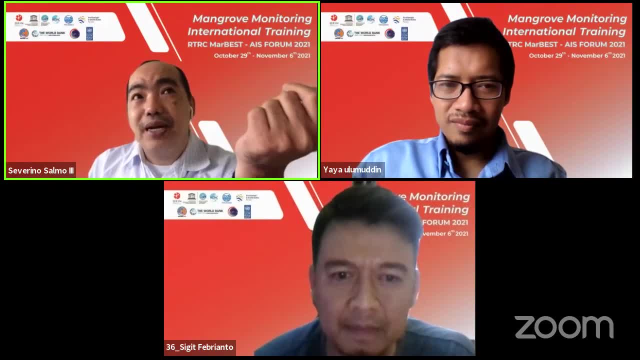 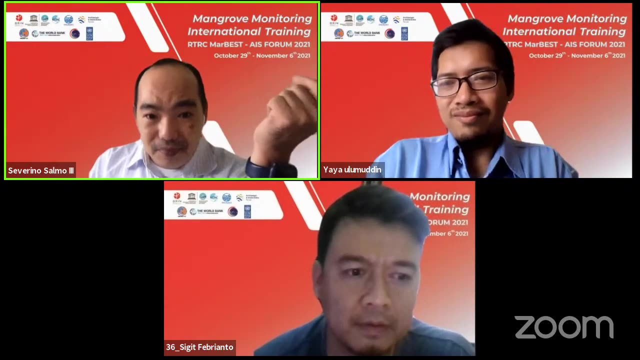 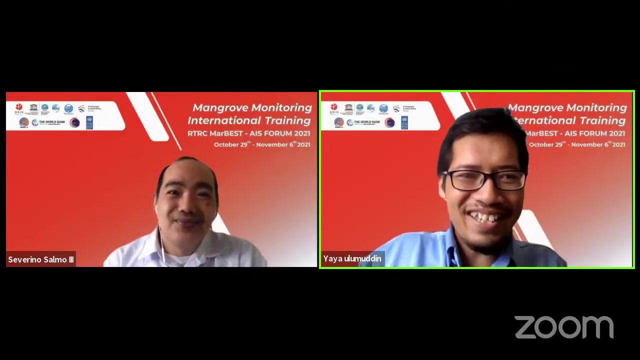 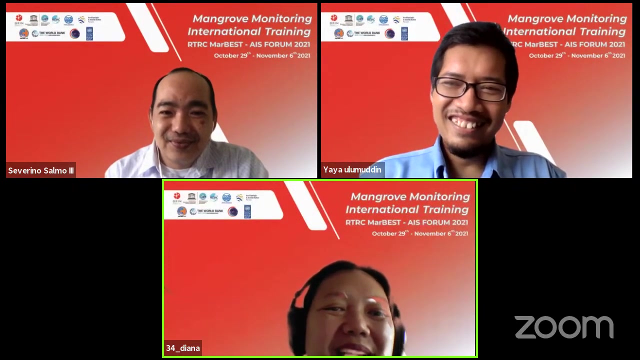 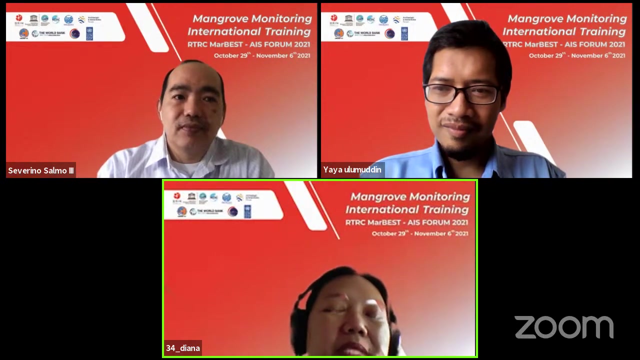 suggested that it will be good if the restoration ecology studies will be conducted in one site wherein you have your chrono sequence. otherwise you cannot compare site one versus site two versus site three, because the conditions are totally different. okay, thank you. welcome, it's um. hopefully it's for that, the things that kathy and i talked before, and that these for example, uh, including the indonesian mangrove. i mean in particular for indonesian mangrove. what factors that cause indonesian mangrove need a longer time to recover compared to some other countries that you mentioned? like some other, 10 years, but for indonesia, like 15, 20, even 25 years. 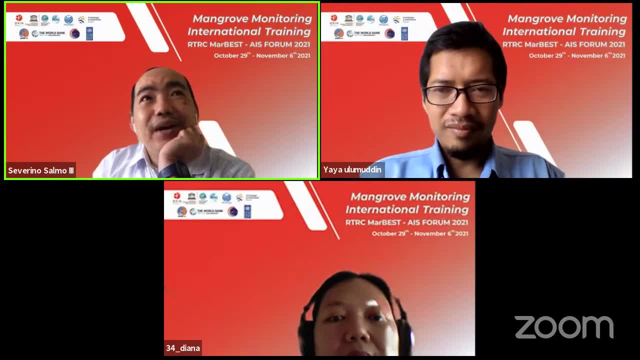 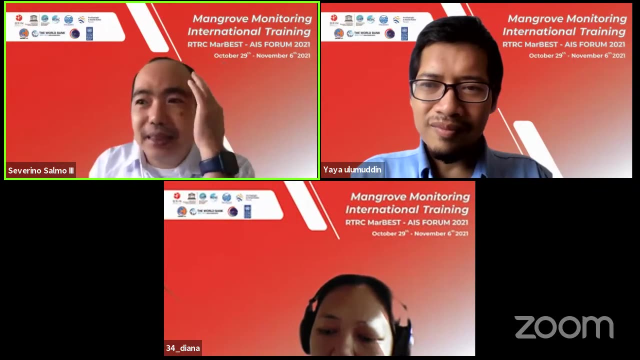 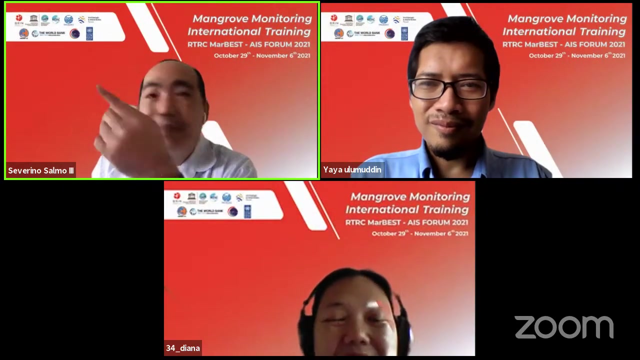 yeah, yeah, what factors fit in that? uh, i i believe it's. it's caused by uh site differences, and i i only read uh dr p does work, wherein he and she studied the tambak in bali. okay, right, so i'm from bali, yes, yes, the other one is in malaysia. i think it's 15 years old, but it's a totally different. 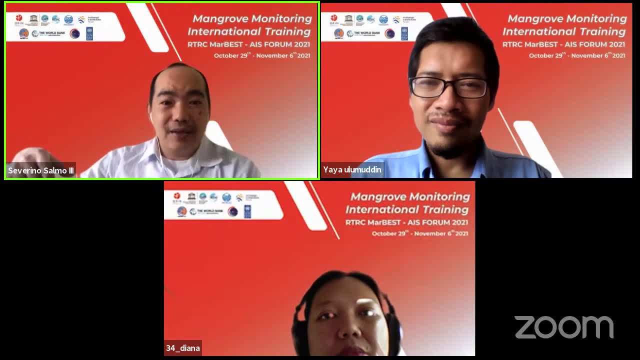 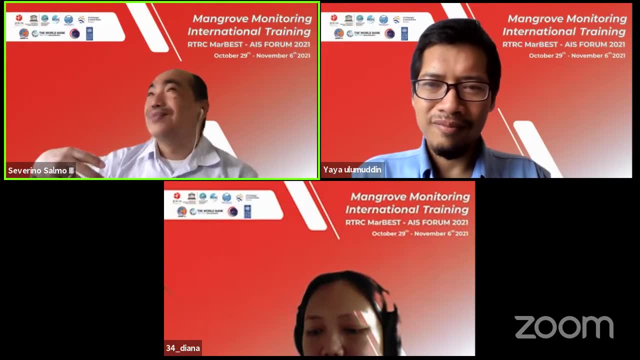 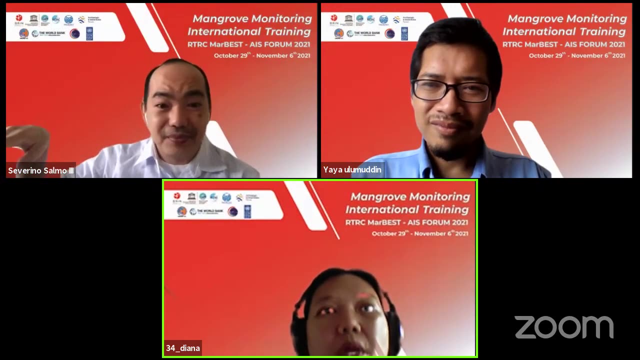 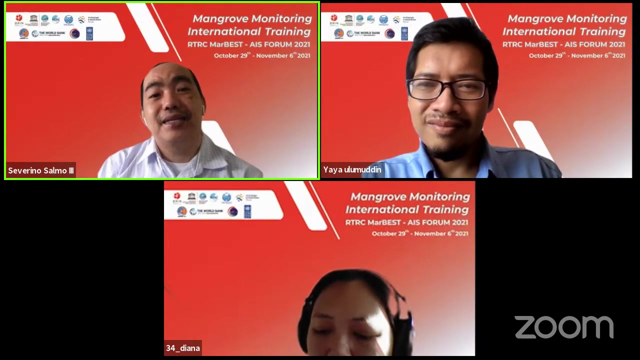 case, you know, um, malaysia is peninsula, okay, philippines and indonesia are our archipelago. so you, you have- well, you don't have typos, but you have, uh, the red plot is quite extensive, okay, and obviously i i will not be surprised if there could be other studies in indonesia that will say, maybe growth is uh. 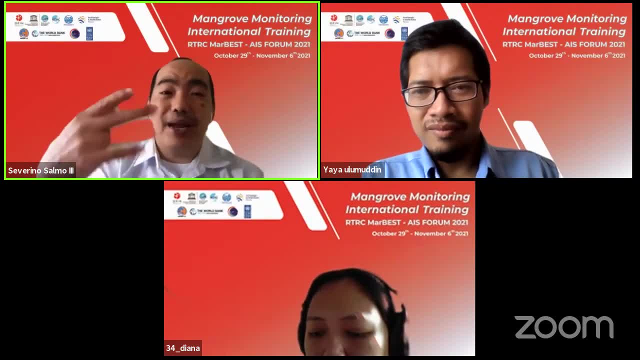 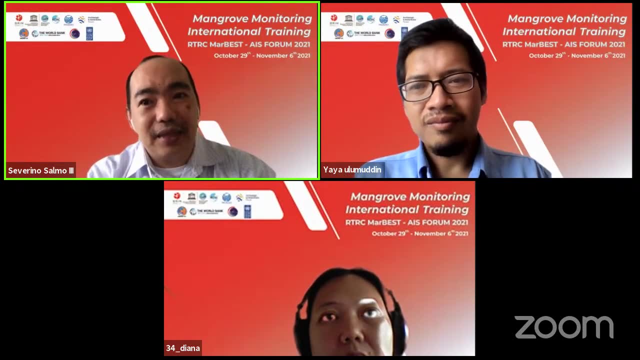 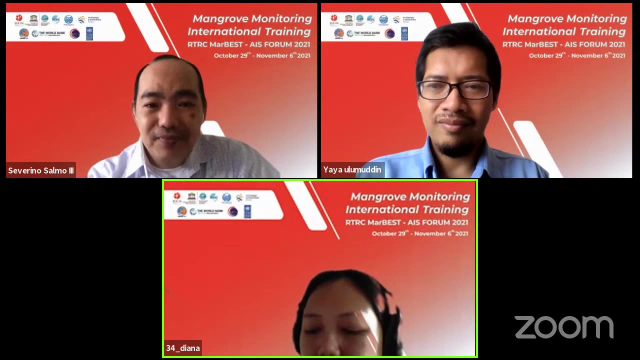 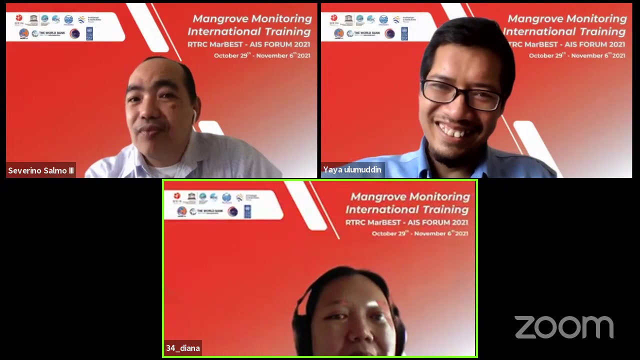 is possible in 10 years time. you do have a lot of rainforest and i think if, if you have mangroves that are closer in forest, i think you will have faster recovery. not not 15, not 25 years. okay, okay, okay, thank you. yeah, can i have one more question? yes, given our limited resource for the mangrove monitoring, how? 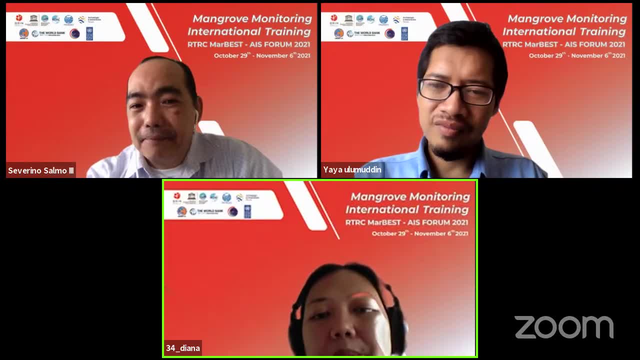 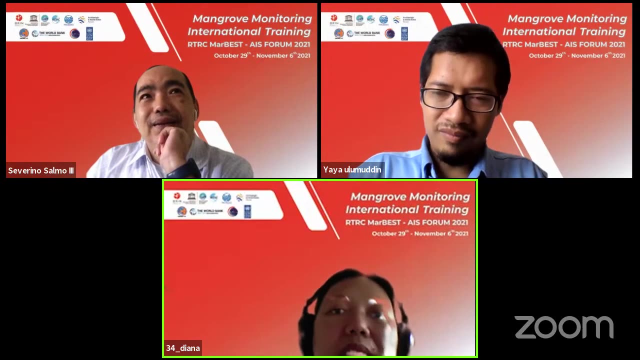 how often, or what is the minimum period that we should resurface our plots to see any changes from the mangrove ecosystem development, Also, given that the UN declaration on mangrove restoration agenda is between 21 to 30. So what is the minimum? 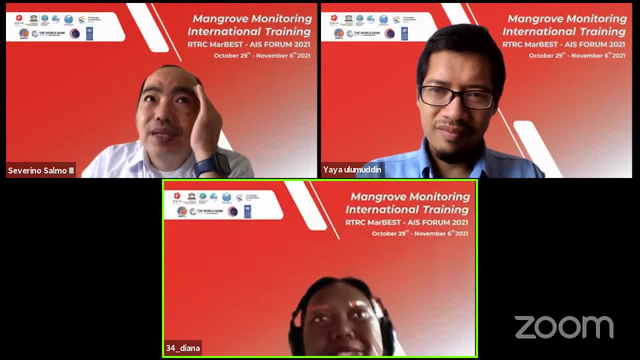 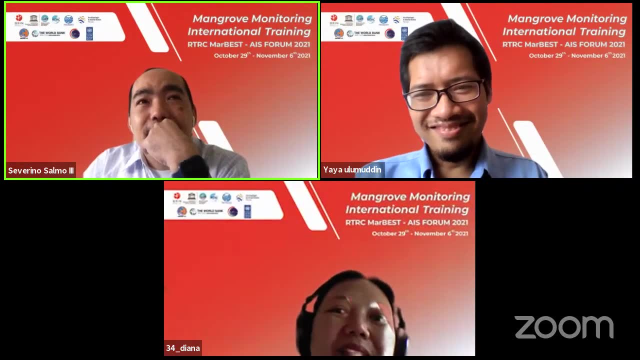 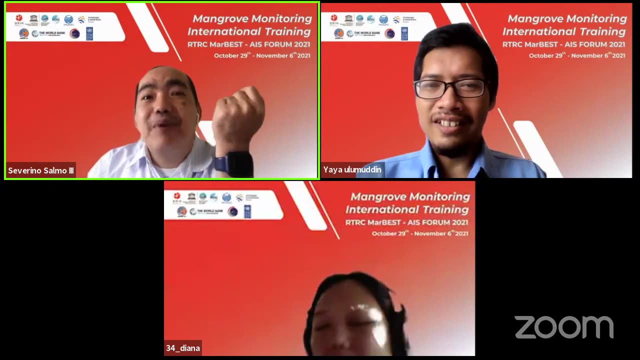 Yes, how often to see the changes? You have a very difficult question. In the Philippines, my basis for saying two assessment per year is simply because we have two seasons: the rainy season and the dry season. right, If I can, if I have resources. 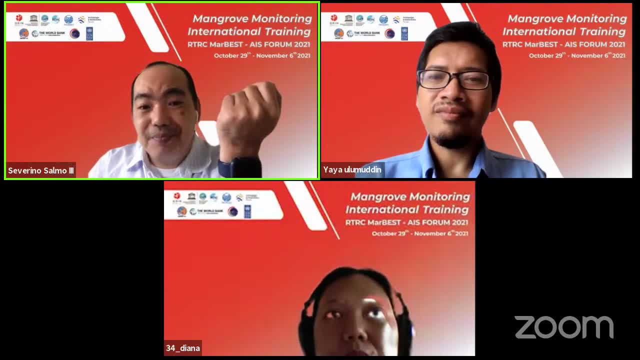 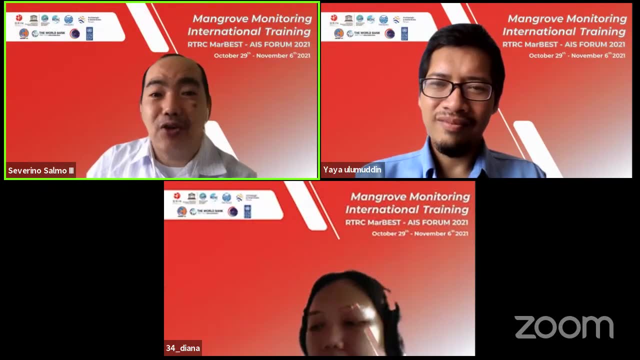 if I have the time and the personnel, I will do it more often because we want to capture the ship. Unfortunately, there are less than 20 mangrove ecologists in the Philippines. I don't know how many mangrove ecologists you have in Indonesia. 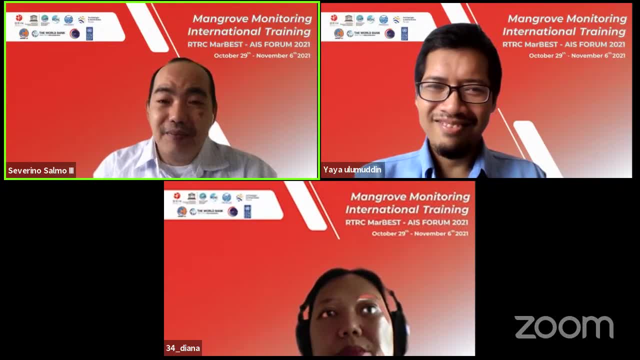 If you have more, maybe you can do more sampling, but obviously it's not the case And resources is a problem. I think once a year will be good enough. There's no question that if you have the means, you can do more. 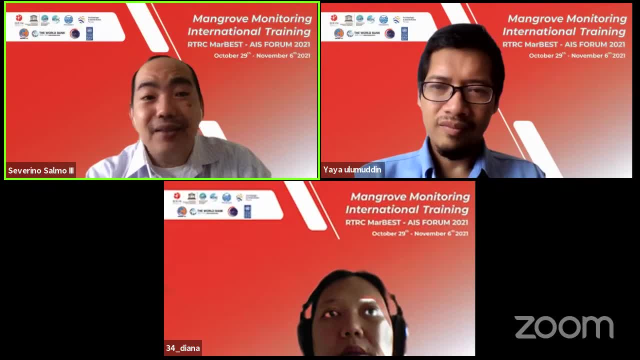 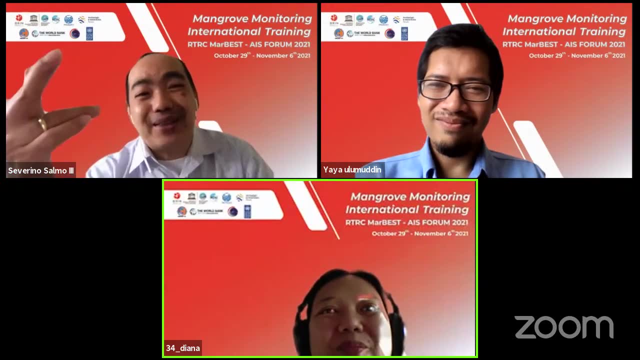 but once a year at least is already good enough, And you will learn something from DE anyway right This morning, So you can compliment your monitoring skills with yours. You cannot go to mangrove. you cannot go to mangroves every day. 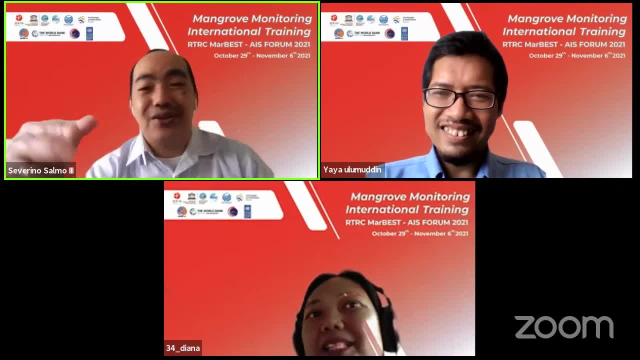 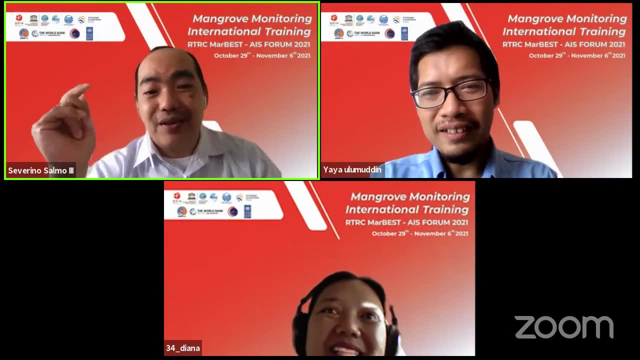 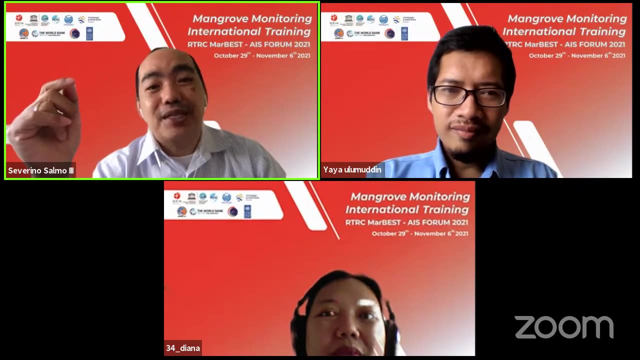 but because of the GEE and remote sensing, I don't know. It's here maybe. Yeah, but there's still no substitute with the actual field sampling. You can compliment both approaches And therefore you cannot do it. There's no need for you to do more frequent sampling. 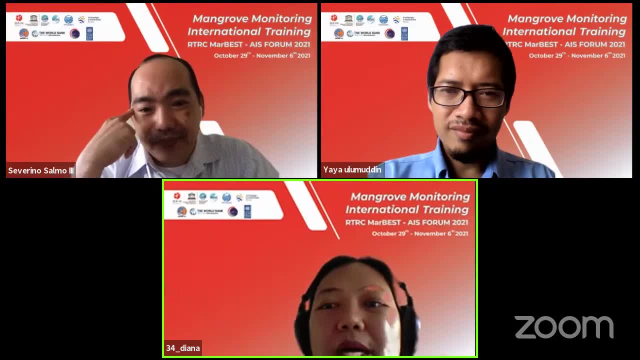 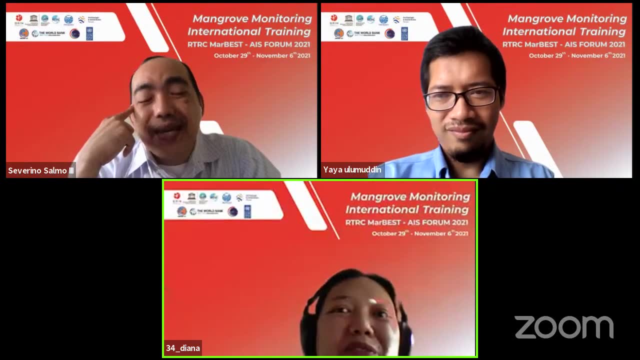 unless you have the resources. So I like to confirm: So it's once. a year is already good. If it's more than that, given our funding, for example, two years once in two years or three years, No, no, no. I think once a year would be a minimum. Yeah, because- imagine this: you plant mangroves now. There's no reason for you to monitor growth tomorrow because there will be no changes, right? Maybe it will grow in three, six months time. 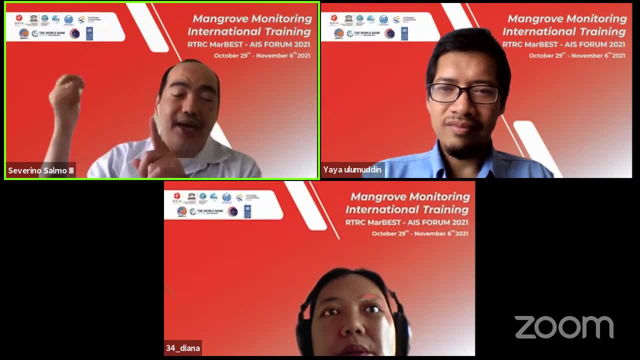 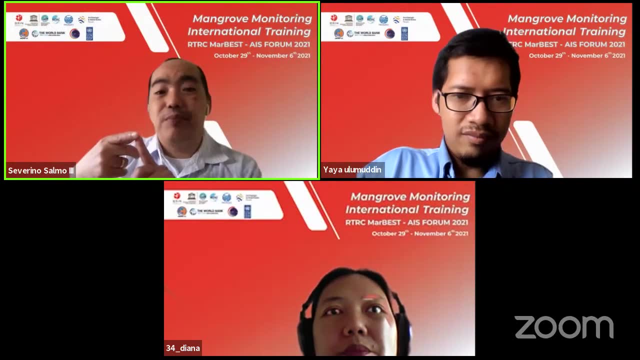 but then it might be good to capture that, because you want to show the, you want to capture self-teening. But in the absence of resources, then one year post-planting would be good enough because, who knows, You can see the progression in the growth of the mangroves. 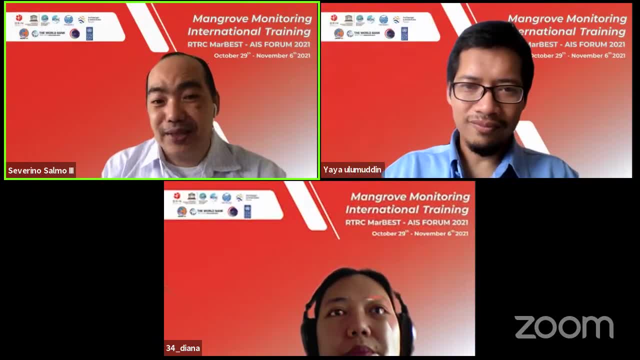 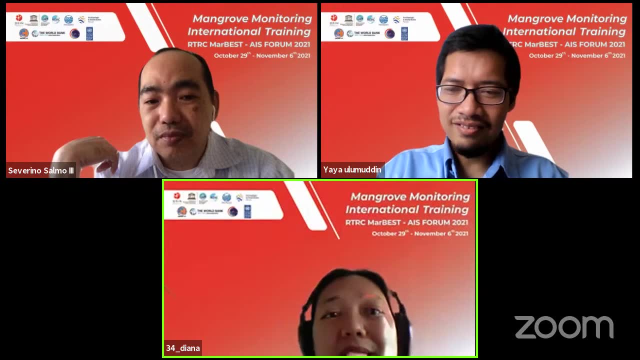 But again, if you have the resources, do it as often as you want. Okay once again. So if like two once in two or three years will be two less, then Yeah, two that's too few, Who knows? Thank you, 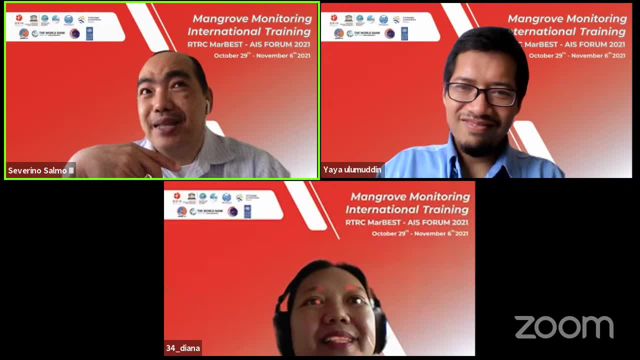 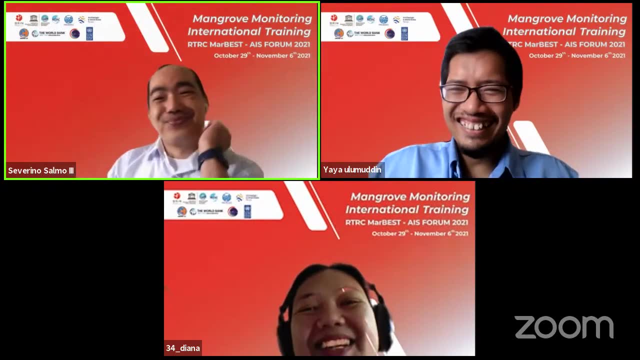 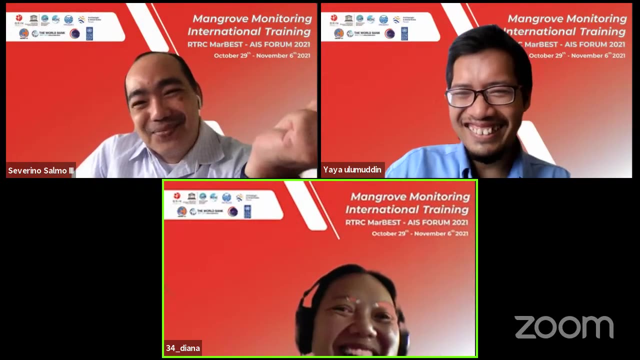 So when you measure after three years, the planted seedlings will not be there anymore. It was eaten by a goat or by a cattle, Thank you. Thank you, Sorry, I'm very funny, It's fine. Okay, next, Sumiran, please. 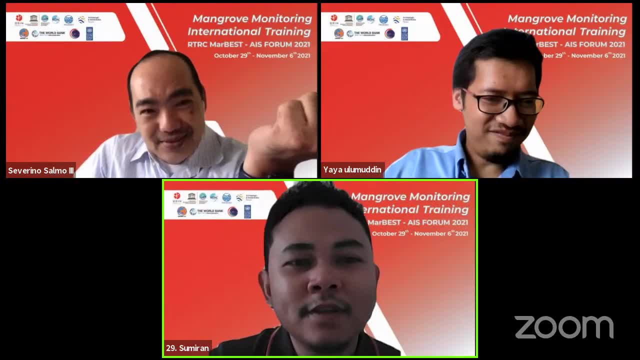 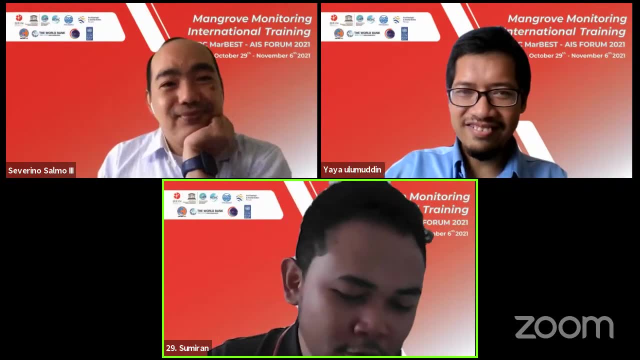 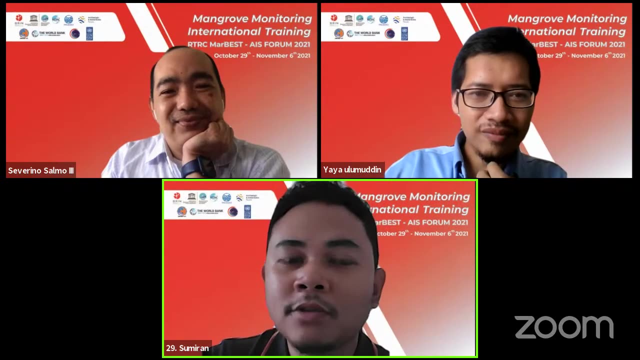 Ask your questions. Thank you, Pak Yaya. My name is Umir, I'm from Mula Warman University And thank you, Dr Seth, for your kind sharing your experience And I would like to ask you about in your experience. 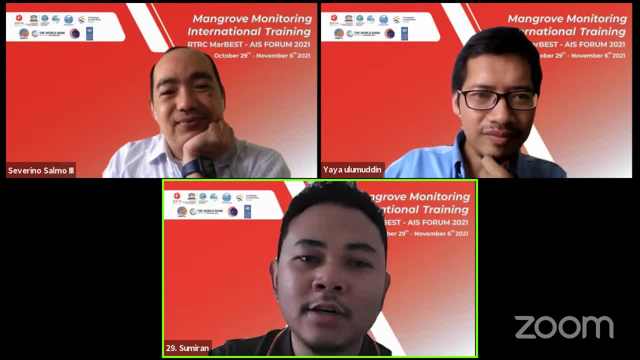 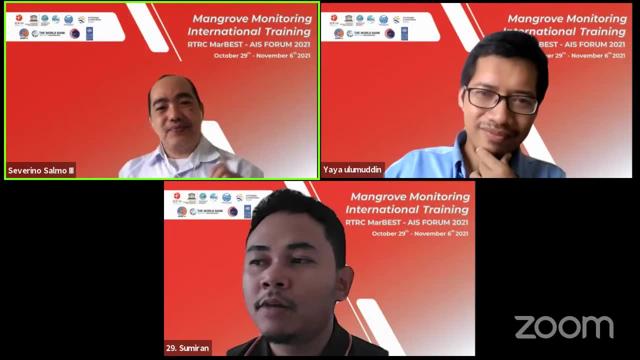 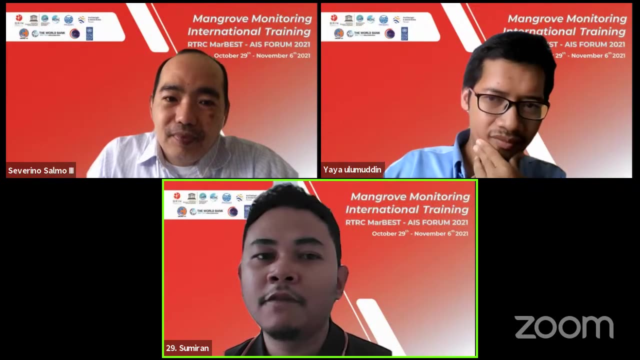 in your research experience, how did you categorize the mangrove restoration area into young mangrove, intermediate mangrove and mature mangrove? Yeah, yeah. Is it based on the age of the mangrove plantation plantation? if yes, how we can get the information? 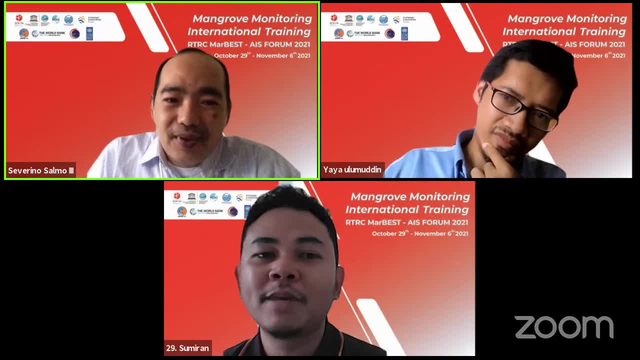 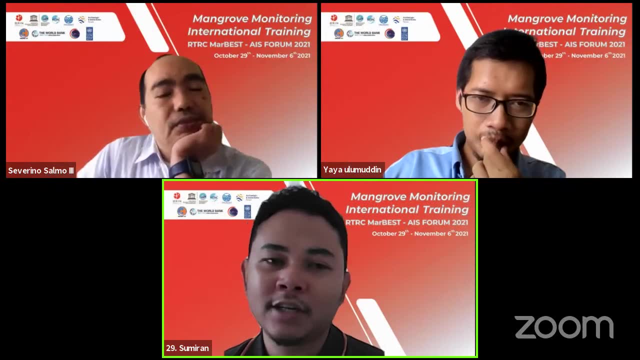 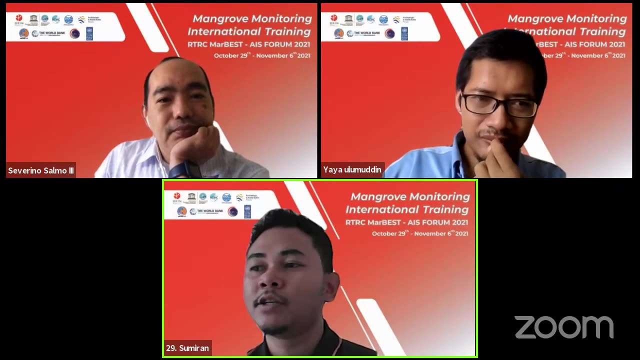 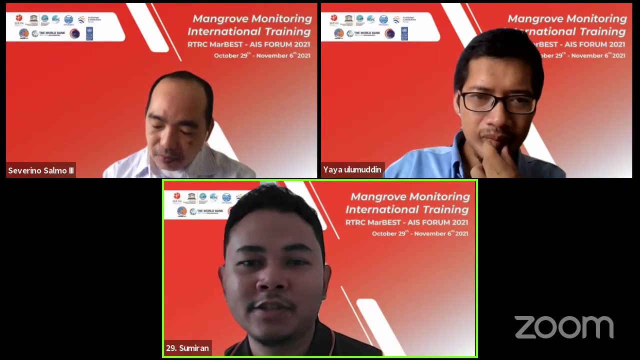 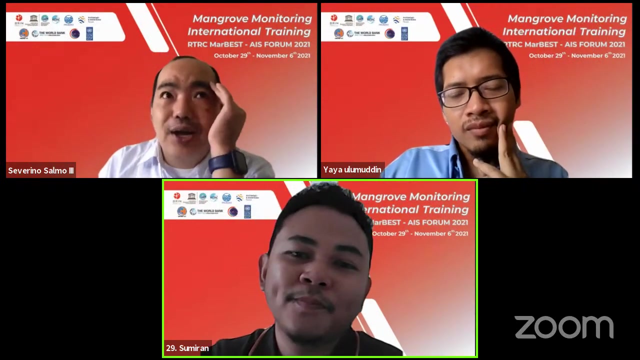 Because sometimes this information is not ready in the local people that are conducting plantation. Sometimes the local people that are conducting the mangrove plantation usually only provide information related to the estimated part of the age, not the fixed age. Yeah, to answer your question first is: 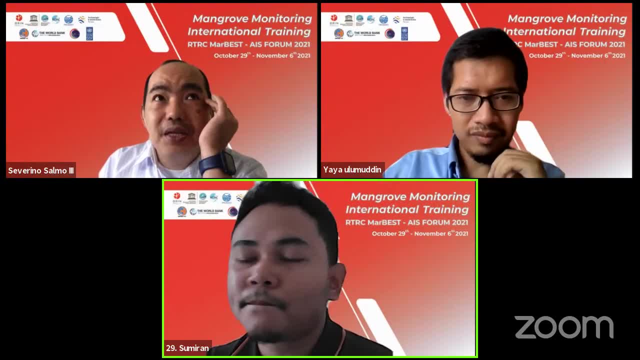 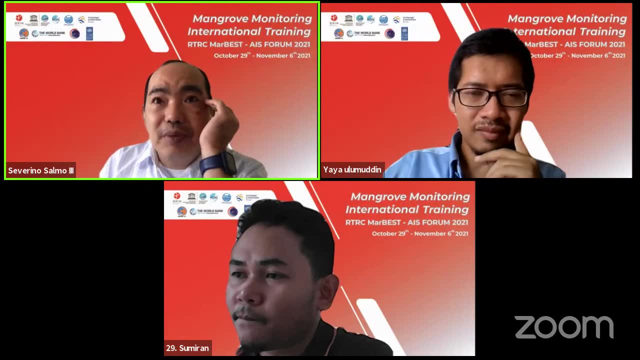 how would I know if it's a young, intermediate or mature? Luckily for me, I know the age of the mangroves And I followed the. I measured the vegetation and the sediment and the fauna And I followed that for three to five years. 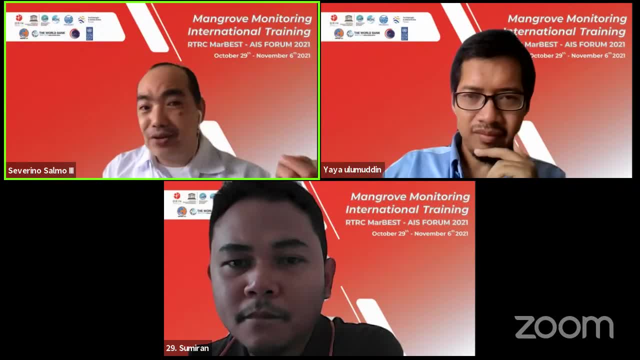 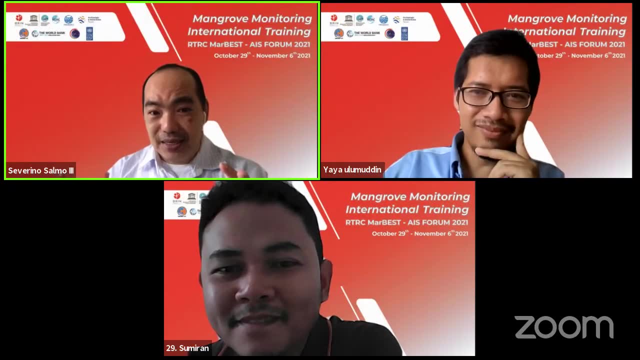 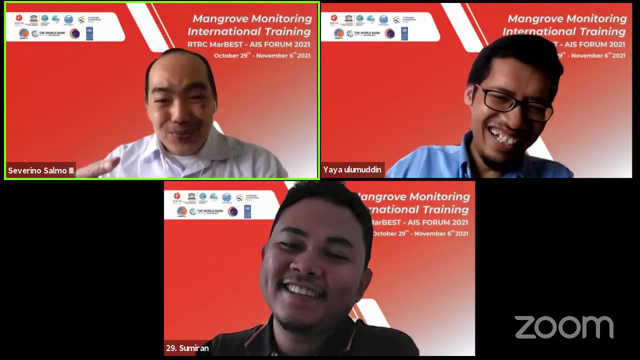 I told you, when I'm doing my PhD, I'm not attending conferences, I'm not attending meetings. It's the only thing that I'm doing, So I'm very focused. Can you imagine yourself measuring 10,000 models: Length, weight, how much time. 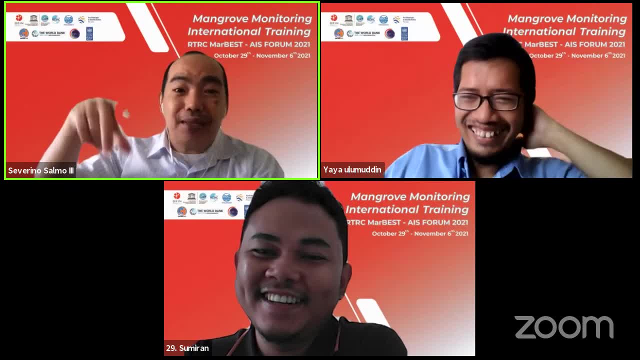 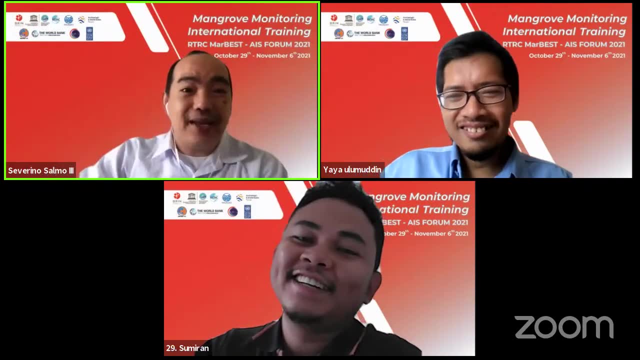 And the sediments, the sediments when you analyze organic matter. Yeah, Yeah, Yeah, Yeah. That's a lot You need to wait for. you have to oven dry it. That's 24 hours already per sample. 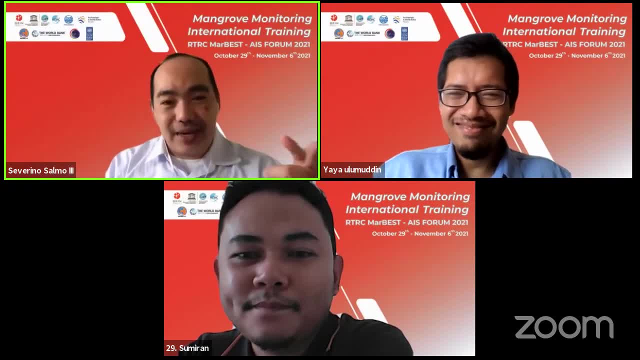 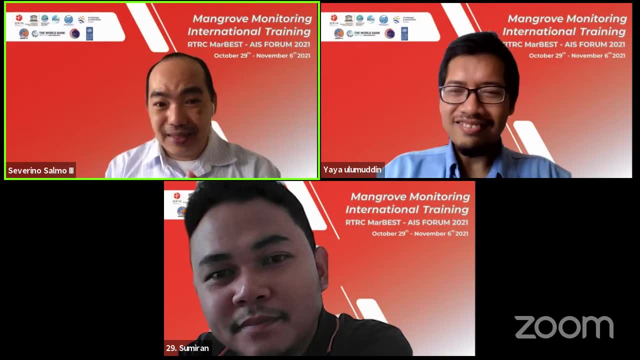 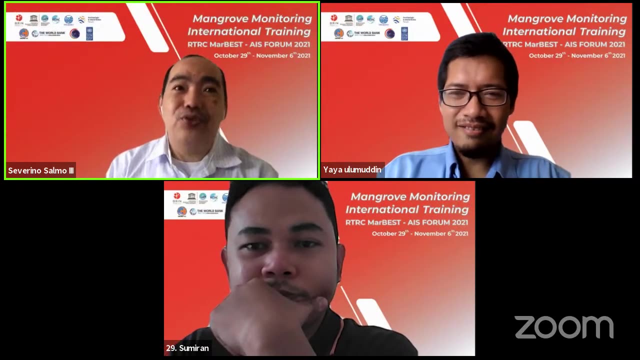 And how many samples do I have? right, That's a lot, Anyway. so I spent three to five years doing only those things. right Now your question: how would you know the age? Luckily for me, those sites are the same sites. 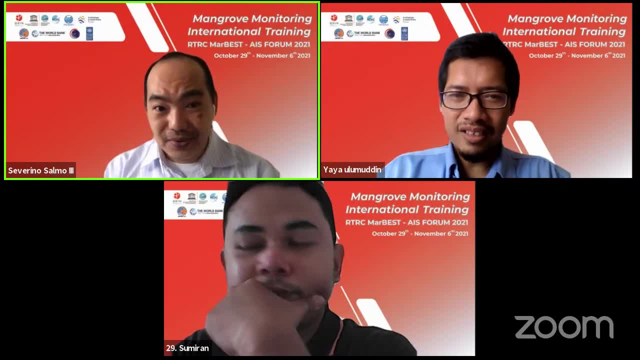 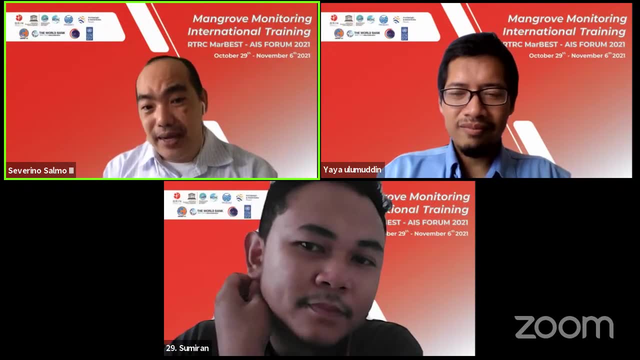 that I studied when I'm doing my master's. OK, Right So, but you're correct, in a way, that most mangroves you don't know the age. But you're lucky, you're very lucky, this morning You have ghee. 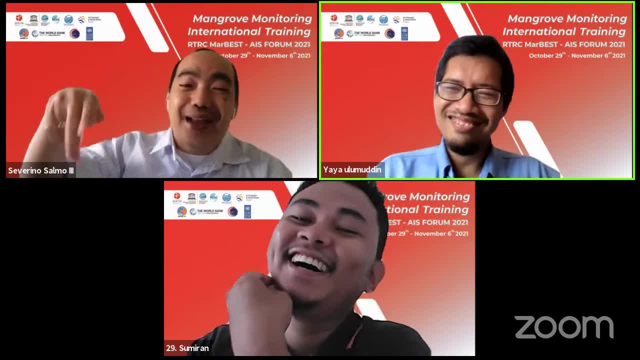 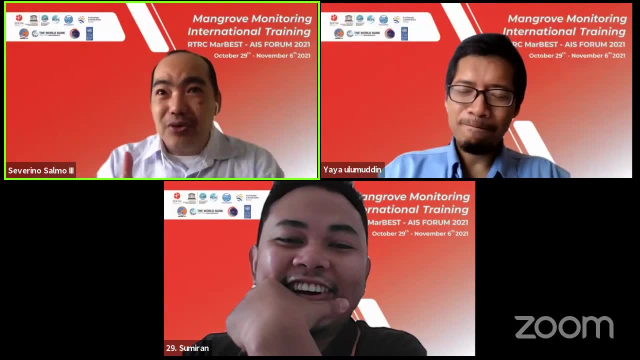 You will be able to track the. you know it's not perfect, But at least you know. if you say that time now there was a mangrove, but years ago there was no mangrove, then I will be able to estimate the age of the mangrove. 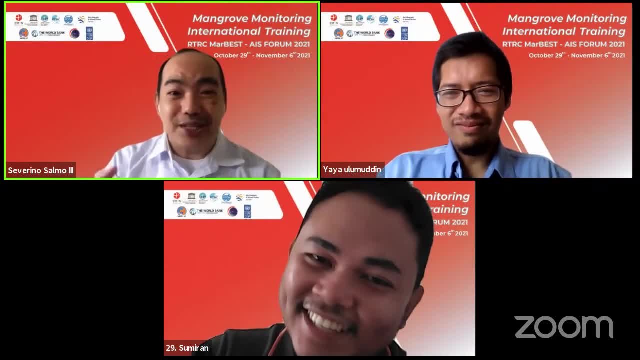 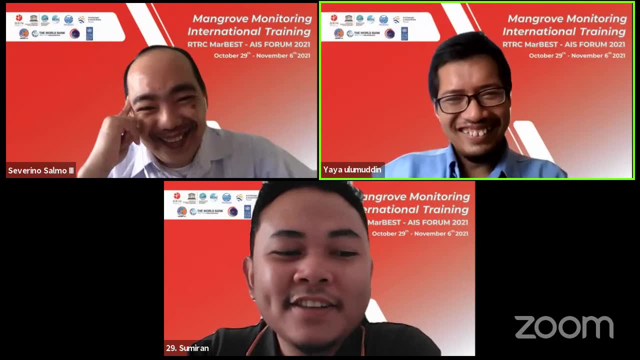 Mm-hmm, Mm-hmm, Mm-hmm. You must be very good in GEE and you had to teach me how to do it. OK, Yeah, That's right, I think. is there any kind of laboratory activity? 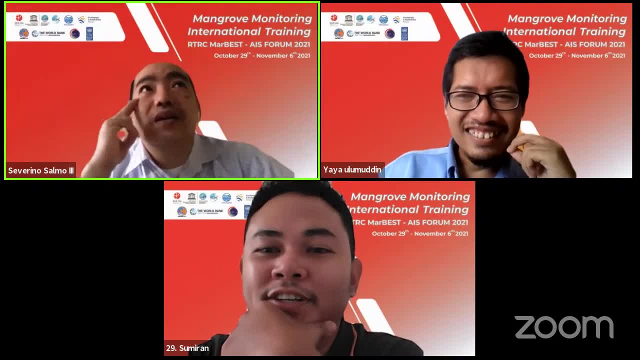 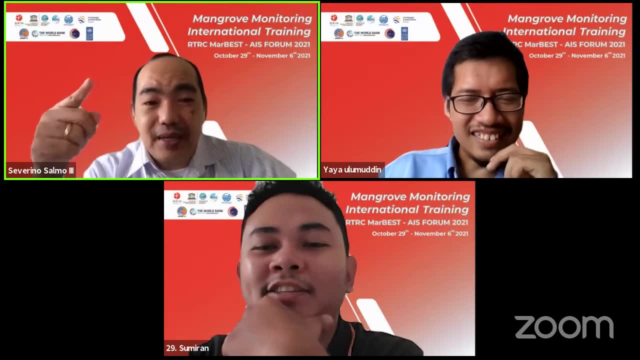 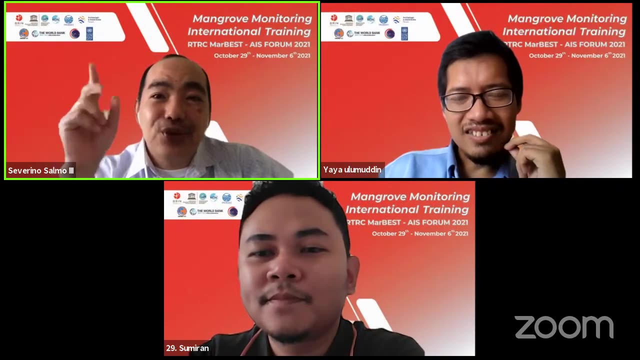 to determine the age of the mangrove. In the past they tried to do the isotope analysis to estimate the. it's a proxy indicator But I think it's not conclusive. Oh, When you go to the mangrove you're. 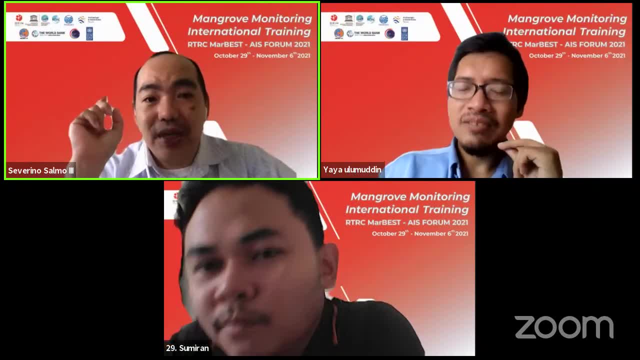 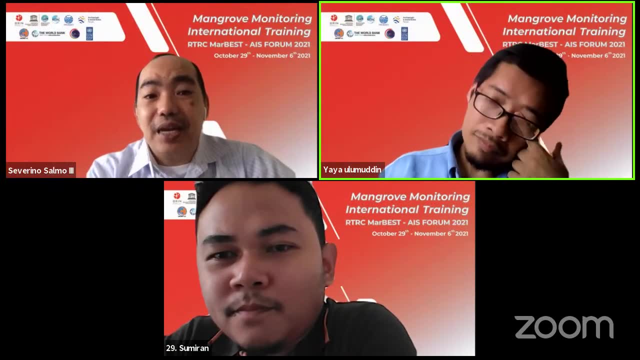 expecting that the isotope signature is only from the mangroves right. That's not the case. If you're in a coastal mangroves, the inputs are coming from the coastal area, And if you are at the back of the mangroves, 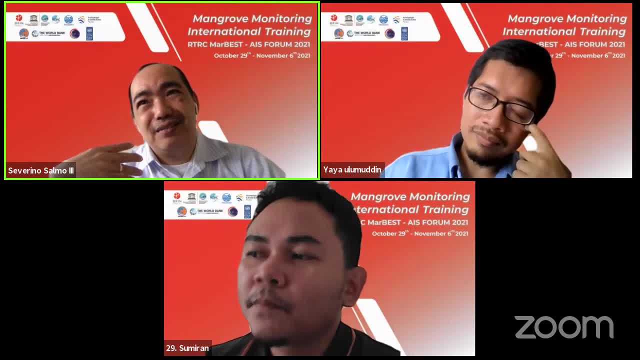 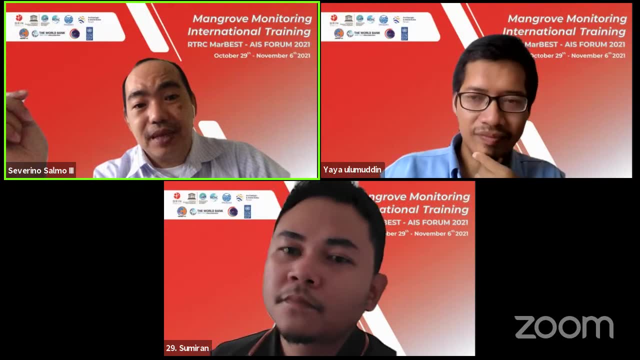 the inputs are coming from the rivers, et cetera. It's very difficult for you to say that the isotopes are mainly coming from the mangrove signature. Yeah, Yeah, Yeah, Yeah, I don't know. For me it will still be a combination of methodology. 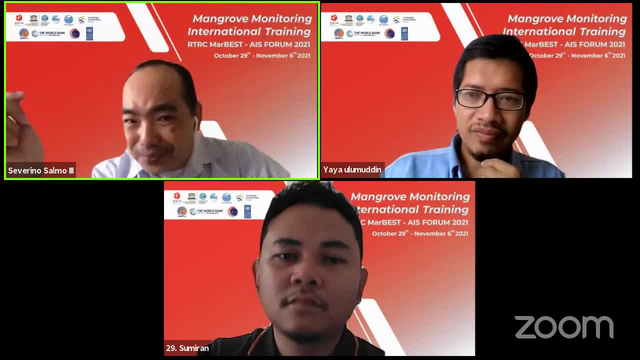 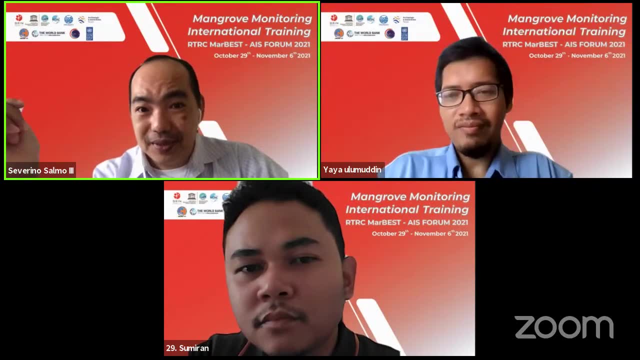 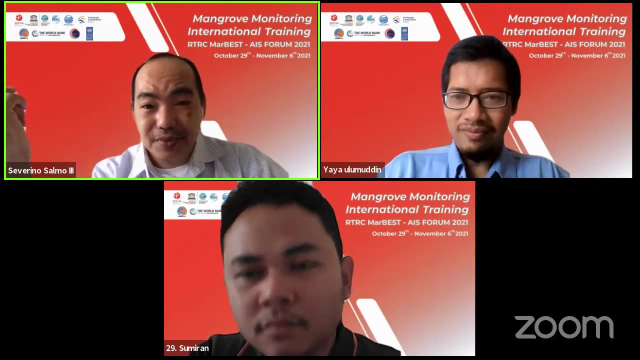 for you to estimate the age, But there are cases- and I know in Indonesia- when tambak is abandoned, for example 1990s, because it's no longer productive. So you know that in 1990, there was no mangrove. 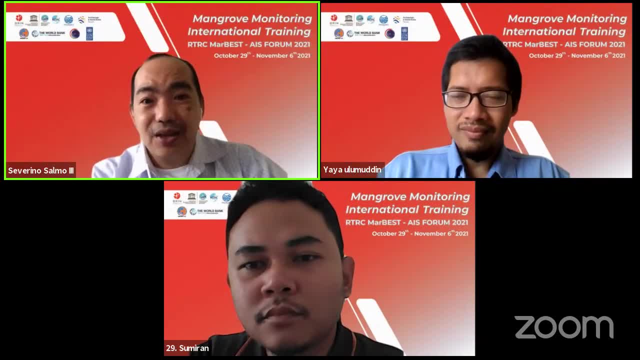 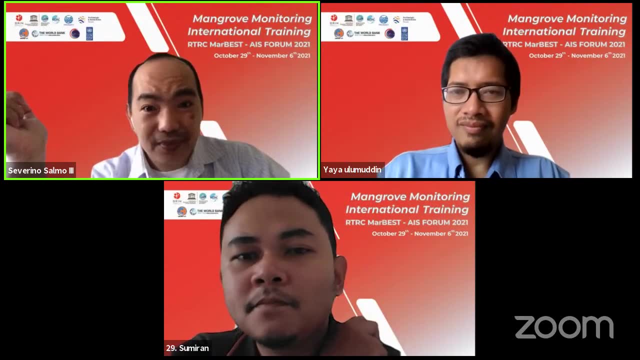 But then 2010,. this is Frida's site. All of a sudden, you saw mangroves that are healthy. Where did that mangrove came from? There was no planting. So you know that 1990 and 2010, that's 20 years. 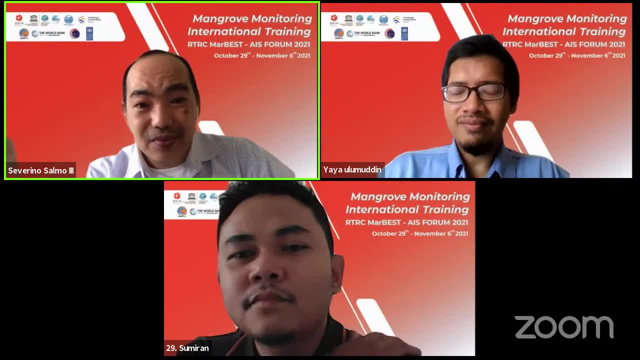 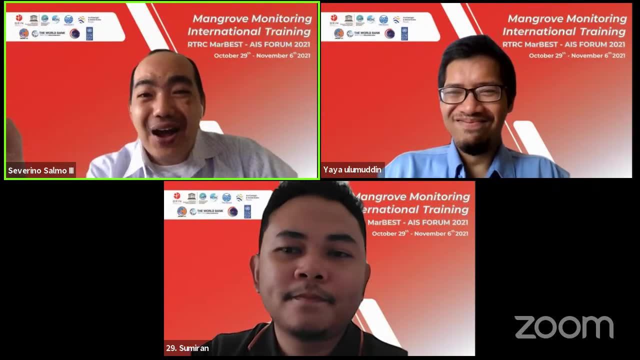 So you know the mangroves, the age of the mangroves, right. So it starts in your own backyard. I don't know where you are now. I don't have mangroves here. I'm living in a faraway place. 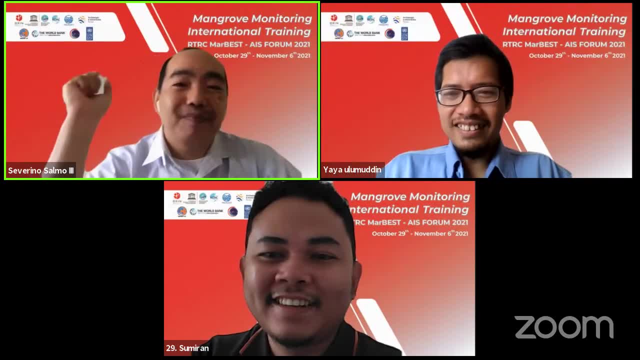 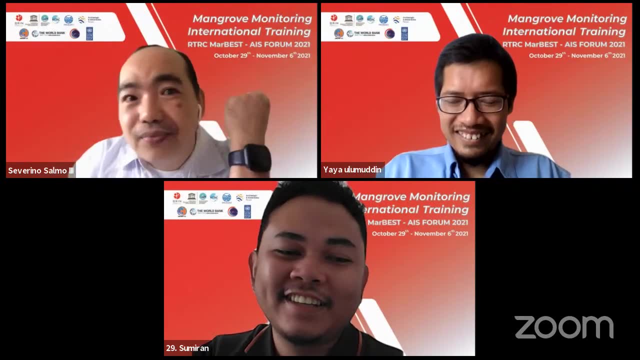 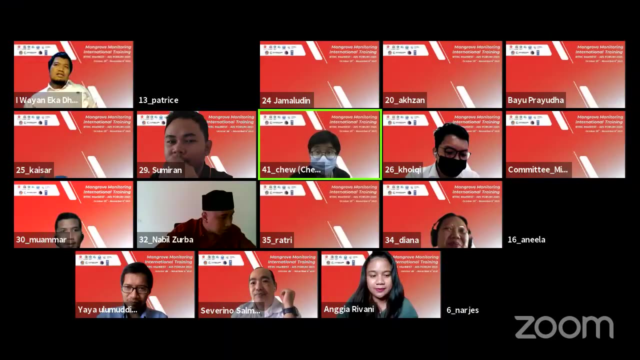 But if you have mangroves in your backyard, start tagging them, make a marker so that you have a reference system already. Yeah, Can I add in some comment regarding this? Yes, please, I'm Chiu from Malaysia. In Malaysia, for example, Matang. 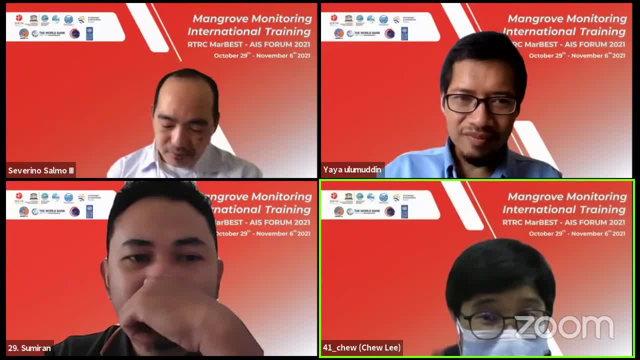 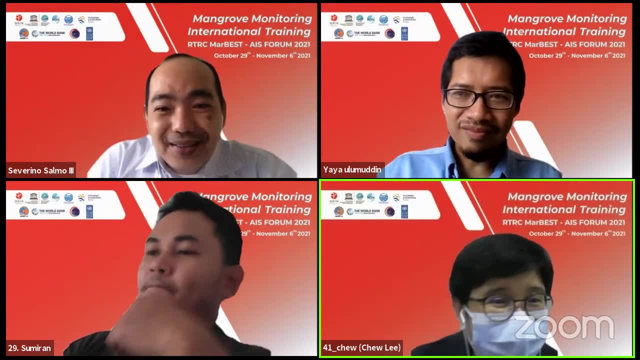 Matang is the forest. It is under the management, So we will be able to know the age of our forest. Yes, That's all from me. Yeah, Thank you, Chiu, for saying that. You know my good friend Aldry Amir, his father. 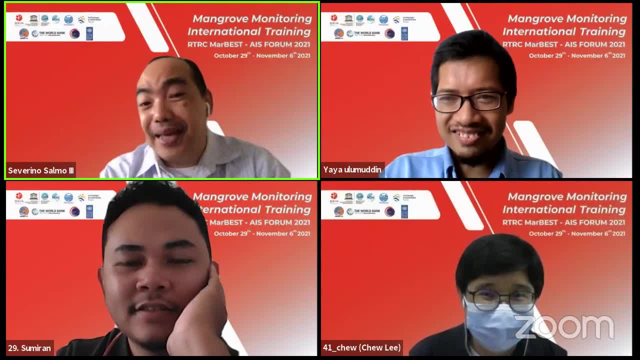 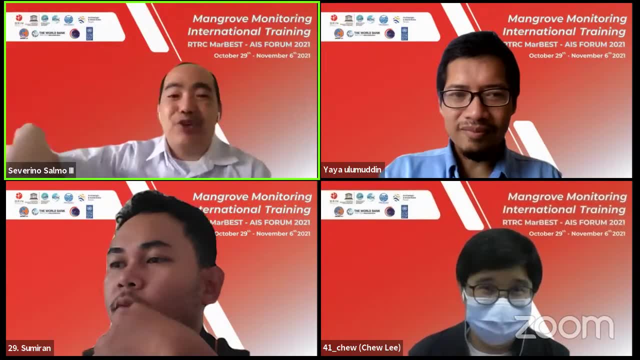 is a park administrator of Matang And they have good records of the age. They know exactly what is the age of the mangroves for a particular. I forgot your term. It's like a square right. It's a managed zone. 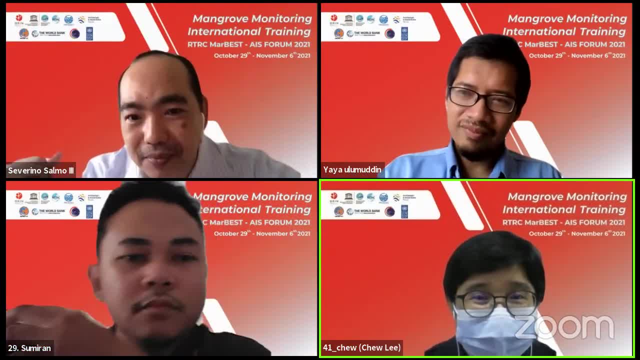 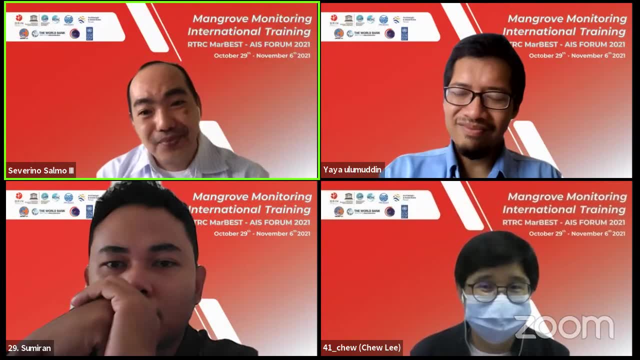 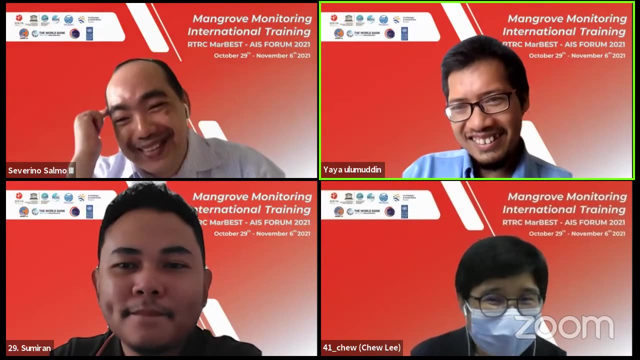 You cut it every 30 years. every 30 years, 10 years for one thinning. So they know the age. Thank you, Chiu. Thank you, Do you know Aldry? Yes, I know him, but I'm not very sure he knows me or not. 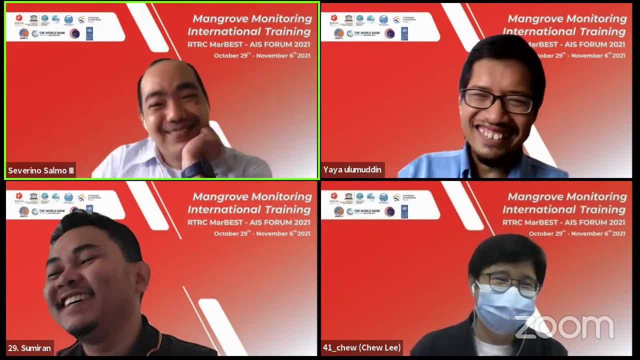 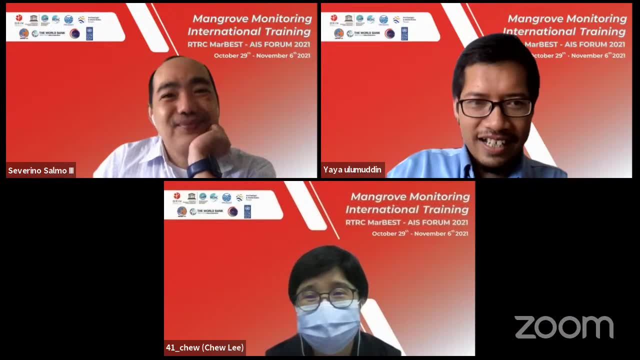 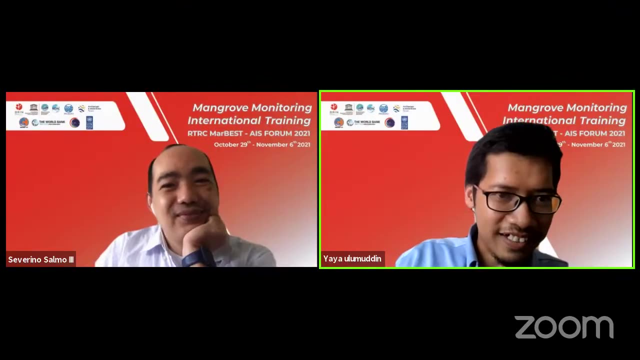 I'll tell him. OK, Amir, is it enough? Yeah, enough, Thank you, Lucas. OK, Sure, All right. Next question is maybe from Patrice, Please, Hi, Good Well, good morning from me. I'm from Malaysia. 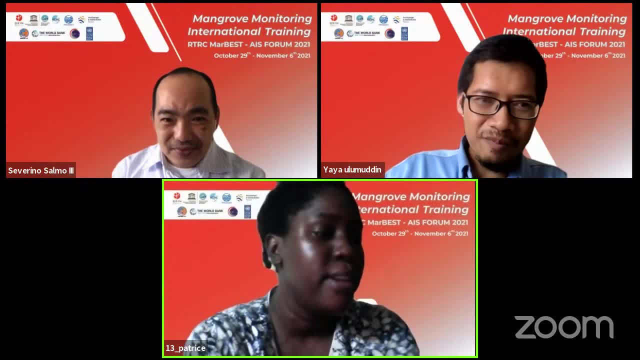 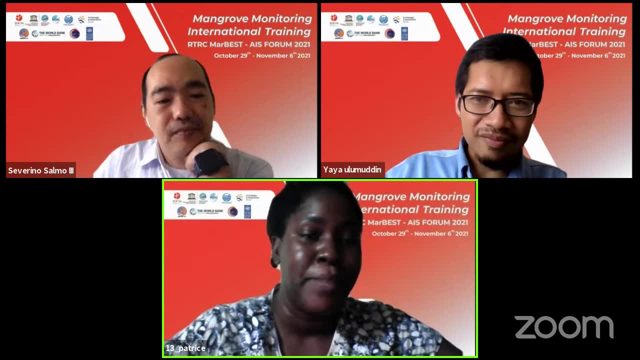 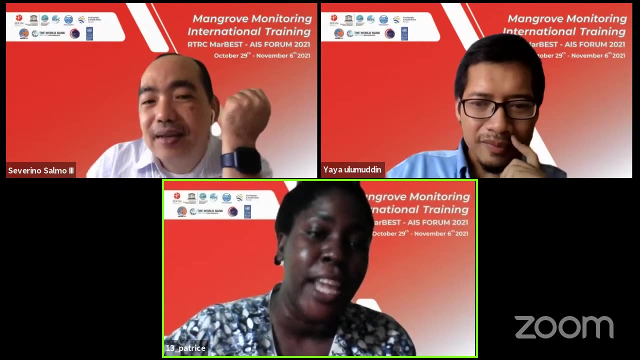 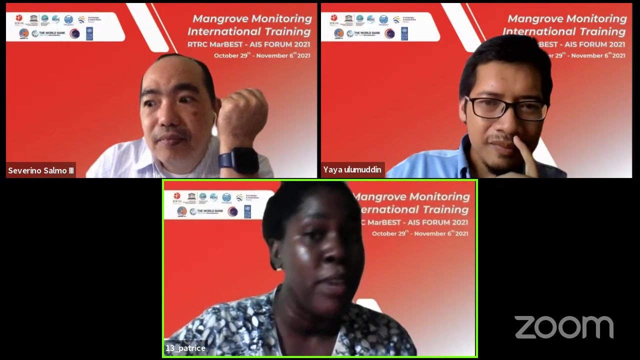 OK, I'm from Jamaica, in the Caribbean, And I wanted to know. you said that one meter baseline core is a must. But what if the depth is not at that level? Can we use lower depth value? And also, if we have the rooting system, it's preventing you from putting it in the core. 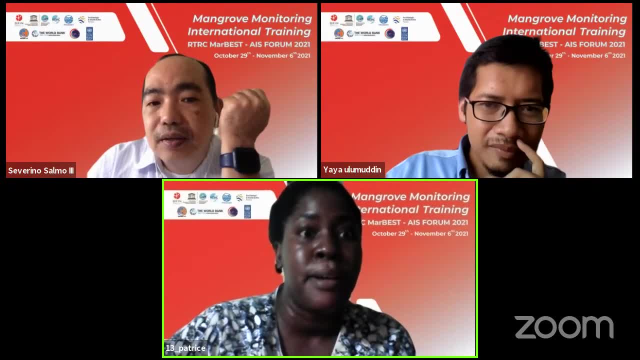 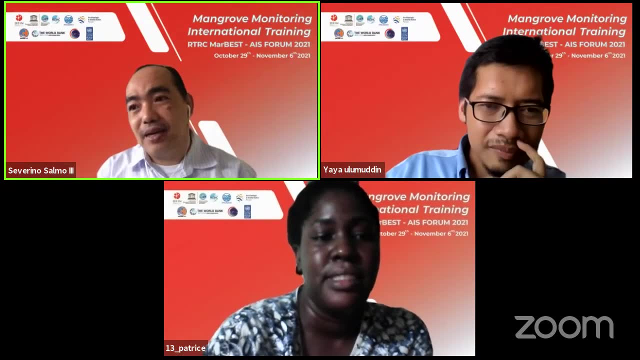 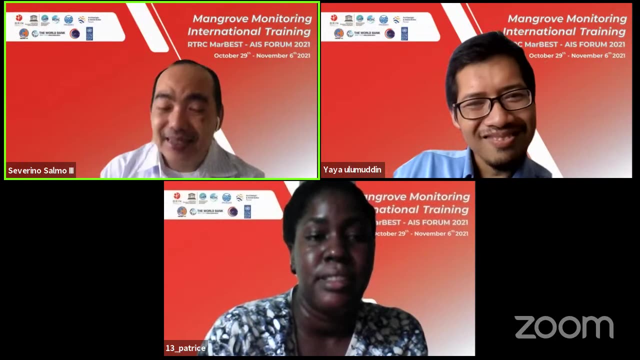 any further. Can we just use that depth as the baseline? Yeah, yeah, Yeah, I got your point. I also have sites that are in coralline substrate. In the coralline substrate, even if you use a hammer, you cannot get anything. 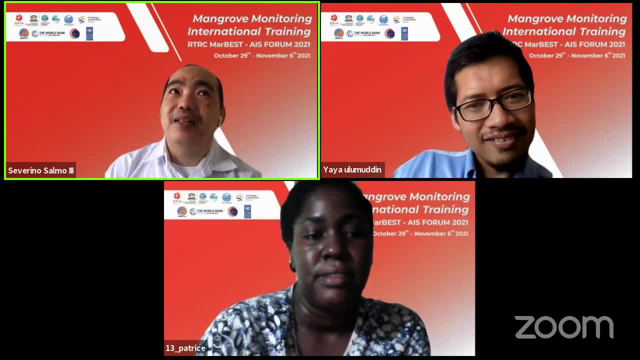 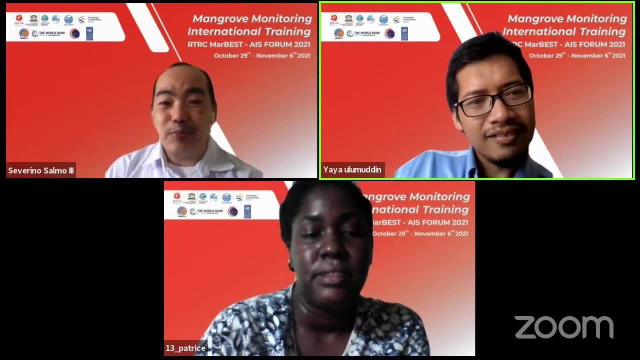 But yes, I know that there are some sites, Even here in the Philippines. it's very difficult to collect samples, But again, you follow the SIR definition. In the absence of a reference system, go for a coralline. In the absence of a reference system, go for a reference system. 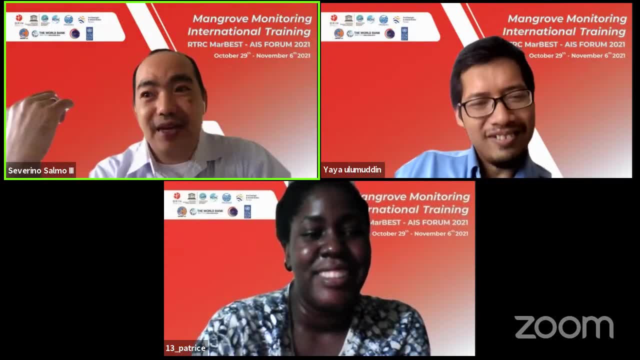 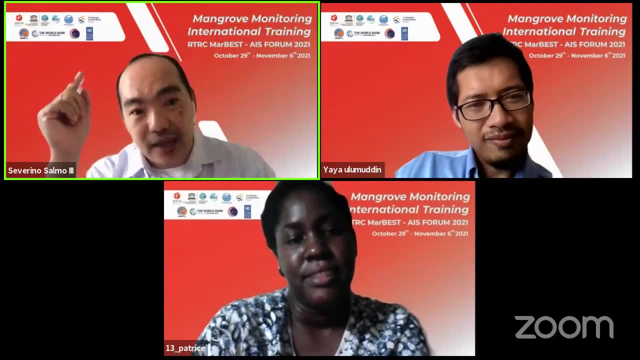 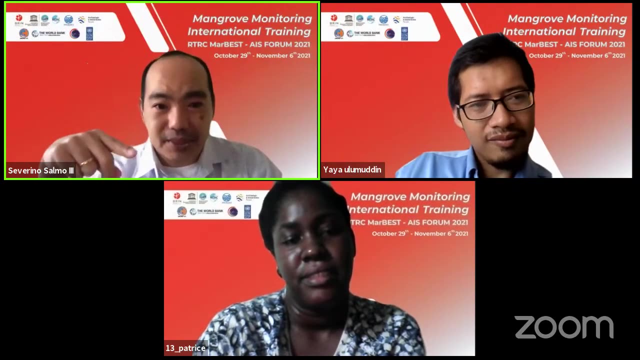 You just have to find the best available reference system. So I think when I suggested deep core samples, because the geologists think that what happens, what are deposited and accumulated in sediment over depths, represents the historical trend And that will give us some ideas. 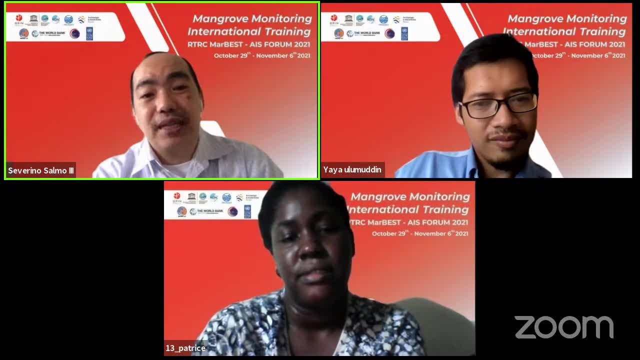 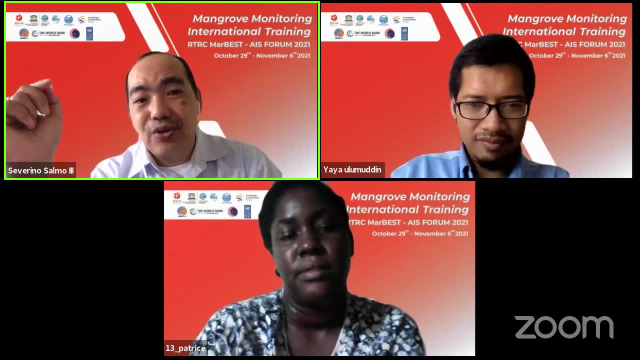 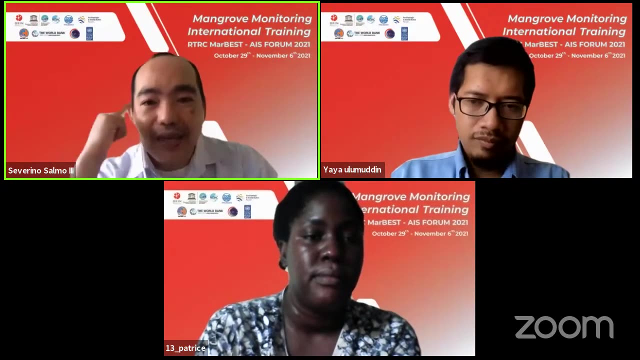 What was the organic matter, nitrogen, phosphorus content in the past And that will. those information will tell us what would be a reasonable target for organic matter or organic carbon content. So my short answer is that if that is the best depth that you can have, then might as 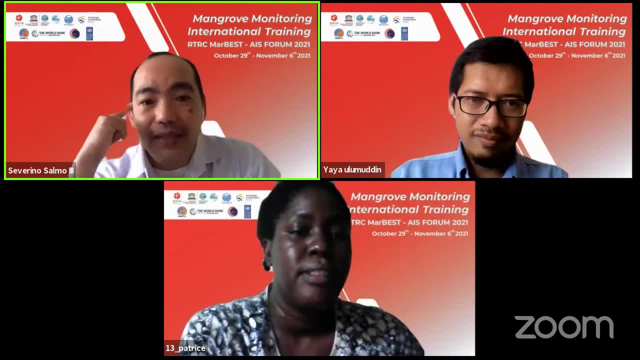 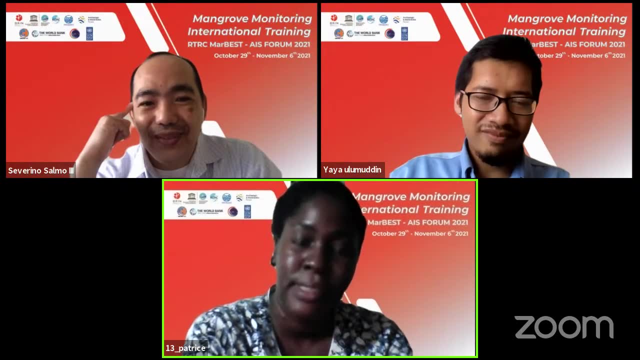 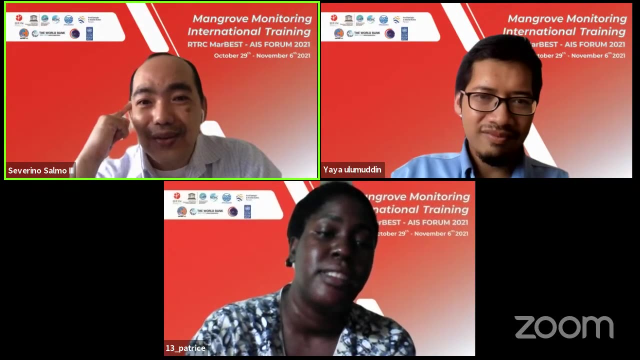 well, use it rather than having nothing Understood. Also, could you say what you use to determine your soil depth? Yeah, What do you use? I use an auger. I think Frida and I are using. you know, Frida, right? 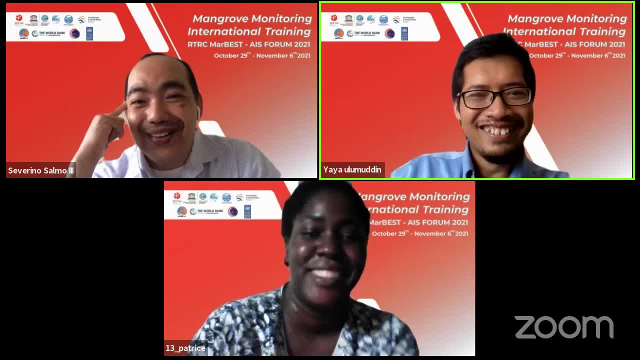 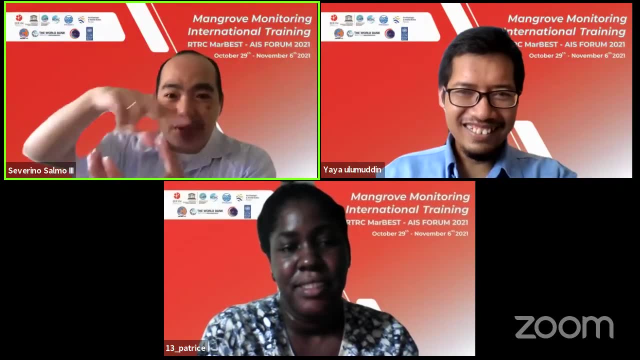 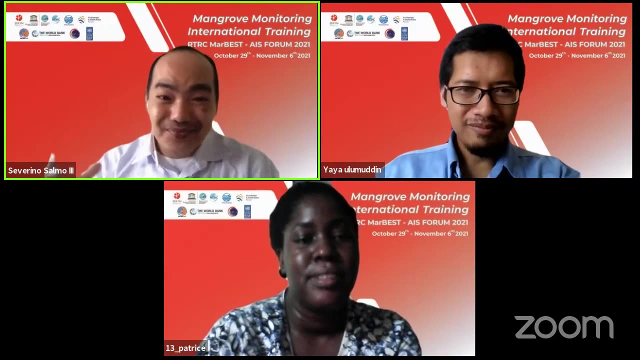 No, I know, Frida, We use the same auger. It's not the usual soil sampler. The soil scientist used a close sampler. It's like that will not work in mangroves. The vacuum will stop. It will not hold. 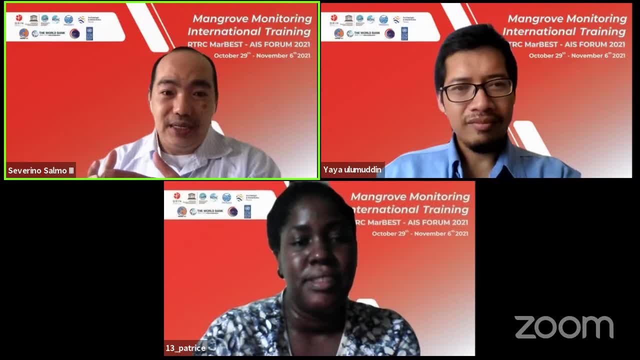 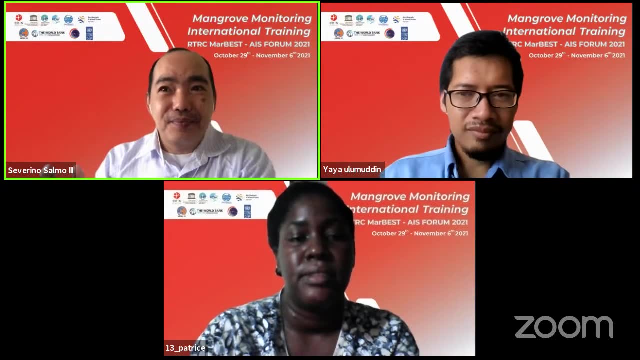 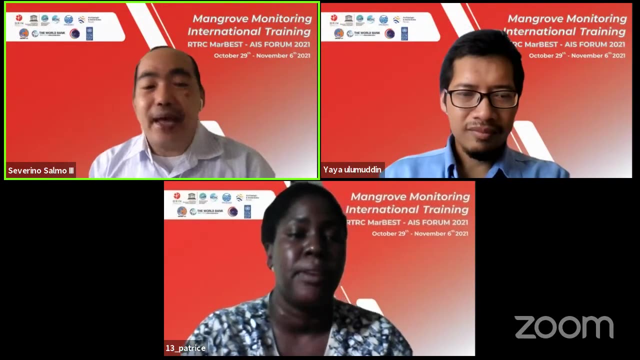 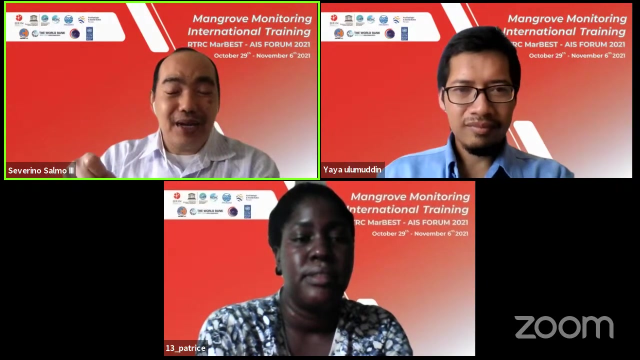 So we use the auger, We use the open face auger, And then it's very sharp for you to slice samples deep in the sediment. That's what I've been using for more than 20 years now. Sometimes people are using a hammer to hammer the sampler, the corer. 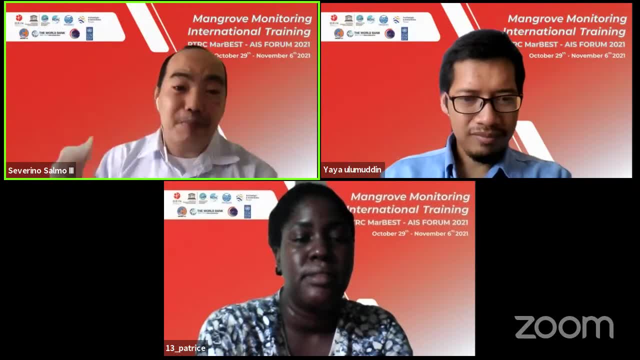 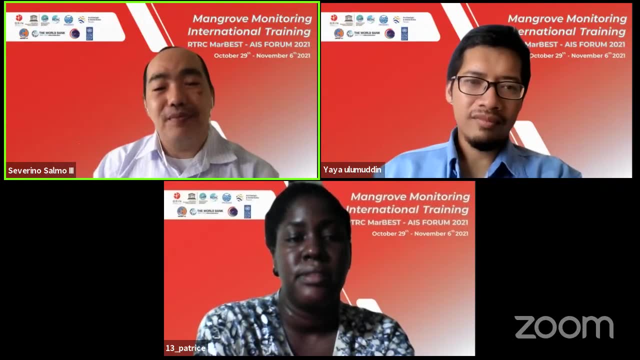 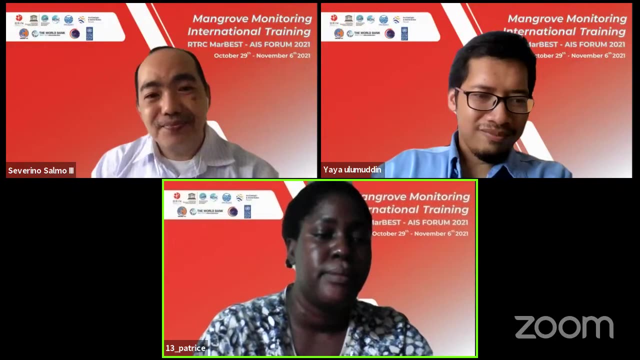 But I don't recommend that Because when you do, when you hammer the sampler, you're changing the sediment compaction already And it will give you a wrong values for organic matter Understood. Thank you, You're welcome, All right. 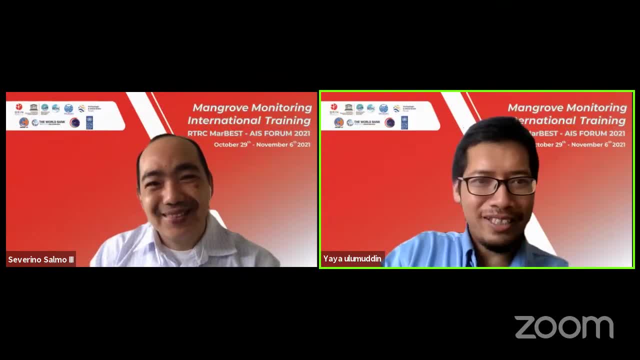 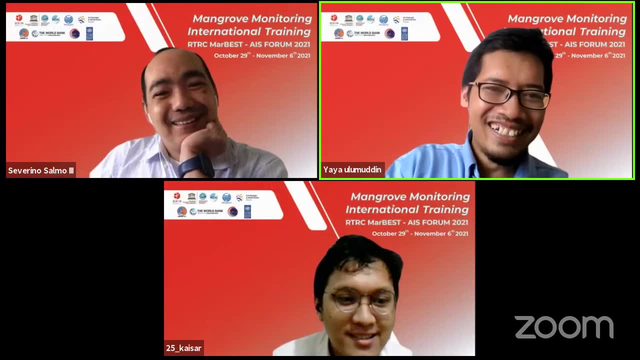 Oh, Anghia again. Do you have any more questions? But before Kaisar? I guess already raised your hand right. Please Kaisar first and then Anghia after that. Okay, Thank you, Mr. 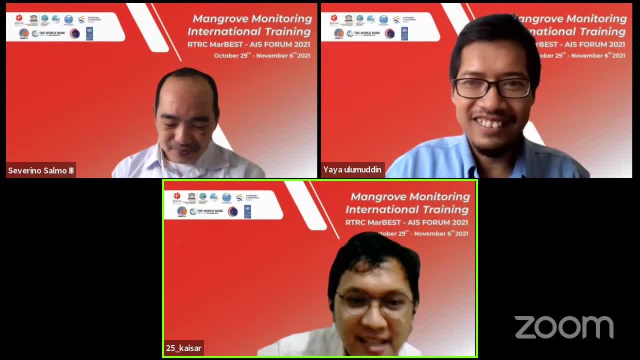 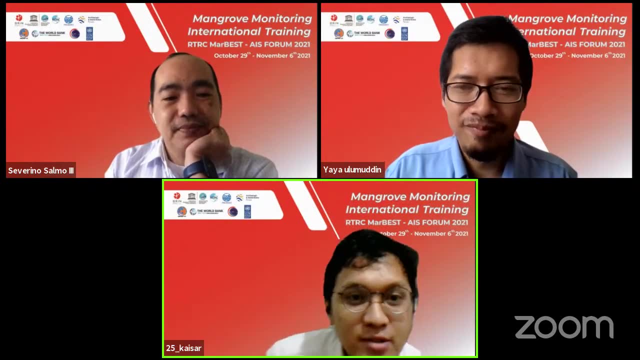 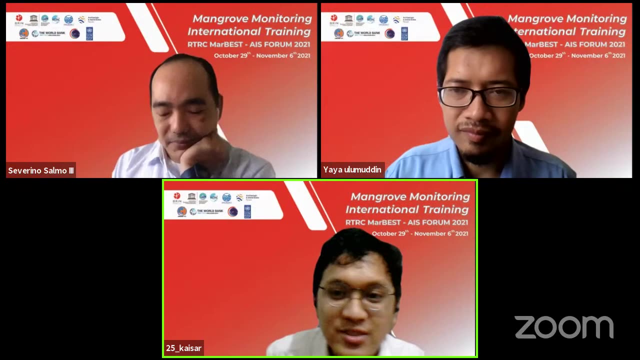 Yaya. So thank you, Mr, for the presentation before. So I have a questions about the restoration, especially So in 2020, we have the national economic recovery And one of the project is to rehabilitate the area of mangrove or the coastal area around in Indonesia. 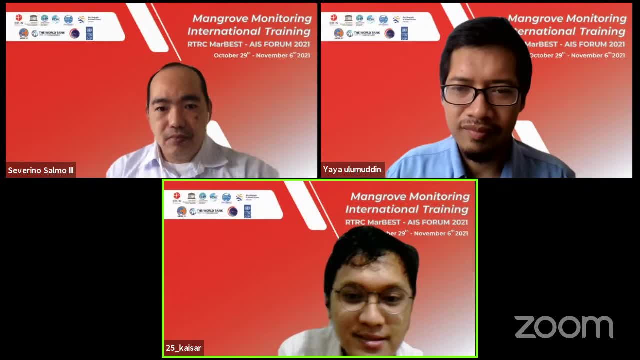 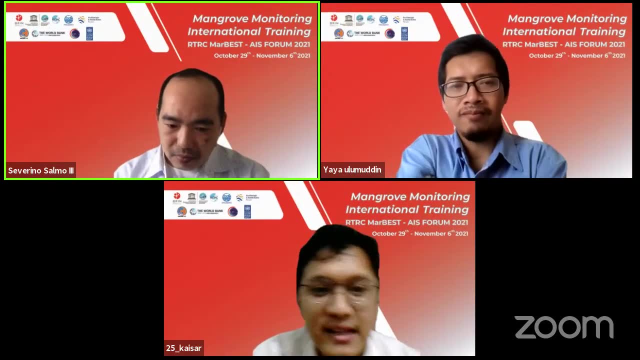 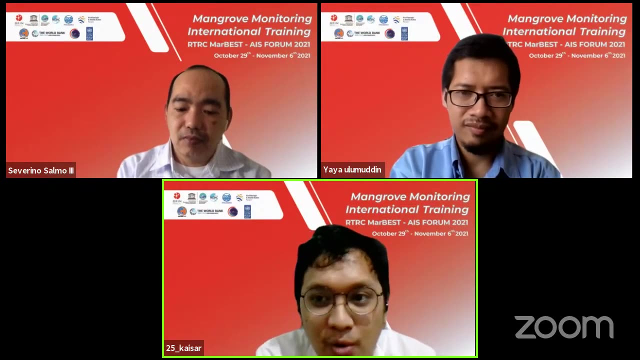 So Just a year before, we just restored the mangrove in Penajam in East Kalimantan And I know that there is some from your presentation. there is some define about the restoration, about the target goals or its success or failure. 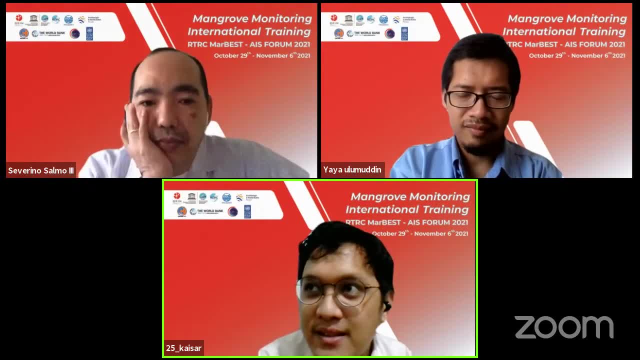 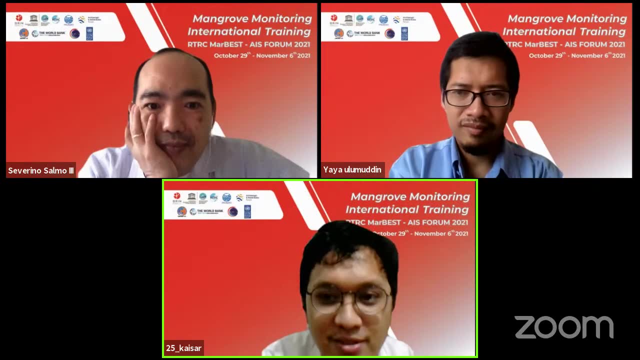 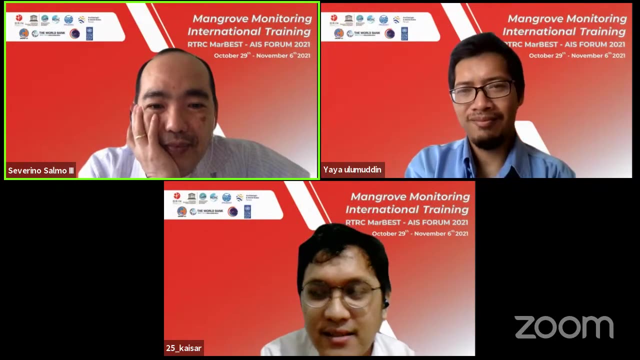 And from the things that I used to know in the restoration we commonly use the what is sulam Replantation or embroidery the seedling? again and again, Is it the moment we Replantation or embroidery the seedling? 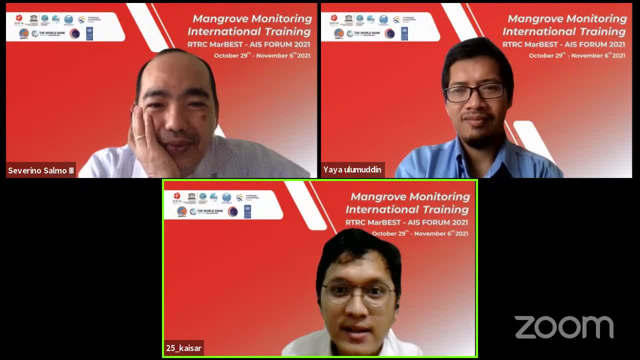 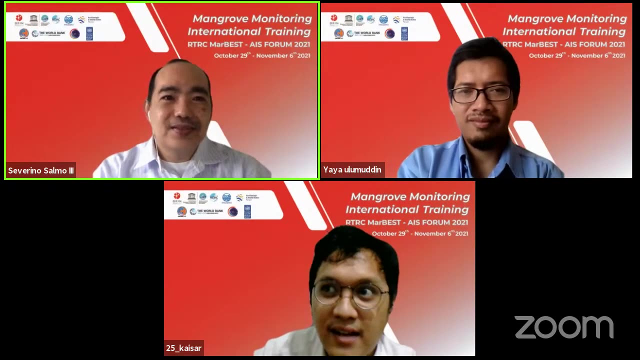 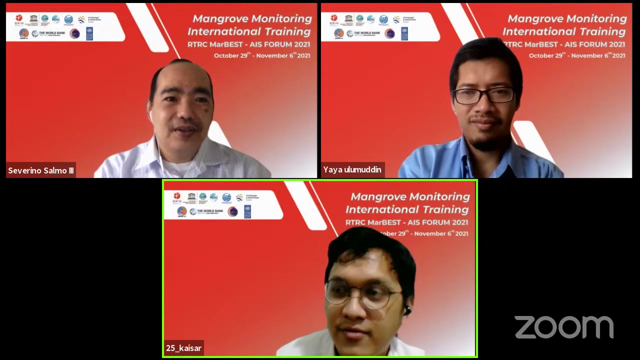 failure, Or we just waiting for another month or years to see the mangrove grow. Because, yes, there is some others threats to the mangrove itself, Like natural disasters, Like yeah, The wave gets so high. So we plant in two different type. in the front area is Evisenia. 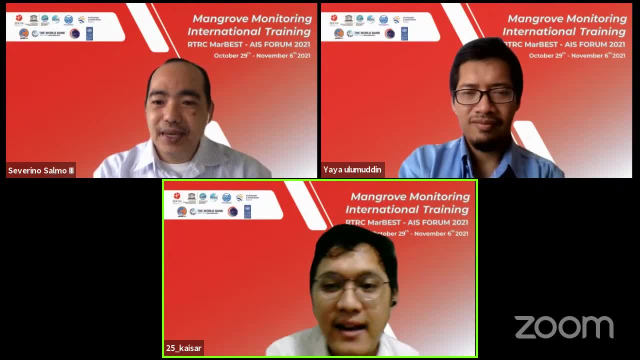 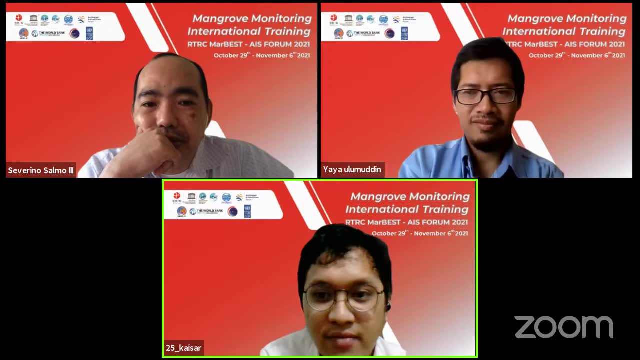 And then behind it this result like that. And then is there any approach that you say: can we can define this in another year or another five years? This is the success: restoration or rehabilitation. And then the second question is being mentioned, before yesterday from the Mr Novi. 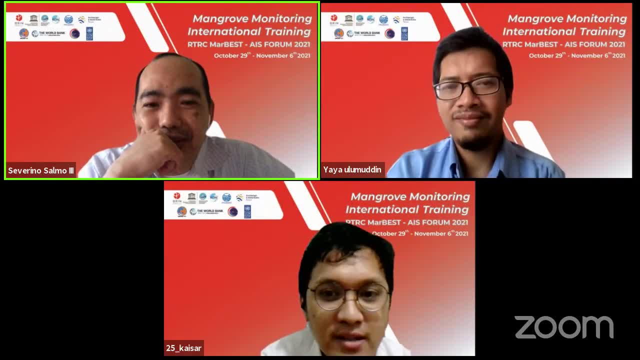 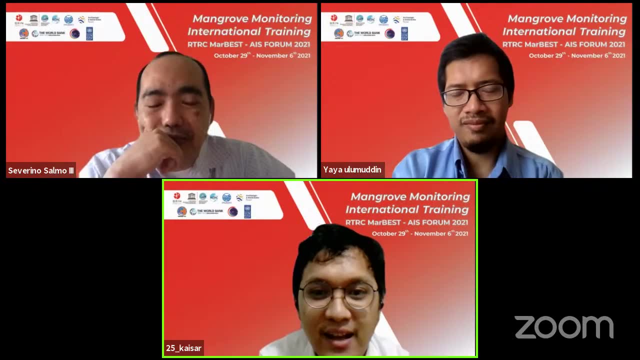 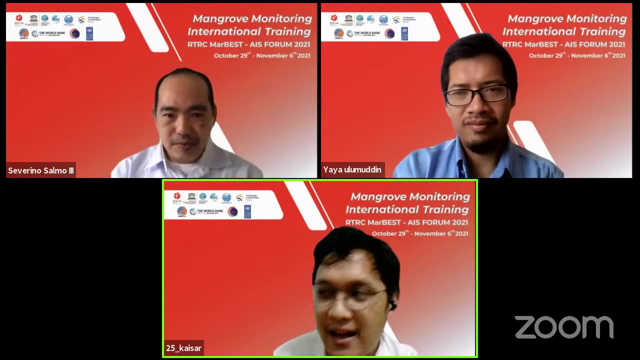 So in some area in Indonesia we have the coastal line degradation about because the tambak or the fishpond, And we do some restoration And after that the restoration having land, and we we plan the mangrove, But before, before, the degradation of the coastline. 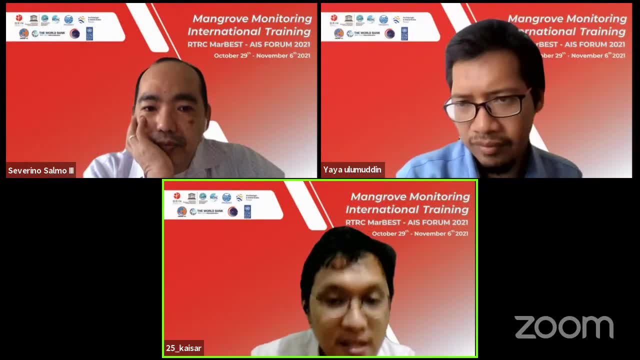 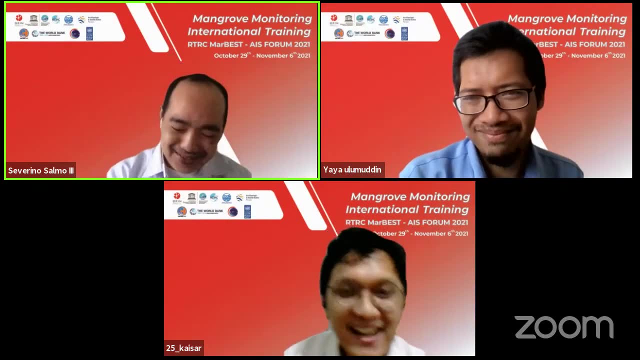 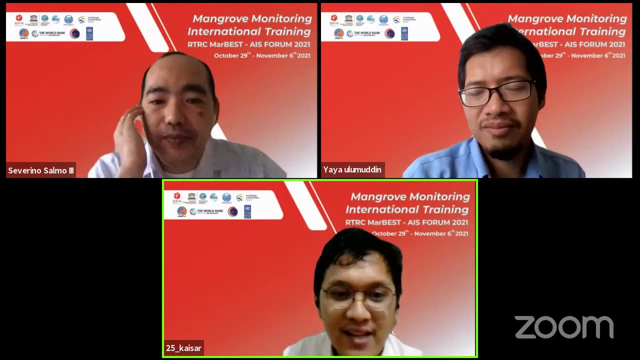 it's a house for our settlement from the communities or local communities, And they claim this is our rights. Is there any cases in the Philippines? Yes, Like that's, because we know in the Philippines the natural disaster like typhoon maybe make the coastal line degradation and new tourists to maybe that. 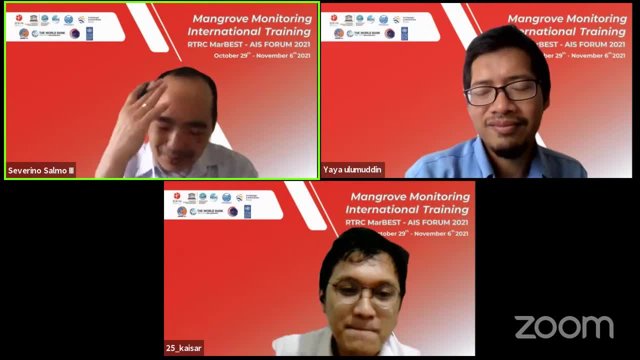 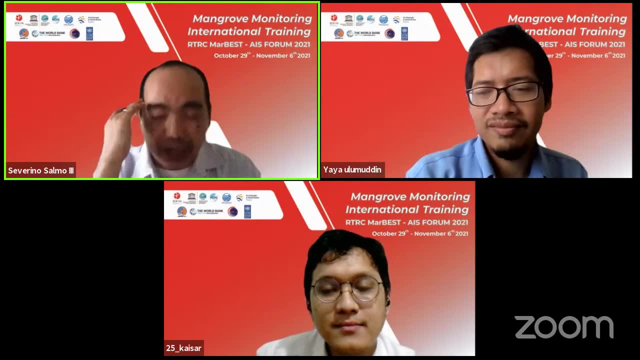 Thank you, Mr Severn. Let me assemble my thoughts first, When you say national economic recovery, I think we're also doing that in the Philippines. I don't have any doubt that if you do restoration, if your restoration program is successful, 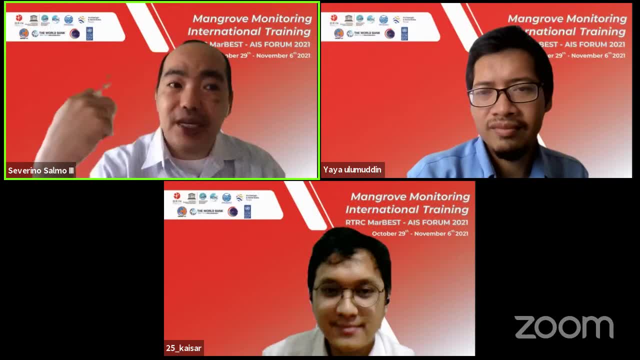 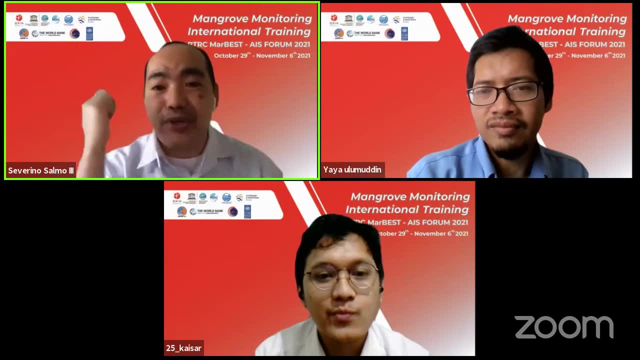 I don't have any doubt that it will give us resources, not just biodiversity but molus. We're eating molus here. I'm sure in Indonesia you're also eating molus, And if you do have a good restoration program. 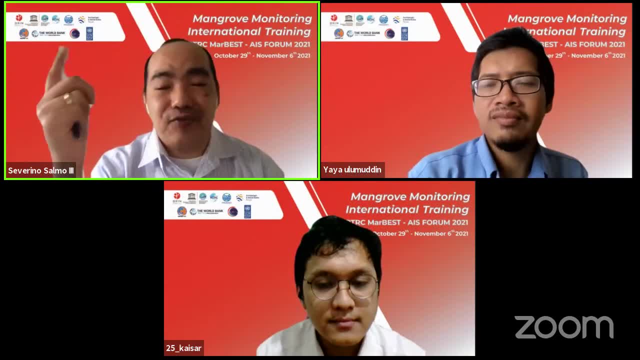 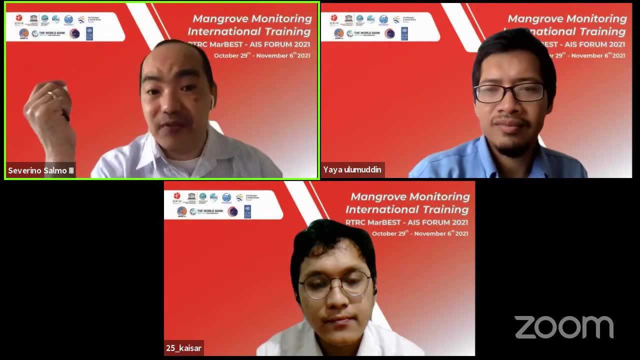 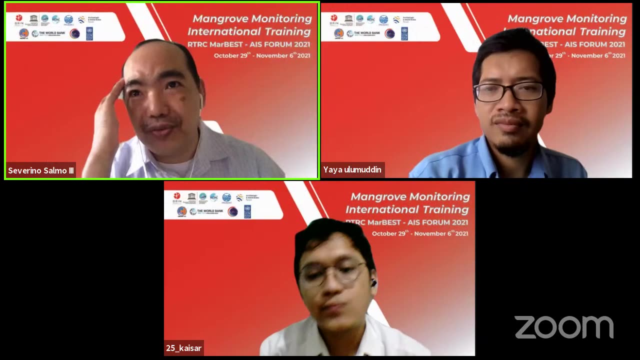 fisheries will be enhanced and fisheries will provide livelihood and income to people Right there, and then it will give you economic benefits, aside from protection from typhoons, disasters, etc. But your other question is like when you do planting, and planting every year. Did I get it right? You plant every year. It's like no, it's like the seedling before It's there, And then we replanting again. Yes, Yes, We have that same thing Because of crabs or anything, something like that. 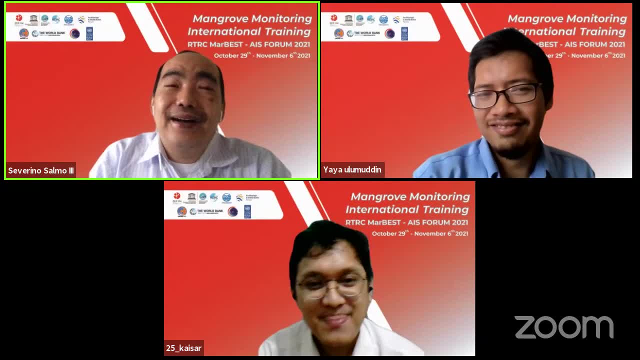 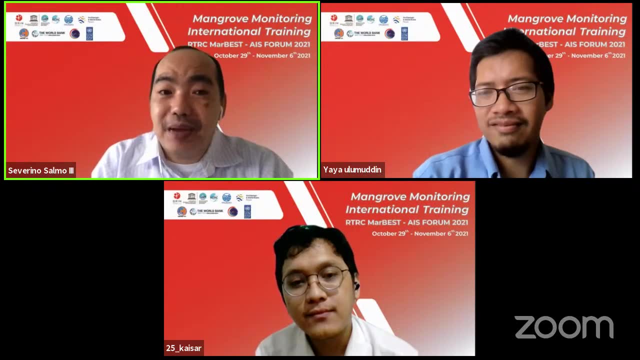 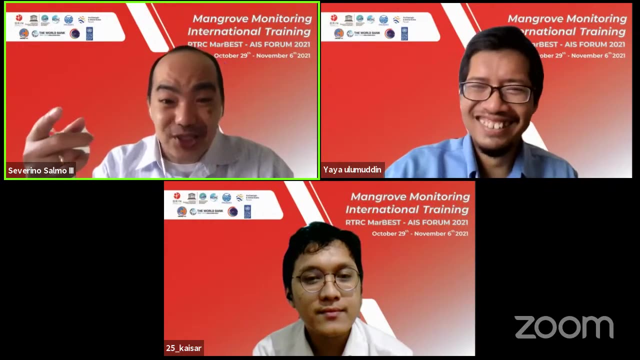 Yeah, Yeah, You know my answer for that. If the survival rate, and if you're doing this over and over again, then something is not right. I'm not saying something is wrong, But something is not right. Maybe it's the same, because I don't want to offend politicians here. 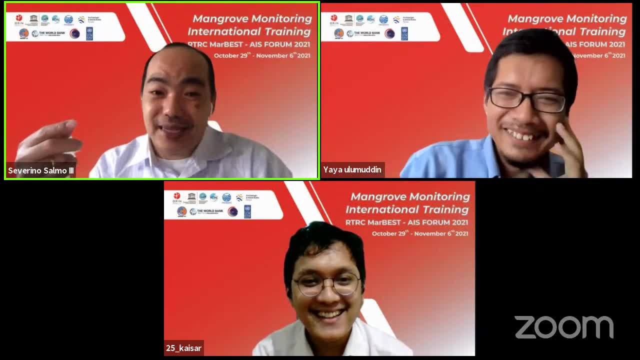 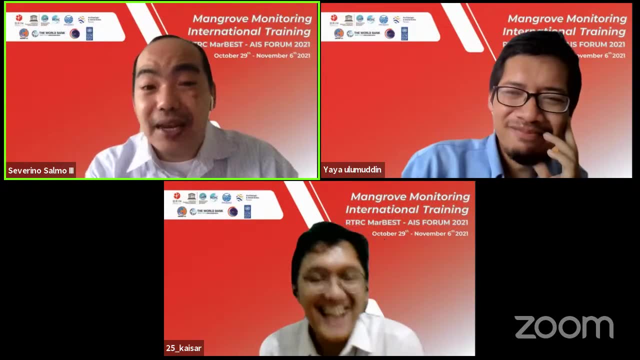 You know, you know the difference when I say something is wrong versus when I say something is not right. That spells the difference. But it's really wrong, You know. Yes, Yes, It's a waste of money. Maybe the site is not really good for restoration. 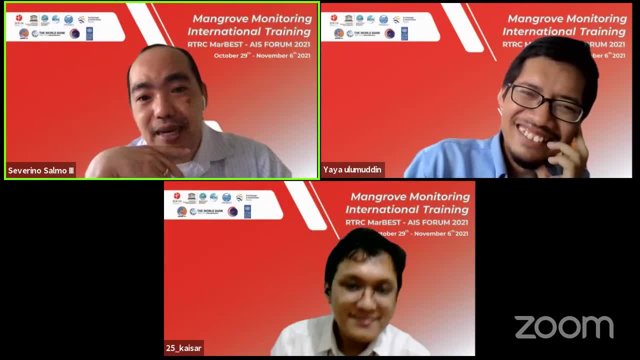 Depth and the coastal degradation. the shifting shoreline will be a big factor. If your planting site is, you know what's the if the tidal amplitude is more than one meter. Yeah, Yeah, Yeah, Yeah, Yeah, Yeah, Yeah. 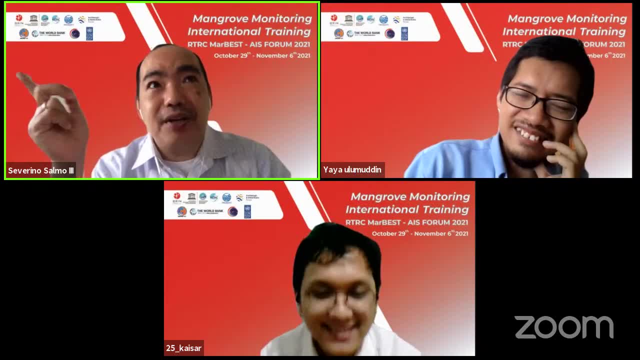 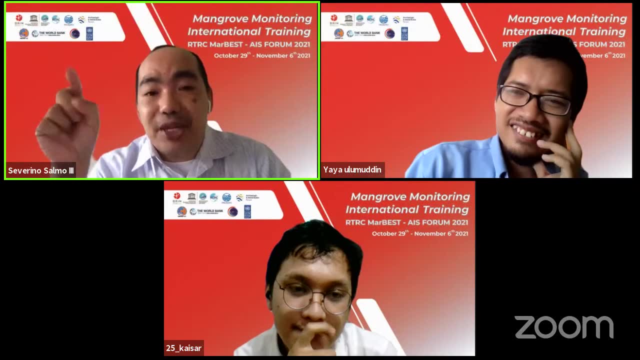 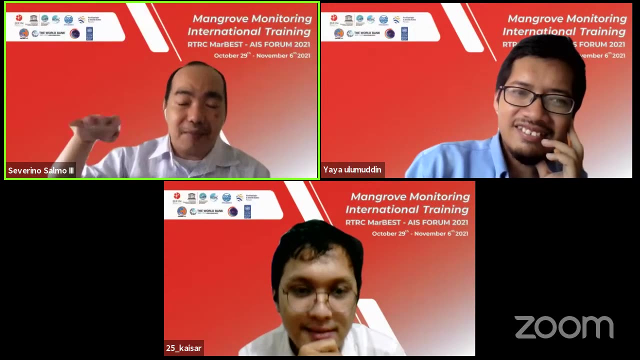 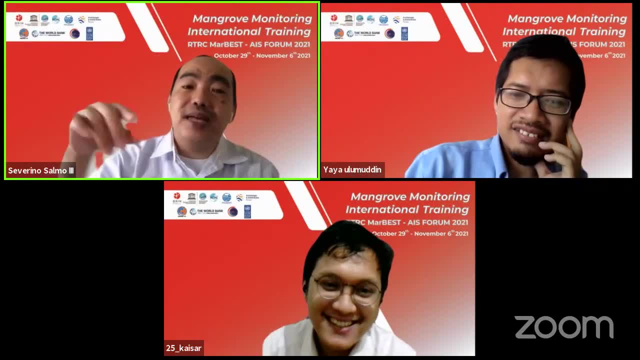 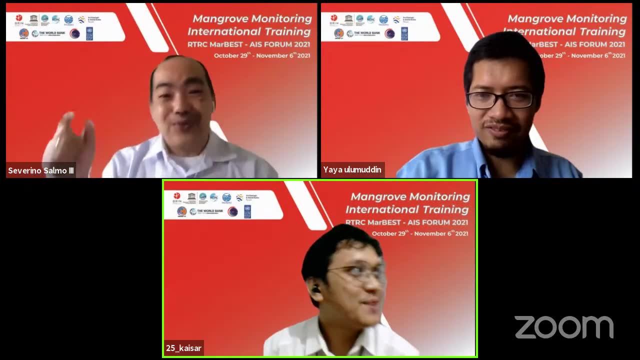 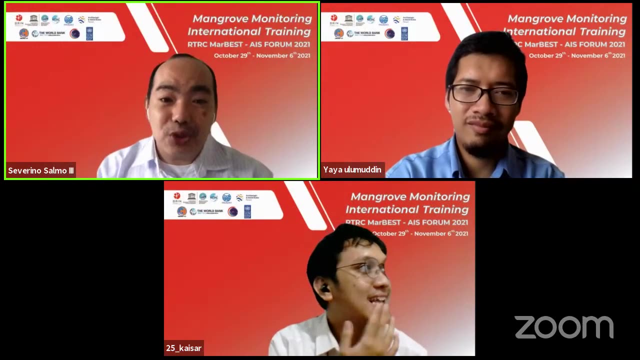 Mangroves will have a very difficult time to grow, because what is the height of your seedling? one meter, Do you have? do you have a one meter seedling? No Right. So if you, if you have a one meter tidal amplitude, then we're not even talking about high tide. 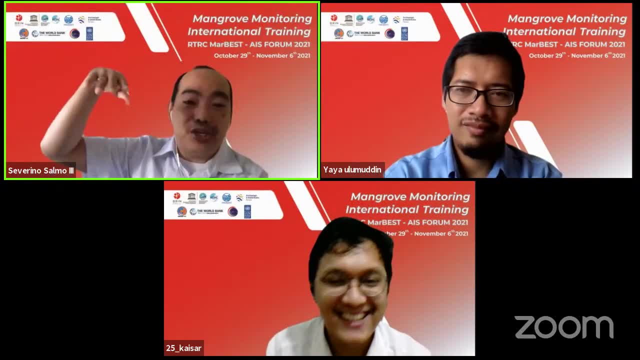 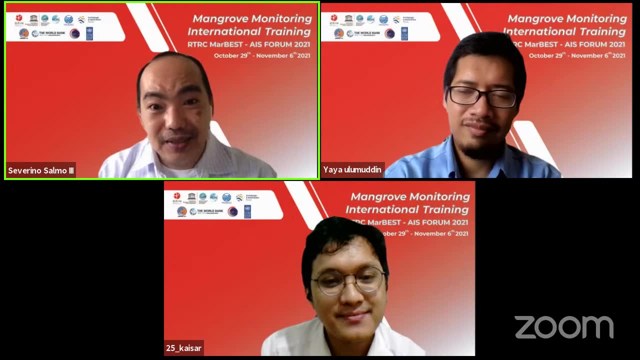 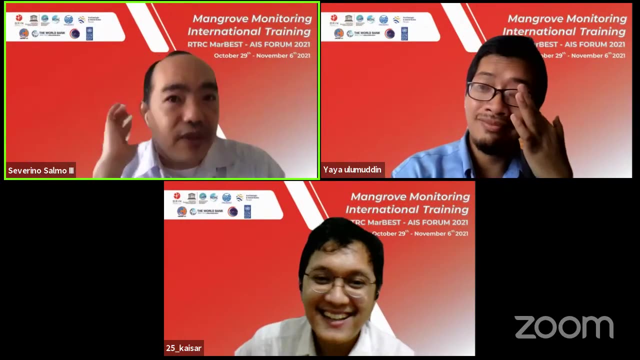 yet obviously that will be additional one meter your planted seedlings. what will happen? it will. it will be drowned right. it will be submerged underwater. yes, it will be. it will be very difficult to grow. uh, i, i don't know. um, there are places in indonesia that are not all places in indonesia. 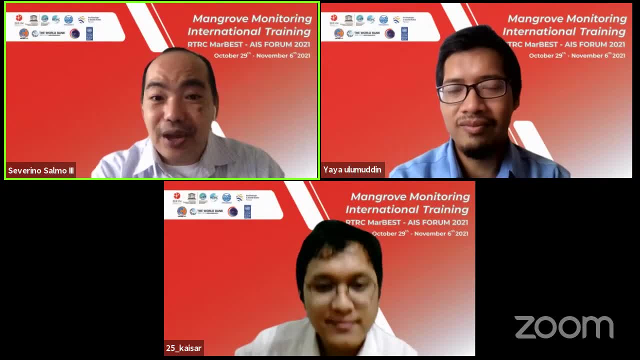 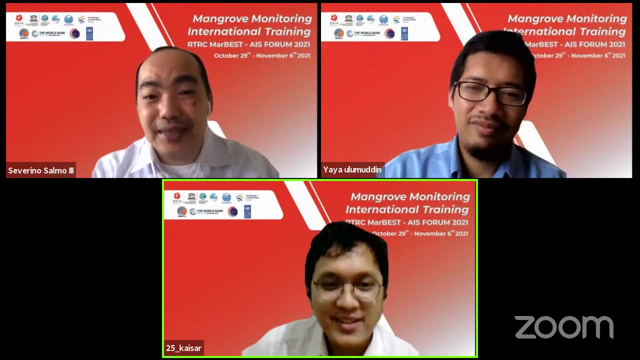 are are degraded like that. right, you have so many places. if you have the money, if you have the resources, why don't you do a restoration in, uh, restorable areas, areas that are correct to to do not, areas that are wrong to do restoration? and i hope i'm not offending 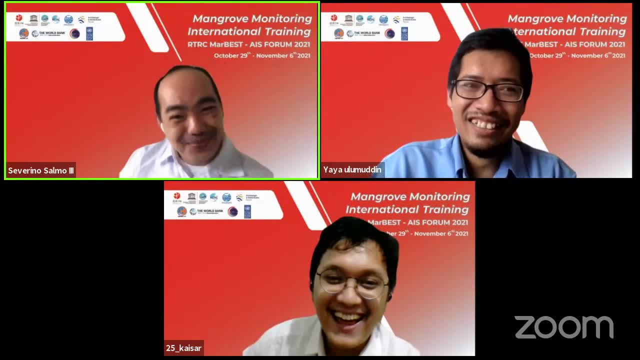 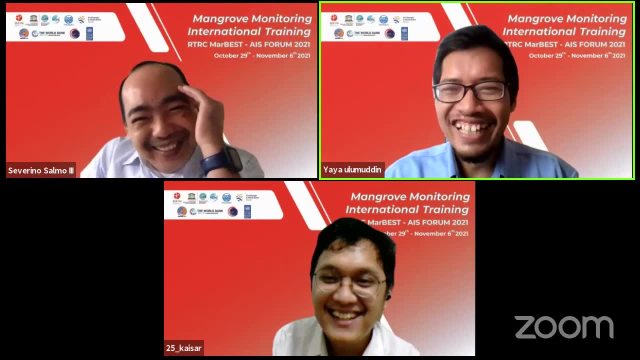 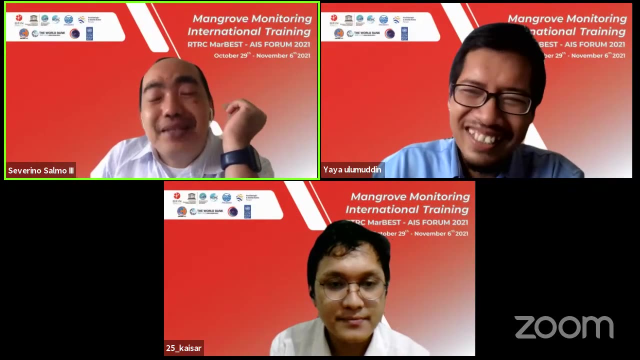 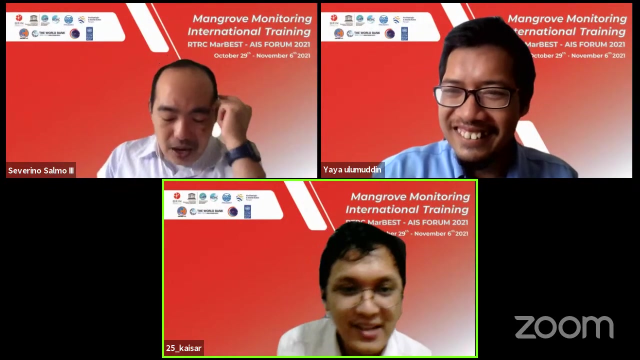 your politician. you know i'm very good with uh- not at all listing of the words. you are being recorded and it's open on youtube, but that's fine, you, so we have to do something. that is right, thank you. oh, for the second question, maybe you have the answer, uh, about the local communities. 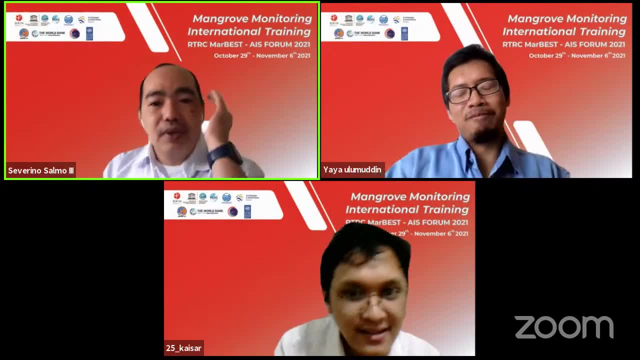 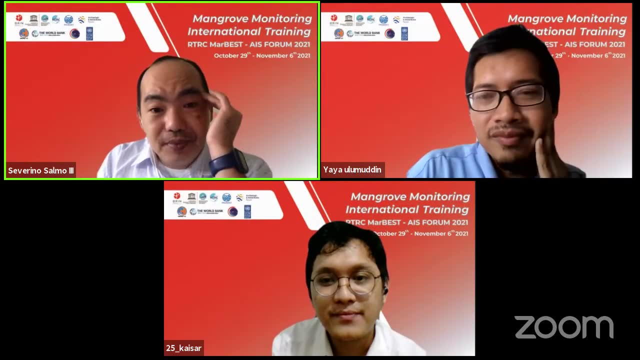 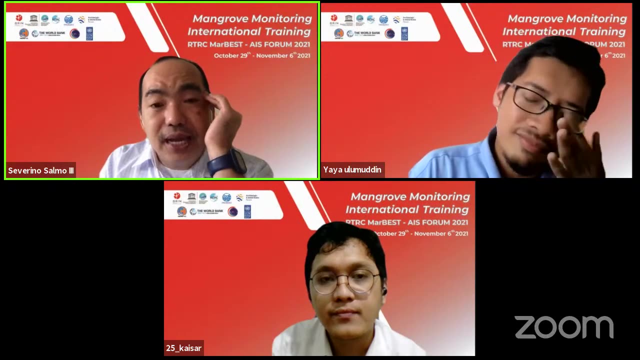 that claim after the land being in philippines maybe, i don't know the cases. yeah, we have cases like that. um, we have indigenous people like, uh, you know, tribes, native communities. we do have special laws for indigenous people. if they occupy a land, that's really them, their, their property. but 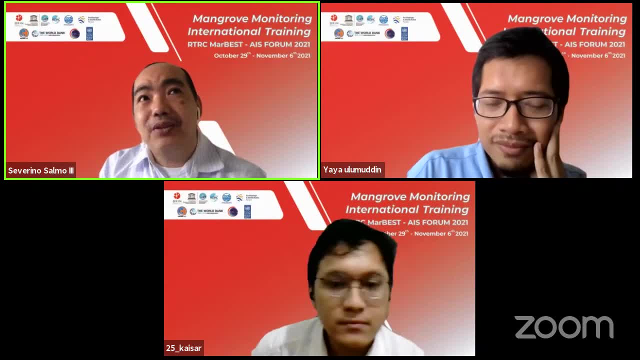 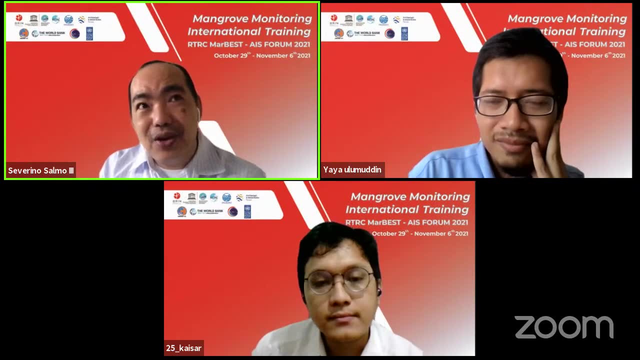 in most cases if a private uh owner will claim ownership to a mangrove, that's very difficult and we always encounter that problem. the way we treat that is that you know if you don't do restoration now, it's not just only you that will be affected. obviously the entire community will be affected and 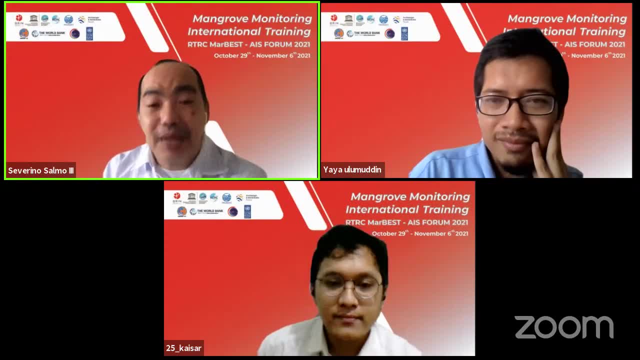 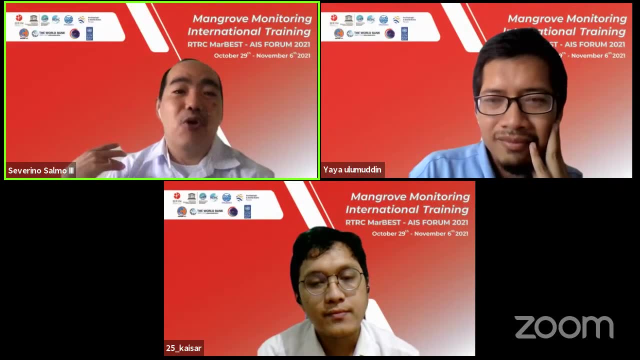 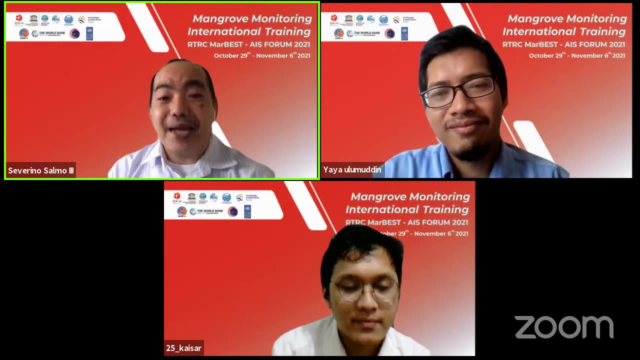 then luck. if you're lucky, you will be able to convince them. if not, then we have the same case. it's like it's like a dead end. uh, nothing we can do about it, because they they can invoke their political rights, their right for ownership and so on and so forth. it's very difficult, but for those 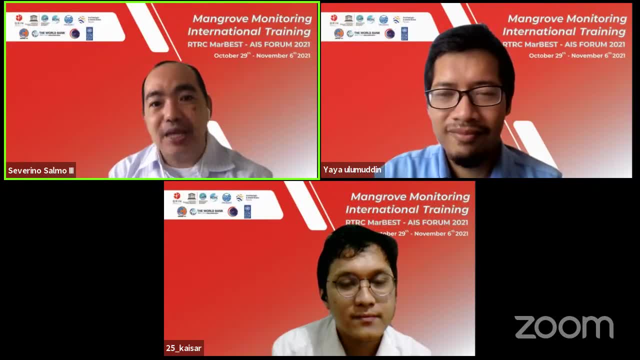 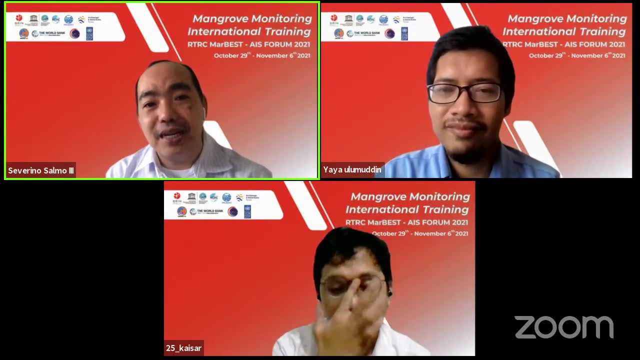 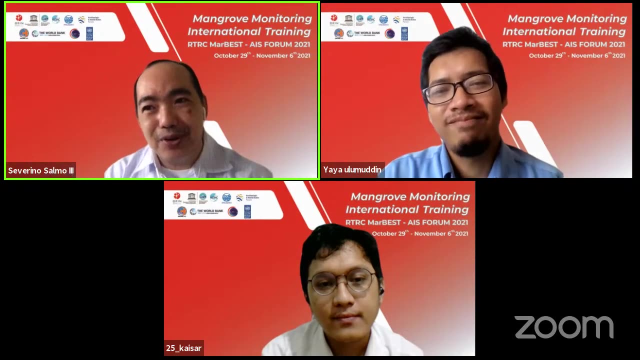 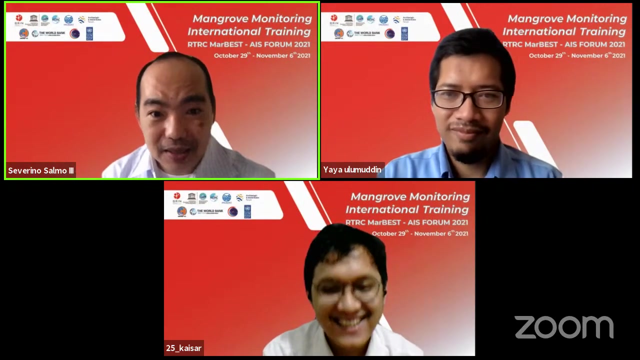 people. i think it's a matter of explaining to them what is the mangroves doing for us, for the humanity. uh, i think they are easily convinced. i find more difficult to convince, um, people who want to do to construct airport in mangroves because they have the money. those are more difficult to convince than the regular people. 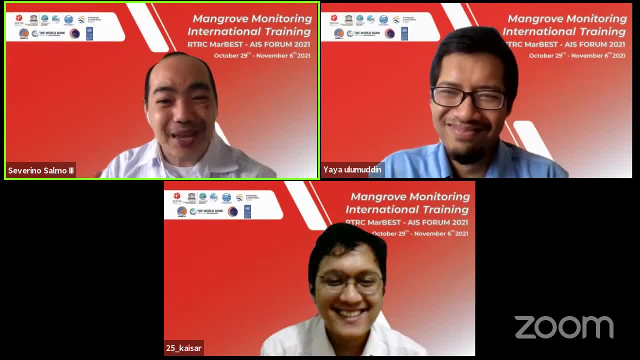 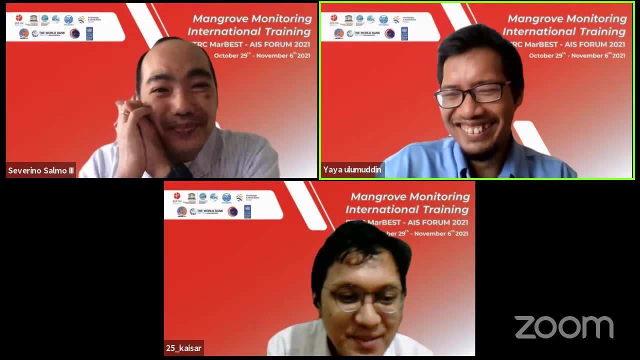 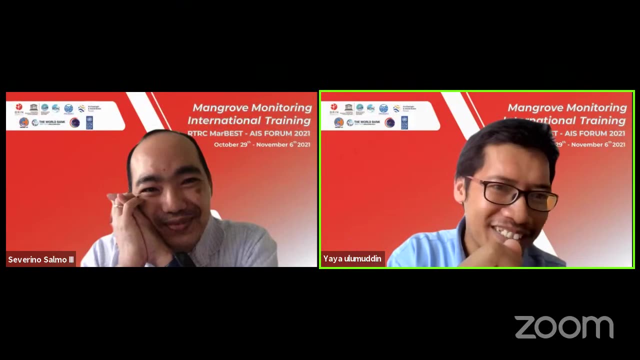 why are you smiling? they had the same case and i accept that this is recorded. okay, thank you, mr safruno. sure, all right? uh, angia, can i give an opportunity to abdullah first, because you have already asked a question. so okay, abdullah, please. 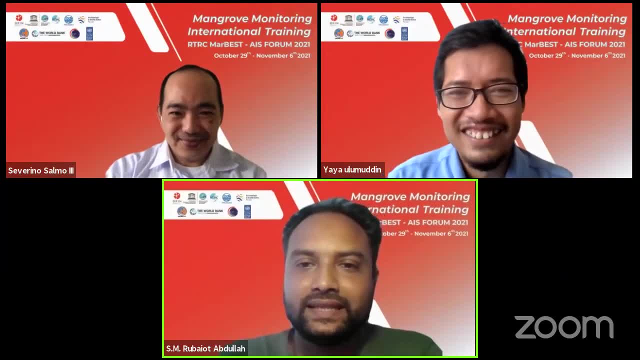 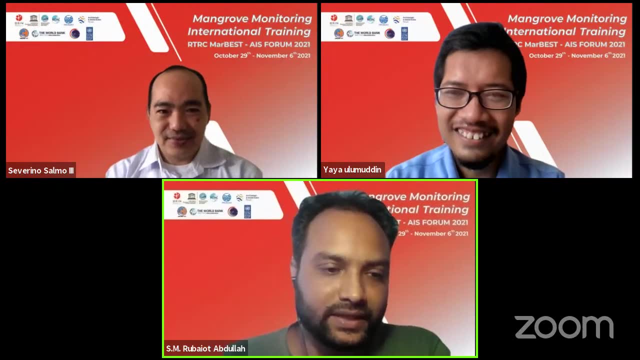 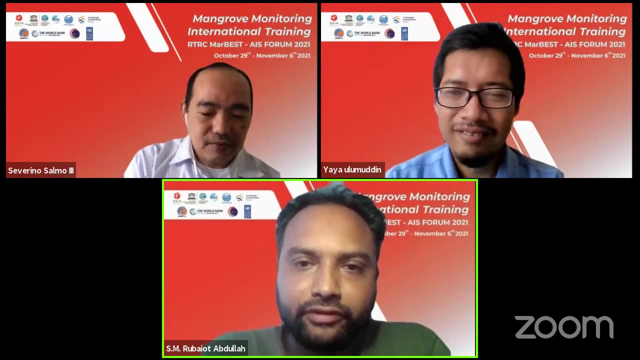 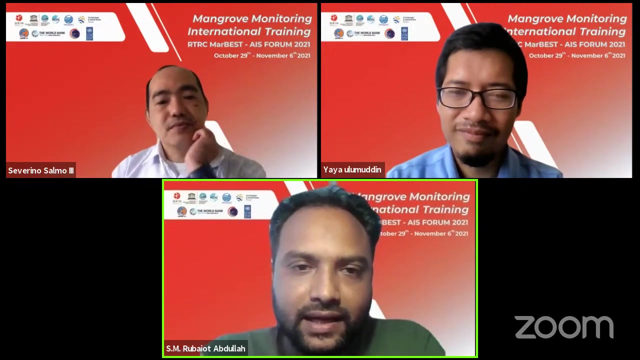 uh, thank you, yeah, yeah, and thank you uh saverino uh for your nice presentation and i'm from bangladesh uh, so you know uh we have uh different types of mangrove forest uh in our bangladesh uh. one is natural mangrove forest and one of the biggest chunk. 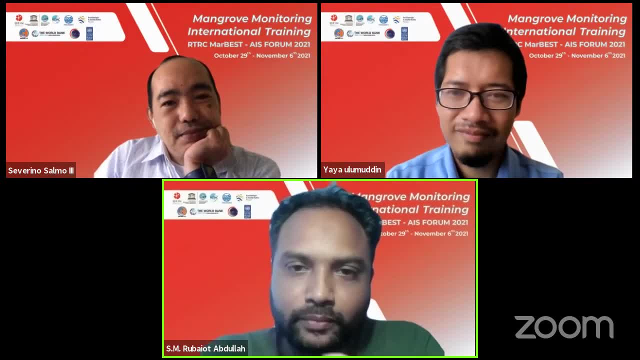 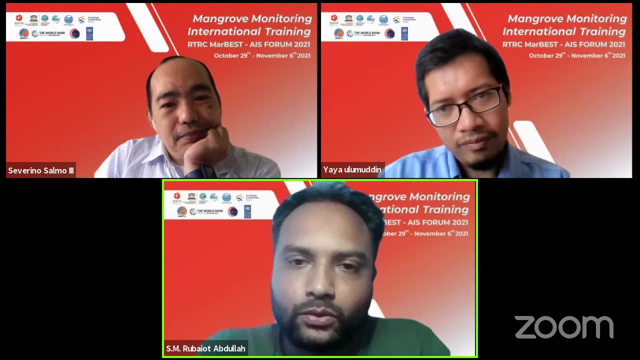 of mango forest uh in the world, the sundarban mango forest, and we have several coastal plantation also uh. but in your presentation you mentioned that uh in southeast asia we have only 22 protected area, but uh sundarbhan uh in bangladesh, uh, it consists of uh 6000 square kilometer. yeah, that's a lot of area. 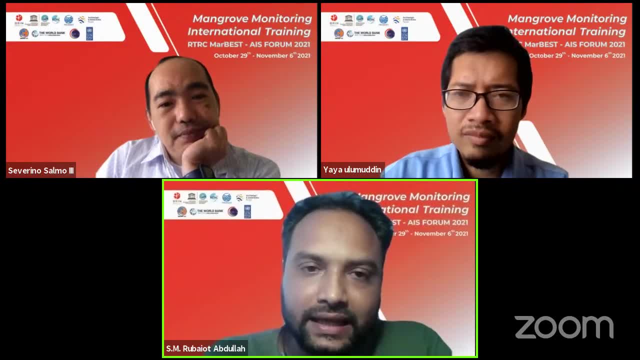 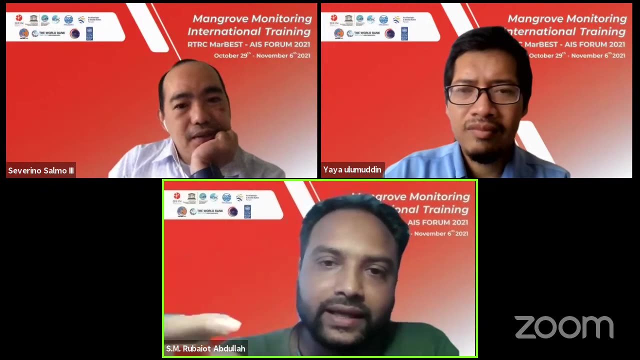 and total area is reserved. so in our country the reserve forest is more protected than any cons any protected forest. yes, yes, yes, i agree. so total area is protected. nobody can enter without any power. so total area is protected. nobody can enter without any power permission this forest. So if you have the permission of collecting some non-wood forest, 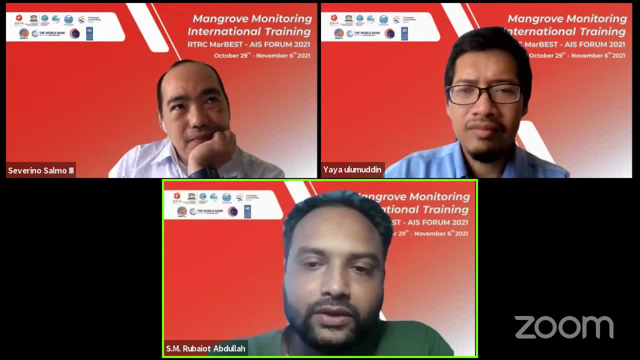 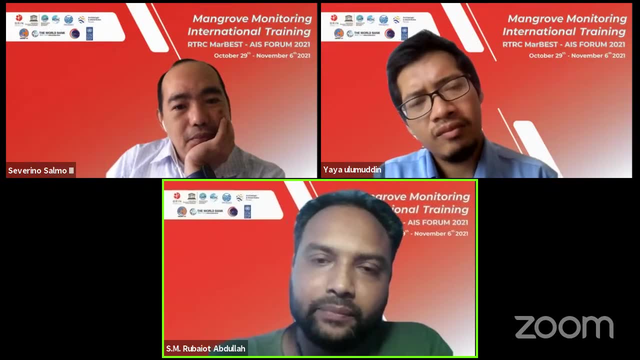 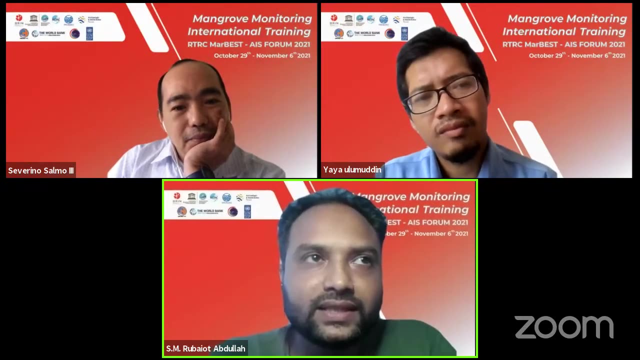 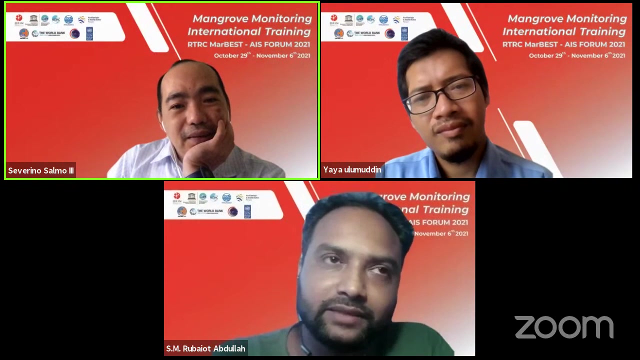 products, then you can enter, and only you can enter for tourism purpose. So I think in this paper I have some doubt actually, whether it is 22 percent or or more. I have some doubt because in Bangladesh and India the total Sundarbans is 10,000 square. 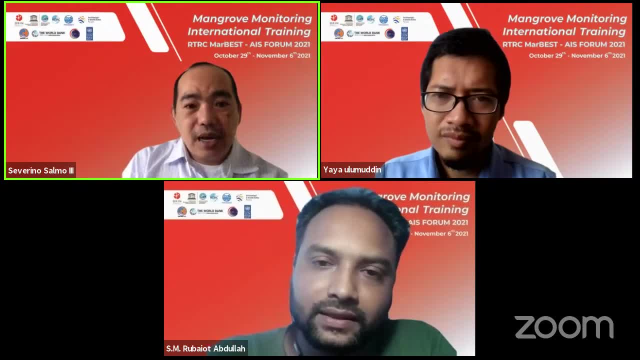 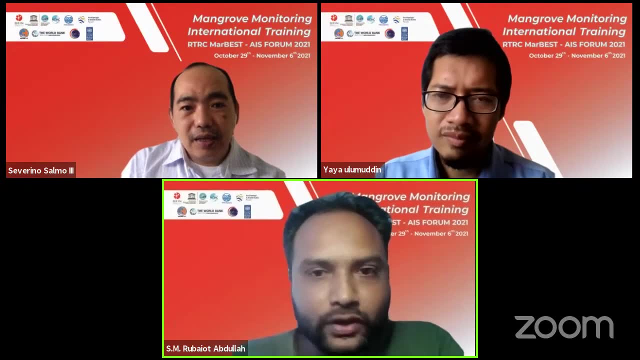 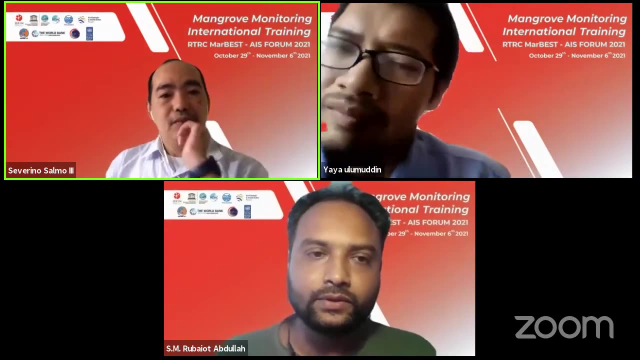 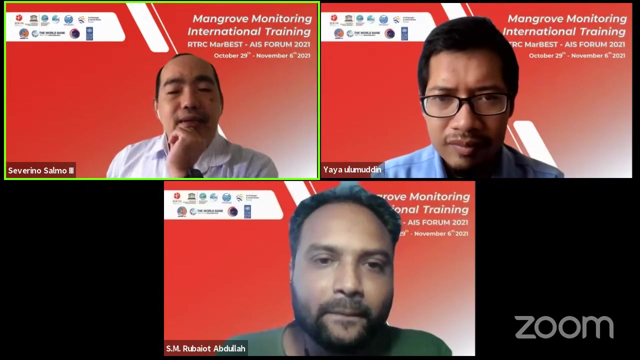 kilometers, But all the forests are reserve forest. It's more than protected forest, But still we have some protected forest and in which every activities is prohibited. So I think the total forest can be considered as a protected forest. Yes, I got your point, But I'm referring 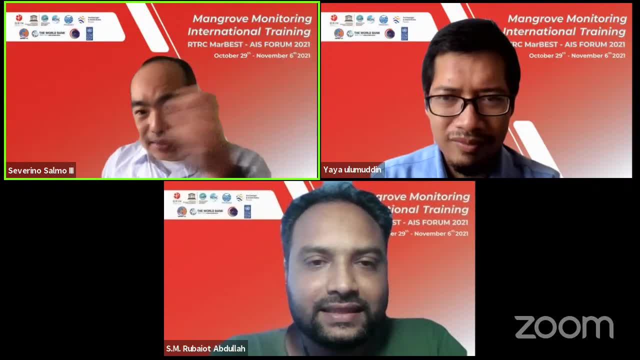 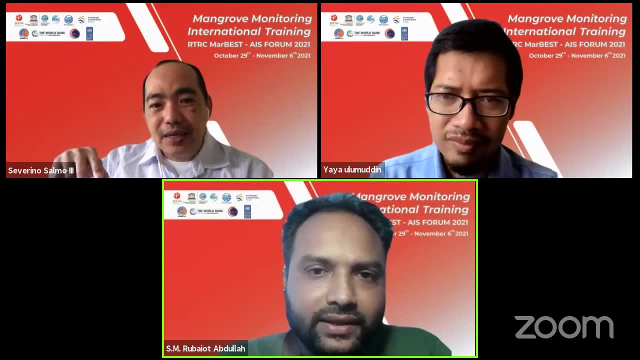 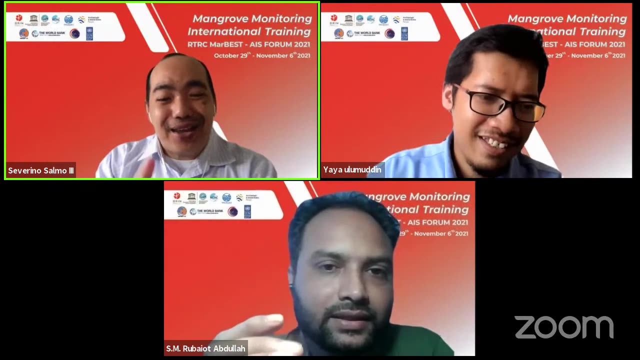 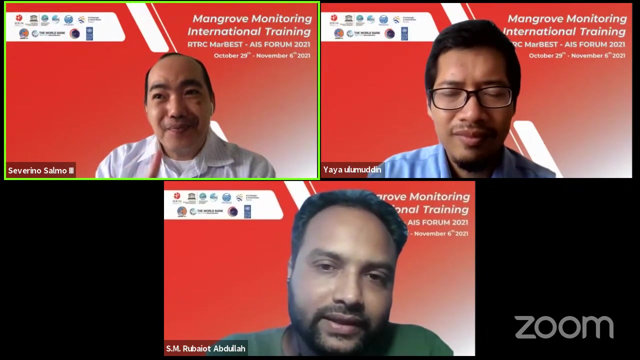 only to Southeast Asian mangrove forest, not the entire Asia. So Southeast Asia, So we are in the Southeast Asia, maybe in Bangladesh and India. Bangladesh is in, correct me guys. Southeast Asia, I know. ASEAN, Association of Southeast Asian Nation Countries, Vietnam, I see, Hold on. 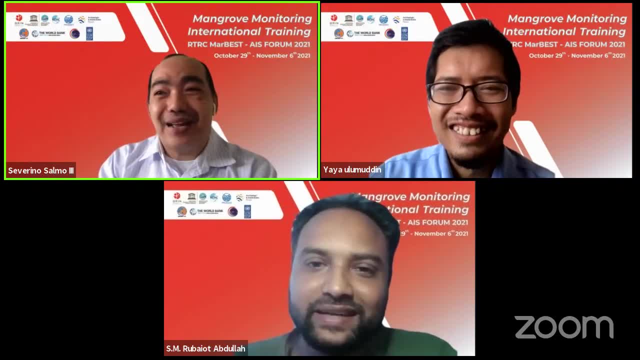 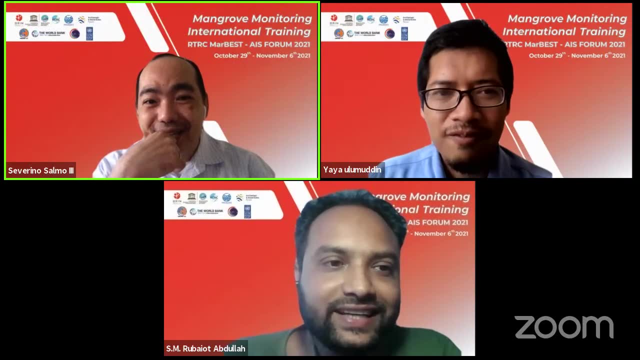 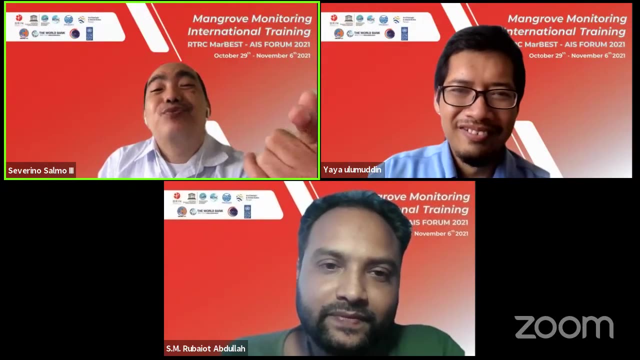 South-Western: Vietnam, Indonesia, Malaysia, Thailand. I think you are in West Asia, maybe Central Asia, Western Asia, Western Asia, yeah So Southeast Asia. people are smiling because we've been seeing it's there for quite several times already. It's about we even. 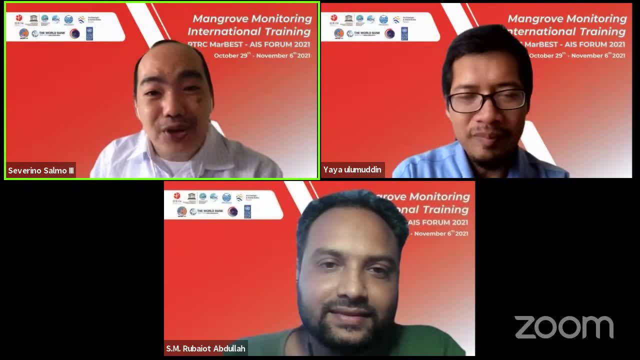 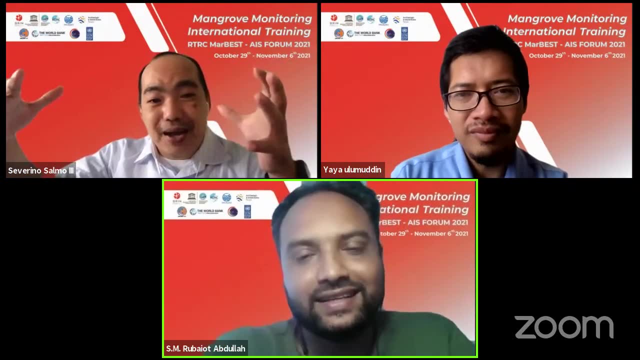 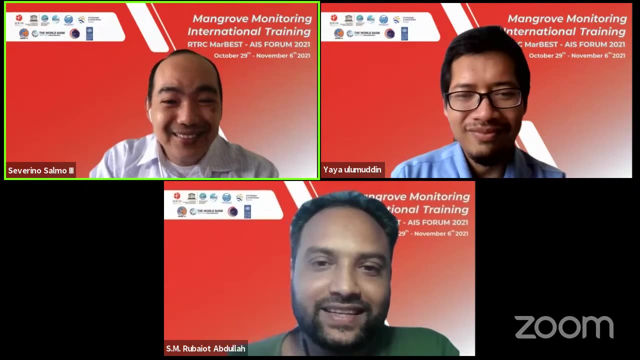 it. we have uh, a mafia, you know, malpindo aldri amir called it malpindo. malaysia, philippines, indonesia. that's because that's the center of, uh, that's the center of mangrove biodiversity. uh there, thank you, asean association, thank you, hold on. 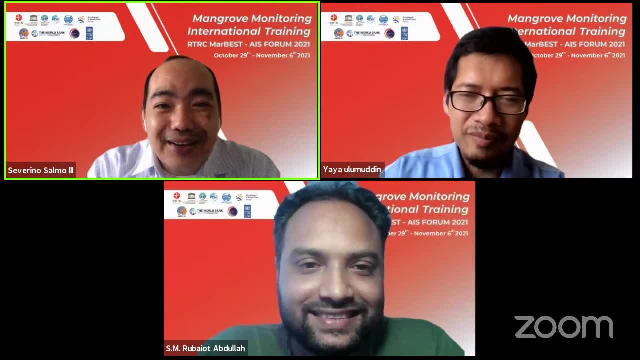 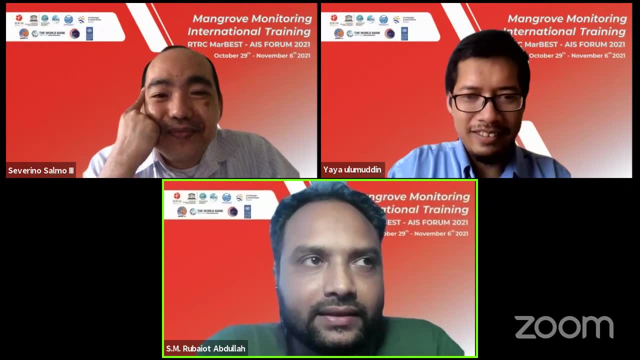 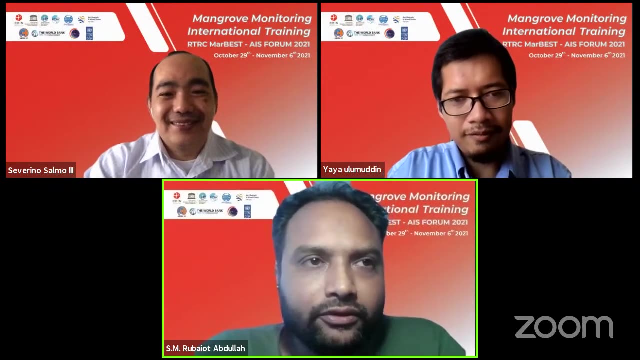 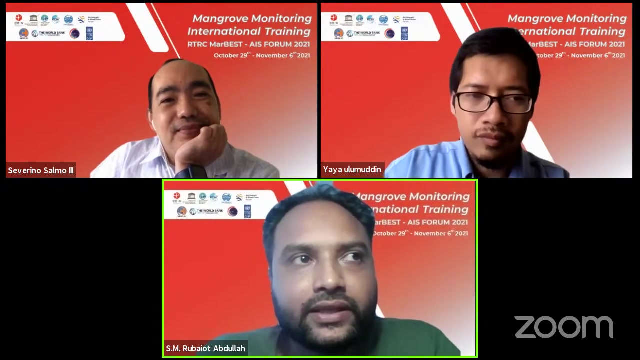 so sorry, sorry, you're not including timor. all right, that's a different topic. yeah, go ahead, abdullah. okay. so another question, uh, about the mangrove restoration. so in sundarban we have some recent change in the vegetation composition and due to the increase of salinity, 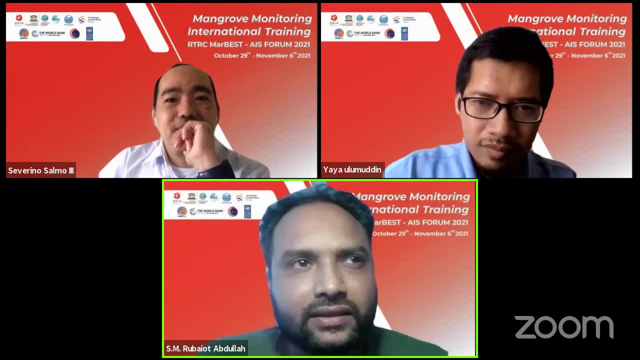 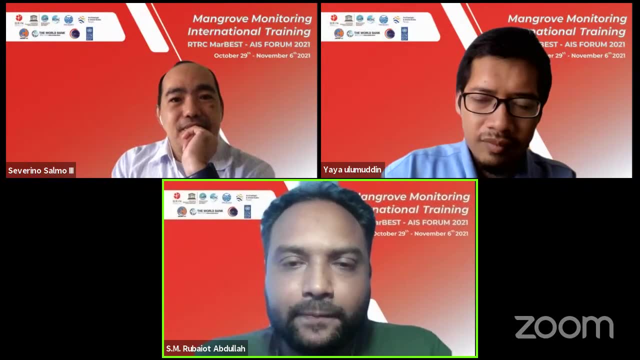 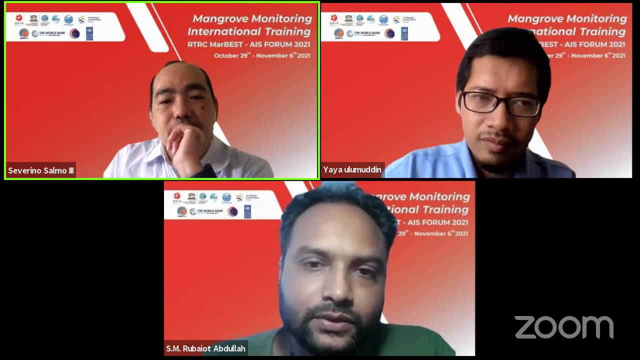 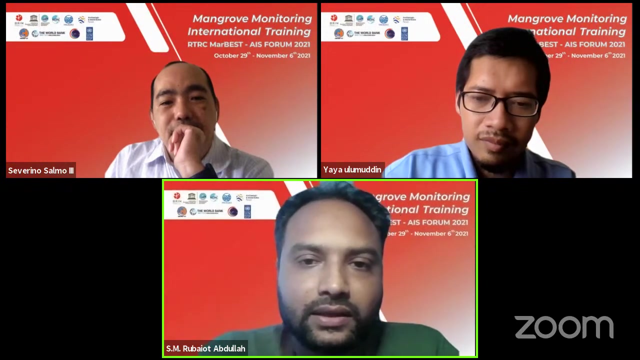 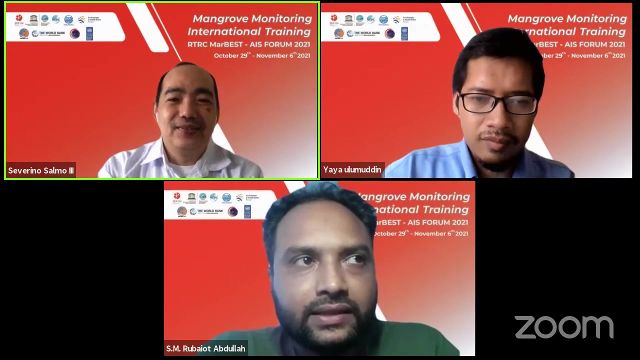 as the salinity increase due to climate change and due to upstream water flow- a decrease in upstream water flow due to faraka barrage in india. so we have some shift of vegetation composition. yeah, into the sundar bonds and in the southwestern part or the western part, we have very high increase in salinity during the recent years and 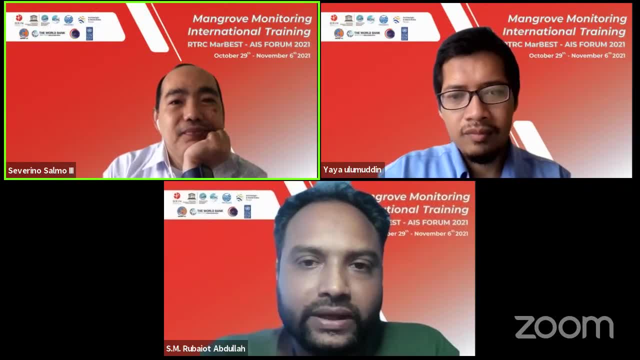 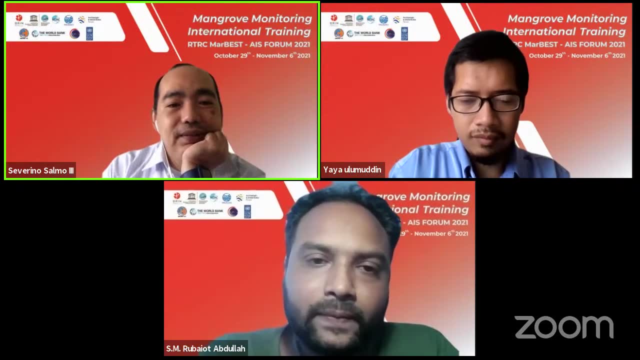 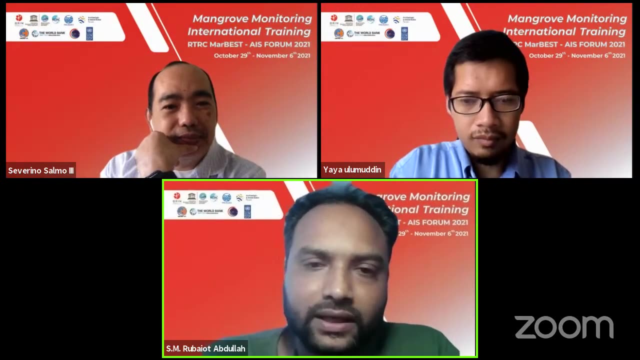 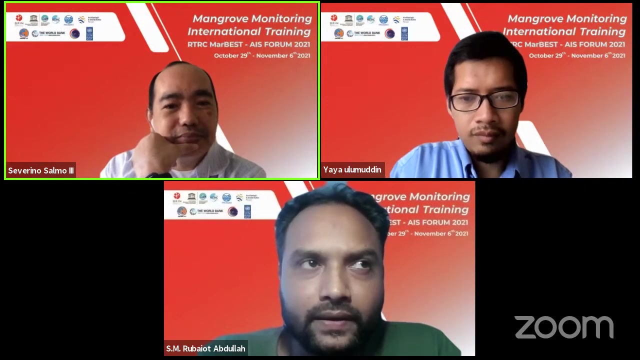 uh. second um, but the vegetation uh we have in that portion uh is syria��probikantra. yes, if you know the uh tree, yes, yes, yes, i know, i know, and in that area we observed that the vegetation is degraded. in between the vegetation we have a lot of uh. 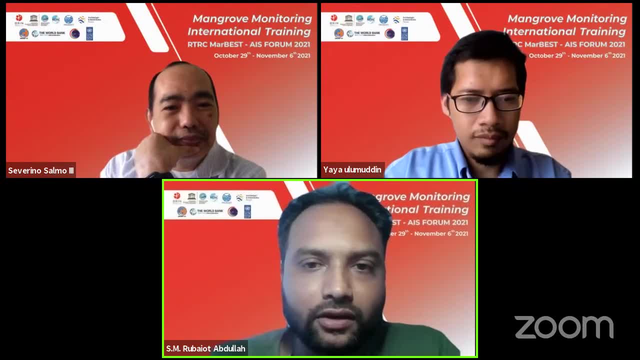 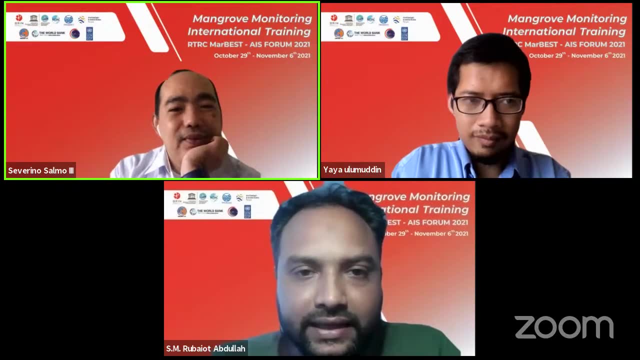 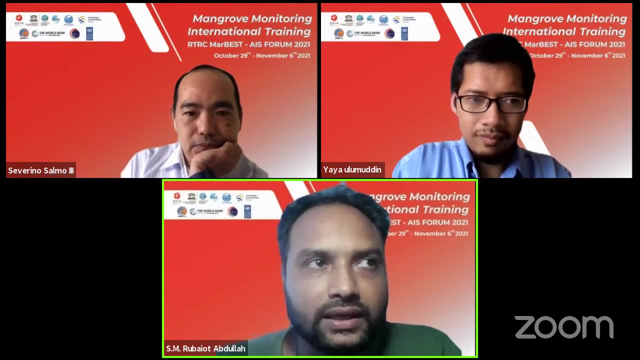 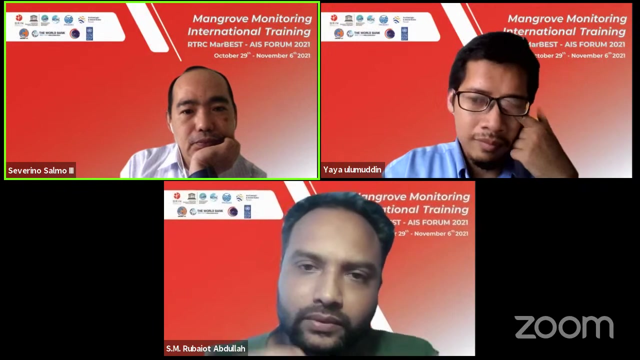 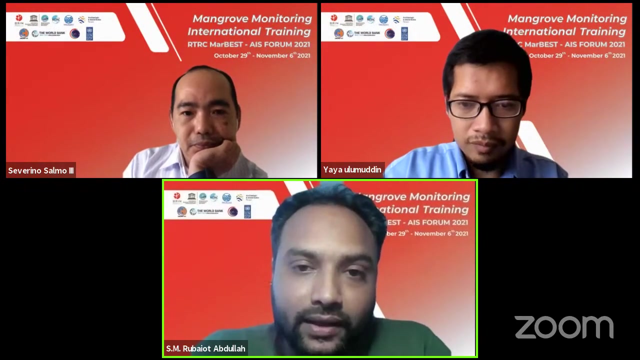 we said ncc commercial coffers, That means they are dry sandy area. The area becomes dry sandy area And there is very little amount of water or a little tidal flow during the very high tide. So how we can restore this type of area to the dry sandy soil? 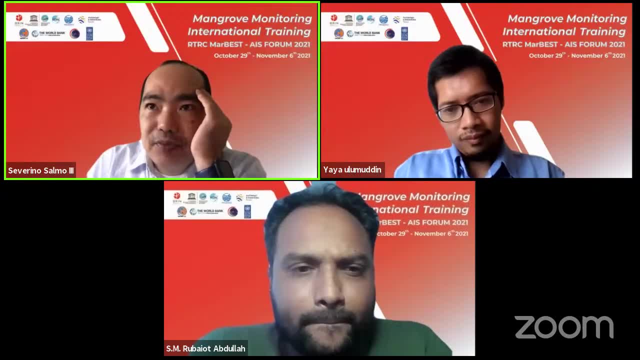 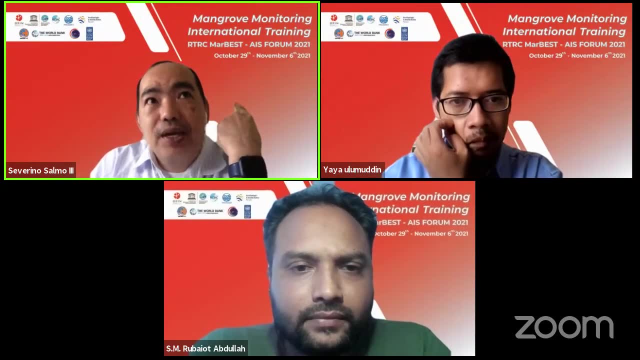 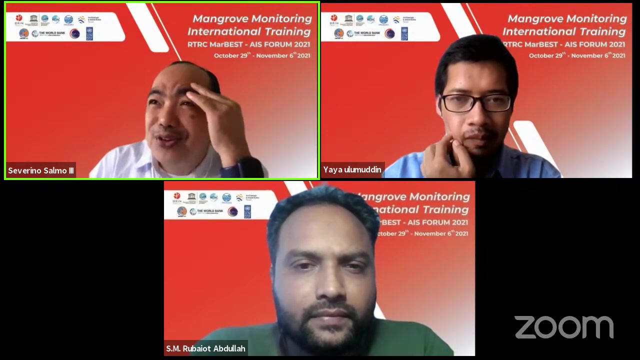 Yes, yes, That's very tricky. In restoration ecology, the immediate action is to remove the stressor or lessen the effect of the stressor. But I know that in your case- and I've been to Kenai In I forgot, maybe with Professor I forgot. 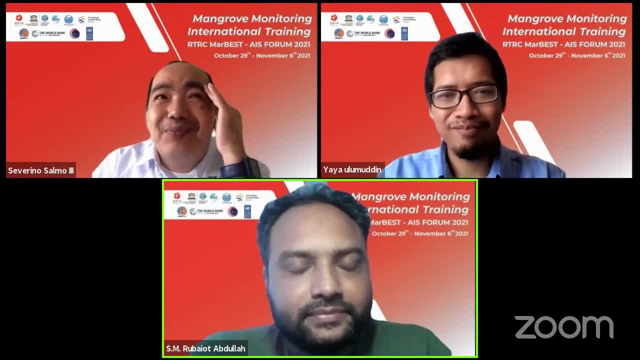 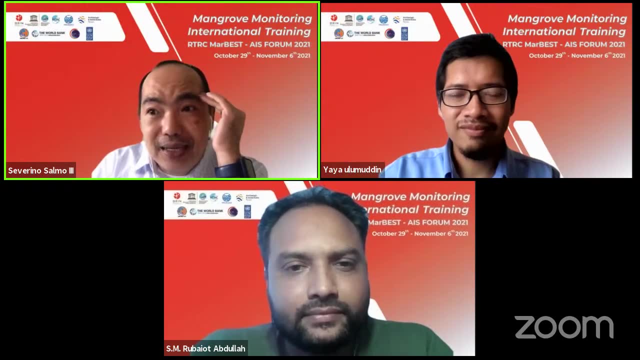 In in India, Yeah Yeah, In Annamalai University, they have similar problems with salinity, And I've never been to Bangladesh, but I can only guess that salinity is really a problem there. What's the solution? I think well. 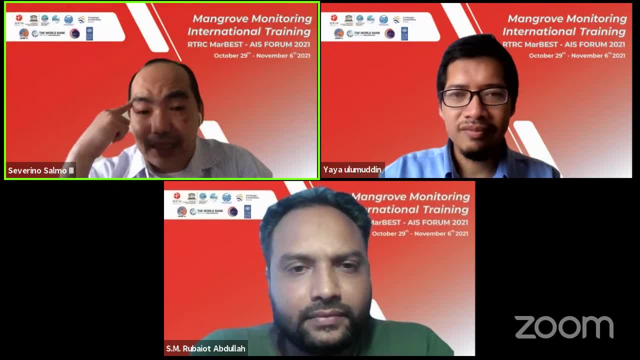 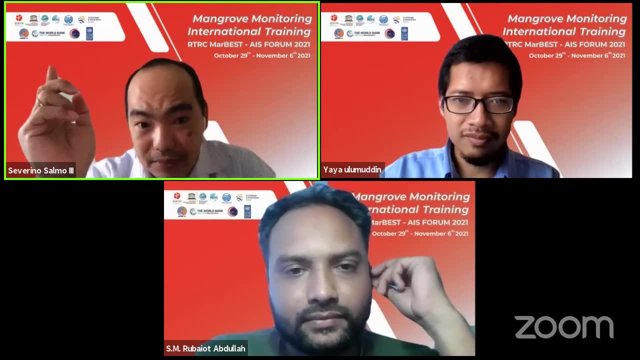 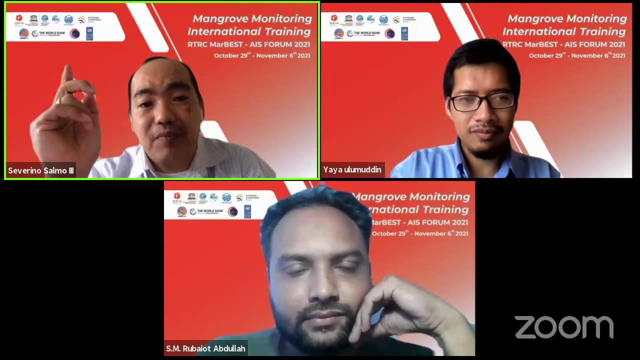 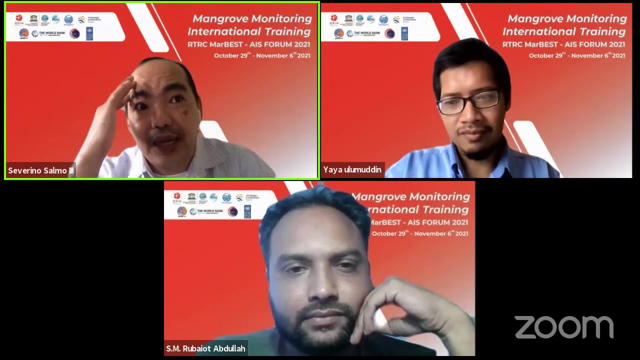 either one is to regulate the salinity by using more fresh water, that is, assuming you have enough fresh water. the other one is to plant species that are adaptive, somehow relatively adaptive to salinity, and you mentioned cereals already, i think abyssinia and to some extent even sonoratia. 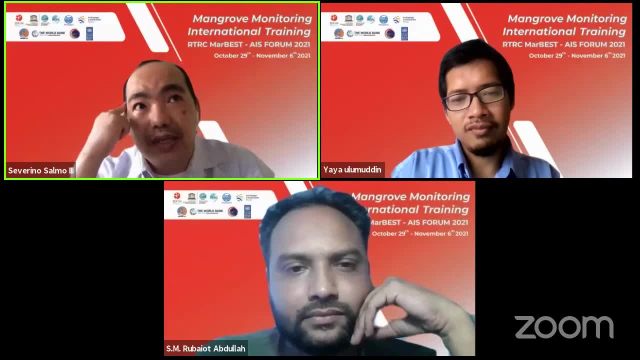 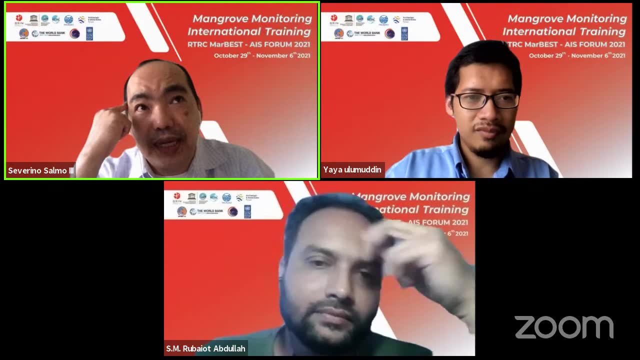 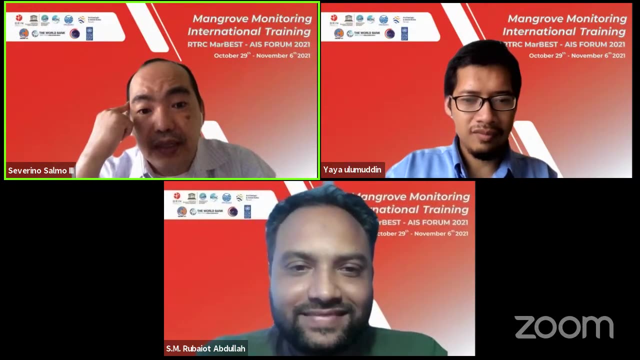 would be a good candidate, but you have to follow certain rules about species succession. but, uh, my, my answer is that you have to assess the extent of the of the salinity disturbance first, and it's not easy, uh, abdullah, uh, if you go, if you go in in middle eastern countries, uh, i think. 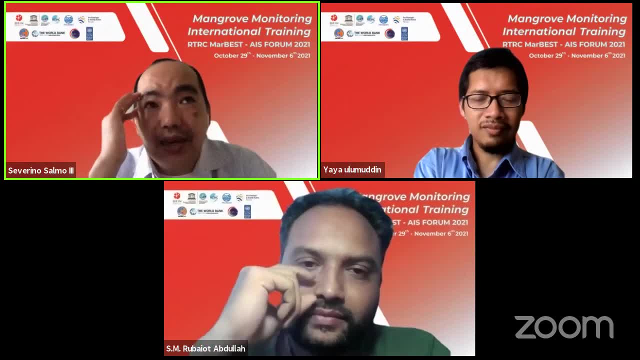 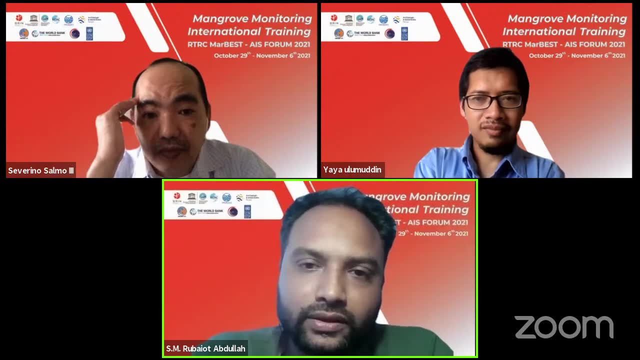 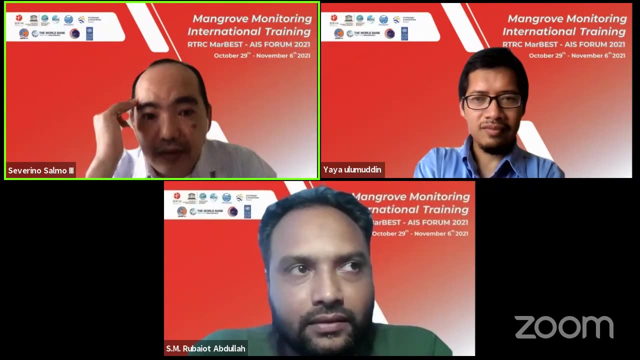 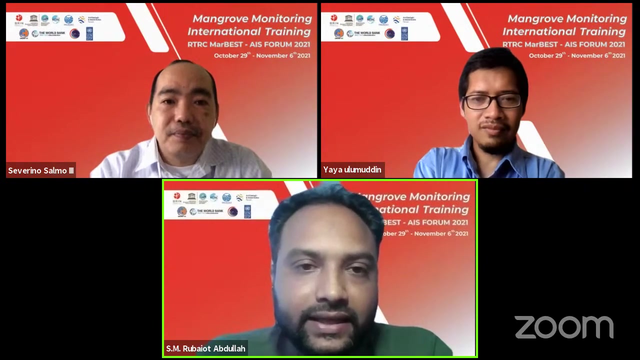 someone's from barina. you, you have your high salinity. obviously your species composition will definitely change. actually, the area is not uh something like uh any other species can grow. yeah, that means the sonoratia or the abyssinia. it is very difficult to grow in this dry, sandy area because they are pioneer and they can grow uh along the river side. 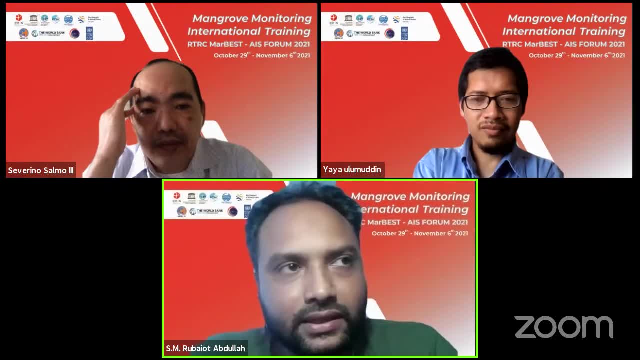 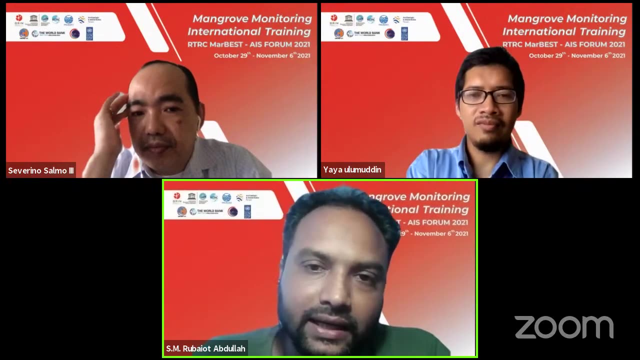 yeah, but in that area it is very difficult uh. but we have some uh other species uh: gylocarpus molucansis and gylocarpus granatum. this type of species can grow or can withstand very high salinity. yes, i agree uh, we uh had this uh tree species. 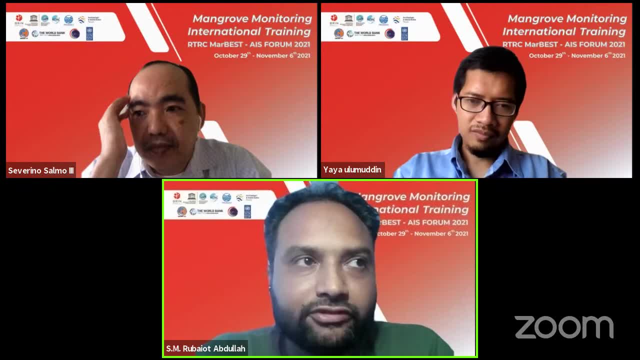 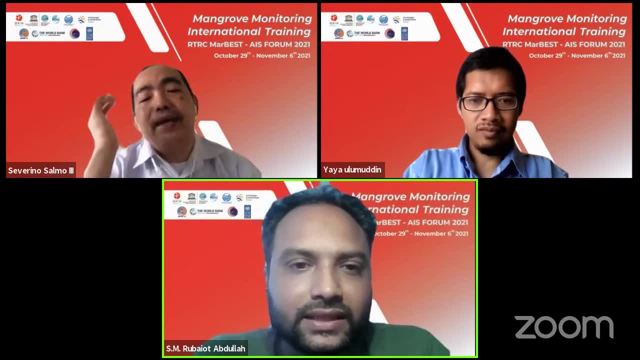 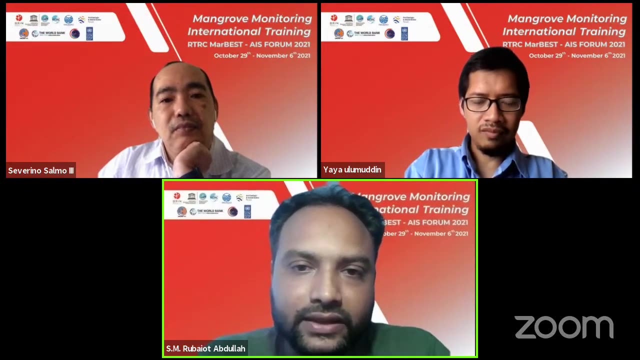 in that region, but the wood is very valuable. as the wood is very valuable, uh, local people illegally cut uh, yeah, yeah, that's a problem and uh, it is very difficult to uh implement assisted natural regeneration. uh, in that area for that species- and this, that is species- is also a climax spaces. 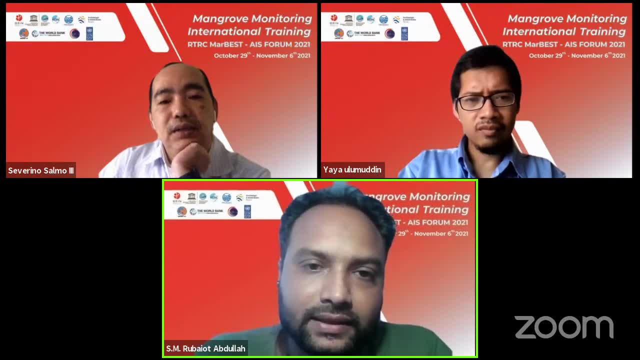 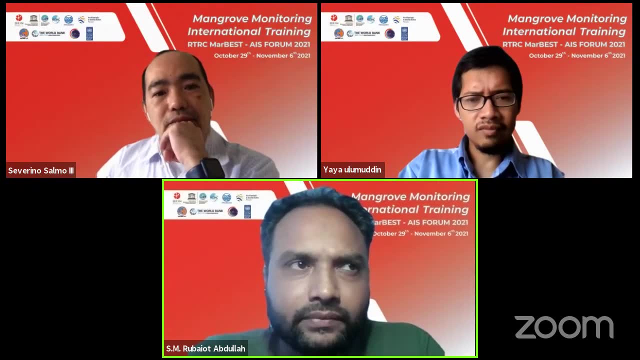 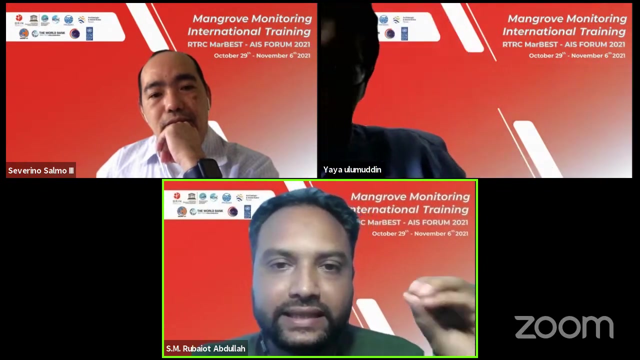 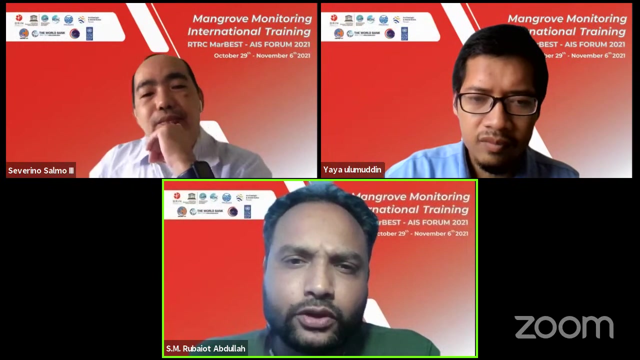 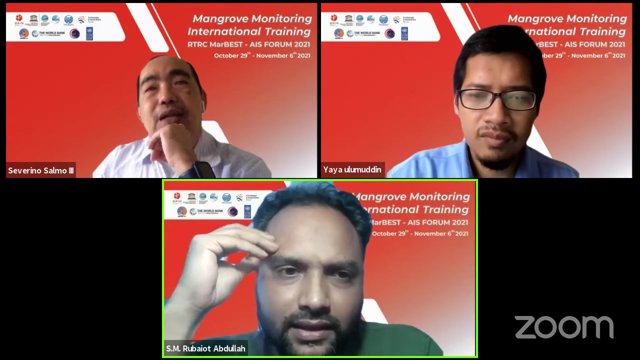 but we don't have enough, uh, these species. so, uh, should we intervene? uh, some other species, uh, or the gylocarpus emollucansis or gylocarpus granatum from other area of the sundarbans. if we, If we're seeding this area with the seed of this species or any type of intervention, do you think any intervention in natural forest is wise in restoration? 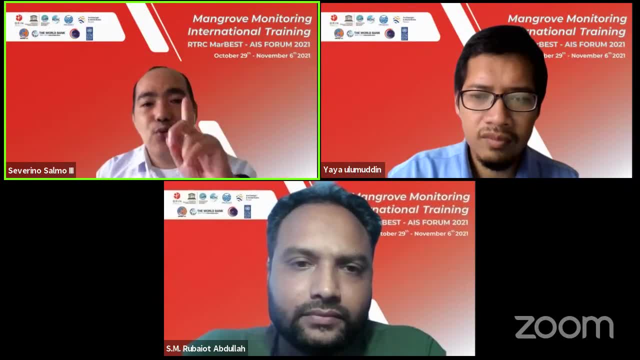 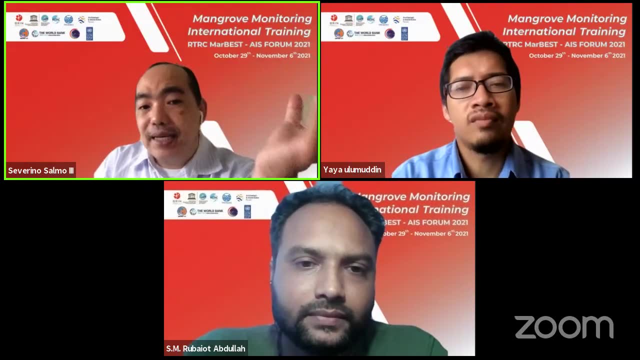 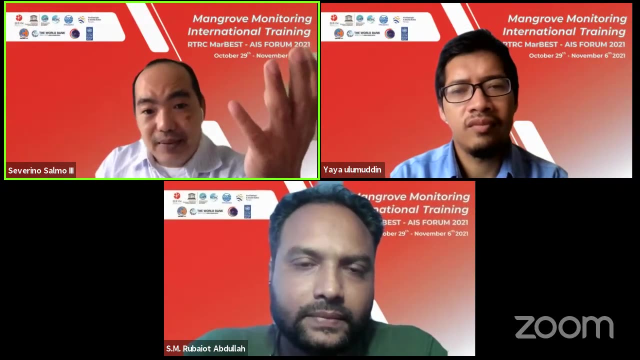 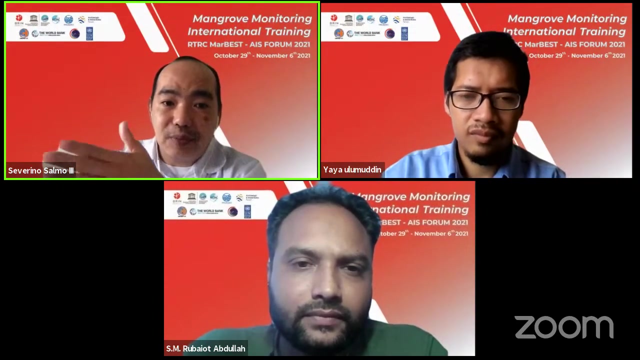 I have two contradicting answers. One, first, if you know that the site is really a former mangrove area, the natural mangroves, then I think it will be good enough to maintain the conservation status. Now, my other contradicting answer is that to address the threat, that of the salinity, and you can do proactive restoration, but you have to be very deliberate on the species selection. 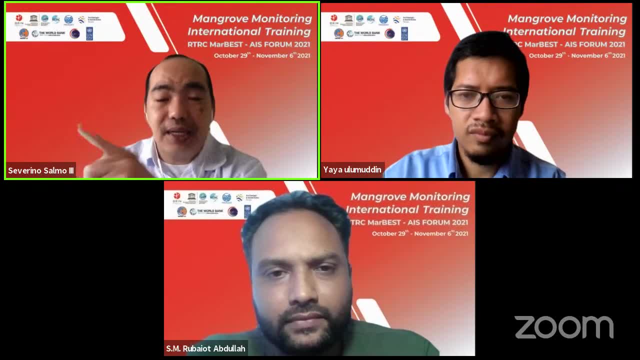 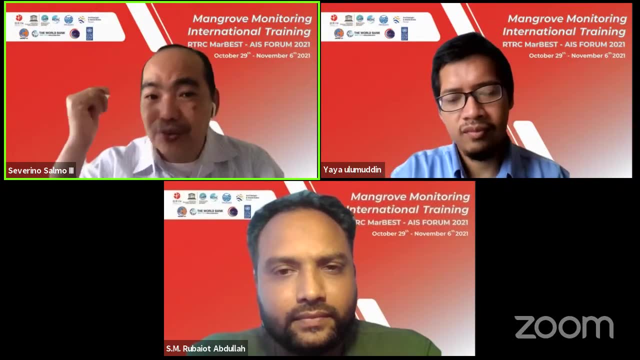 And things that you mentioned that are adaptive to salinity. There's an issue with the silocarpus, etc. But I love mangroves. I will do mangrove ecology, mangrove restoration, But I think you have salt marsh in Bangladesh. We have some salt marsh Now. if mangroves will have a very difficult time to establish, salt marsh is an equally important ecosystem, Right, So why not again? my premise is that I love my mangroves and I would do anything to conserve my mangroves, but salt marsh is not bad. 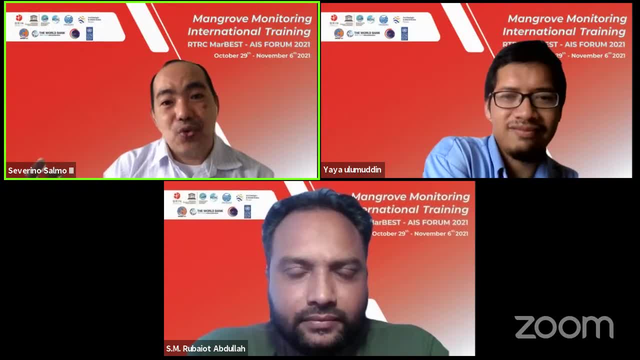 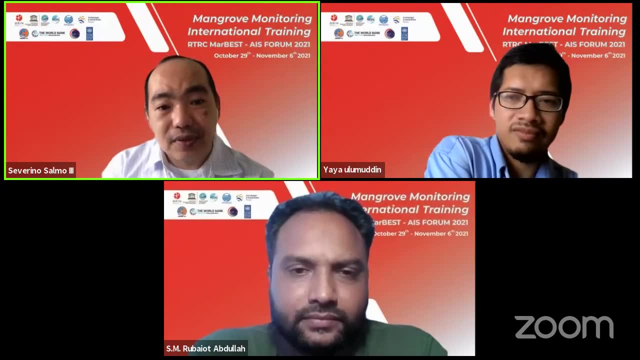 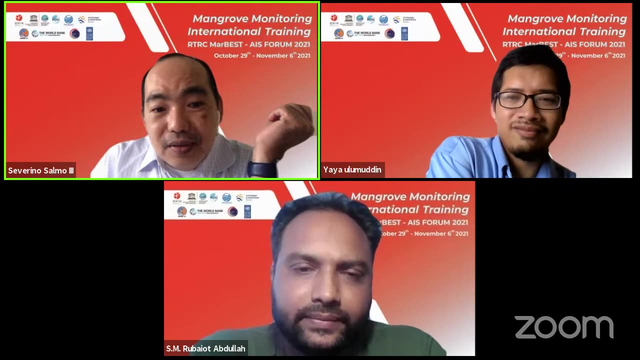 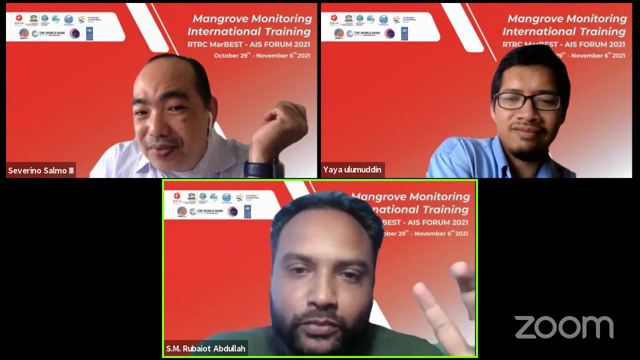 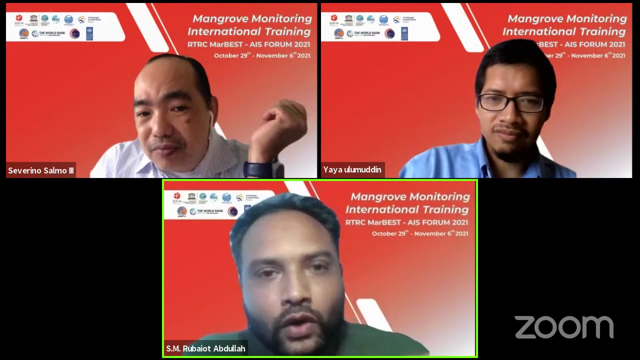 It's an equally important ecosystem. Why not invest some time with the salt marsh restoration? Well and good if you can do both, Okay. But in our country we have some, actually two, schools of thought. actually, some researchers think that in mangrove, no other species other than mangrove should be planted in the mangrove area. 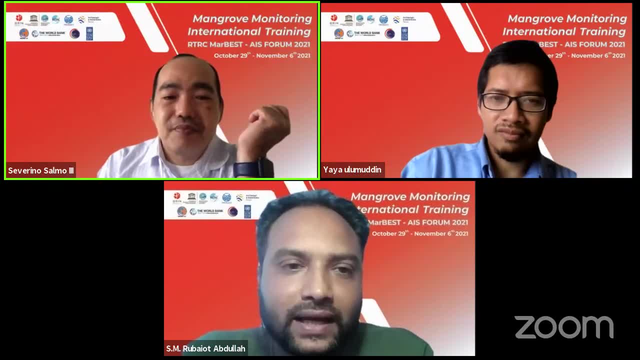 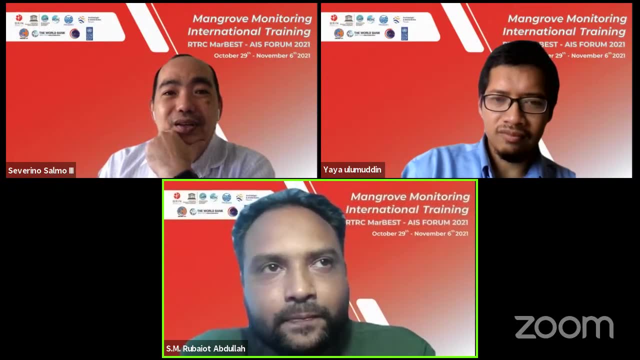 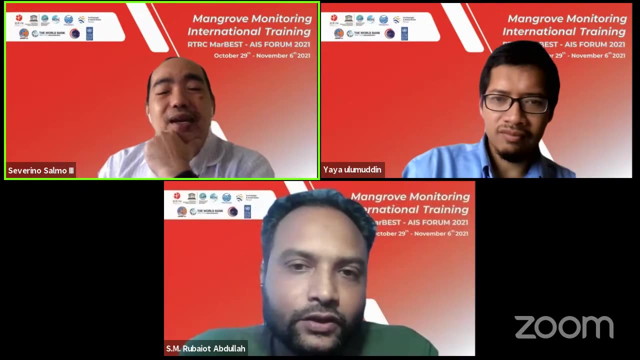 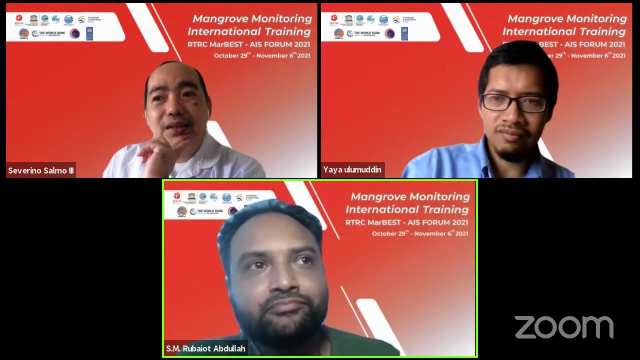 And some researchers want to plant some terrestrial species inside the mangrove, In which there is Maybe no salinity or no tidal water input. So there is some controversy actually among the researchers. some want other terrestrial species to plant in that area. 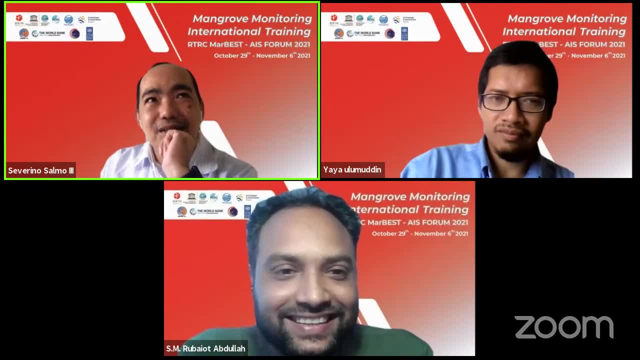 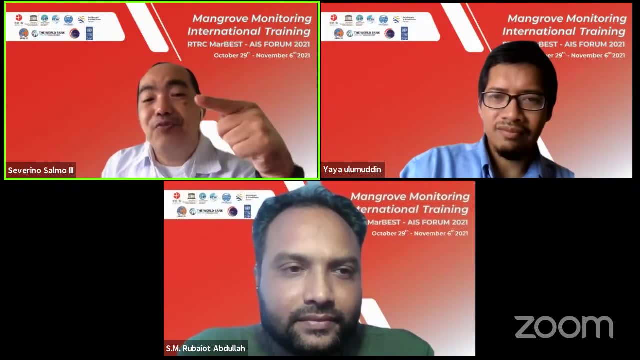 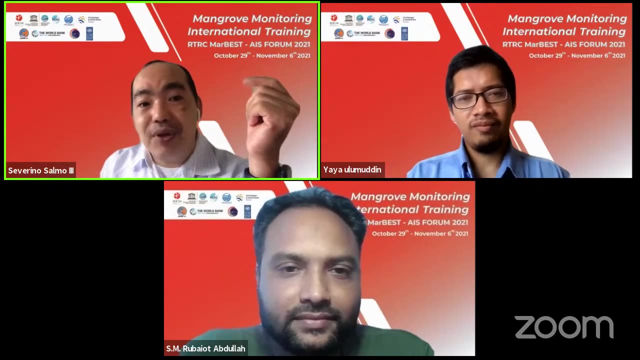 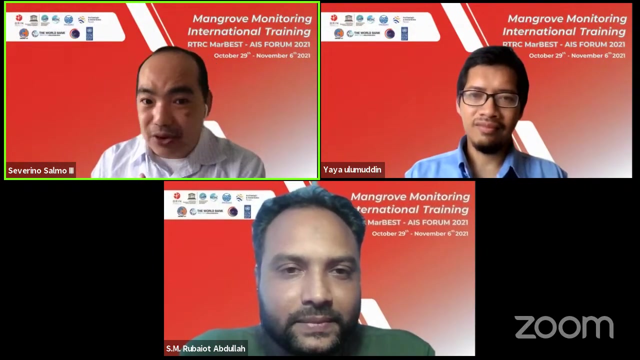 That's a very interesting discussion and unfortunately I don't have much experience in Bangladesh. I only mentioned salt marsh, But if your foresters are, If they are confident enough with planting terrestrial species, if they have the basis, then I will go for it rather than you know mangroves. mangroves will not survive without seagrass and coral reef. 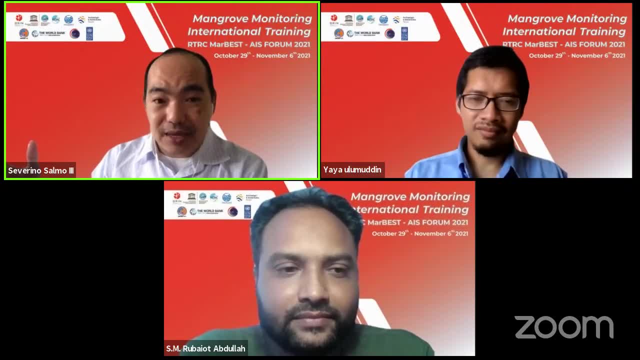 There's this interconnectivity connection among ecosystems, The same way that your mangroves in Bangladesh is related to the salt marsh and the forest species. Okay, So, while we love mangroves, we do recognize that mangroves, Mangroves alone, will not be sufficient enough. 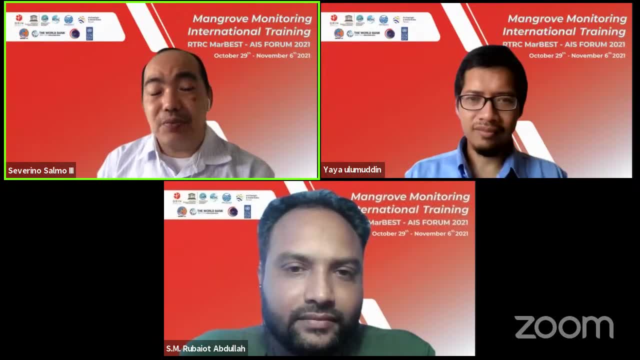 It has to be complemented with other restoration programs, And I think in your case conservation is also not enough anymore. You have to complement that with other restoration programs. And then we have the debate now on how to do restoration, And I mentioned about the salt marsh. 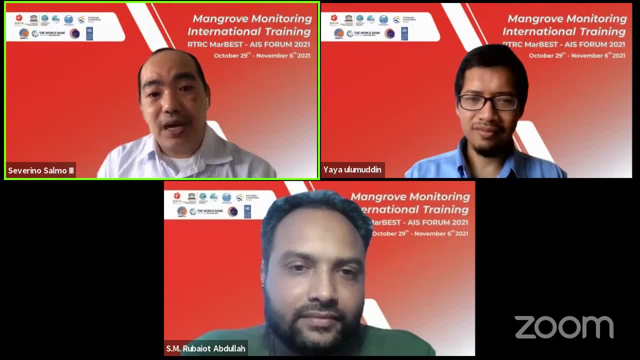 Maybe the forester people in Bangladesh have a good basis for suggesting that they introduce Terrestrial species. I never encountered that. in the Philippines We have a different case. I don't know if Indonesia tried that- planting terrestrial species in mangroves. 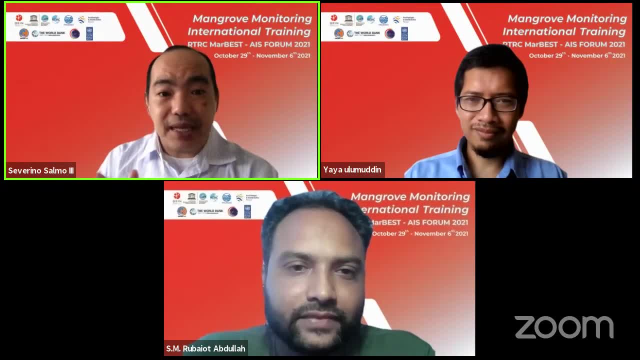 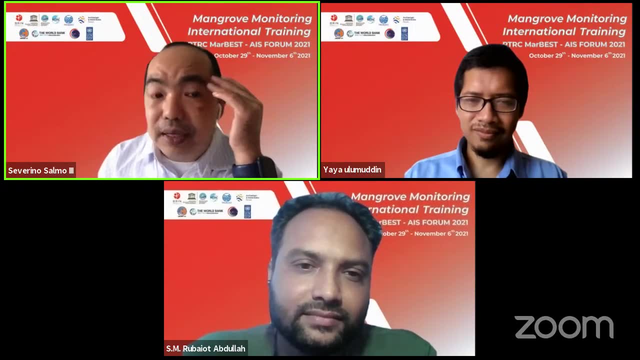 Maybe Indonesia doesn't need it for now, But I think Bangladesh. I will agree definitely with you, Abdullah, that there's really a need for restoration, But I don't know. I'm candid with you That controversy is a good scientific debate. 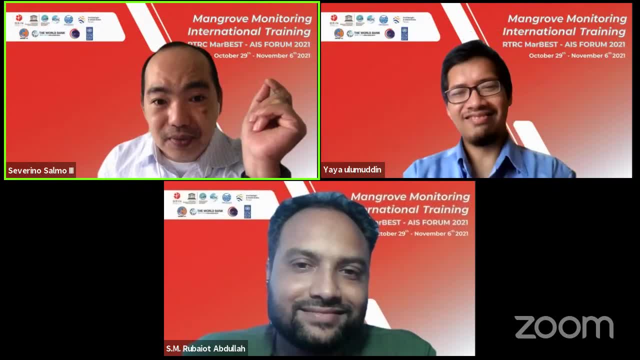 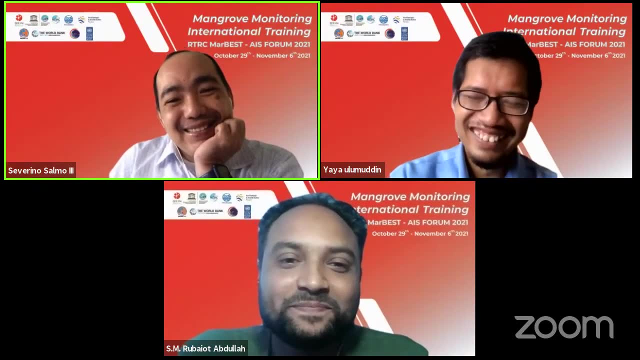 But I don't have straightforward. I don't have a straightforward answer for now. Okay, last question. Sure, I'm taking much time, That's okay. So the last question In mangrove. I have several visits in mangrove, in Sundarbong. 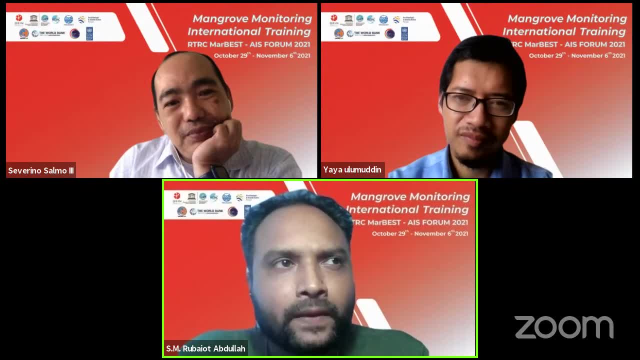 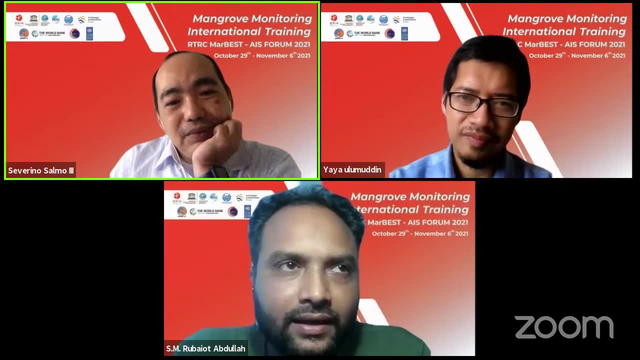 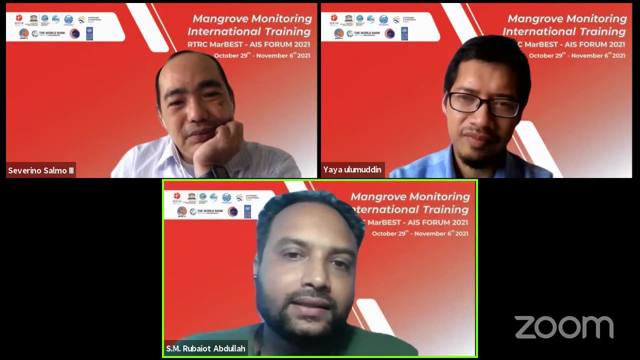 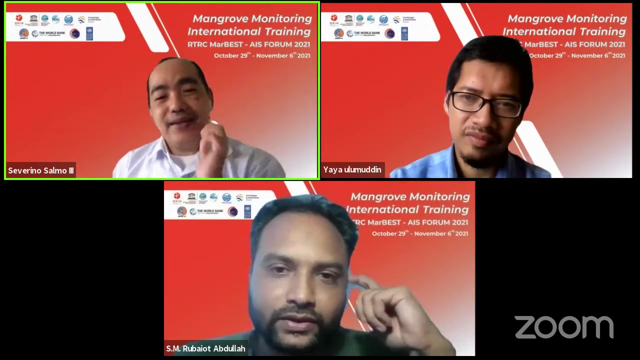 But I observed Several sites have the mollusks, the crabs, And they are very abundant, But with the more healthier situation or more healthy composition, I did not find any mollusks or any crabs there. So some area we have a huge number profuse or a huge number of mollusks and crabs. 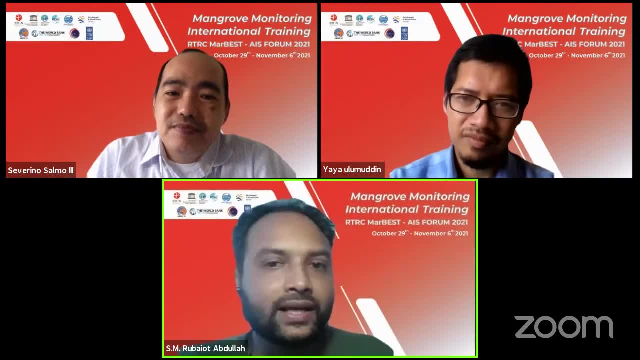 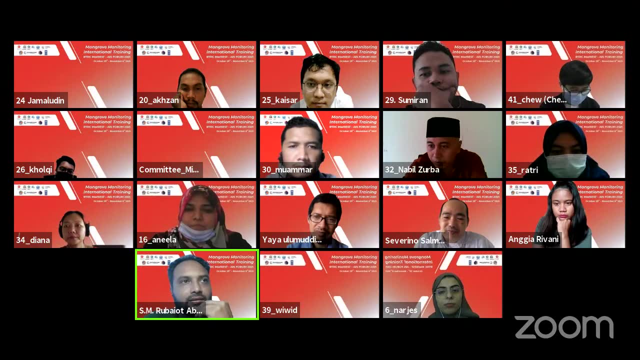 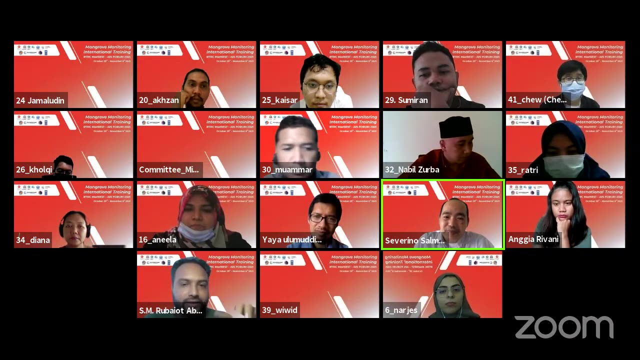 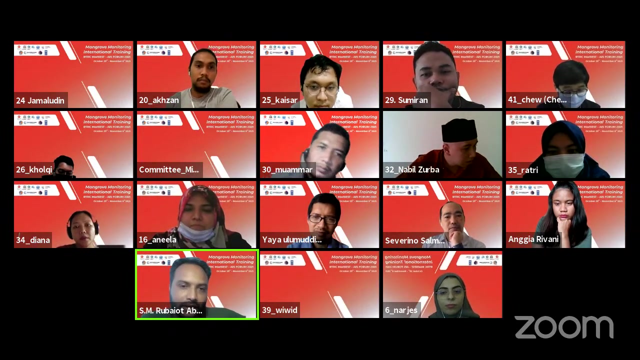 And they borrow the soil and make some- How can I say, Make some small, teeny, hill-like structure? Yeah, it's a mound, A mound, yeah, exactly the mound. And lots of seed stack in the mound And there is profuse regeneration. 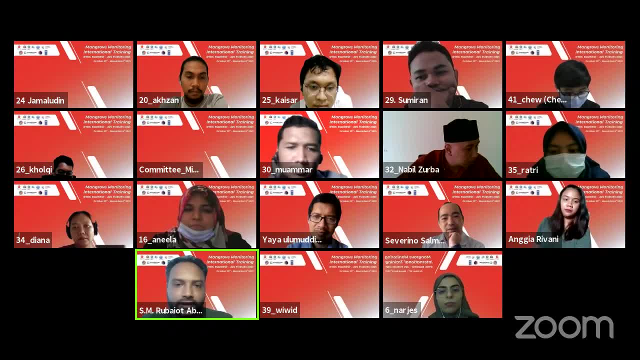 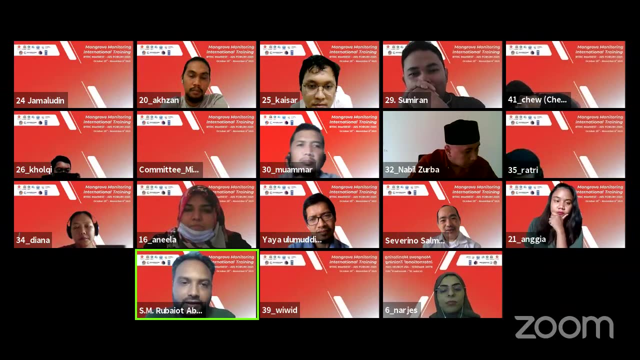 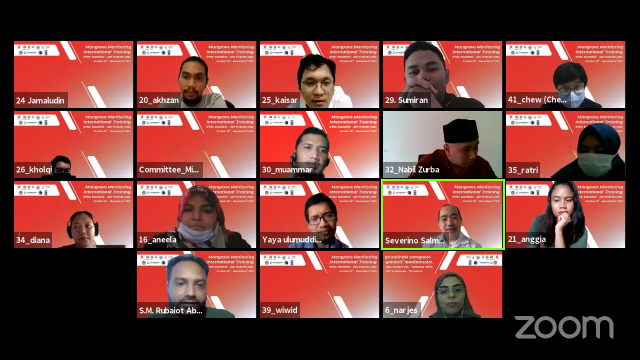 But some other area. they are very good in health, But here we cannot find any Mollusks or crabs, Yeah, yeah. So how can we correlate the indicators of mangrove health with crabs or mollusks in our situation? 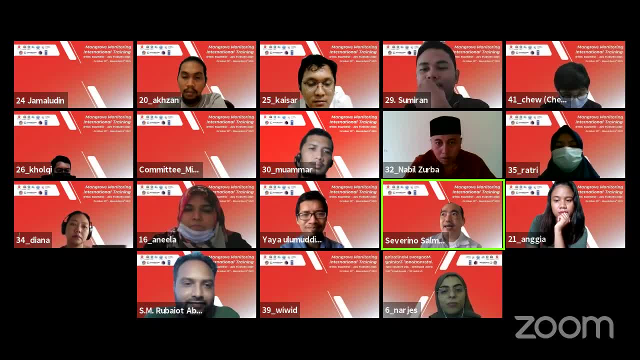 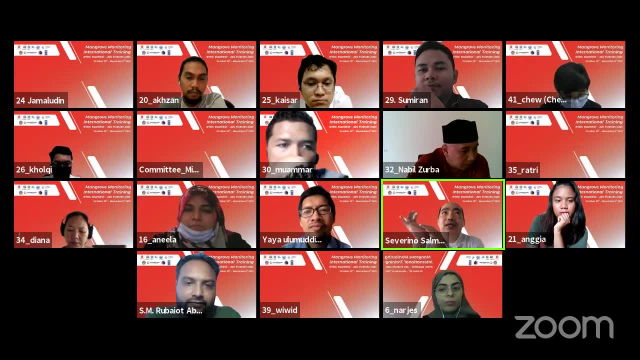 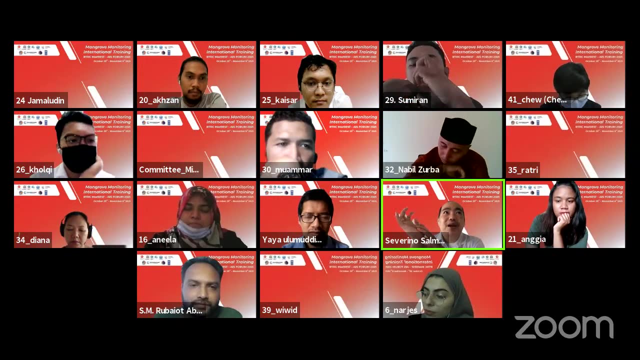 Yeah, yeah, That's a very good question And I think I also encountered that. Let me cite you an example Down south here in the Philippines. yeah, it's almost similar to what you mentioned: Very healthy mangroves, no disturbances, but no crabs. 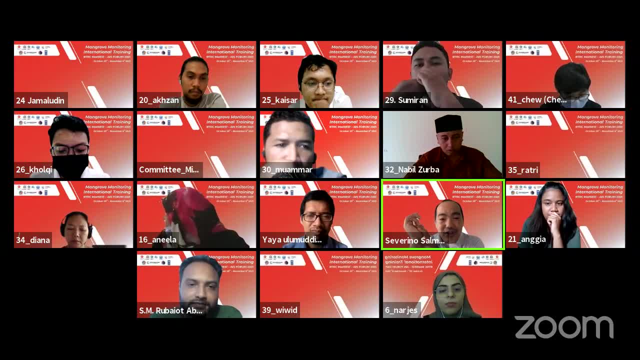 I think that's what you mean, right? Yeah, Although the mangroves are healthy, but there are no crabs, right? There are several reasons. One could be seasonality And the other one is that. But mollusk is quite consistent with the healthy mangroves. 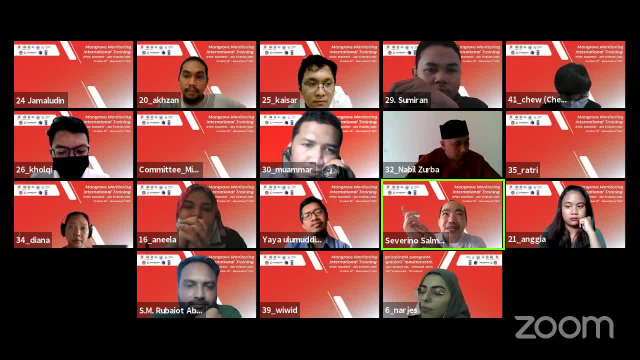 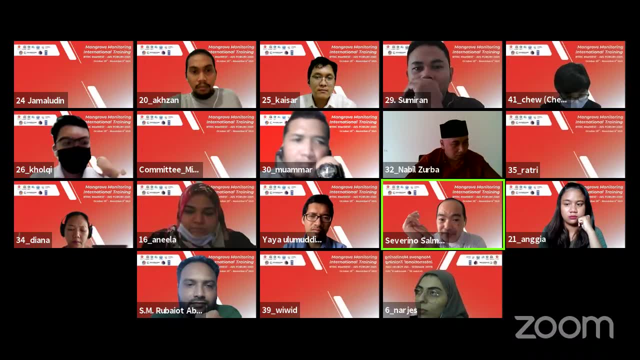 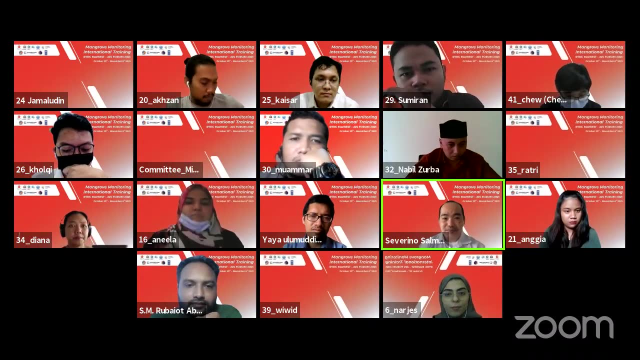 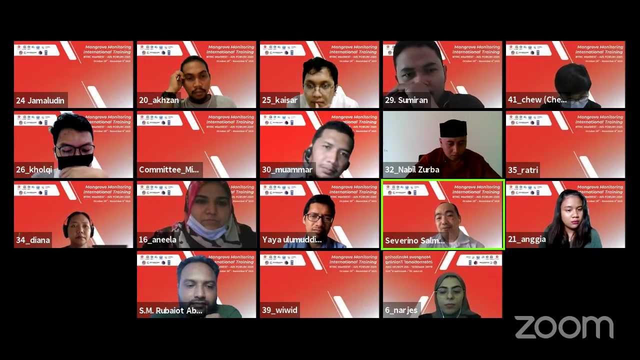 But let me go back to crabs. Even though your mangroves are healthy, there are cases wherein there are things that are not visible for us, Like when we collected the sediment samples- the one-meter sediment samples- we never know. Only then that we realized, and then people mentioned to us, that it was a former mining area. 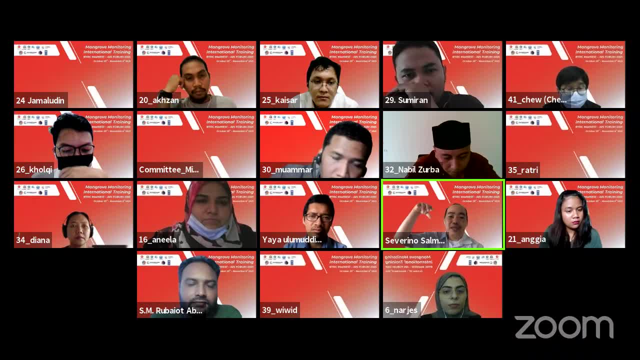 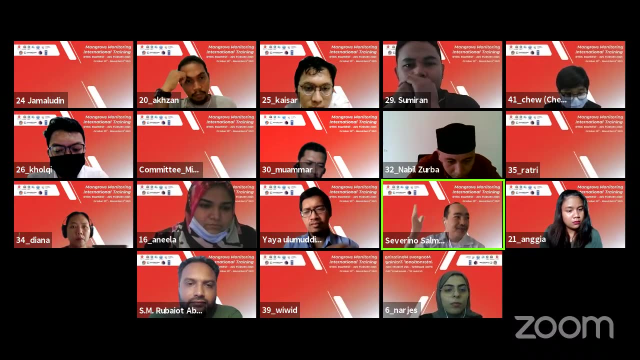 So, true enough, when we collected the one-meter depth samples at the bottom It's like colored orange yellowish. We didn't know that it was a former mining area. Now you know, the mining effluents are made up of zinc, cadmium, heavy metals. 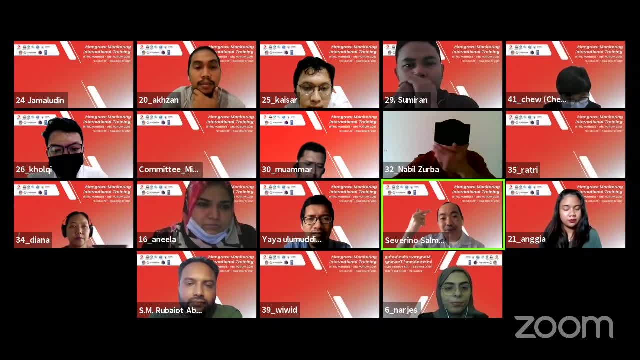 And obviously your animals will not like that. And if you don't know those things, if you don't know the history of the site- just like what we did when we went to that site- then you will conclude that, Ah, mangroves are healthy, but no animals, no biodiversity. 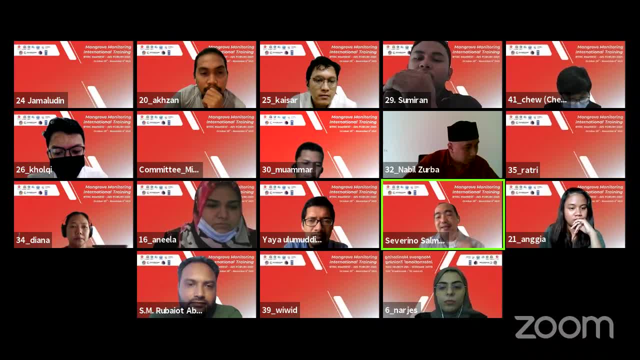 When, in fact, there are several factors that could affect them, And that's the reason why you really need to do a consistent monitoring, Consistent monitoring plants, monitoring plants, and very frequent. Again, if you have the resources, it should be more than one per year if possible. 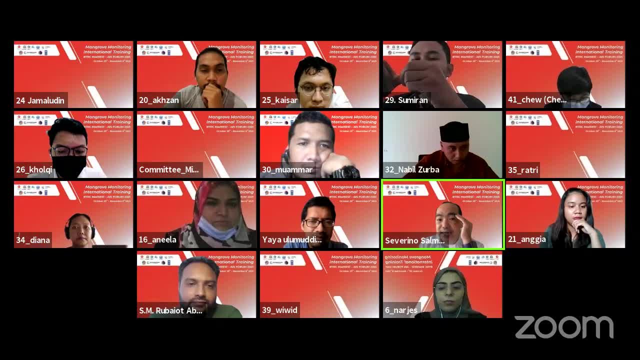 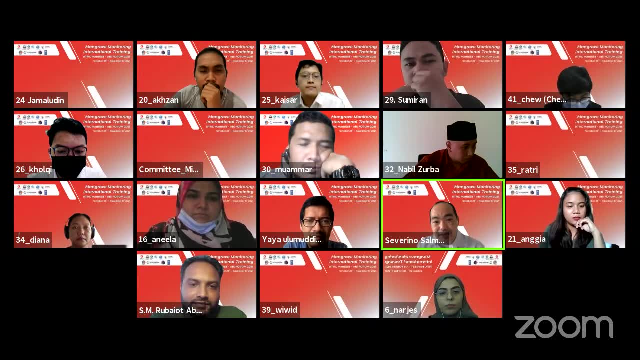 But yeah, I agree with you. It's really possible that you You will not see animals And it will be very interesting to observe the diet of the animals that you will observe there. Maybe that will tell us something About the species. 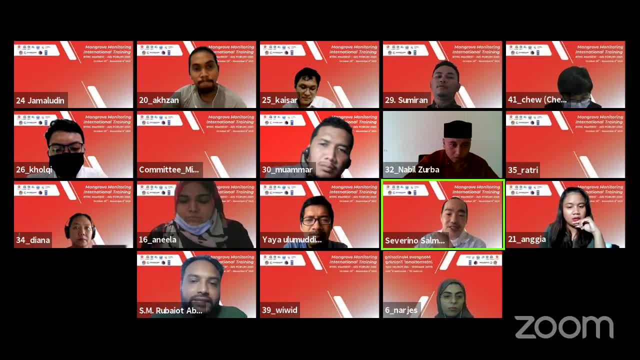 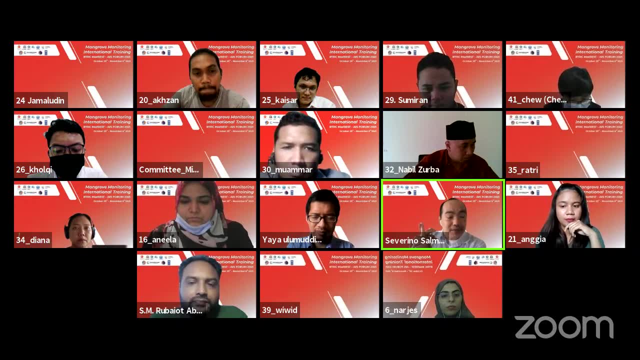 No, the diet, The food that is ingested in the stomach of the animals. If it's very low in organic matter, it means that there are very few available food in the mango And there are some groups. Okay, It can be. 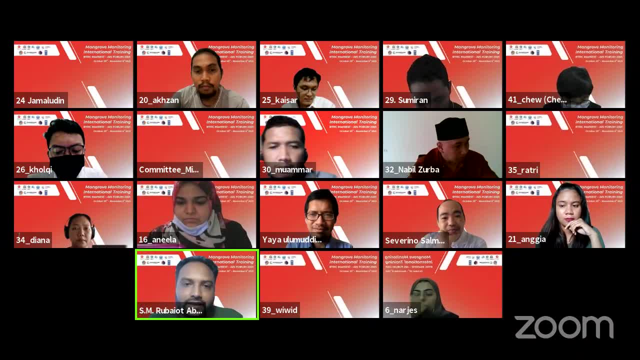 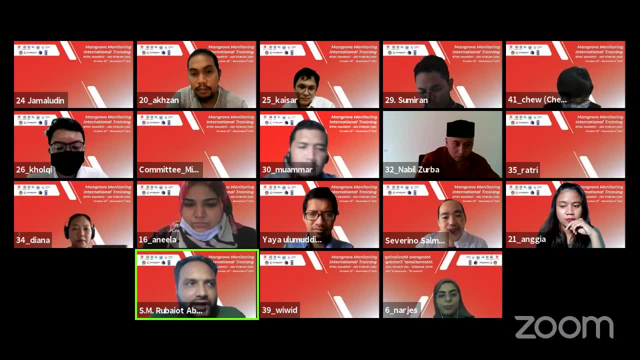 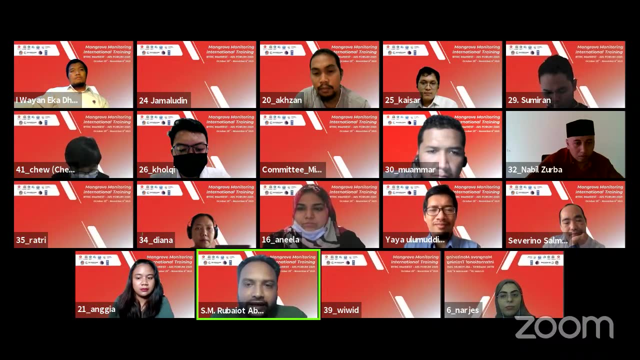 It can be. Yeah, yeah, It's possible. So there are lots of vegetation composition in our area. So in some areas if there is a sundry and the leaves are very tough and very fibrous, so maybe the vegetation composition can be one of the reasons that in the vegetation composition, 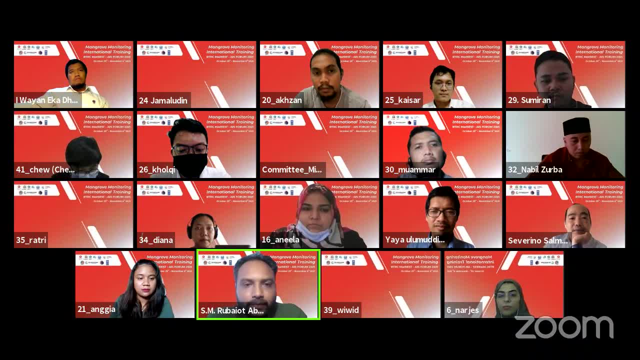 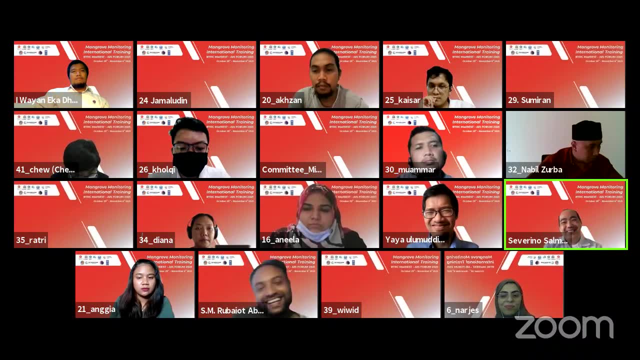 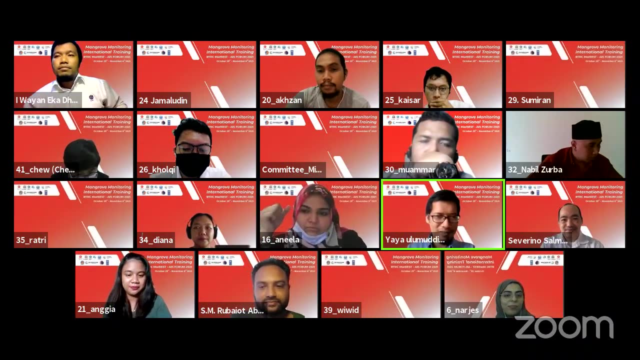 we cannot find animals, Yeah, and salinity- Salinity will really matter. even so, we have to. you have to measure salinity. yeah, okay, so thank you, thank you all right. all right, so maybe this is, yeah, the last questions. maybe, angia, please, sorry for asking again. 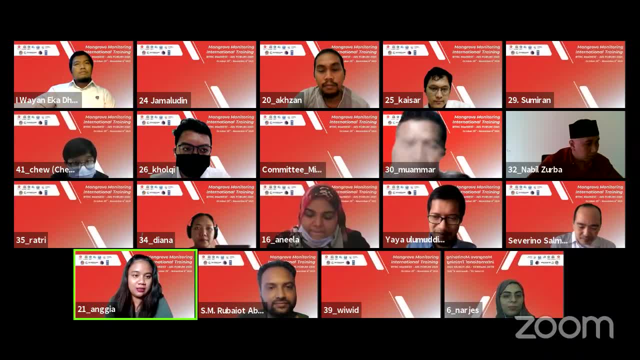 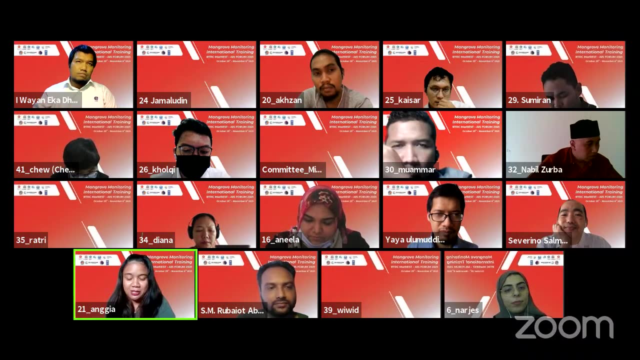 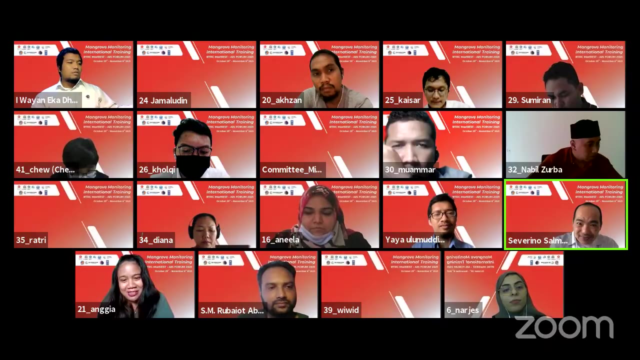 i don't know, it's a unique or usual thing that happened in mangrove ecosystem. in the other area in here there are so many small malus eat the leaves of mangrove, so the leaf of mangrove have so many holes. what do you think about that? because you mentioned earlier, because 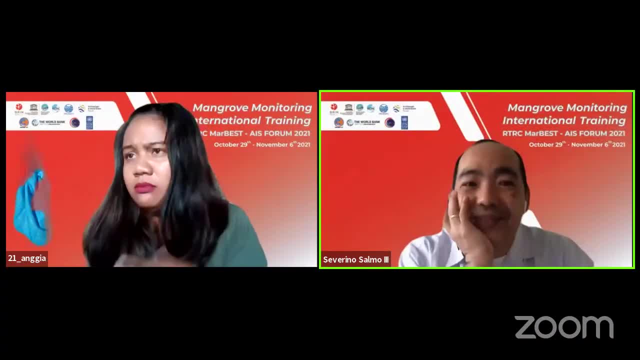 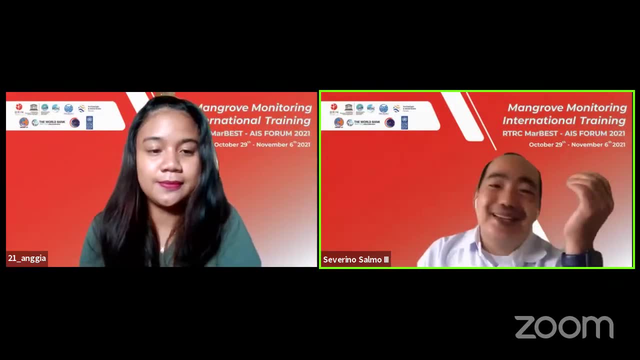 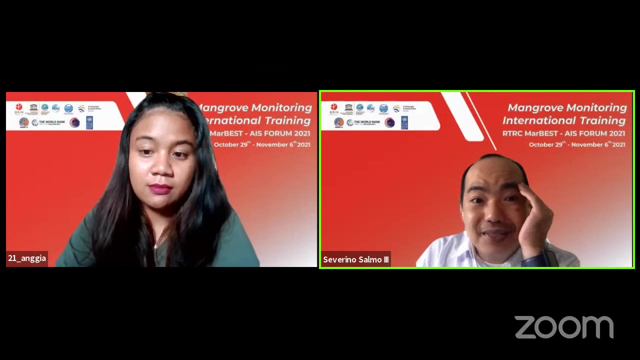 the malus is one of the indicator indicator of mangrove health. yeah, thank you. yeah, yeah, uh, it's thank you for asking that. um, i love molus, uh, when i see leaves that are being eaten by by molus right there, and then i can say that mangroves are providing habitat and food to various animals, especially. yeah, 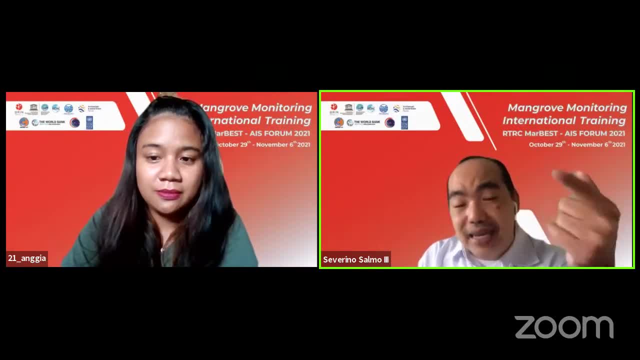 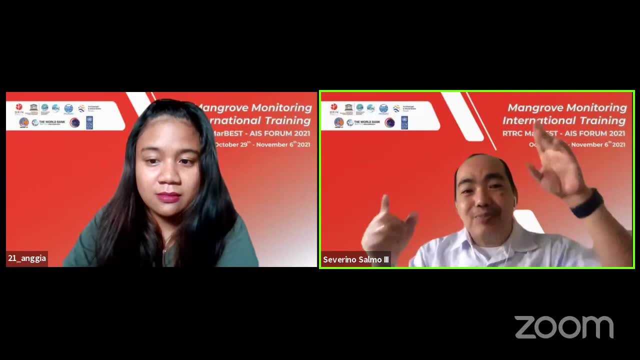 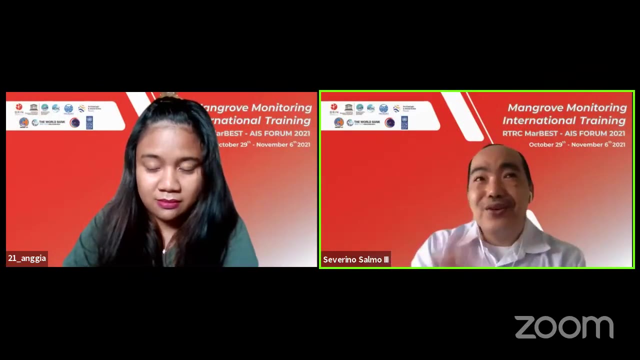 especially if you see holes. that means the models are eating or feeding the. the mangrove leaves and you know it will not stay there, because molus has to store the food. they have to go deep to store their food so that, uh, when there's these uh limitations in food, they have. 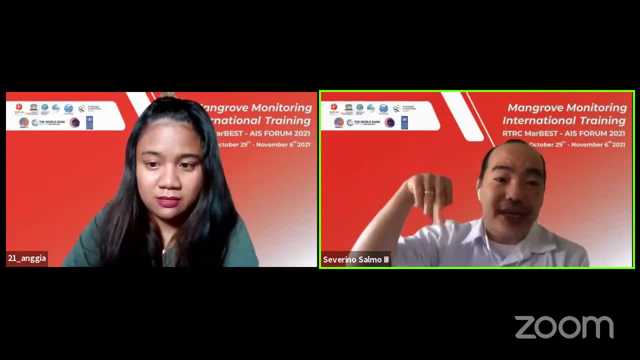 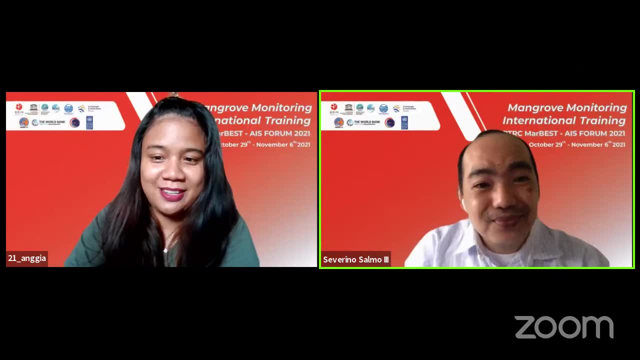 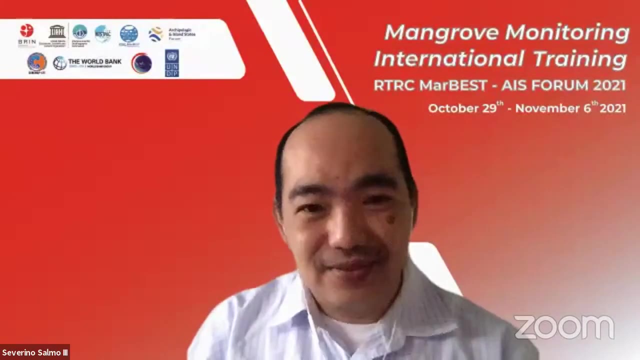 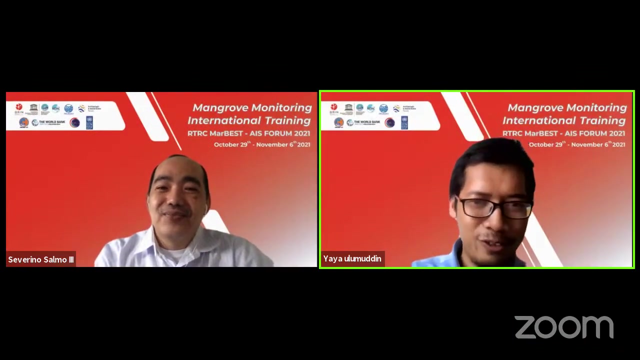 a reserve, and when they do that, they borrow inside the sediment and that will enhance organic matter accumulation. so that's good, okay, and so thank you, yeah, all right, oh, is there any questions? we still have? uh, about nine minutes, so, seth you, you, you. you have plenty of time for talk, for discussions and discussions- very fruitful. 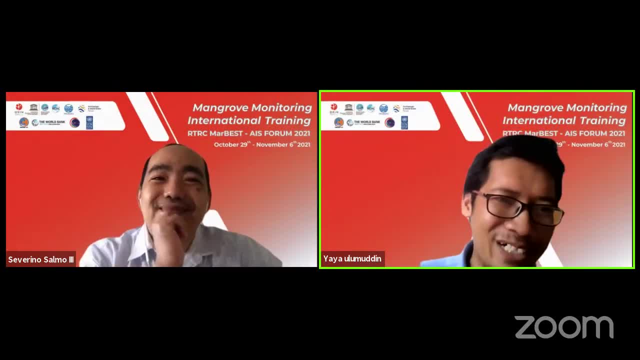 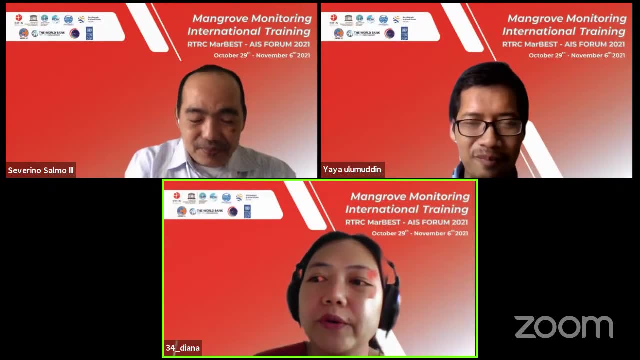 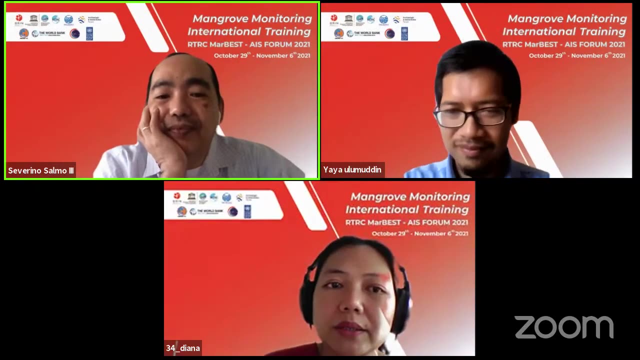 yeah, yeah, oh, diana, please, you still have a question, please, continuing the question from angia. for the seedling, the mangrove seedling leaf eaten by the molas, can it cause the death of the seedling and cause the the low rate of success? yeah, uh, not much with molars. if you're referring to the general, 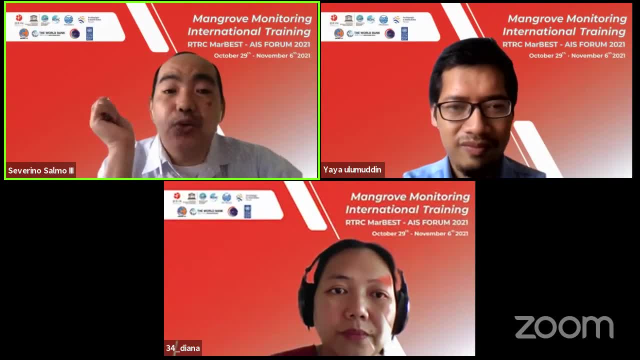 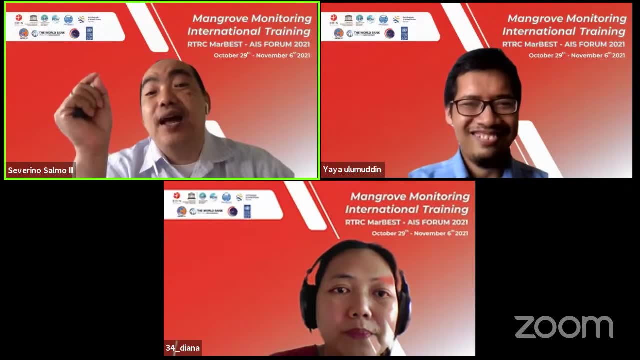 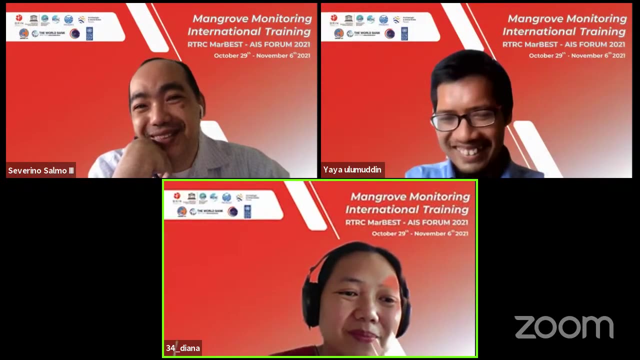 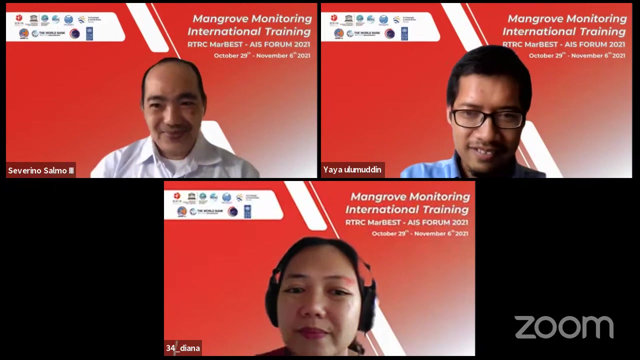 seedling growth and survival. but it would be the crabs, especially the uka species, they, you know, once they, once they bite the, the propagules, it's really fatal. yes, okay, yeah, thank you, okay, goodbye, oh, thank you, yeah, uh, yeah, uh, recently i, i. 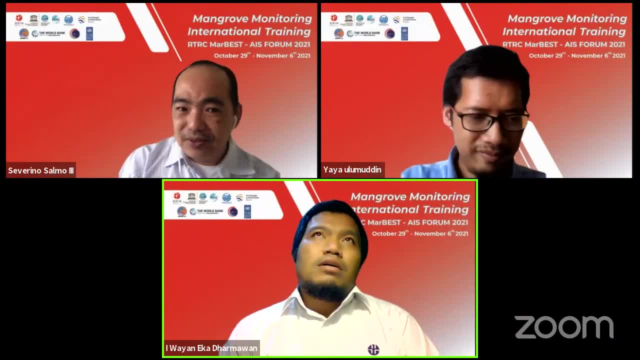 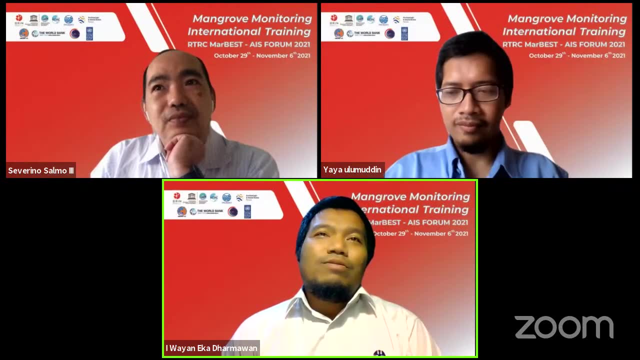 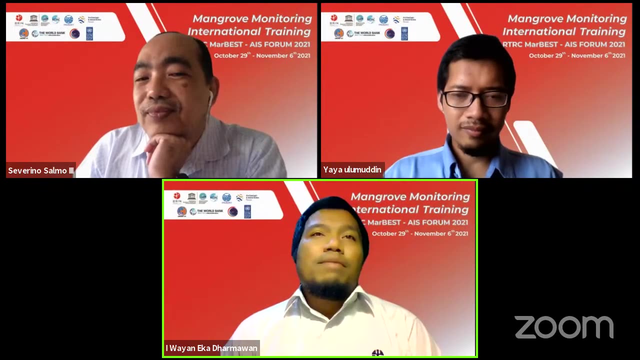 as i have studied about the mangrove health index in indonesia related to uh, with dr yaya also and also our team in this example for oceanography. we, we took a lot of sample also. it's maybe uh, but less than 10 000. we, we took a lot of sample also. it's maybe uh, but less than 10 000. 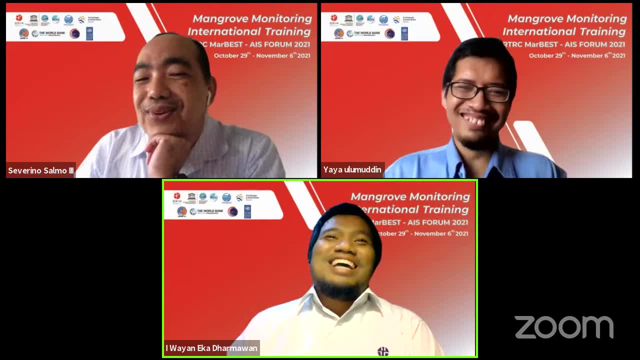 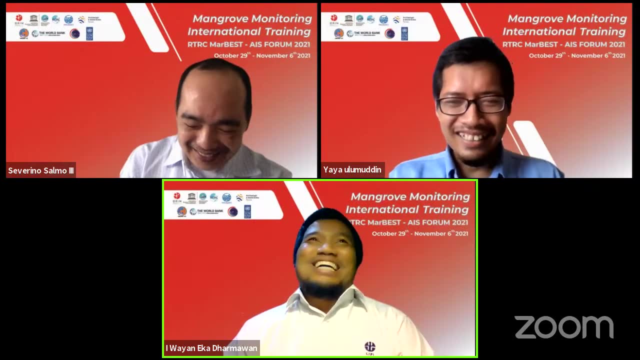 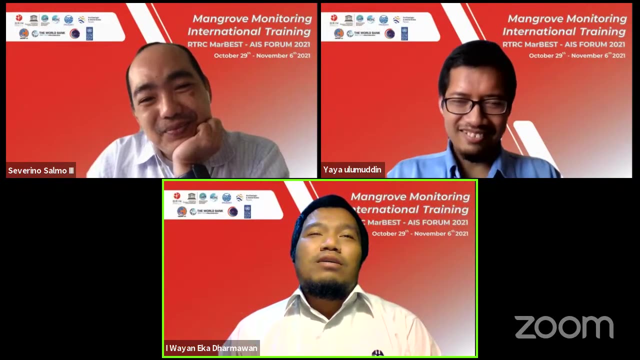 we, we took a lot of sample also. it's maybe uh, but less than 10 000, because i, i didn't read when i heard that 10 000 molas. oh my god, that's why i hired some we. yeah, we hired some students to uh, to do uh simple things, so that i, we didn't do that later. 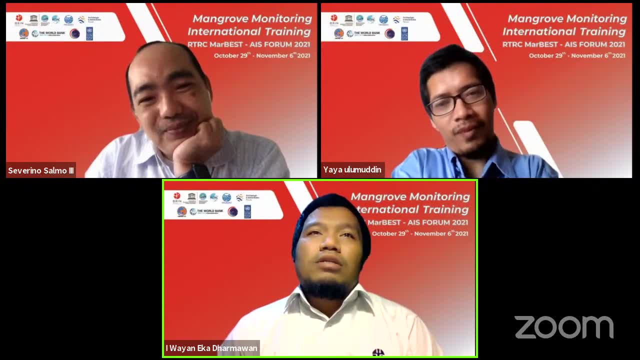 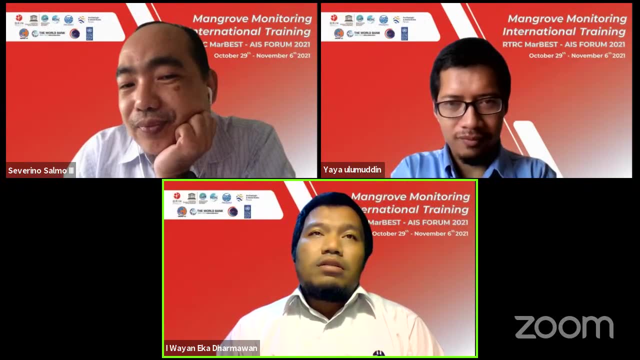 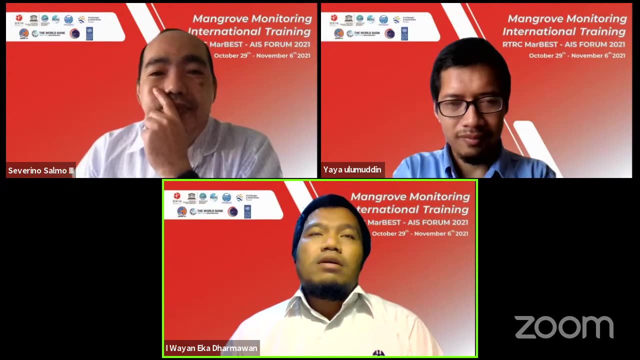 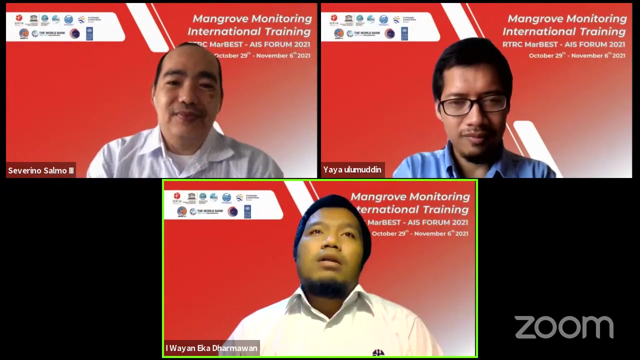 uh, but i have some confusing here. maybe you need your suggestion. uh, like, uh, we, we studied some area, different, different types of area, maybe one exploring a big, large river and the other one is a small island, but all of them has a great number of mh high the health, health you know. 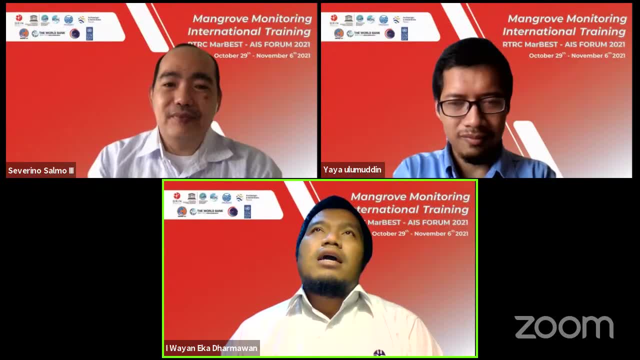 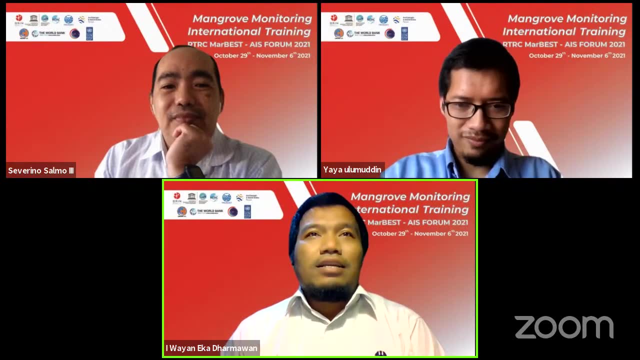 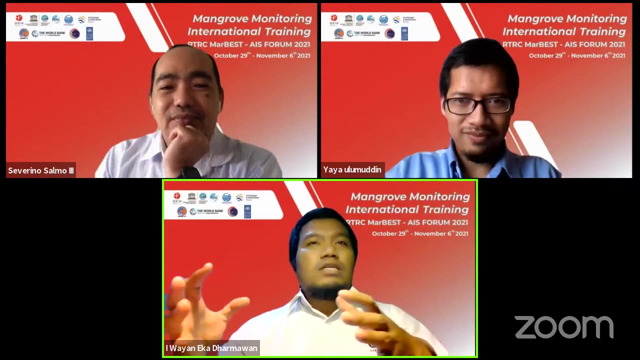 is quite good, great, great uh is. i think we can classify that in a 15 condition. maybe, like you say, maybe that is a reference side, but among, among the condition of the island, of the geomorphological setting of the, the of our, our study is different of uh, the diversity of 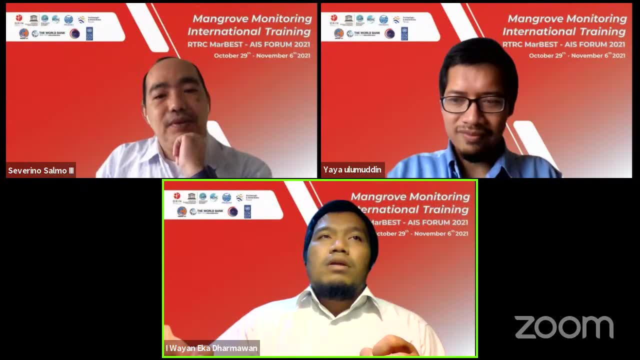 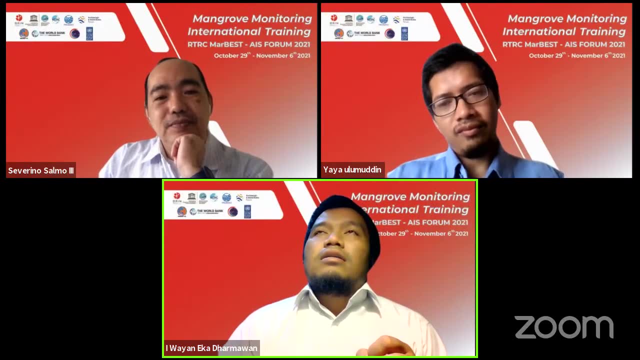 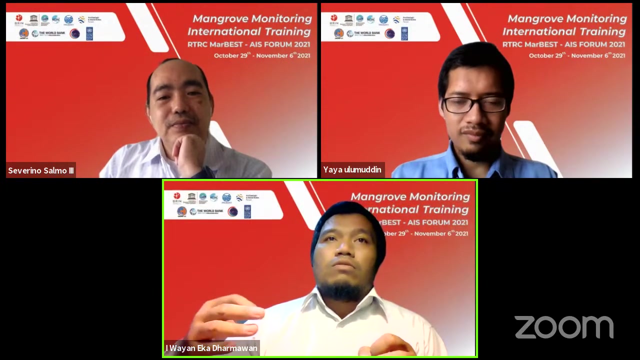 yeah, maybe, maybe do you have any suggestions, like in papua, in a small island in papua, in biak, the. the geomorphology of this island is a in the lagoon. in the lagoon because because of the pacific, uh, pacific, uh- wave is quite strong, so a mangrove hiding in the, in the 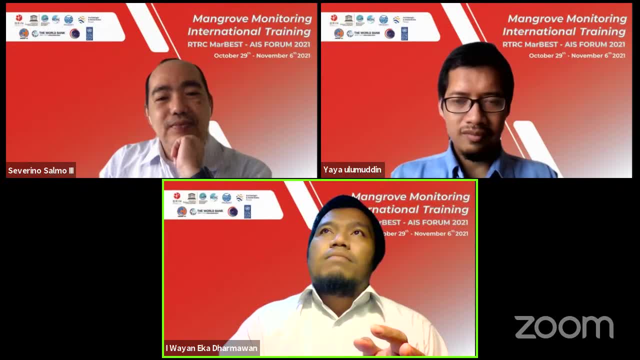 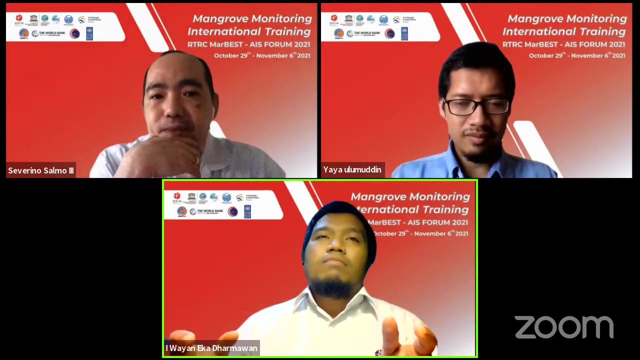 lagoon and one of the the other side is in the merauke. merauke is a big historian and uh a silky, uh mangrove, uh soil, but uh, both of them uh is uh quite uh in a good condition, in a pristine condition, but the, the diversity and abundance of the molasa, it's so different, yes even. 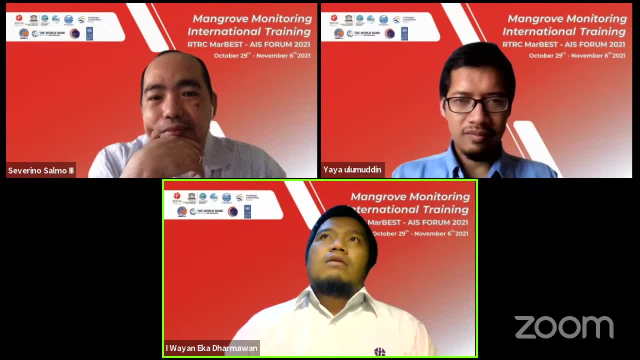 in 10 square, 10 meters of the area, trees, or in fauna or every fauna, but when, when we move to the merauke, there is a lot of molasses. yeah, maybe do you have any suggestion. uh, how could we do about this? because the msi, the 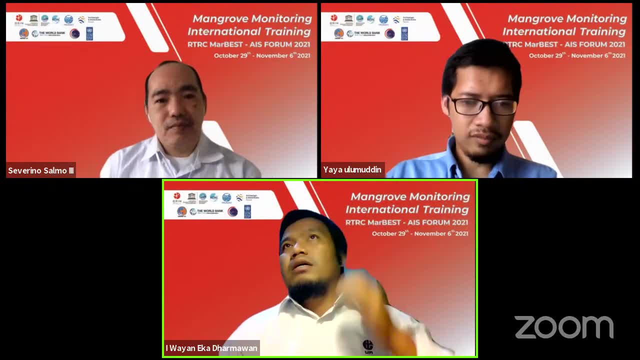 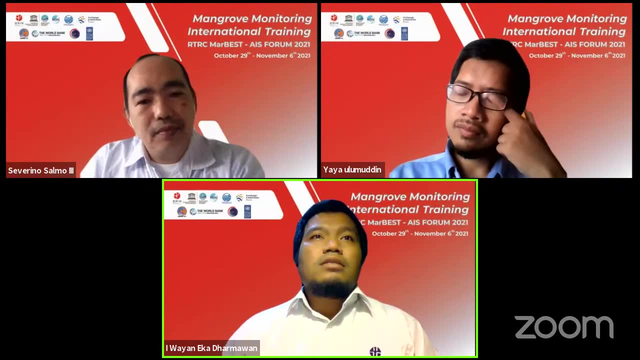 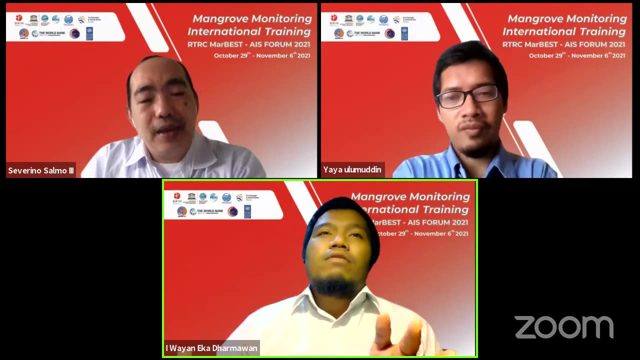 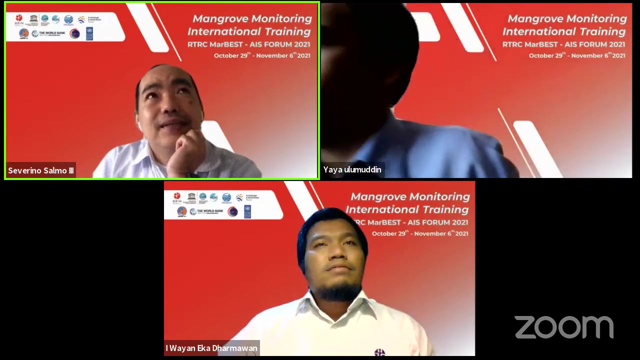 mangrove index, or maybe, maybe i have some. uh i wonder, i wonder in depth, uh, it's kind of geomorphological setting. has uh, has the maximum uh number, maximum diversity of the molasses? maybe, maybe, yeah, do you have anything? uh nothing. well, what i can say is that nothing: 100 uh guarantee. 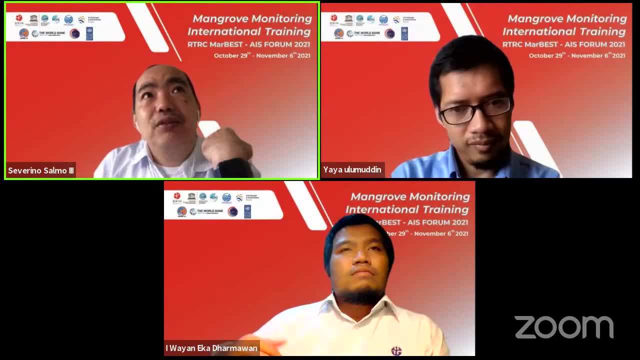 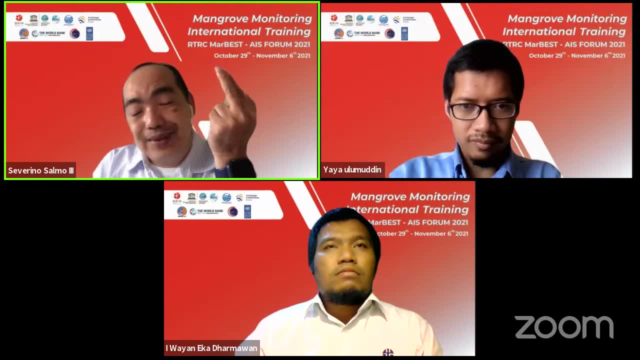 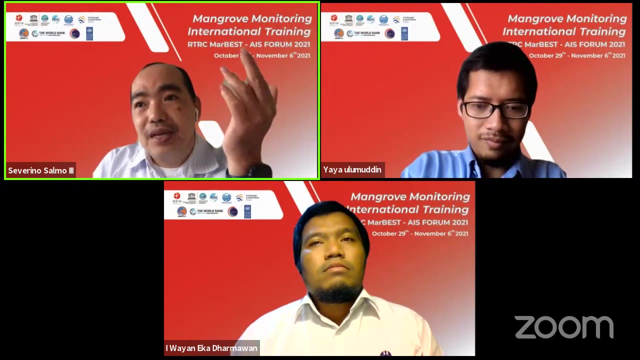 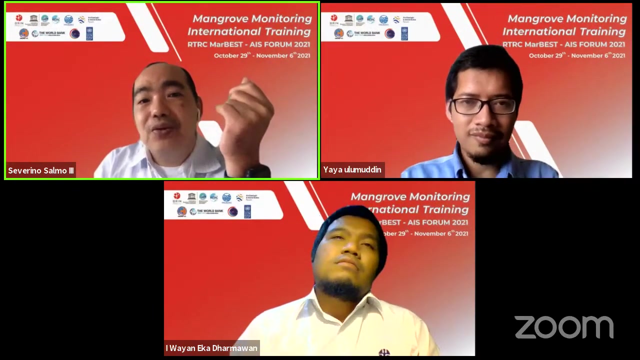 to answer your question. but you know, i i started my talk about the definition of concepts, what really is a restoration, and it's could be ecological or ecosystem, uh, restoration. the other thing is about the uh, the establishment of a reference system, that's. that's the reason why i don't really use 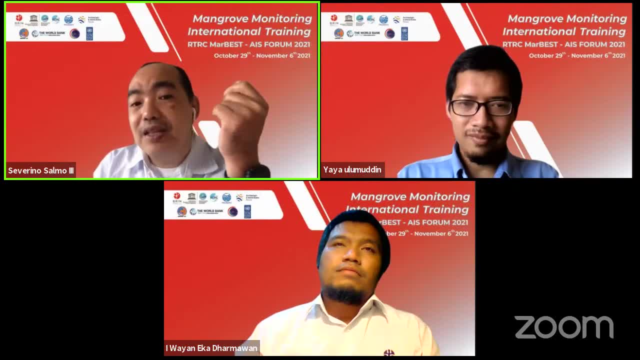 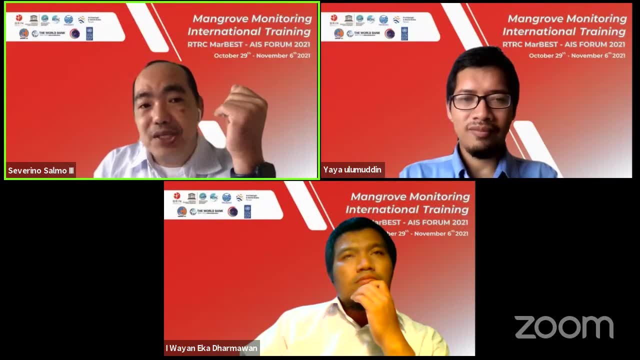 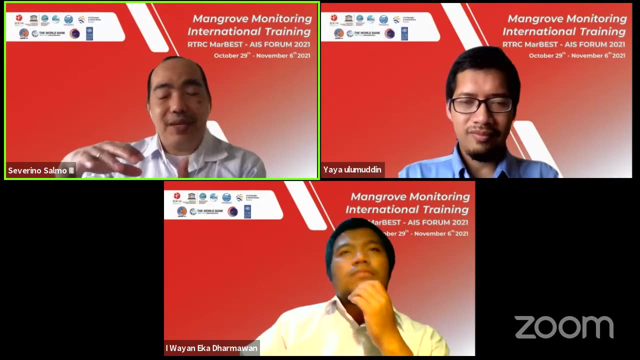 abundance and biomass, it will really be very difficult. i'm more interested to see the ship, the chains in the species composition, the chains in dominant species. or you raise theonoche, email the hom��, or if you have a healthy system and you have, let's say, 10 species in a reference system and it it's not changing, it's always, then 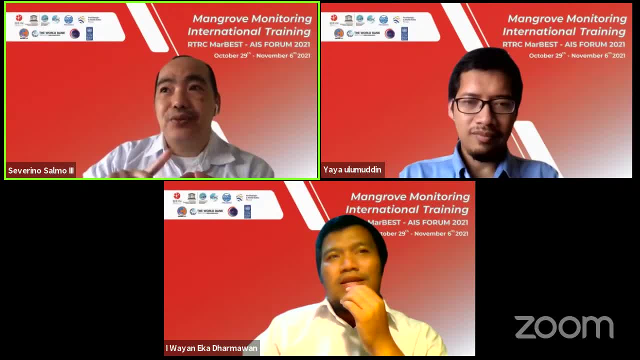 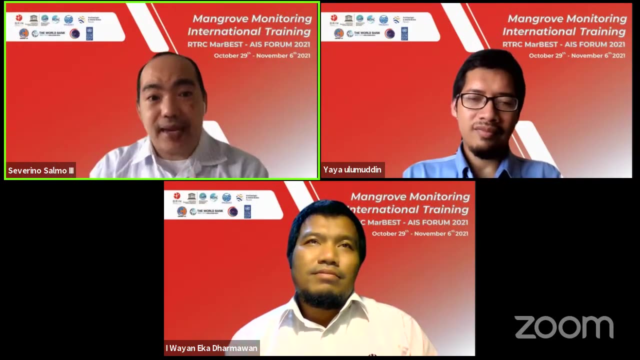 right, then i can say: but i need to, i need to assess: are this species pioneer species or mangrove dependent species? and if the mangrove dependent species are not changing, even though there are only 10, then i would say it's like 10.. specificek. 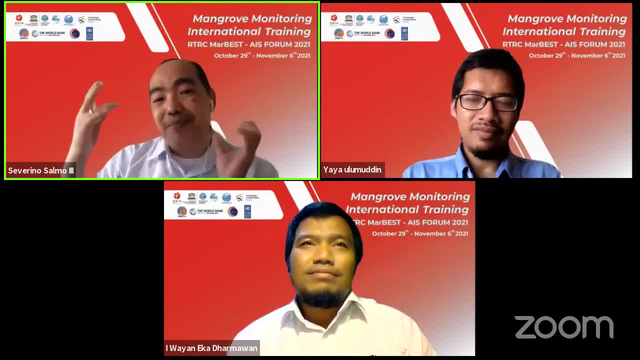 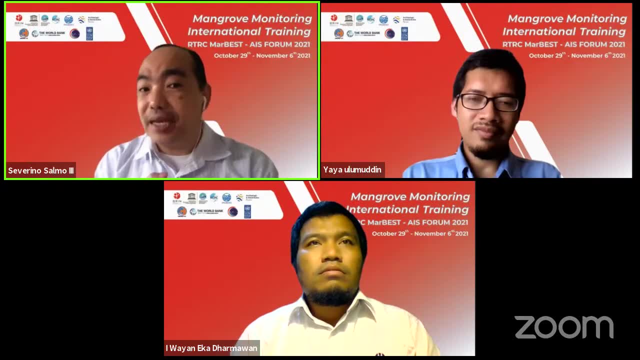 which is it does so much better, but maybe even if 70 percent oforde does so, but we wouldn't change that would say it's really healthy. but if i have a mangroves that have more than 100 species, but 99 species are pioneer species, 99 species and only one that is mangrove dependent species. 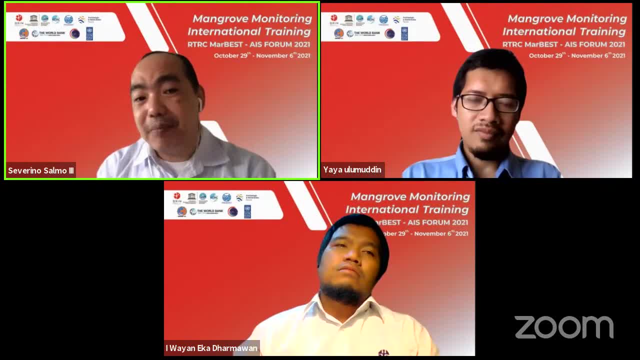 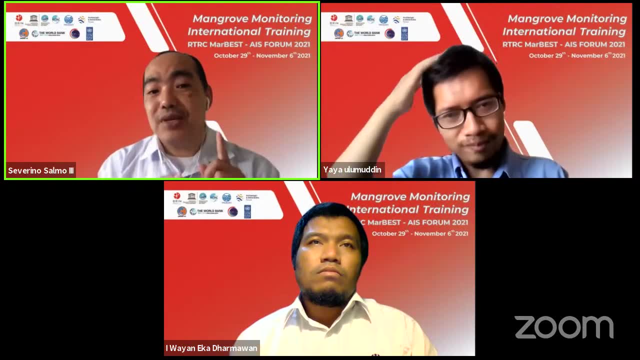 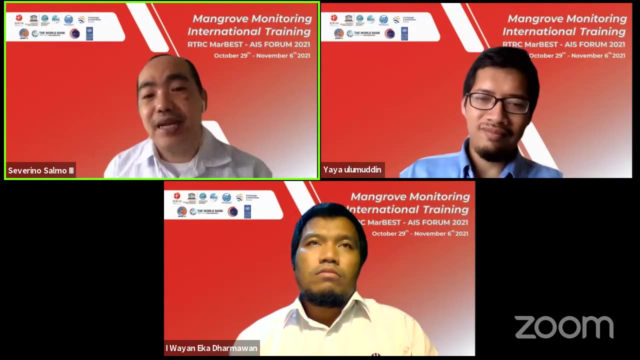 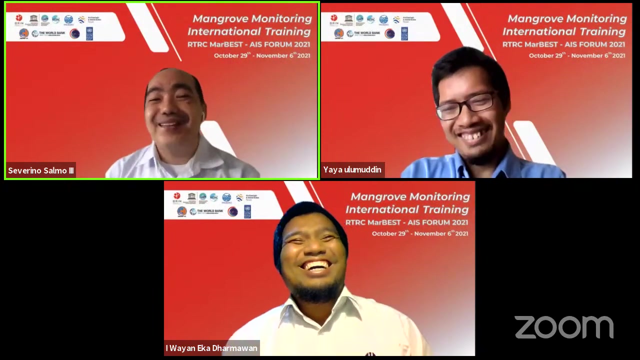 then i would say, even if it's healthy, then the diversity is not supported. again, my suggestion, my suggestion: before we have to document the restoration indicators and restoration trajectory that change over time and that's not easy to do. yes, yeah, yeah, yeah and uh, please update me with your, uh, with your monitoring. yeah, yeah, yeah, but in in. 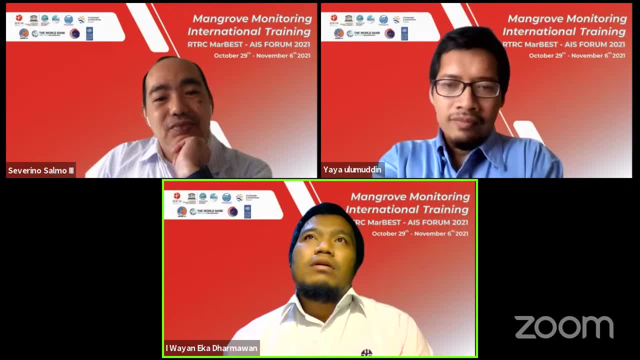 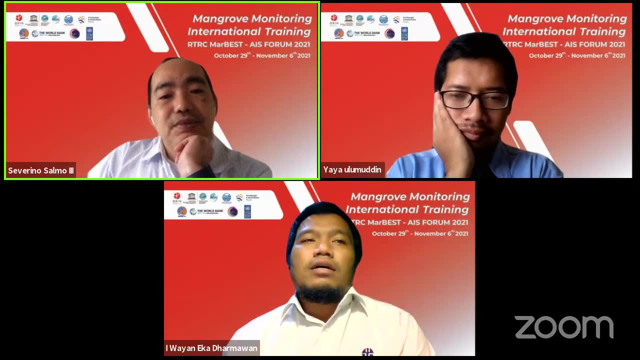 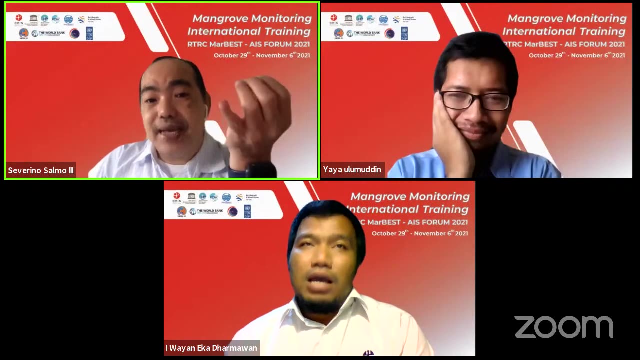 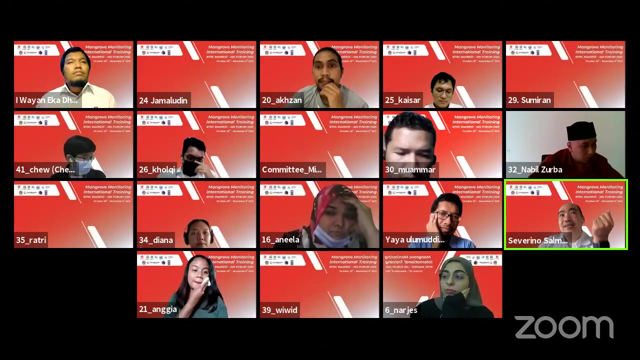 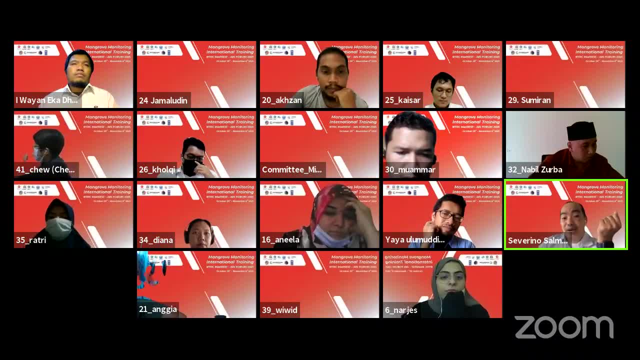 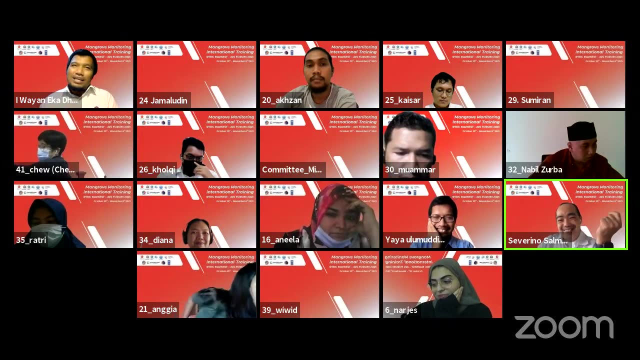 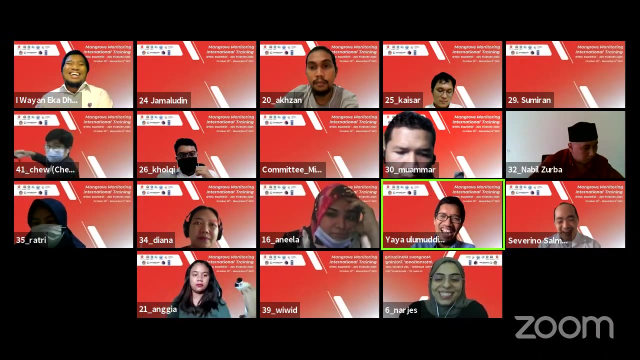 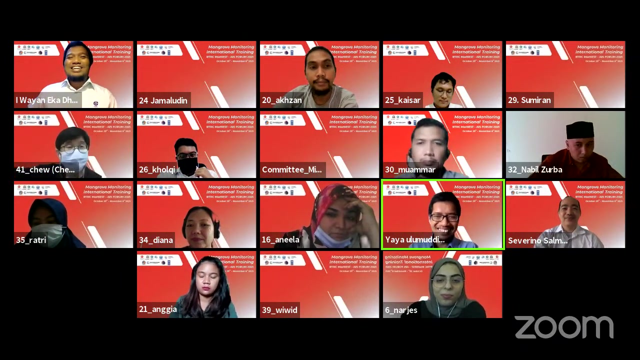 we're doing is attributed to the restoration program. that's the reason why we have to establish what is a reference system and please remember restoration indicator and restoration trajectory and restoration trajectory. yeah, okay, thank you, sure, i'm sorry for the participants. i also asked, i think i think so, but this is probably have enough time for uh discussions. 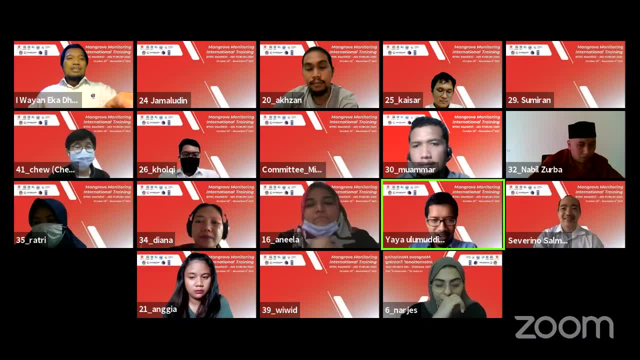 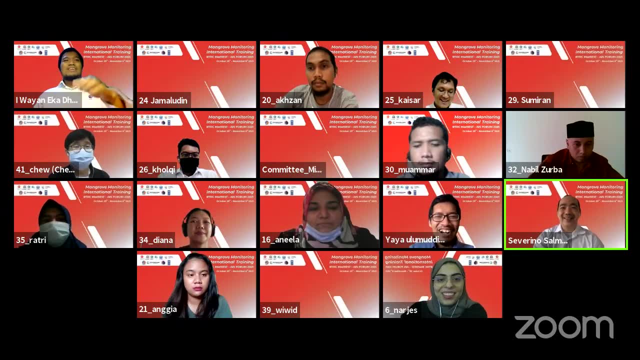 okay, uh, it's a 329, but actually, uh, oh, oh, steph, you are still there. i thought you already wait. okay, uh, it's a 329, but actually, uh, oh, oh, steph, you are still there. i thought you already wait. okay, um yep, confident. 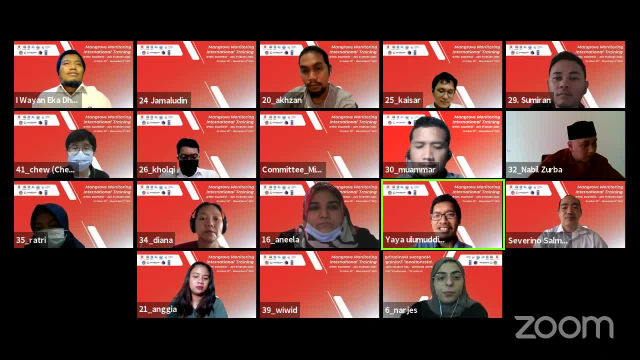 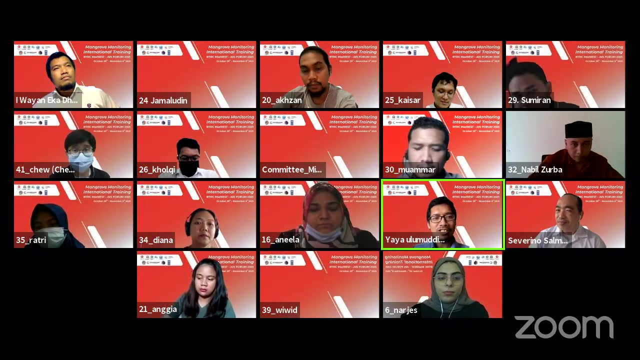 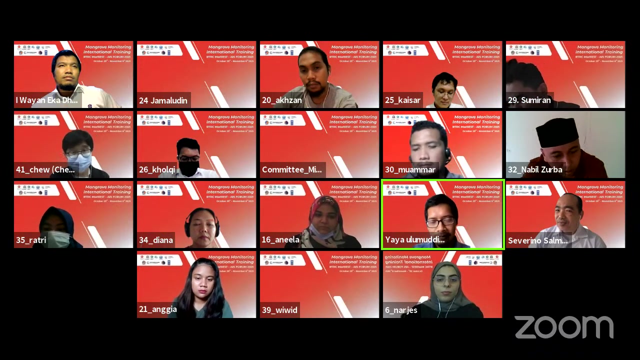 uh, yeah, it's awesome. so then, from here, focused on Okay, um, wow, okay, um, so, um, yeah, yes, i think, uh, you also, what is your class brewing nuo? on the active environment also, or any defining uh, which the that uh, uh, pubal, we conceptualize the mangrove health index. 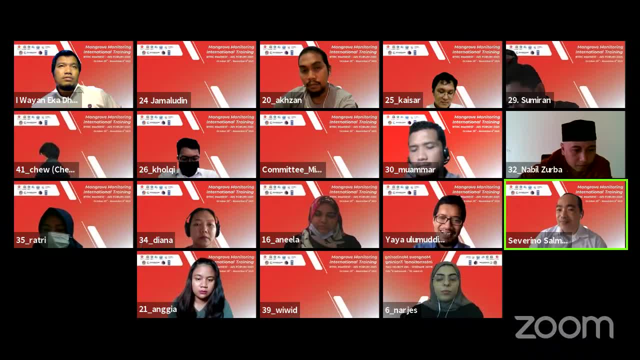 on the structural complexity, as you said, And that's the easiest way for us in Indonesia, rather than to collect all of the data for judging this is health or this is not. I think structural complexity it's enough for doing that. yeah. 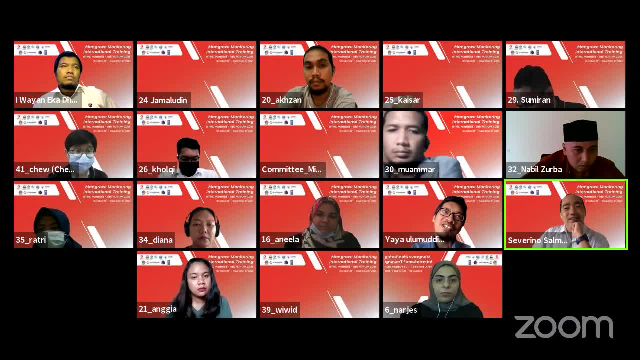 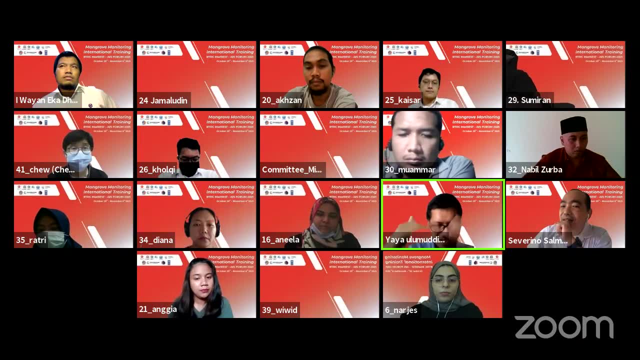 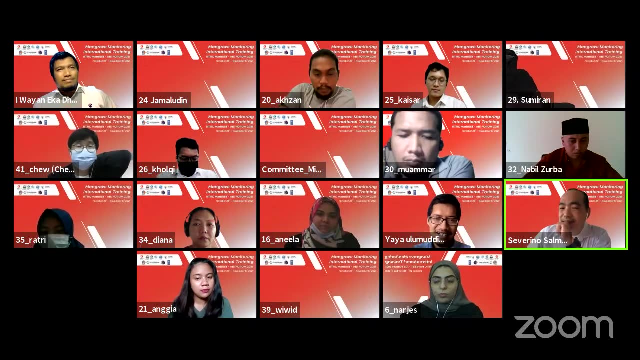 Yeah, yeah, yeah. And it said the structure. there is a correlation between structure and molasses shifting. yeah, molasses community and also the soil quality. Yeah, That's it. Yeah, so I think in that case we still- what do you call it? 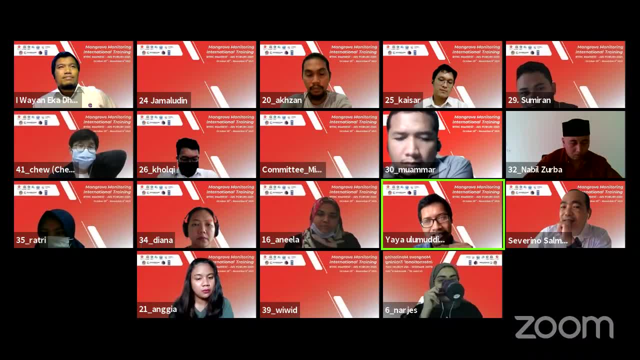 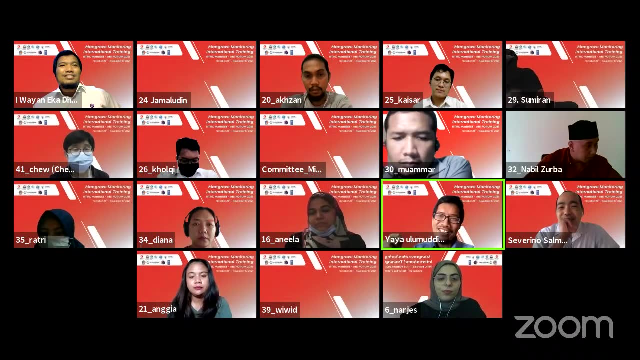 It's still grounded on the theory that we can use structural complexity as the indicators for making decisions. This is a good mangrove and this is a bad mangrove. is that right? Yeah, But still, in our situations, we, still, we have to make sure. 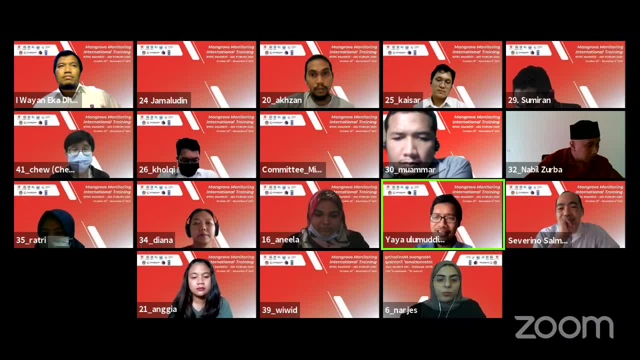 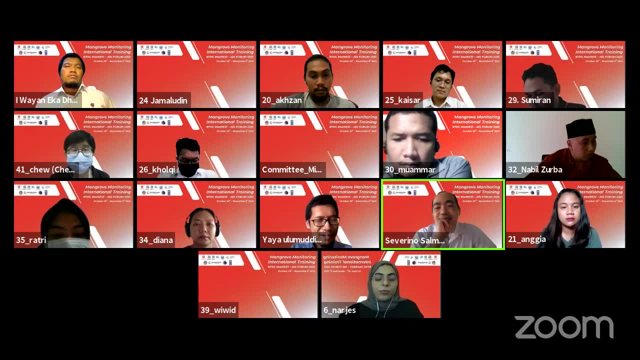 as Wayan said, sometimes in good in health mangrove we cannot find any molasses or something like that. Yes, yes, Yeah, yeah, yeah, But that's thank you very much for you. Sure sure, My job is already done. 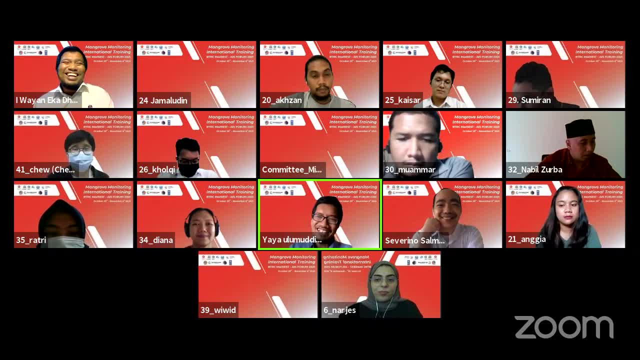 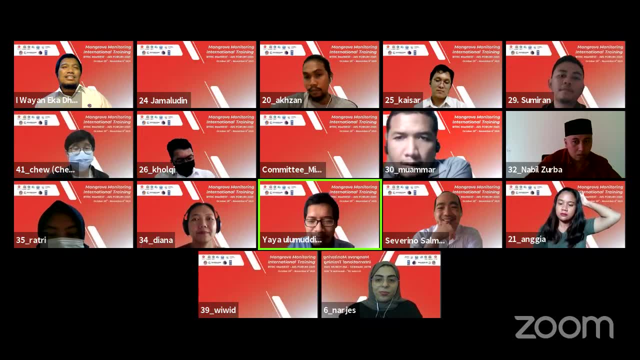 It's health job is already done by you, And then later in Saturday we can discuss more. Yeah, yeah, My assistance. Okay, Do you have last words? closing words for this session please? Oh well, aside from the group. 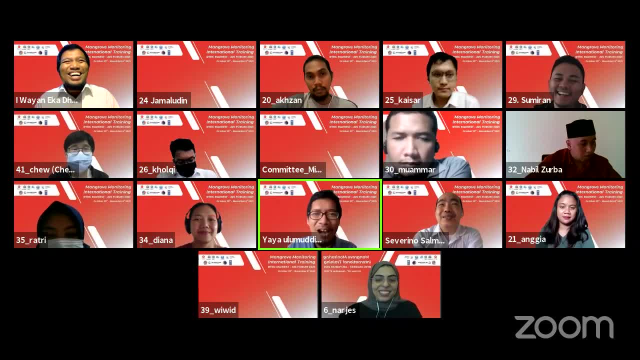 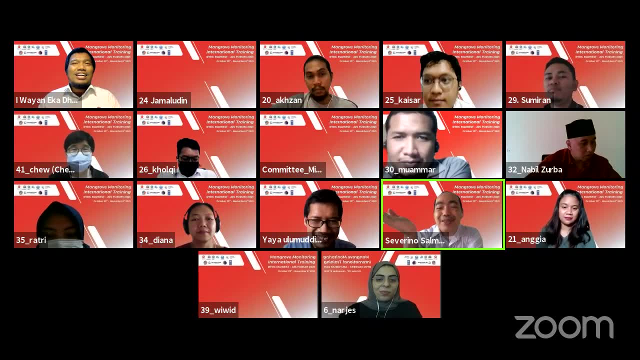 I'll give you a photo later, Okay, Okay, So after after you, you're closing your word. Yeah, Yeah, I enjoyed having the talk with you guys. I see the enthusiasm with the participants And, again, I love the mangroves. 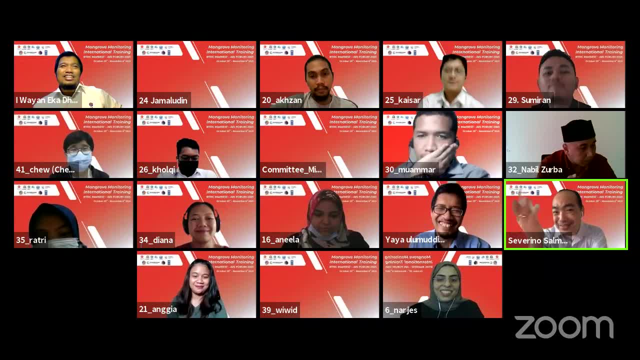 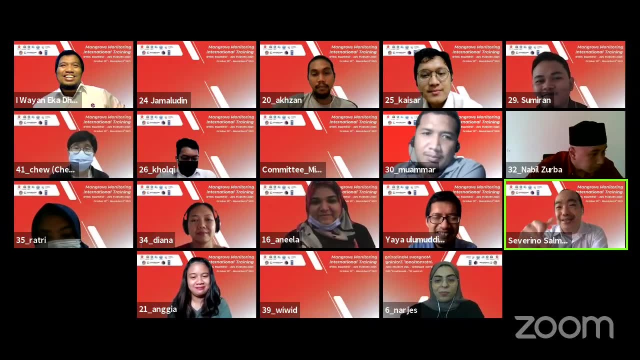 I love the smell of the sediment. You know the the sulfide thing, it's really good. And I love the biodiversity thing. But what I love most is when I see young guys like like you guys, Not Yaya, the younger guys. 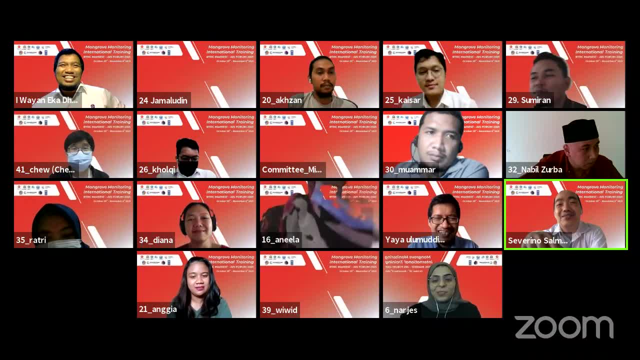 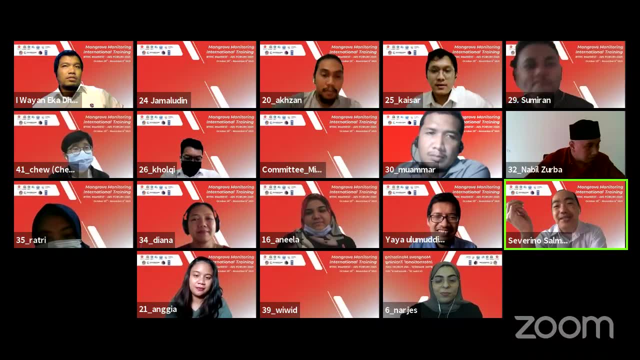 When I see young guys that are interested in mangroves that somehow the future is bright. We will see each other, maybe virtually, in 2030.. You and I will ask each other: what have we done in 2021? And, I hope, by 2030,. 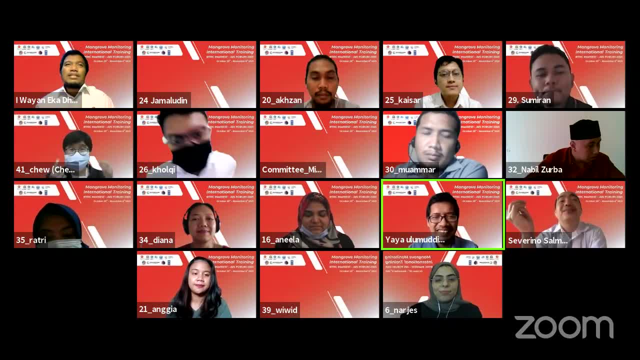 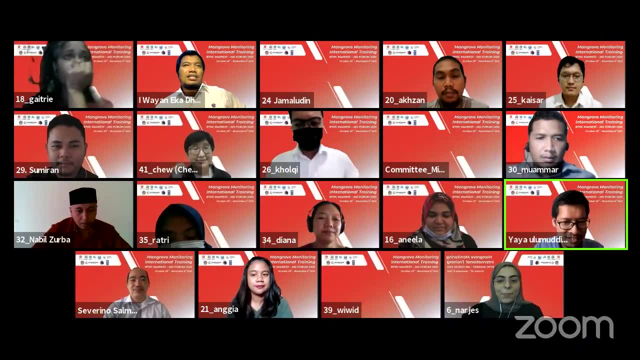 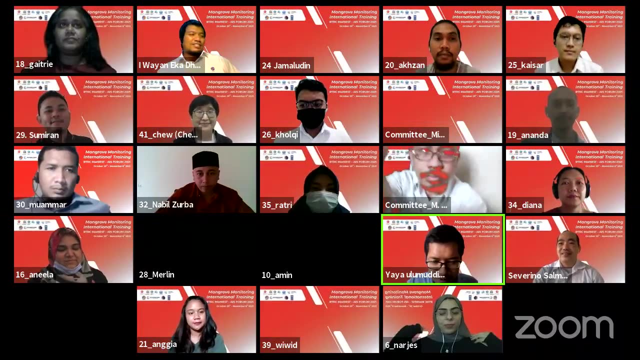 we have a better world to live in, Right? Thank you so much. Thank you. Thank you again. That is the last sessions, the last four decisions, And we will have a photo group. So, Pak Yunus Yaya, please send me the photo. 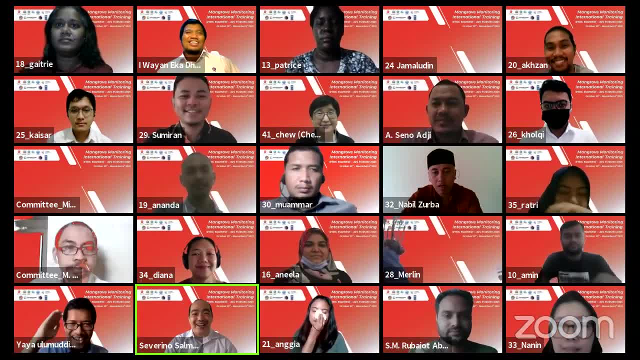 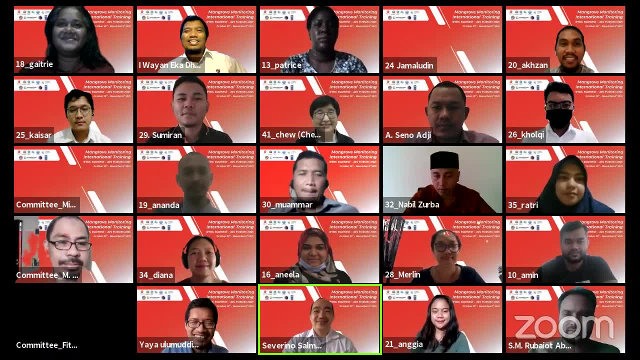 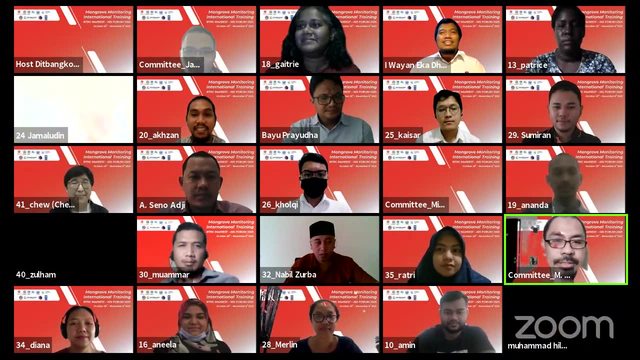 And the manual for the GEE. I will try to learn. Okay, I will too. Okay, Well, Pak Yaya Yep, We are going to have photo session. Pak Tribu, please help Take the shots, Okay. 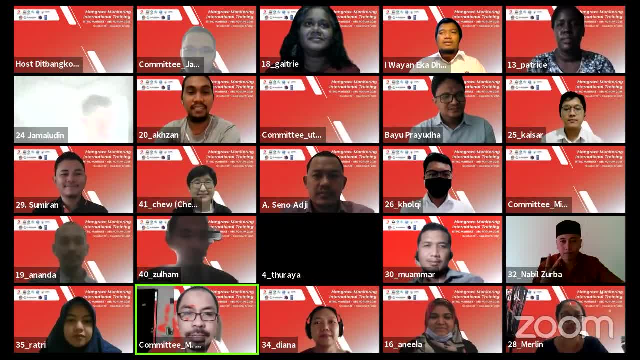 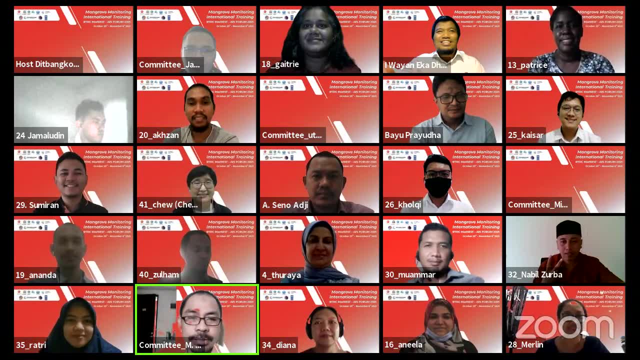 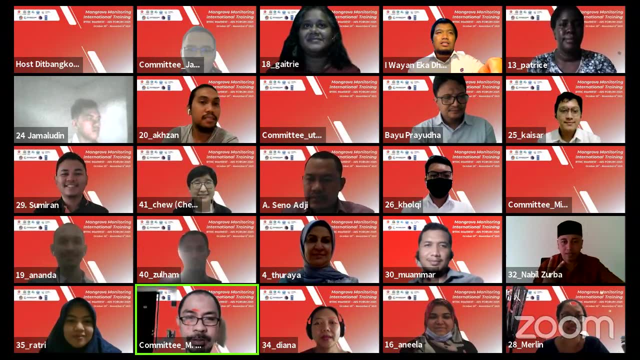 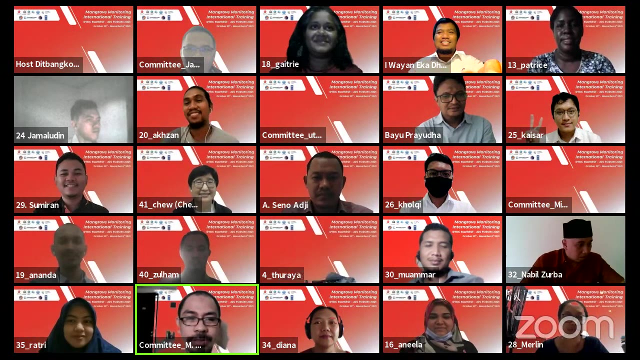 For page one, First, Second, Okay. Page one: One, Two, Three, Okay. Next: Page two: No One, Two, Three, Okay. Thank you very much, Thank you, Thank you very much, Thank you. 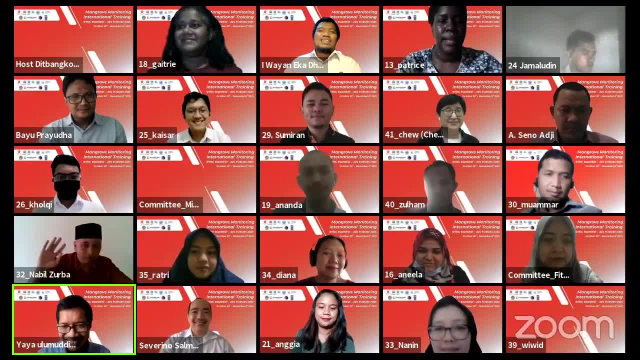 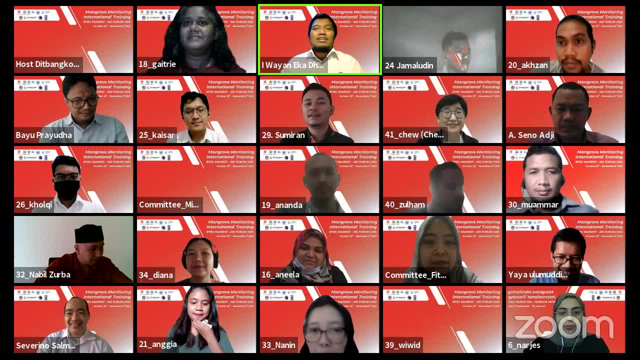 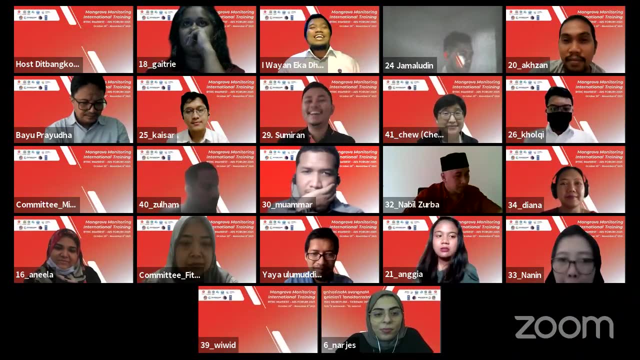 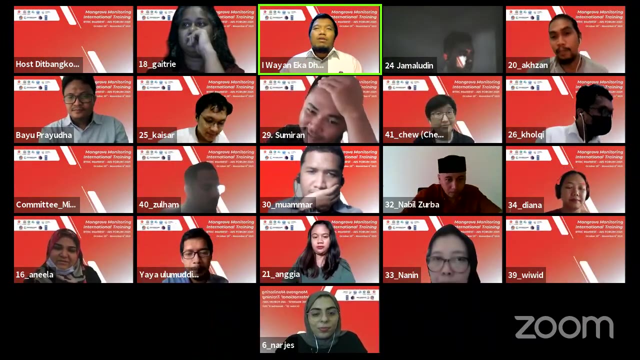 Thank you, Thank you everybody. Thank you, Bye-bye, Bye, Sure, See you next time, Okay, So Thank you. Thank you, Yeah, Okay, This is the end of this session today. Maybe all of you should.